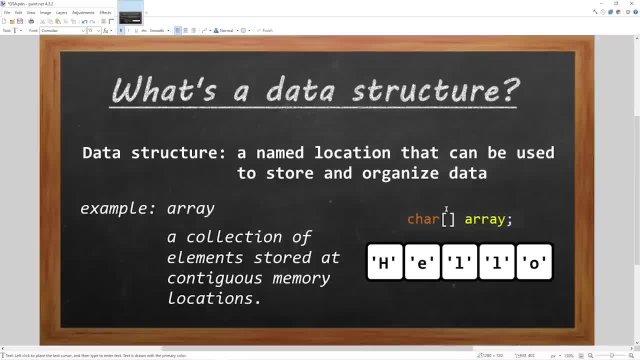 this data? A tree is a data structure. What about arrays? We have a little bit of experience with those. An array? An array is a collection of elements stored at contiguous memory locations. That's another example of a data structure. It's basically a named location that can be used to store and organize. 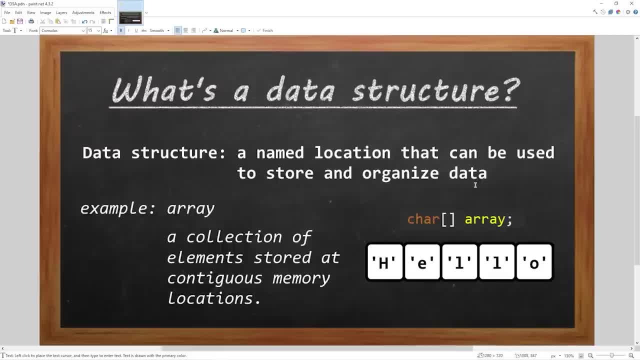 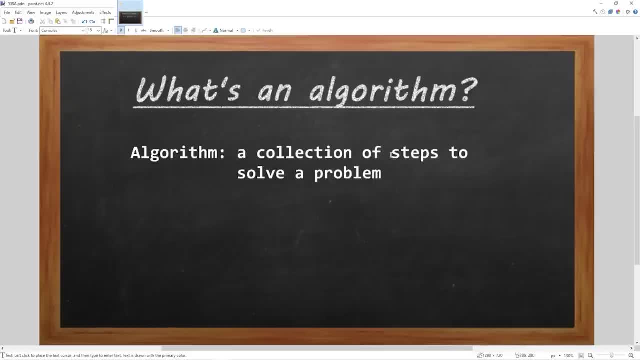 data. Different data structures store and organize data in different ways. Each of them has their own pros and cons. Well, what's an algorithm? An algorithm is a collection of steps to solve a problem. It's the steps to a solution. Here's an example: I'm hungry and I need a pizza. That's my 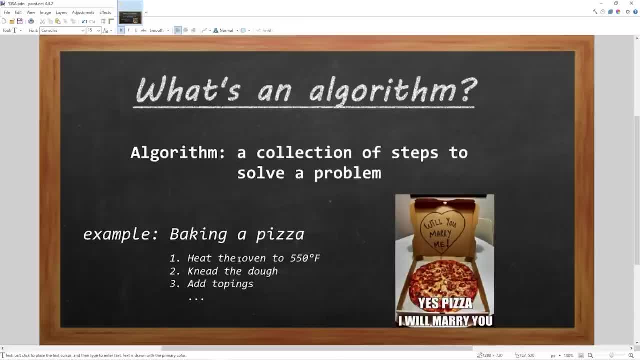 problem. An algorithm to bake a pizza could be: one: heat the oven, two, knead the dough. three, add the toppings and then eventually, you'll solve your problem of not being hungry anymore. So that's a real life example of an algorithm. One algorithm that you're probably familiar with is a linear 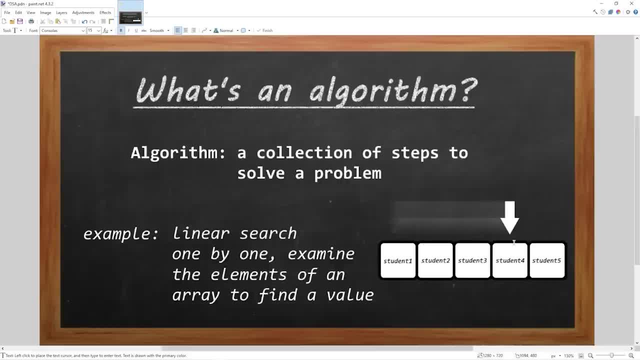 search. Suppose we have an array of elements and I need to find a value. Using a linear search, we would, one by one, examine the elements of an array to find a value. A linear search is an example of a searching algorithm. I know what you're probably thinking. 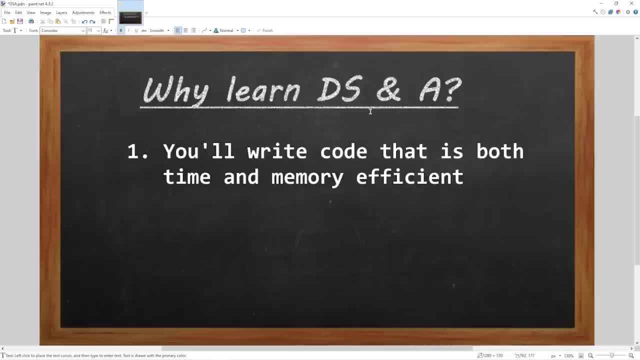 Why do I need to learn data structures and algorithms? What's the point? Well, let me tell you. You'll write code that is both time and memory efficient. And two commonly asked questions involve data structures and algorithms in coding job interviews, Do you? 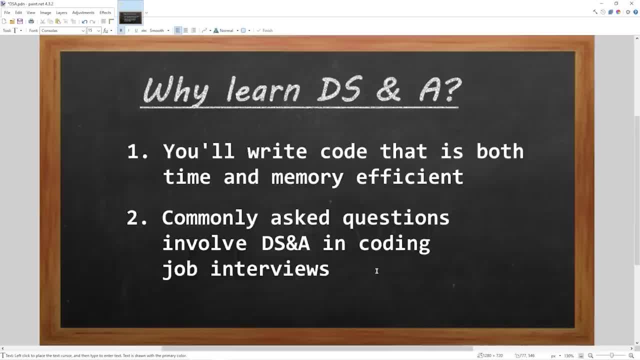 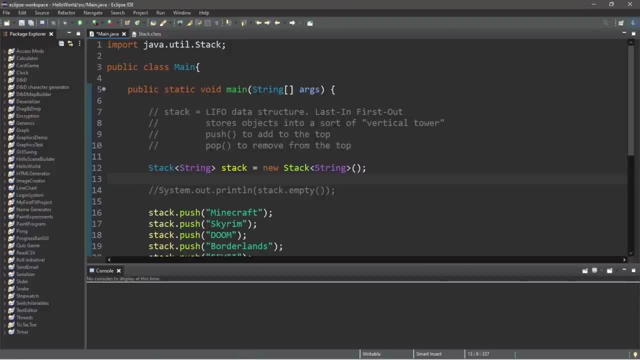 know how to reverse a doubly linked list. No, no, you don't do you. So you should probably watch this series. So, without further ado, ladies and gentlemen, let's begin. Hey, what's going on? everybody, It's your bro. Hope you're doing well In this video. I'm going to 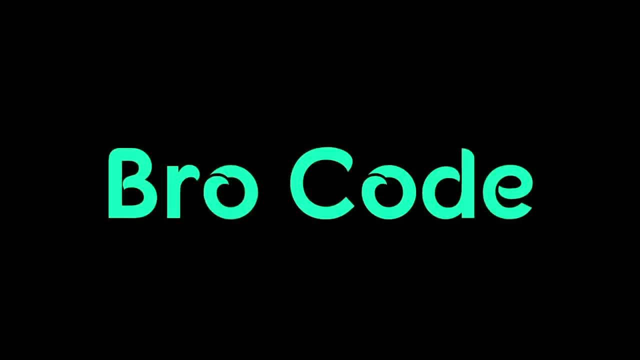 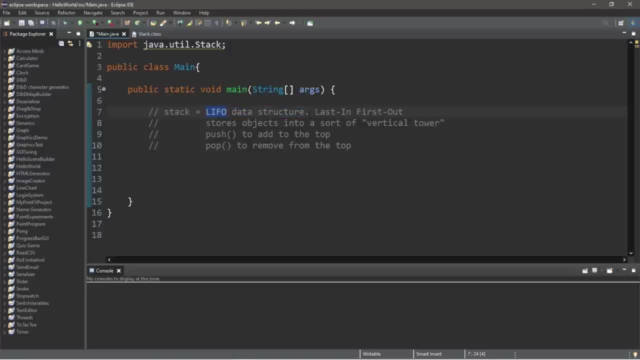 show you how to reverse a doubly linked list. So sit back, relax and enjoy the show. All right, everybody Stacks. A stack is a LIFO data structure. LIFO is an acronym for last in, first out. This allows us to store objects into a sort of vertical tower. 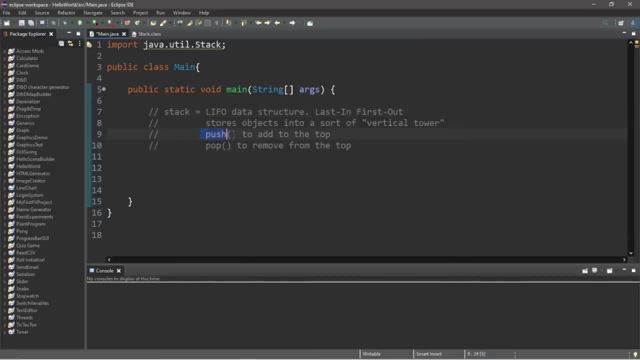 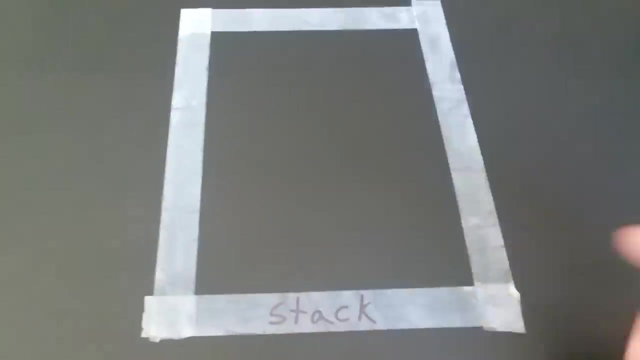 like a stack of books or a stack of CDs. We use the push method to add objects to the top of the stack and the pop method to remove objects from the top. So here's a real life example of us creating a stack data structure. After declaring our stack, we can add objects to our 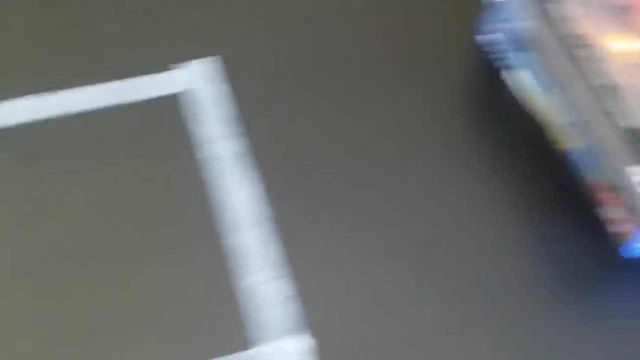 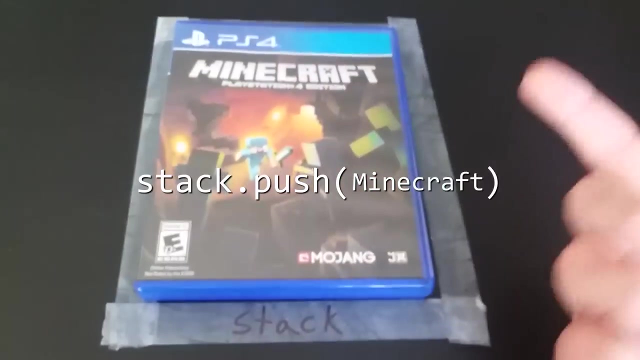 stack. The objects that we'll be adding are various video games. To add an object to our stack, we use the push method, like we're pushing something onto our stack. So let's push Minecraft onto the bottom of our stack And then next we'll add Skyrim, then maybe some Doom. 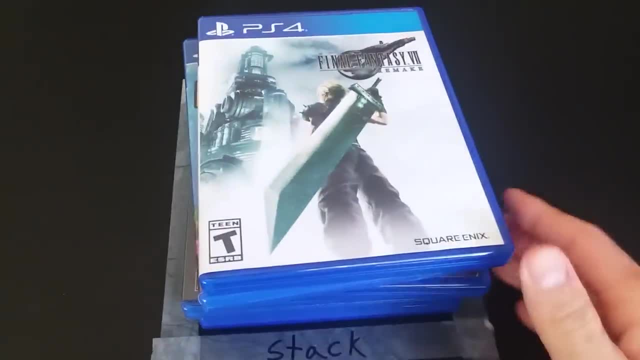 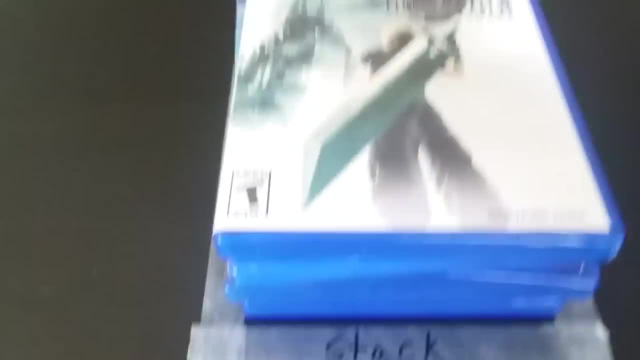 then Borderlands and then Final Fantasy VII. So this is a LIFO data structure. last in, first out. To access objects on the bottom of our stack, we first need to pop or remove objects from the top of our stack. If I need to access Minecraft on the bottom, I don't want to pull. 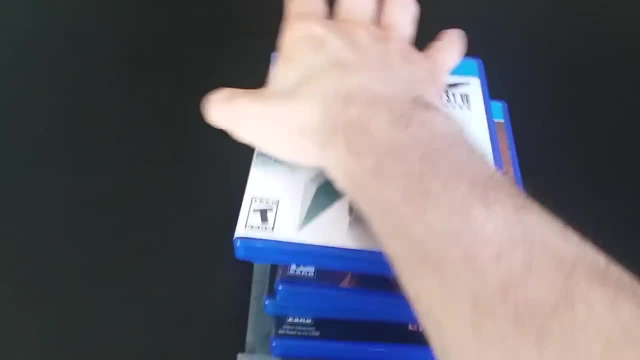 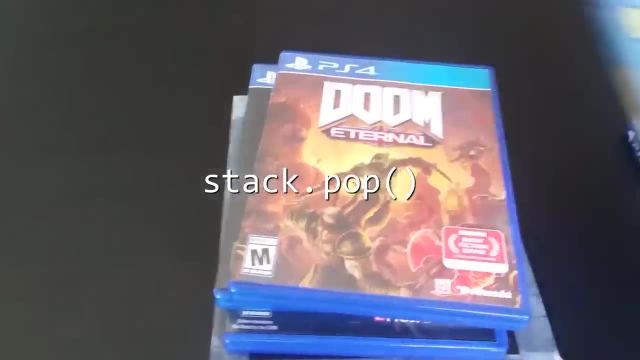 this from the bottom, because everything on the top is going to fall right. So that's kind of the concept. So in order to access Minecraft on the bottom, I need to pop or remove objects from the top in order to access objects on the bottom. So, in order to access Minecraft, I need to remove. 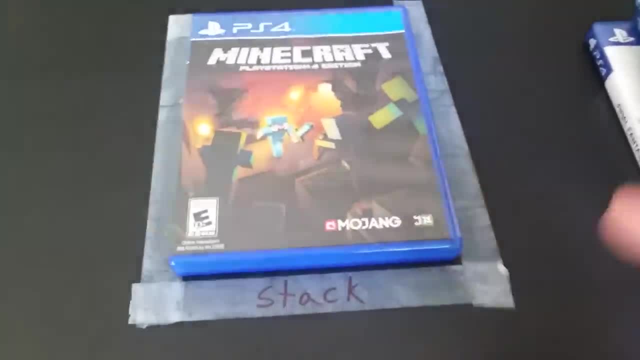 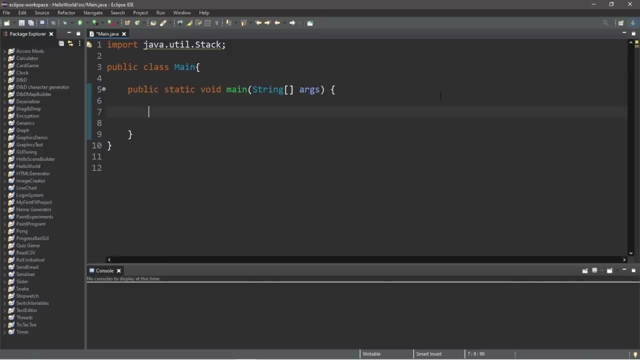 all the games on the top of my stack. So that's kind of the point of a stack data structure. Now let's create a stack. The language you use really doesn't matter. for the most part, You can implement a stack in Java, Python, C++, C, Sharp- The language really? 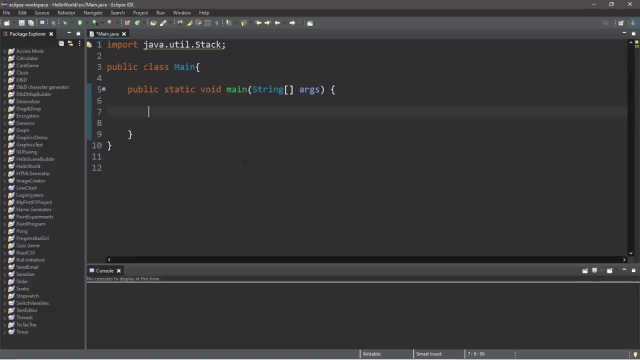 doesn't matter. However, the syntax might be slightly different. I just so happen to be using Java, so I'll stick with that. Now, to push objects onto our stack, we first need to declare our stack and instantiate it. So let's do that Stack. Then we will list the data type of the objects that we 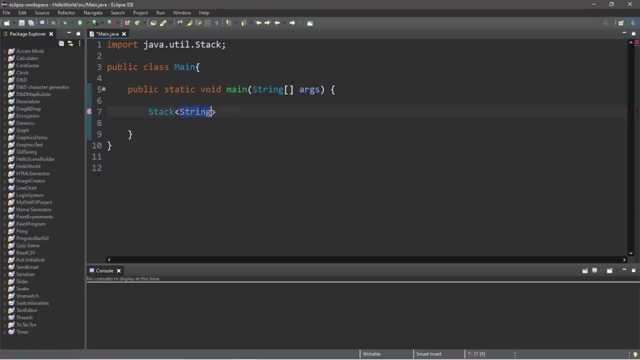 have on our stack. Luckily, strings are a type of object and they're fairly simple, So we will create a stack that can store strings, the names of video games, And I will name the stack stack to keep it simple. Stack stack equals new stack, And I will list the data type and then add a. 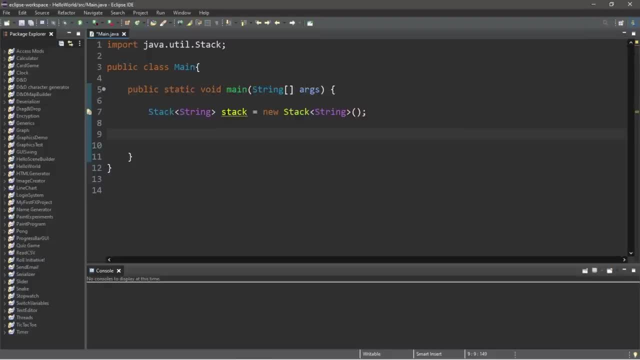 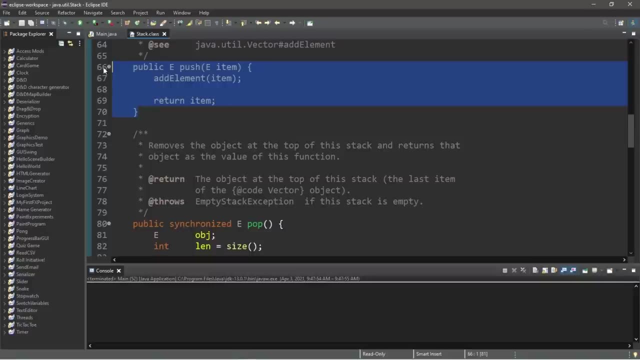 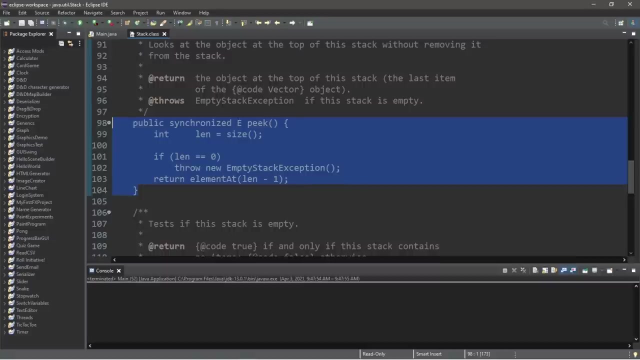 constructor. Okay, so we now have a stack data structure. Now, with stacks, they have five unique methods. Let's take a look Now. with stacks, we can push an item onto the top of our stack. We can pop an item from the top of the stack. We can peek at the item at the top of the stack. We can 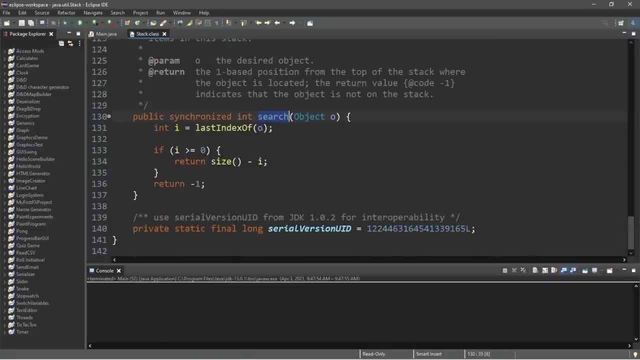 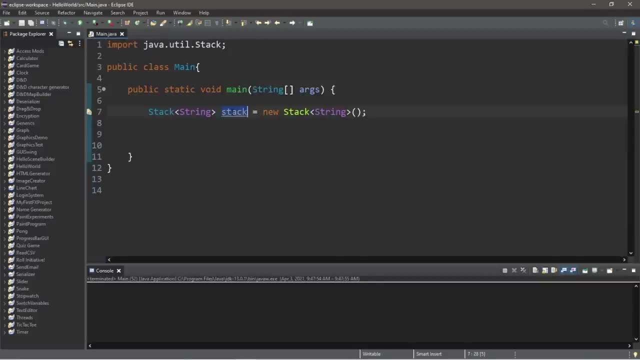 check to see if our stack is empty And we can search our stack for an item. So those are five unique methods available to stacks. Let's first check to see if our stack is empty. So let's use systemoutprintln stackemptymethod. And currently our stack is empty. That is true. 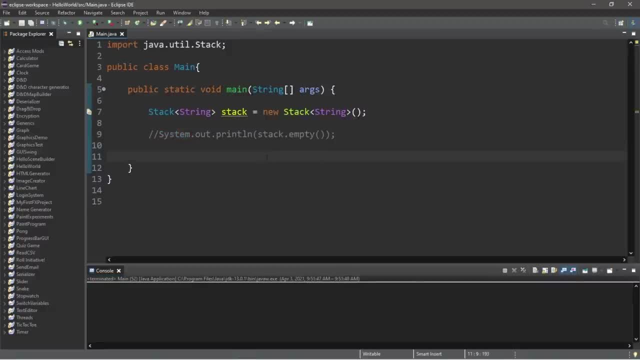 but that'll change soon. So let's push some games onto the top of our stack. So we type the name of our stack, stack and use the push method, then pass in our object. So we will pass in a string the name of a video game. Let's add Minecraft first. Then let's add 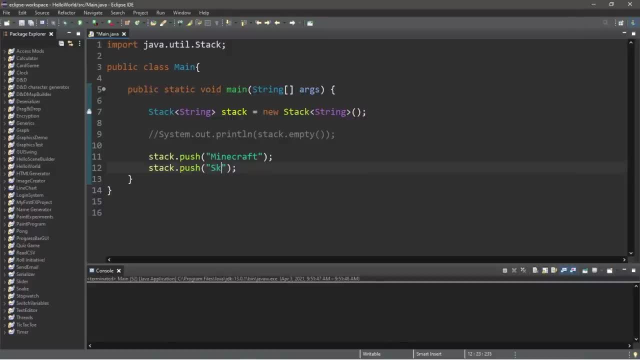 Skyrim, Then Doom. You can pick your own games if you want, I don't care. Then Borderlands And then Final Fantasy VII, FFVII. Okay, let's check to see if our stack is empty now, So let's move. 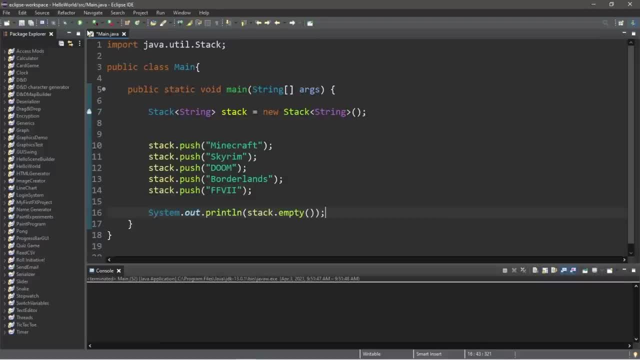 this line of code to the bottom And run it, So our stack is no longer empty. This returns false. So with a stack we can at least take a look at the items within the stack without removing them. So let's use systemoutprintln and I will print my stack. So this will print all of the 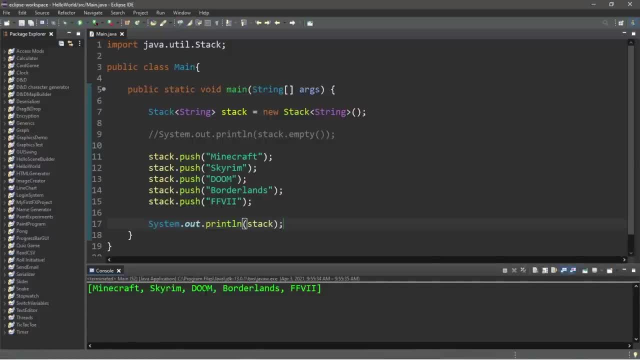 objects within my stack, beginning with Minecraft, then Skyrim, Doom, Borderlands and Final Fantasy VII. However, by printing our stack, we're not removing items from the stack, so that's completely fine. So this time, let's pop the topmost item from our stack by using the. 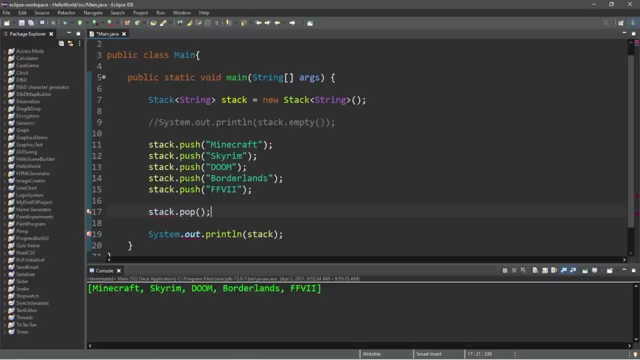 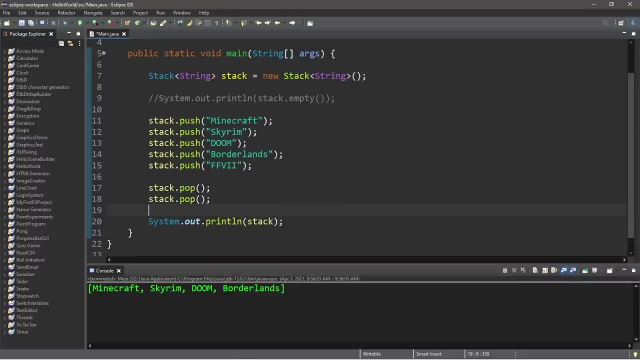 pop method, stackpop, And we don't need to list an object because pop will always remove the topmost object from our stack. So now Final Fantasy will be missing from the stack, So let's repeat this again. Well then, this will remove Borderlands, and then Doom, then Skyrim. 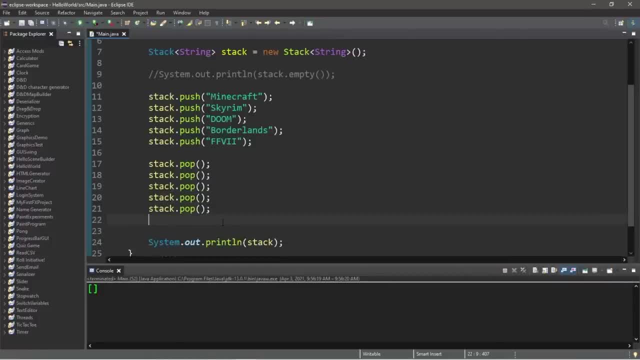 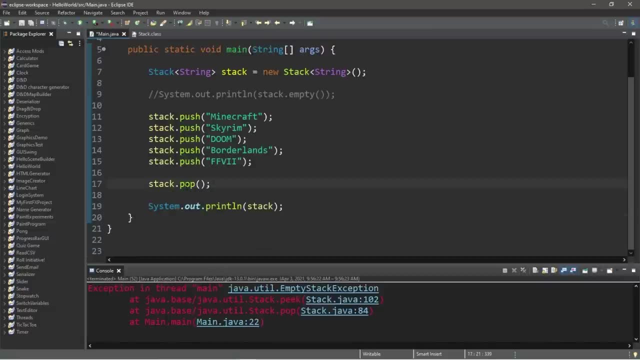 and then, lastly, Minecraft. Then if you pop again, this is what happens: An exception, Empty stack, exception. So that's something to keep in mind. Now, when you pop the topmost object from a stack, this will actually return that object, If you need. 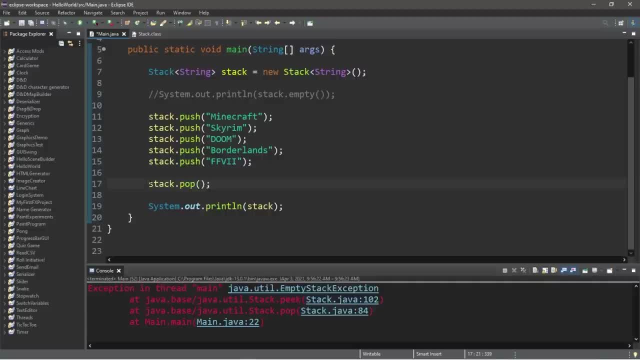 the object from the top of the stack. you can pop it and then assign it to something. So let's say, string my fav game equals stackpop And then I will print my fav game And this will print Final Fantasy VII, And it should be missing from the top of my stack if I was to print my stack. 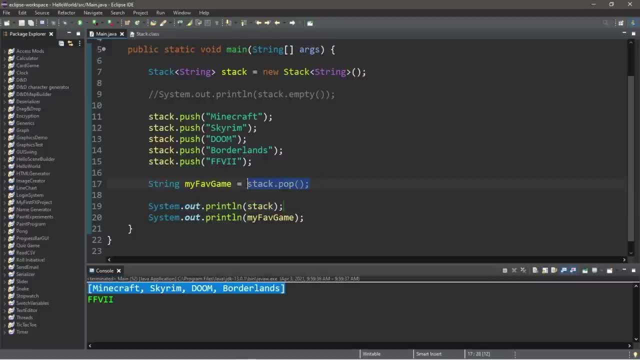 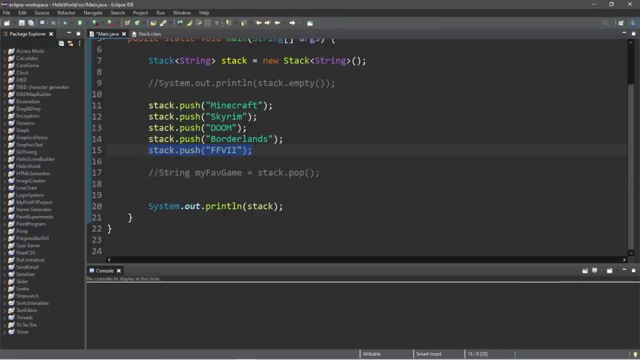 So Final Fantasy VII is no longer in my stack because I popped it, then assigned it to the string variable of my fav game. So in order to take the topmost object from a stack, you use pop and then assign it to something, If you ever need to take a look at what the topmost object is within. 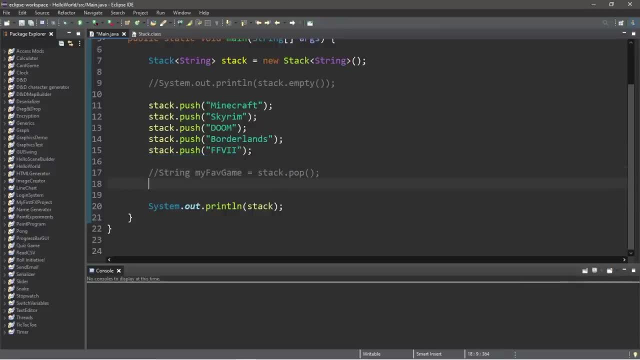 your stack. you do not want to use pop because that will remove it. You can instead use the peek method of stacks. So what I'll do is systemoutprintln and then immediately follow this with printing my stack. So let's run this. So the topmost item with the stack. 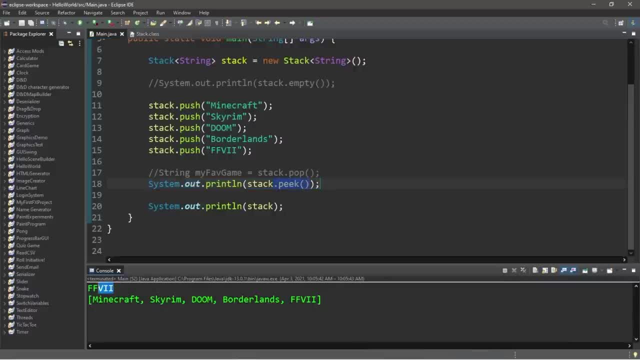 my stack after using the peek method is Final Fantasy 7.. Then, after printing my stack, Final Fantasy 7 is still at the top of my stack. So if you ever need to take a look at the object that is at the top of the stack without removing it, you 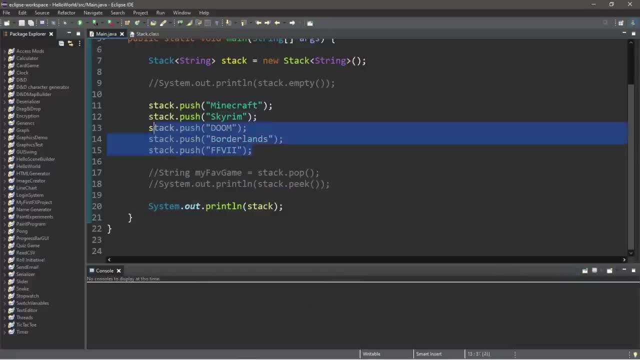 can simply use the peek method. If you need to search for an object within the stack, you can use the search method. let's print stack dot search and we pass in our object as an argument. So the very first item in a stack will have a. 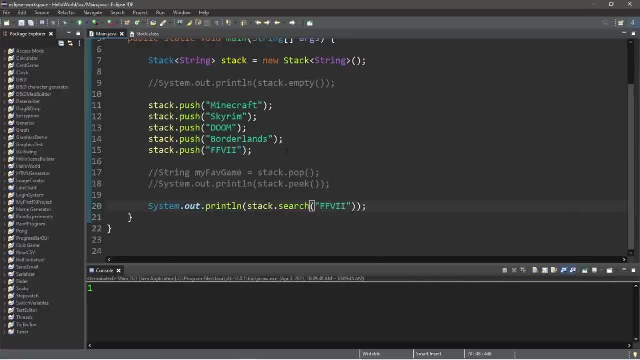 position of 1.. You would think it's 0,, but it's actually 1.. Now let's find Borderlands. That will be in position 2 from the top, then Doom would be of course 3,, Skyrim is 4,, then Minecraft is 5.. So if you search for an item that is not 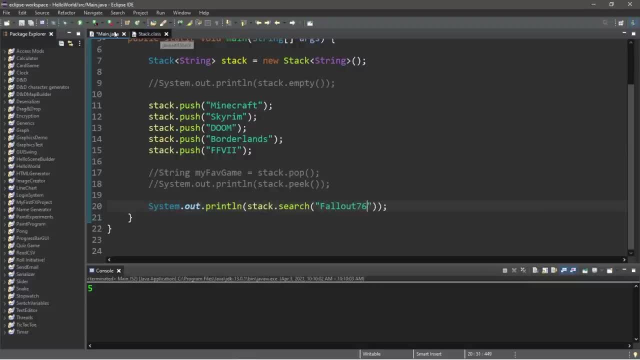 within the stack, like Fallout 76,. well then, this will return negative 1, which is great. If search does not find this object within your stack, it will return negative one. So with stacks, we can actually run out of memory. 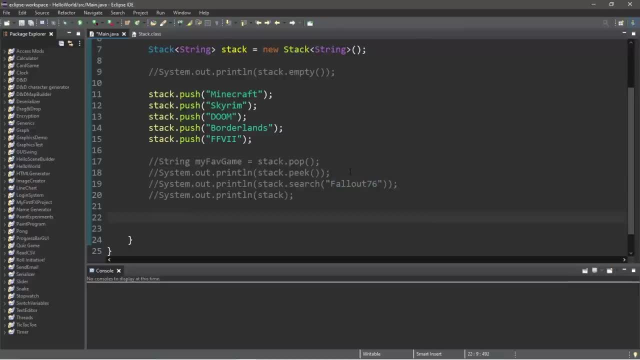 So let's add like a billion copies of Fallout 76. We find Bethesda's warehouse of unsold Fallout 76 games, So we'll create a stack of a billion copies of Fallout 76. We can do this using a for loop. Int. i equals zero as long as i is less than like one billion. 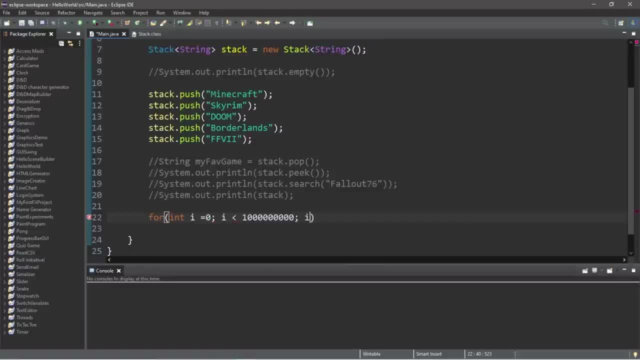 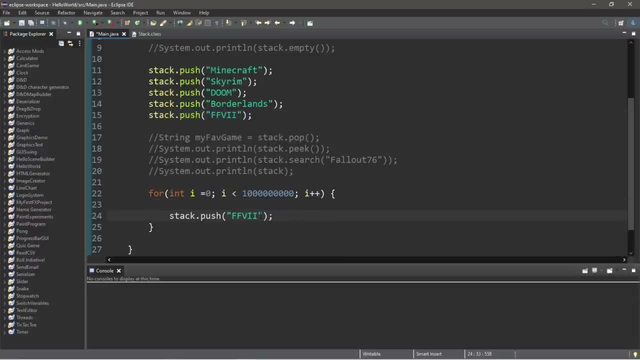 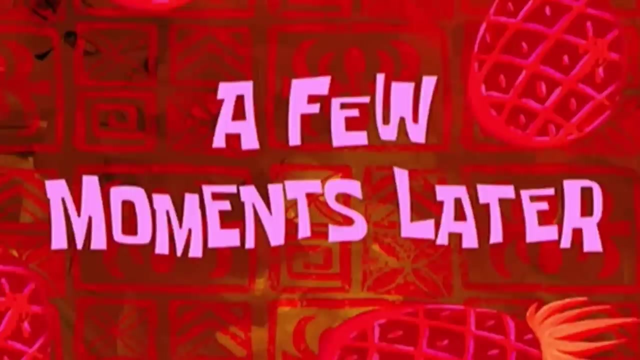 That's probably close enough, Increment. i then we will push a copy of Fallout 76 to our stack. So stackpush Fallout 76. And this is what happens. So we will run into an out of memory error due to the Java heap space. 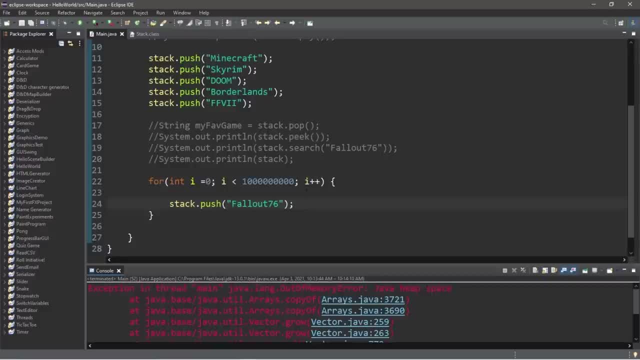 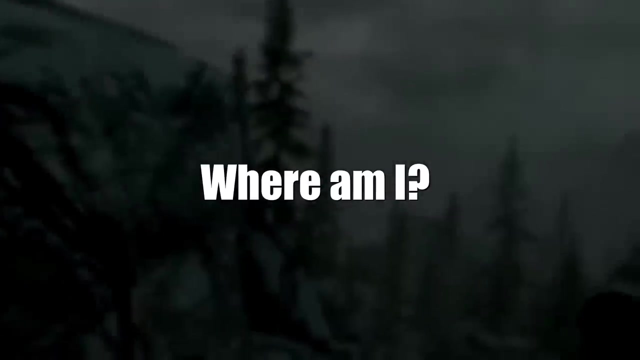 So it is possible to run out of memory when adding objects to our stack. Now, this is an interesting feature that may or may not happen to you if you add a billion copies of Skyrim onto a stack. Damn it, Todd Howard, you did it again. 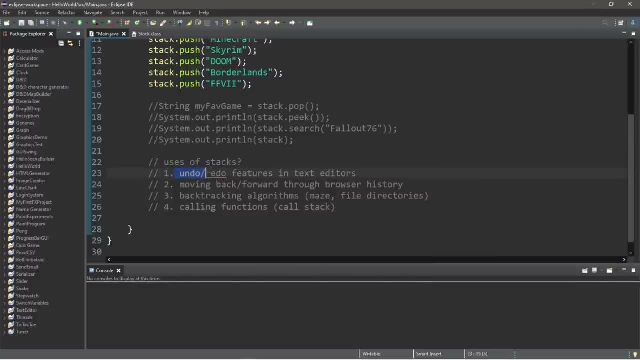 Now what are some uses of stacks? Here's a few examples. One: we can use them in undo- redo features in text editors, Like when we go to edit, then undo typing or redo typing. we can move back or forward through browser history by hitting the back or forward button in the top left corner of most web browsers. 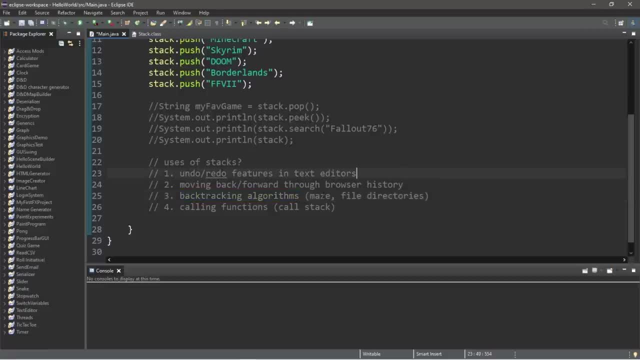 We can implement them in backtracking algorithms if we need to navigate a maze or search through file directories. And another is that we use them when calling functions. Whenever we call a function, we add what is known as a frame to the call stack. 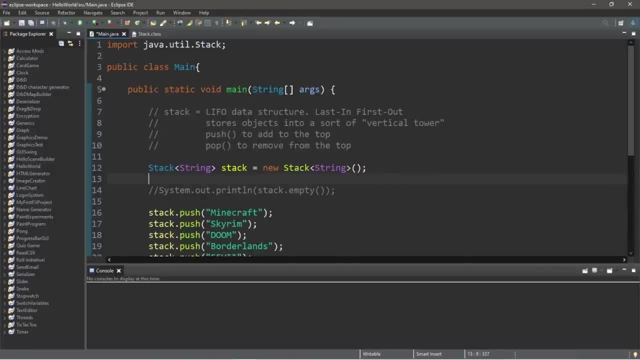 But I'll probably save this topic for another video. So in conclusion, everybody, a stack is a LIFO data structure. Last in, First Out, It stores objects into a sort of vertical tower, a stack of objects. You use the push method to add objects to the top and the pop method to remove objects from the top. 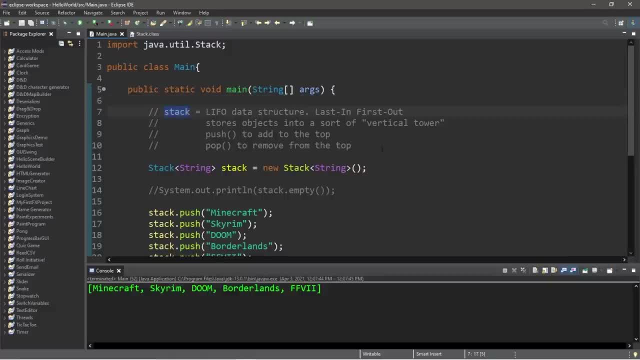 So those are stack data structures. In the next video we'll be covering queues, which work a little bit different. So if you can give this video a thumbs up and drop a random comment down below, But yeah, that is a stack data structure in well, computer science. 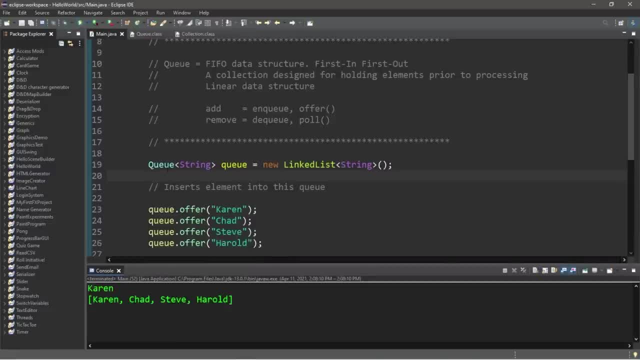 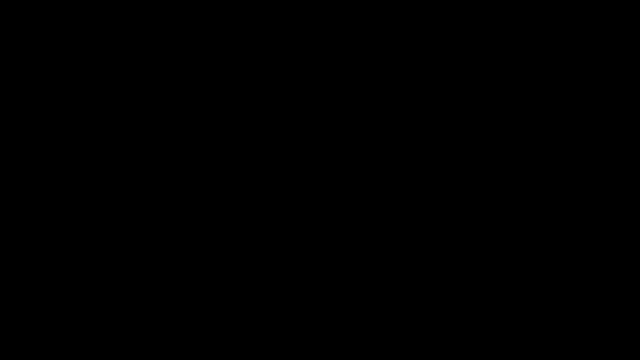 What's going on? everybody? It's your bro. Hope you're doing well. In this video, I'm going to explain queues in computer science, So sit back, relax and enjoy the show. If you find this video helpful, please remember to like, comment and subscribe. 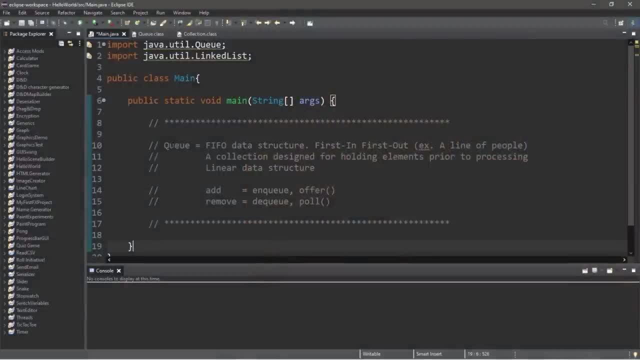 Your support will help keep this channel running. Whoa hey, we're talking about queues today, So queues are a FIFO data structure, not to be confused with FIFA. FIFO as in first in, first out. An example would be a line of people. 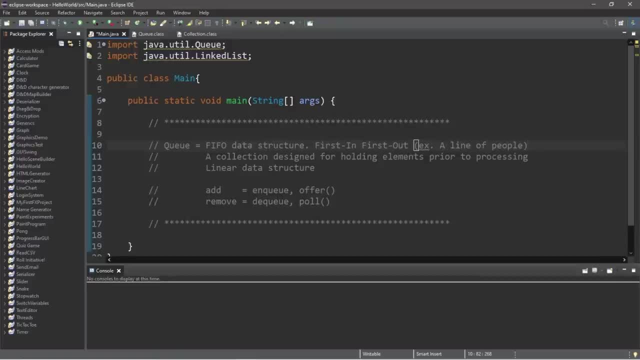 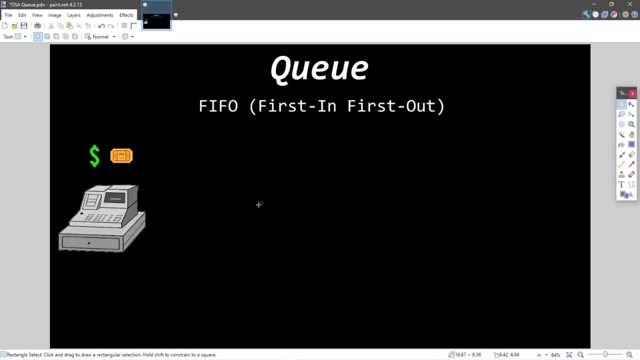 It's first come, first serve. Whoever's there first gets held first. So this is a collection designed for holding elements prior to processing. It's a linear data structure. Here's an example. Imagine that we're a cashier and we're selling tickets to a concert. 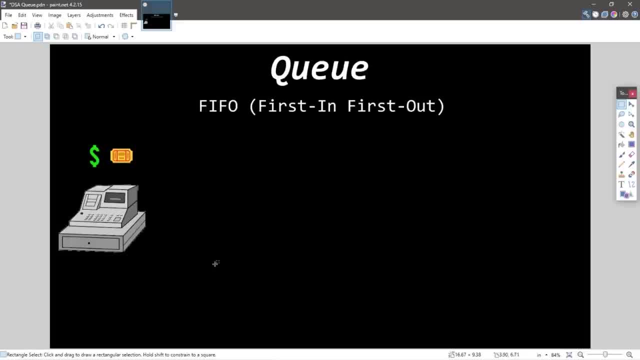 We will help whoever approaches our register first. It's first come, first serve. In other words, it's FIFO: First in, first out. Unfortunately, a wild Karen appears and she would like to talk to the manager. Now. Karen is going to waste everybody's time, so it's going to be a while. 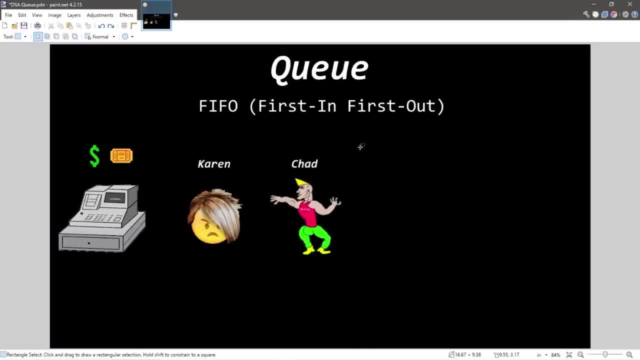 In the meantime, Chad enters the line. He will enter in at the back and wait his turn, Followed by Steve and then Harold. So Karen is at the head of our queue, our line- And Harold is all the way at the back- our tail. 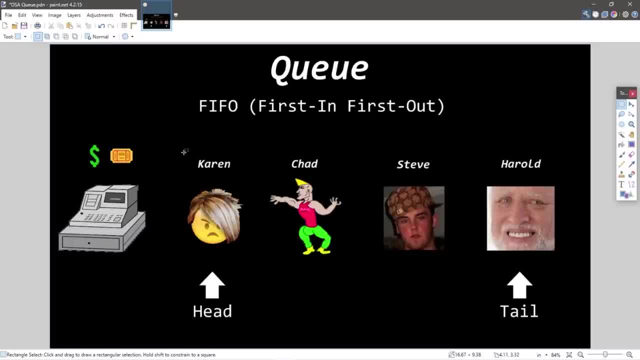 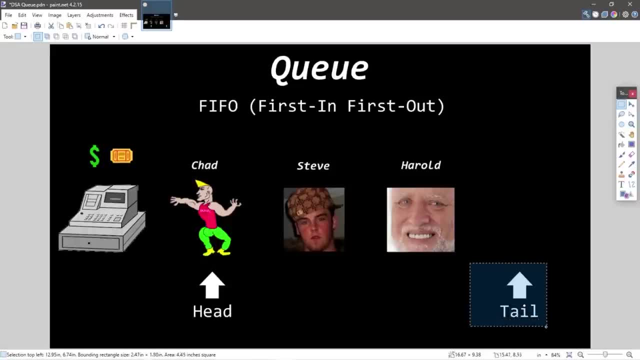 As you can see, Harold is very anxious right now. Once Karen has been defeated, Chad will move to the head of our queue. So Chad will now be helped next, And Harold will still be at the tail until somebody else enters the line. 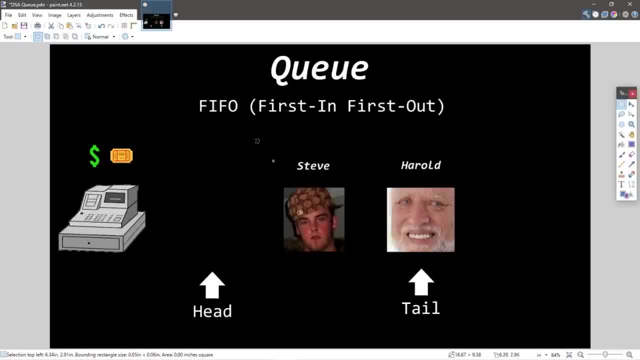 Once Chad has been helped, he will move out of our queue- And Steve is at the head now And the tail will move as well- And then, once Steve has been helped, Harold is the only one currently waiting in line for his tickets. 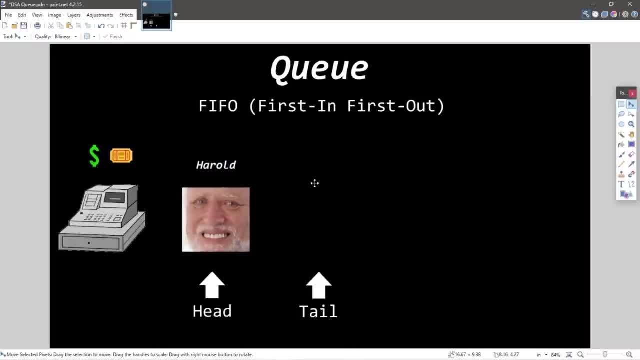 He will be at both the head and the tail of our queue. So that's kind of how a queue works. It's first come, first serve FIFO. First in, first out. If you were here first, then you will be helped first. 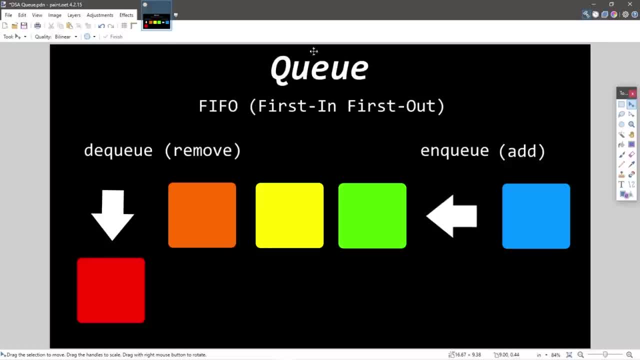 Now, the concepts of adding and removing objects from a queue are known as both NQing and DQing. NQing is the concept of adding an object to the end of our queue- our tail- And DQing is when we add an object to the end of our queue, our tail. 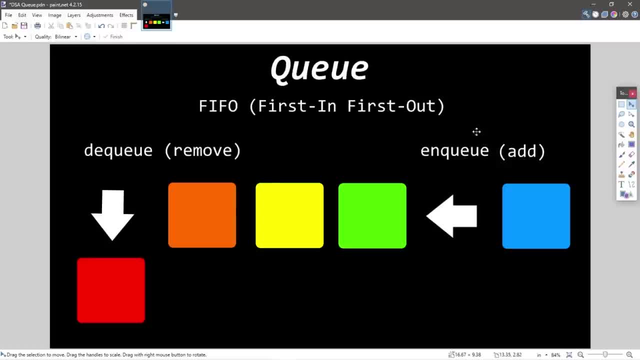 And DQing is when we remove an object from the head of our queue. Now, what methods do you need to NQ and DQ from a queue? Well, it really depends on the programming language that you're working with. A lot of you voted for data structures and algorithms using Java, so I'll probably stick with Java then. 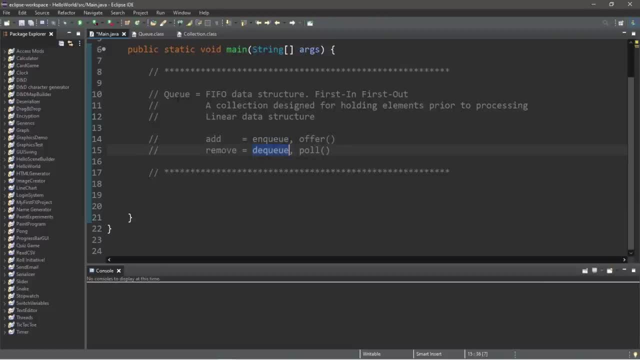 Here's an example. Now to NQ and DQ. we need, well, a queue, So let's create one Queue. Then we need to list the data type of the objects that we're going to add to this queue. 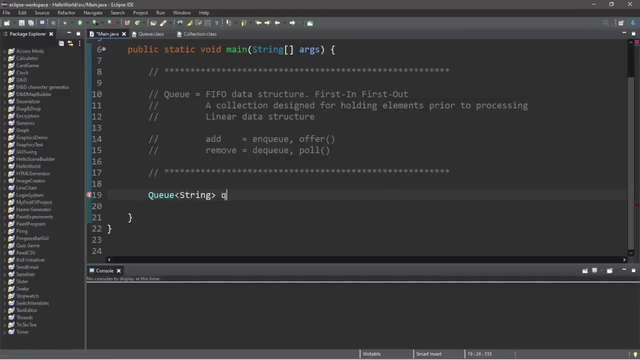 Let's work with strings, because strings are objects and they're fairly simple, So I will name this queue- queue equals new. Now check this out. I will attempt to create a queue object and instantiate it, And the data type is string, and I will add a constructor. 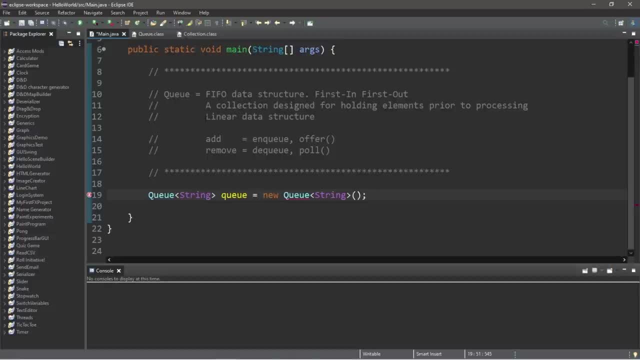 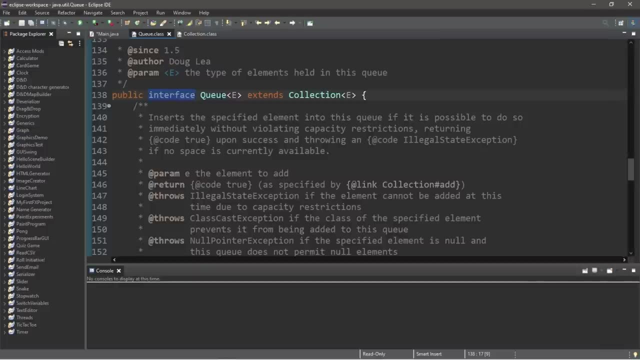 Now we cannot instantiate the type queue. Here's the reason why. So if we take a look at the queue class right here, queue is actually an interface and not a class And, based on our lesson on interfaces, we cannot create an instance of an interface. 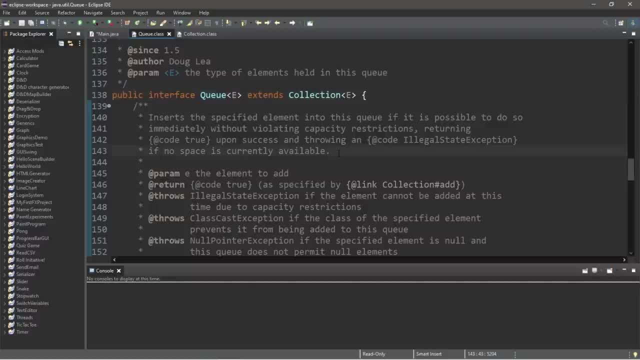 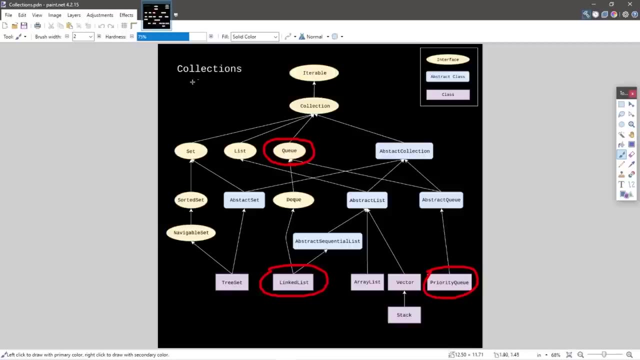 An interface is meant to be more of like a template And we can apply to another class. So to utilize queue technology, we need a class that implements queue. Now, taking a look at our Java collections hierarchy, there are two classes that implement queues. 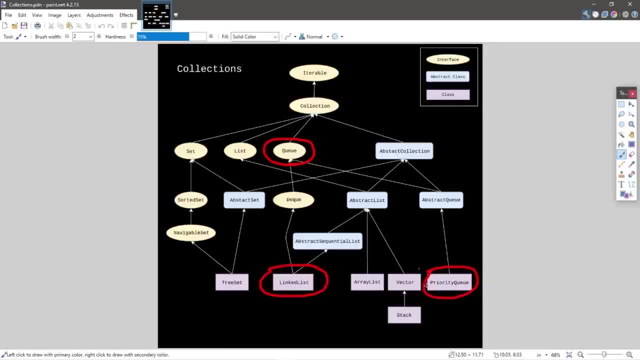 One of which is the linked list and the other is the priority queue. Now, priority queues, they will rearrange their elements based on a certain priority, So they wouldn't be a good example. So, to utilize the features of a queue, we are going to create a linked list because 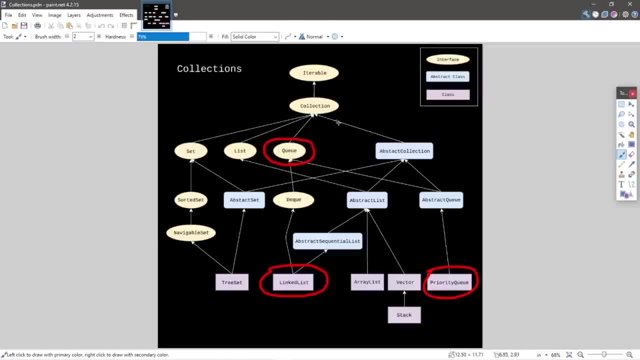 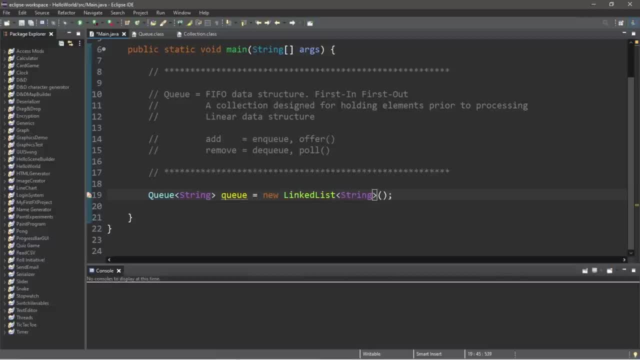 we cannot instantiate a queue itself, Because it's an interface With. that being said, let's change equals new queue to equals new linked list. We won't be focusing on any of the features of linked lists. We'll save that for another video. 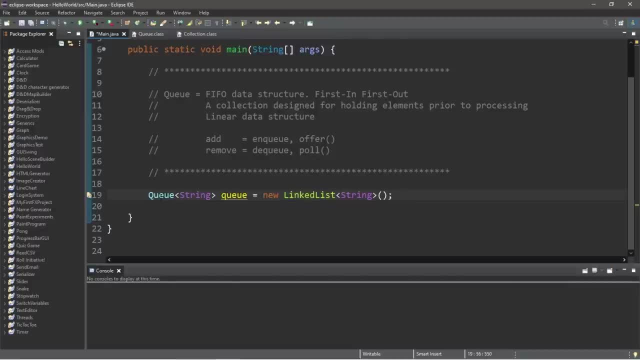 Maybe the next one, I haven't decided yet, So we will only cover the features that linked lists will utilize via the queue interface. Now, with the queue interface, there are three methods that we inherit from the collections: parent, class, Add, remove and element. 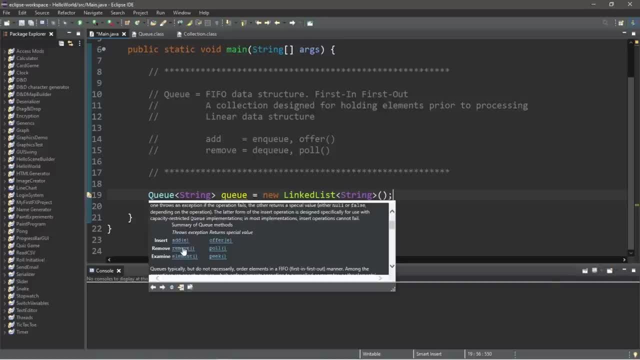 These will do approximately the same thing as enqueuing, dequeuing and peeking at the top. most element, However, they throw exceptions and, according to the documentation, it's actually better to use this column of methods instead. These will return a special value. 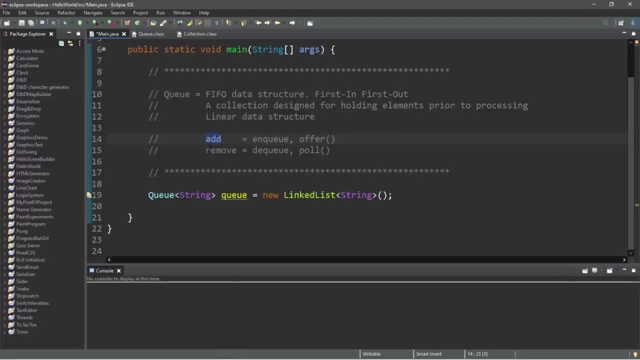 We have offer which will enqueue or add an element to the tail of our queue. Pull will dequeue. It will remove the head of our current queue, And then there is also peek. It will remove the head of our current queue, And then there is also peek. 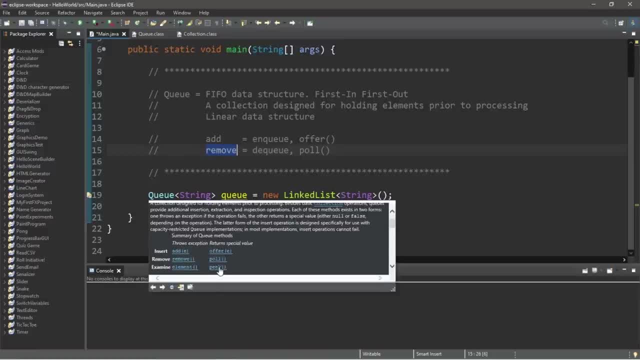 It will not remove the head, but it will examine it and return it. So those are the three dedicated methods that we implement via the queue interface. There are some additional methods too, which we'll cover later, which we inherit from the collections class. 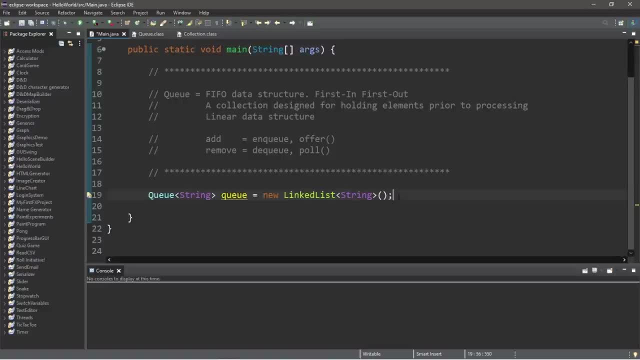 So let's begin by offering a bunch of people to our queue. This is how we enqueue, or add elements to our queue. So first in our line we have Karen, So to add her to the queue we would type the name of our queue: queueoffer. 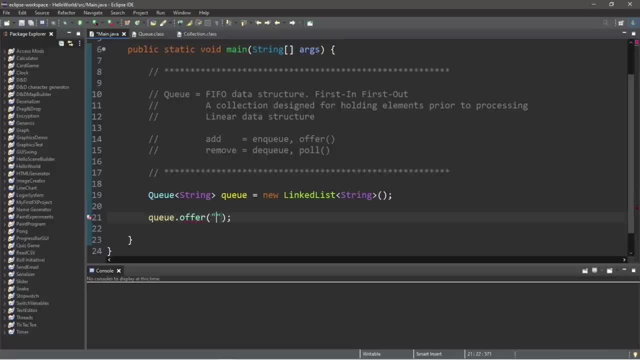 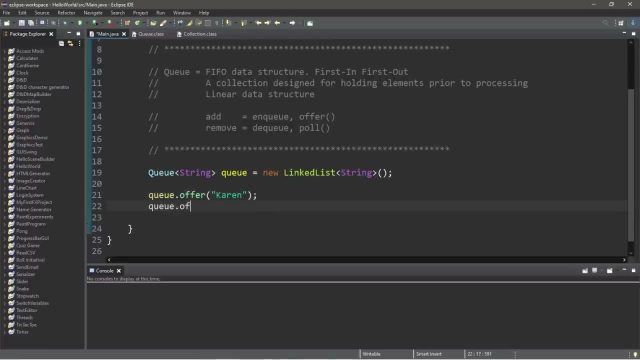 And we will offer Karen to the front of our queue and she would like to complain to the manager. Next we have Chad queueoffer Chad. Then we have Steve And lastly Harold. Okay, now, if we were to display our queue, we'll place it within a print line statement. 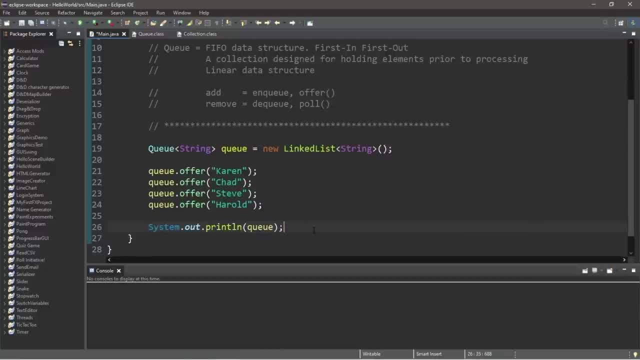 We will put in a print line statement. We will put in a print line statement. We will pass in queue as an argument And this should display our queue in order. First we have Karen at the head, then Chad Steve, then Harold at the tail. 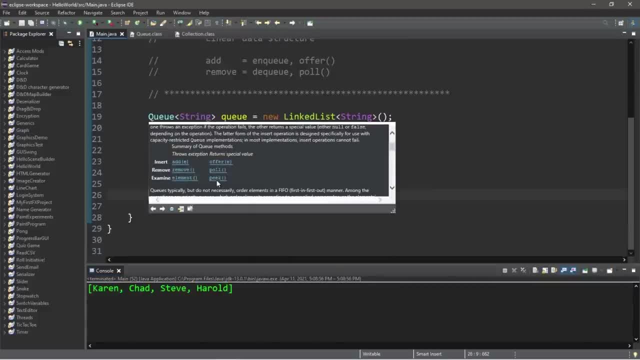 One method that we implement from the queue interface is the peek method. We can use the peek method to examine and take a look at the object at the head of our queue. We're not actually going to remove the object at the head of the queue, but take a look. 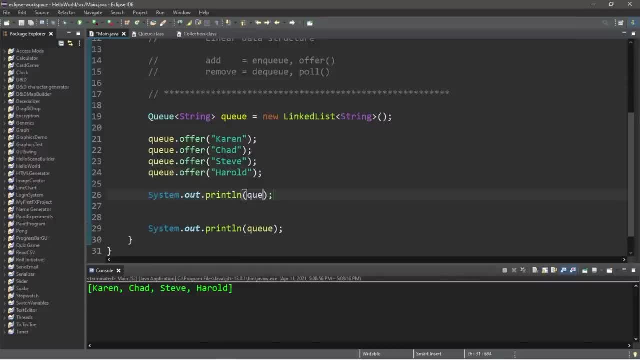 at it. So within a print line statement I will use queuepeekmethod And we're going to do that peekmethod. And after peeking over our cash register- unfortunately Karen is at the front of the line Now to dequeue- we can use the pull method. 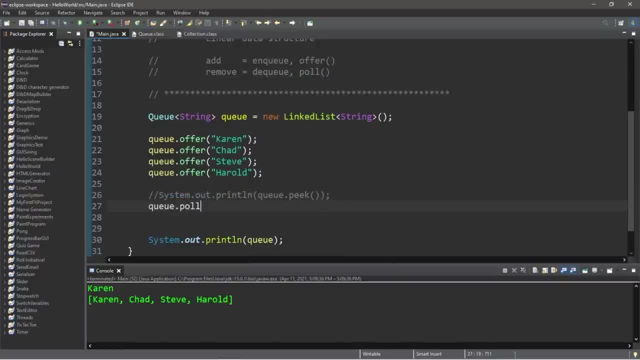 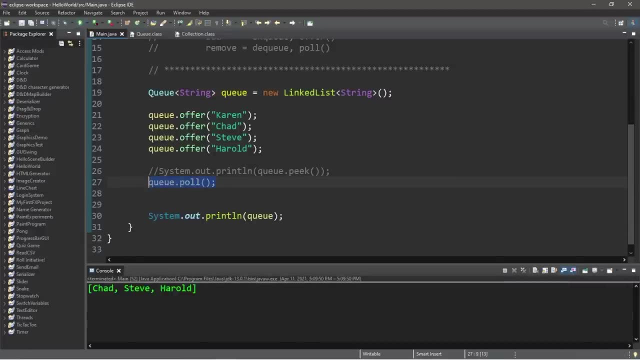 So type queuepull And this will dequeue your queue. So Karen is no longer at the head of our queue. So let's pull a couple more times for practice. So after pulling twice, Karen and Chad are now gone. Using pull a third time will remove Steve. 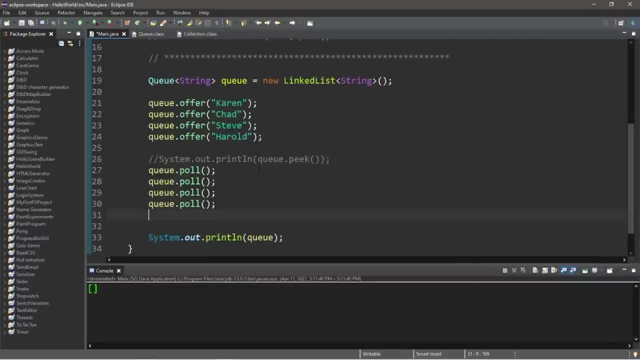 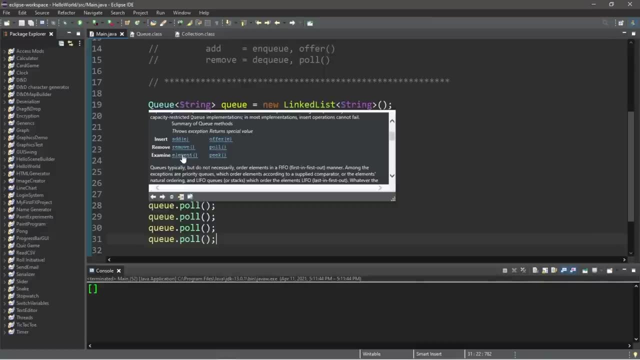 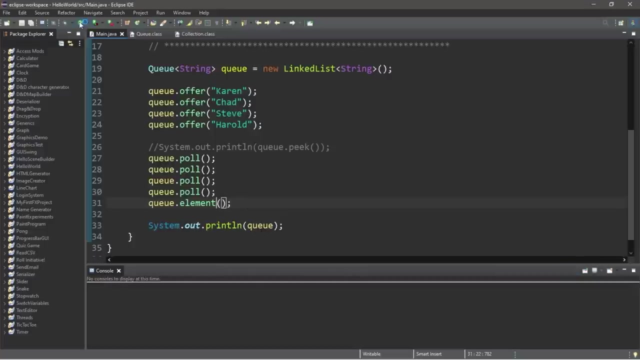 And lastly, Harold. Now, the nice thing about the pull method is that it will not cause an exception. According to the Java documentation, you can use element to peek, but it will throw an exception. So if I was to use element at the end, this would cause an exception then. 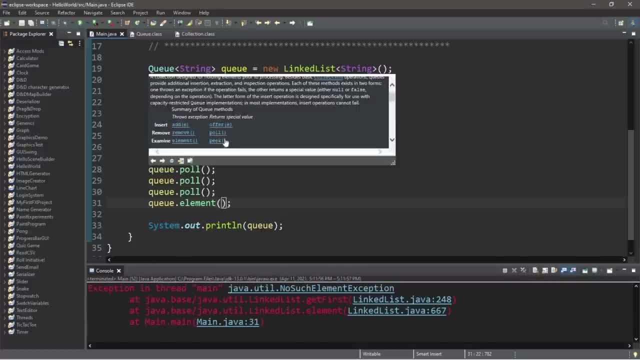 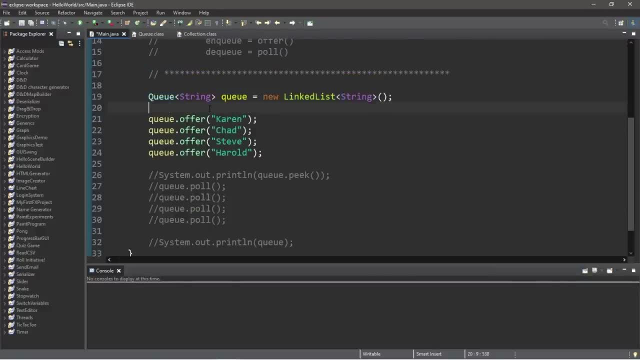 So usually it's preferable to use this column of methods. even though they're similar, These will not throw exceptions: Offer, pull and peek. Now with queues, there are some additional methods that you might be interested in. The queue class will extend the collection class, so the queue class inherits everything. 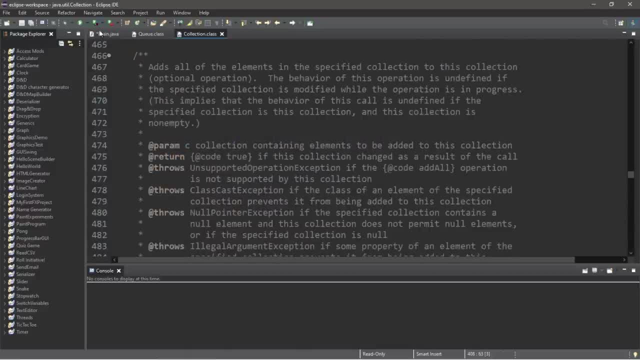 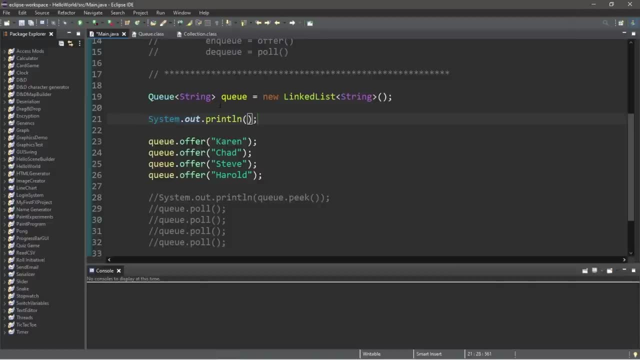 that the collection class has, And there's some pretty useful methods within. here I'll show you a few. So the first is that we can check to see if our queue is empty. So within a println statement I will type queueisEmpty. 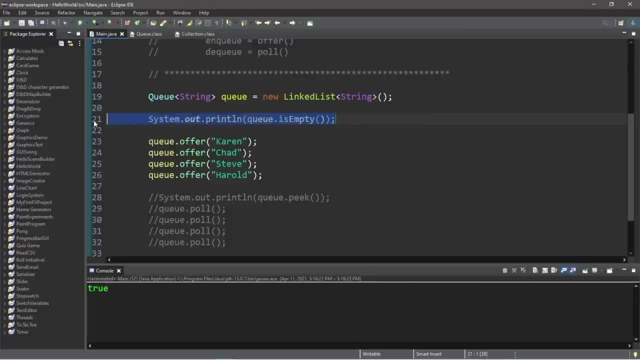 And if our queue is empty, this will return true. So if I move this line of code After we offer a bunch of strings, a bunch of people to our queue, if we check to see if our queue is empty, that will be false. 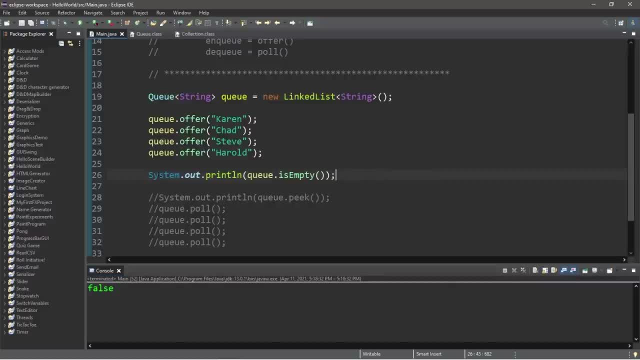 There are people currently within our line, So that is the isEmpty method. We can also check to see the size of our queue. How long is our line System dot out, dot println queue, dot size And the size of our line. our queue is four. 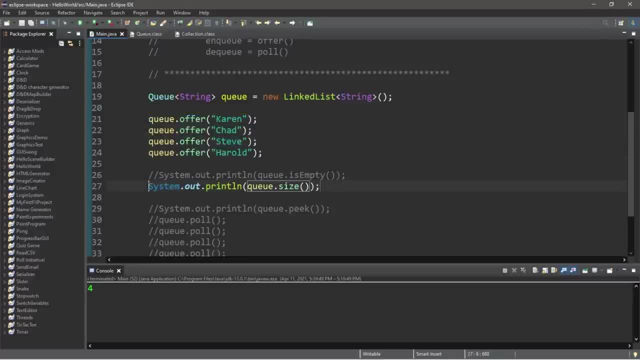 Four objects. We have four people waiting in line to be helped. So that is the size And another is the contains method. We can check to see if our queue has a certain object that we're looking for. So within a println statement I will type queue dot contains and then pass in an object. 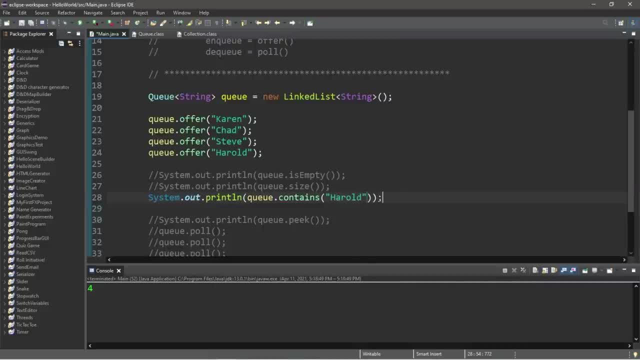 Let's check to see if Harold is at the back of the line. He's been waiting here patiently. Queue dot contains Harold And according to the contains method, Harold is in fact within our line. That is true. However, this method does not give the index the position. 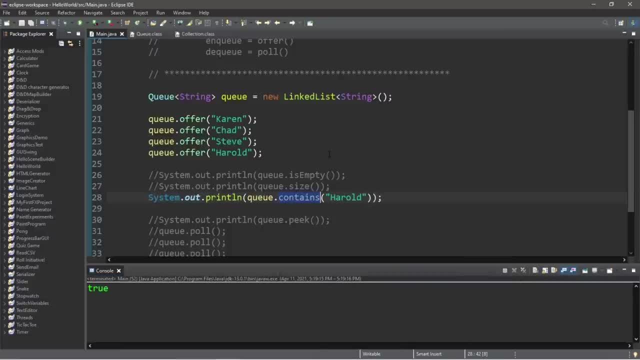 Imagine that we yell out: hey, Harold, are you there? And he yells back: yeah or true? That's kind of how the contains method works. So these are three useful methods that queues inherit from the collection class. Now where could queues be useful? 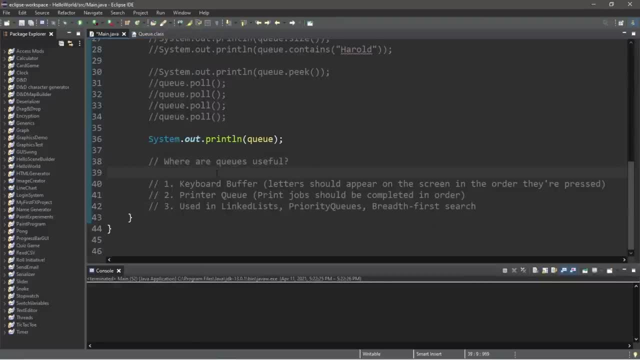 They're actually used in quite a number of things, but here's a few examples that came to mind. So one: they can be used in keyboard buffers. Have you ever typed so fast that the computer couldn't render all of the characters onto the screen? 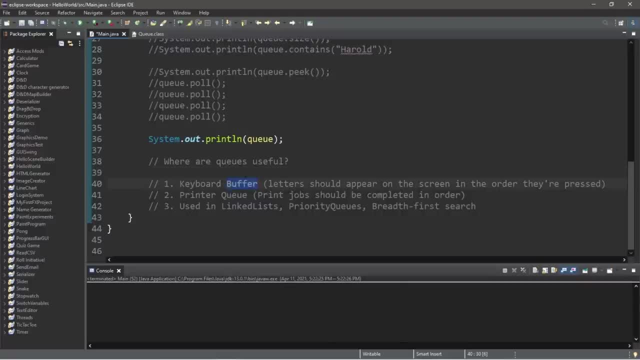 All of those characters were added to a buffer. They were all displayed in sequence and they were waiting for their turn to be displayed. So with a keyboard buffer, letters should appear on the screen in the order that they're pressed right: First in, first out. 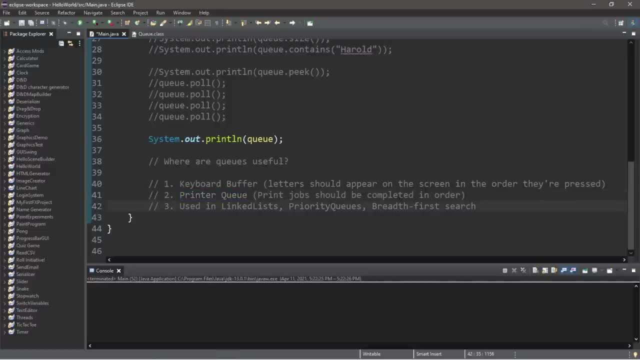 They're also used in printer queues. Print jobs should be completed in order, So we would start with page one, then page two and just follow that pattern And, as we discussed before, they're used in linked lists, priority queues as well as. 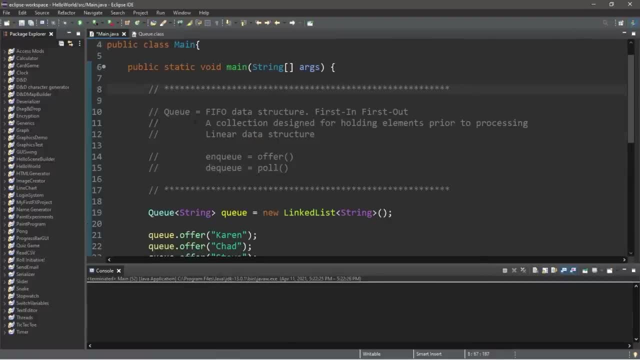 breadth-first search algorithms. Well, everybody. In conclusion, a queue is a FIFO data structure. First in, first out. It's a collection designed for holding elements prior to some sort of processing. It's a linear data structure. Imagine a bunch of people waiting in line. 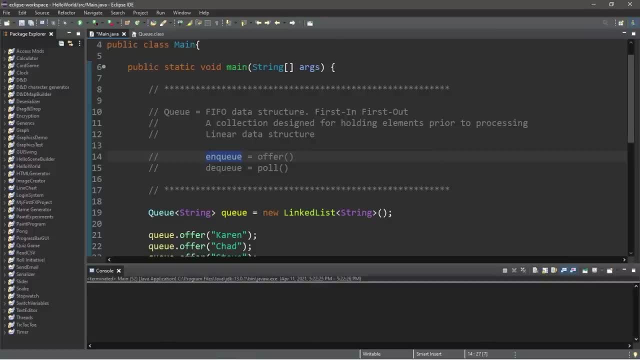 To enqueue that means to add an element to the tail of our queue. to the end. We can use the offer method in Java. To dequeue, we would use the pull method in Java. That will remove the element at the head of our queue. 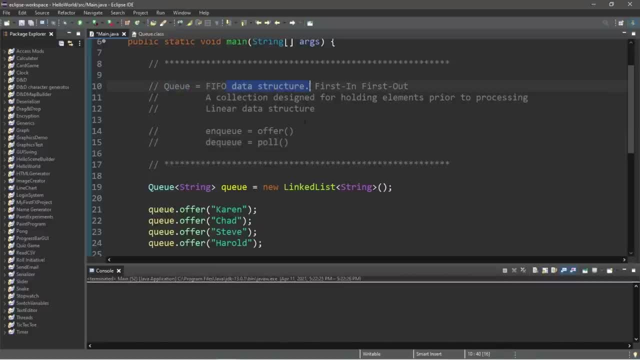 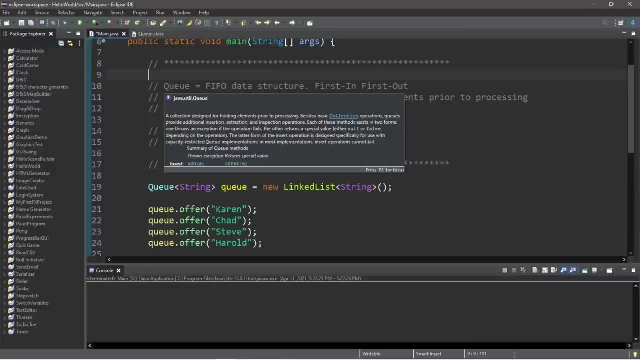 So that is the queue data structure In the comments down below. let me know what you would tell Karen if she asked to speak with your manager. And that, ladies and gentlemen, is the queue data structure in the field of computer science. Heyya, everybody. 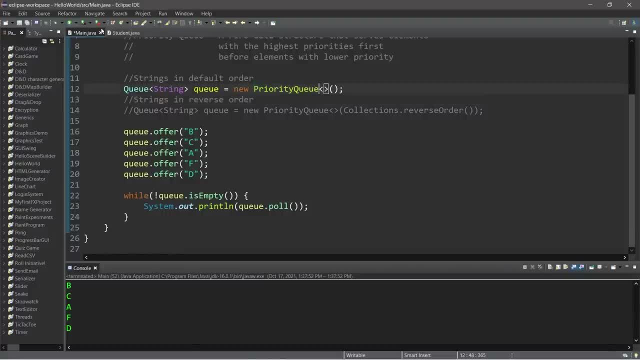 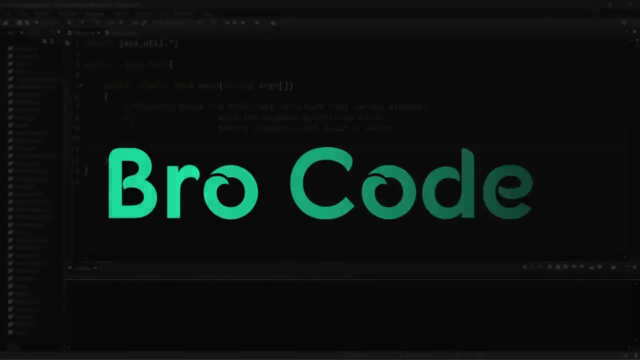 It's your bro, Hope you're doing well, And in this video we're going to discuss priority cues in computer science. So sit back, relax and enjoy the show. Heyya, What's going on? everybody, So priority queues. 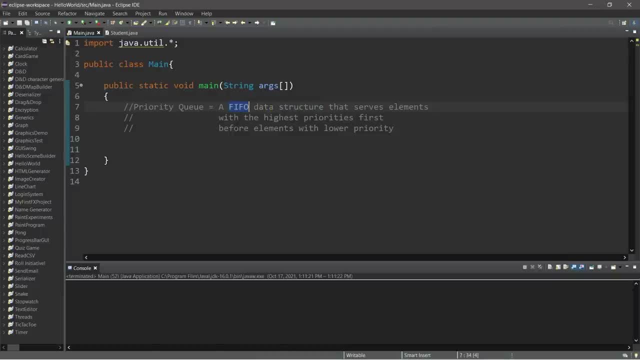 priority queue is a FIFO data structure: first in, first out. however, a major difference with priority queues is that before we start polling and serving elements, we put them in some sort of order. higher priority elements are served first before elements with lower priority. so here's an example. let's say 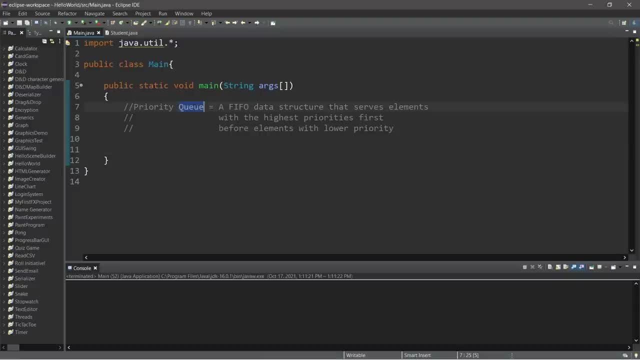 that we have some student GPAs and we'll place them all within a queue and then a priority queue and take a look at the differences. so let's create a queue, the data type is queue and we are going to insert some doubles, some GPAs. I'll name this. queue equals new. now, queues are actually interfaces and 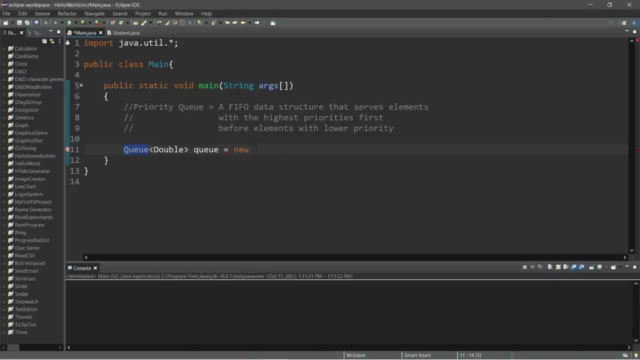 we can't implement them directly, so we need to use a class that utilizes the queue interface- one that I know of is a linked list- then finish instantiating it. now to add data to a queue, we use the offer method- queue dot, offer- and then pass in a GPA. let's make sure that these are not in order. 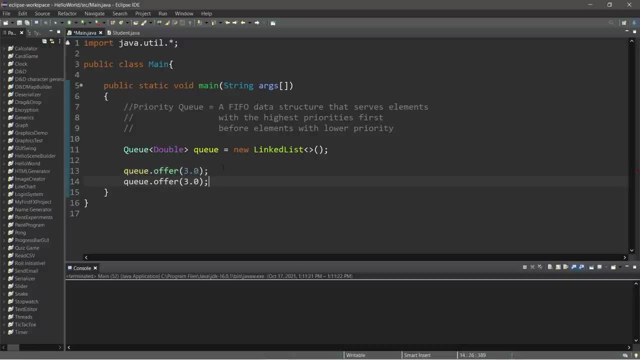 how about a 3.0? then the next student has a, let's say, 2.5, then a 4.0, 1.5 and 2.0. okay, now let's display the elements of our queue, one easy way in which we can do that. 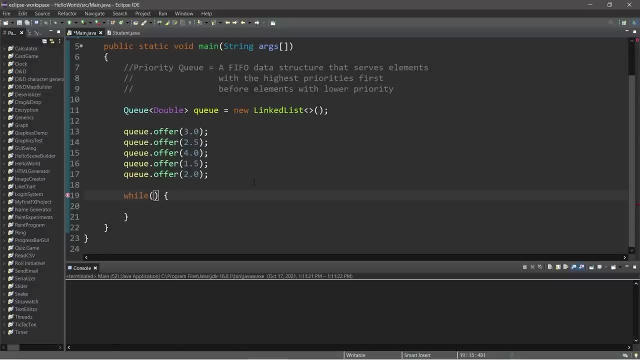 is to use a while loop, and this is our condition. we'll continue this while not logical. operator q dot is empty method. while our queue is not empty, pull each element and display it. so, within a print line statement, let's use q dot pull to display and remove each element, beginning with the first one, and then 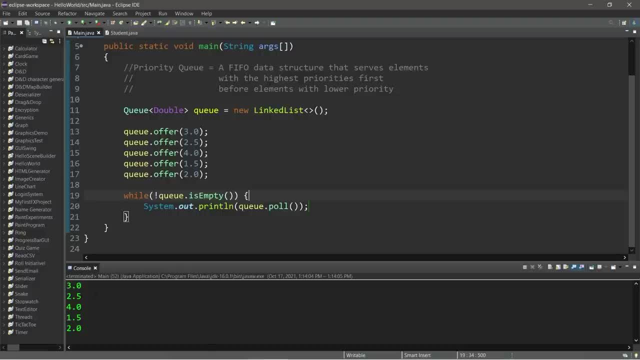 working our way to the end. so this will display the elements within my queue. so these are in: first come, first serve order. whatever element we were offered first, we are serving that element first. if an element was added last, well, then it's served last. so that's a standard queue. now, with a priority queue, we're going to arrange them in some sort. 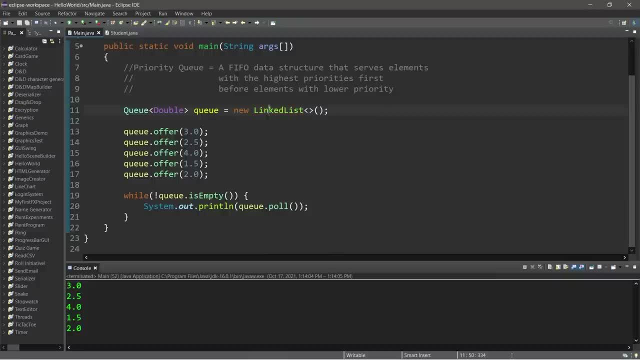 of order before we actually pull these elements. so let's change our linked list to a priority queue and run this again and let's take a look at the differences. okay, these are all in order now, and so if we're working with numbers like doubles, these are arranged in ascending. 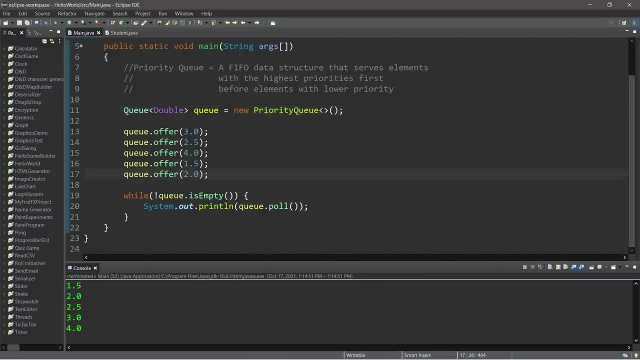 order, beginning with the smallest element. let's pretend that these are grade point averages, gpas. why might we want to put these in order? let's say: whatever student performed, the worst gets two hours of free tutoring. whichever student performed, second worst gets one hour of free tutoring and third gets half an hour free tutoring. now, if you need these, 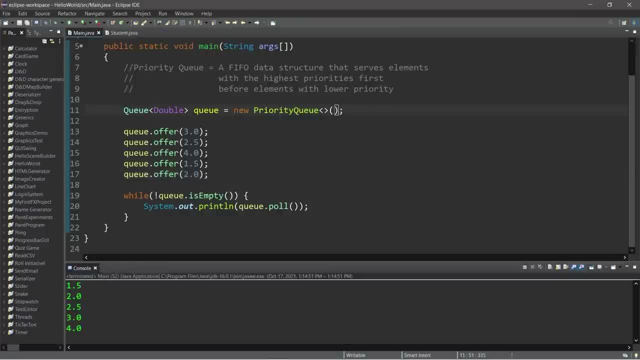 in descending order. well, there's one change that we're going to make. within the constructor, we can pass in a comparator, but that's a little advanced for us and we haven't discussed that yet. So there is a default comparator that we can use. found within collections: Collections dot reverse. 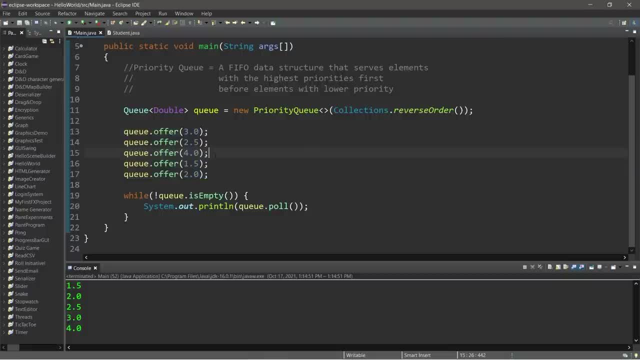 order method, So these elements will be in reverse order. then, In this example, let's say that whichever student has the best GPA will receive- I don't know- a gold medal, like the Olympics, and the second best student will receive a silver medal, then a bronze medal. 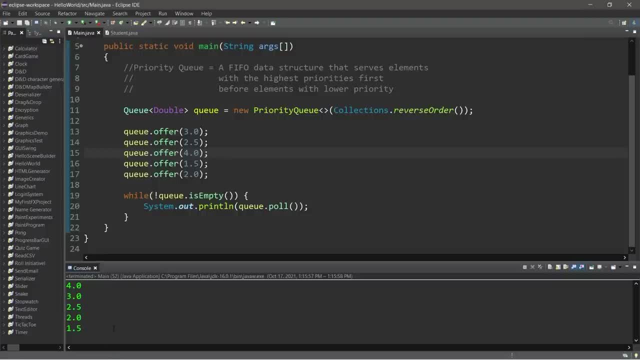 and then every student after that, I guess, will receive nothing. But that's okay, though. they got some free tutoring in the last example. Okay, now let's change the data type, Let's say that these are now strings, and let's put these in standard order. So let's change these two strings. 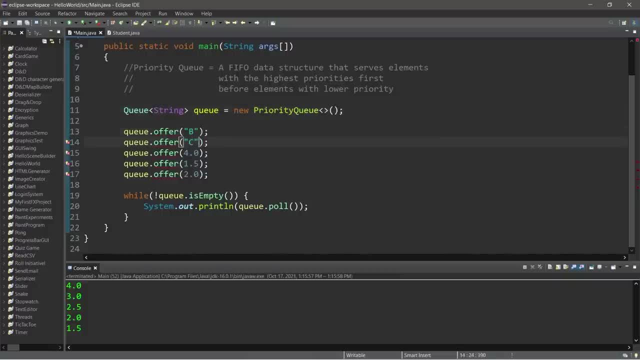 Maybe this student has a, B, this one has a, C, A, F. and what are we missing? D. If we have a priority queue of strings, well then these elements will be in alphabetical order, So if we need these, in reverse alphabetical. 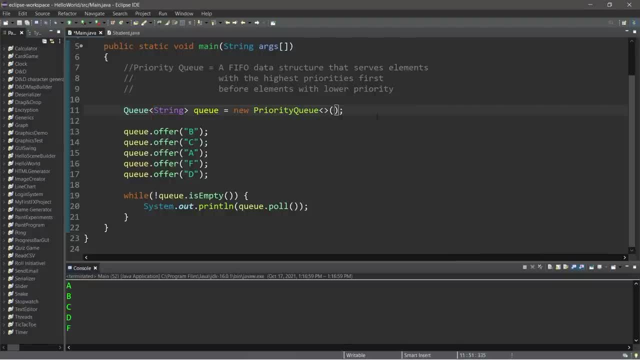 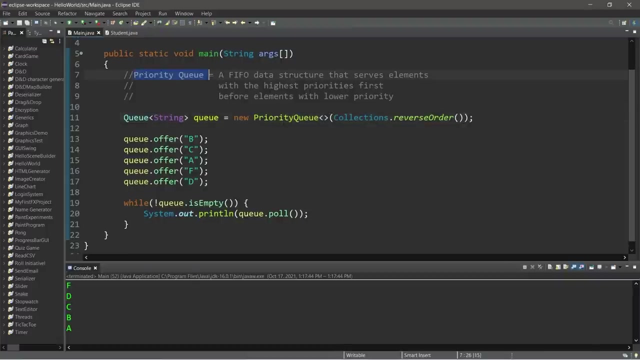 order. again, we can pass in a comparator and then one that we can use is from collections: Collections dot- reverse order. And these elements within our priority queue are now within reverse alphabetical order. So, yeah, that's a priority queue. Think of it like a queue. however, we first sort these elements based on a certain priority. 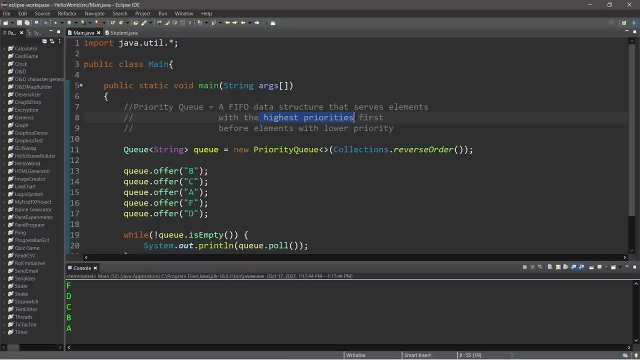 we will pull and serve the elements with the highest priorities first and work our way to elements with lower priority. So, yeah, that's a priority queue. If you would like a copy of this code, I'll post this to the comment section down below. and well, yeah, those are priority queues. 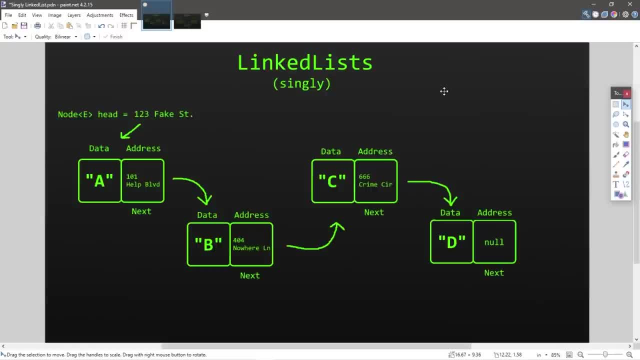 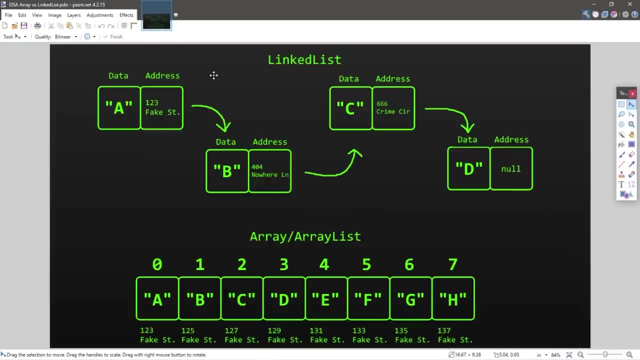 in computer science. Hey, what's going on? everybody, it's ya, bro, hope you're doing well. In this video we're going to discuss linked lists and lists and computer science. so sit back, relax and enjoy the show. Now, before we dive straight into linked lists, we're going to take a closer examination. 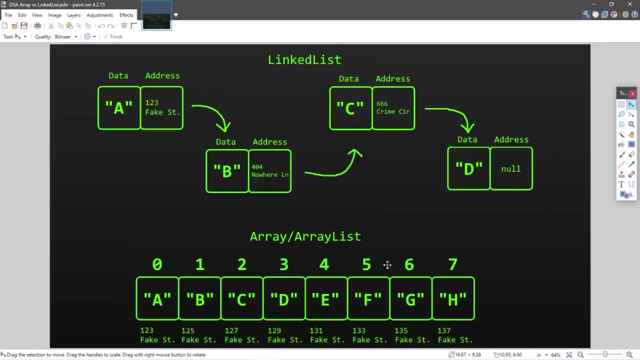 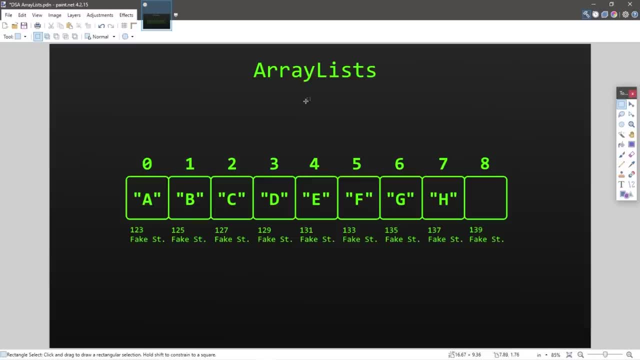 of arrays and array lists. We will see what disadvantages that these data structures have where linked lists excel at. so we'll compare and contrast the differences between the two. With what we understand with arrays and array lists, these data structures store elements in contiguous memory locations. 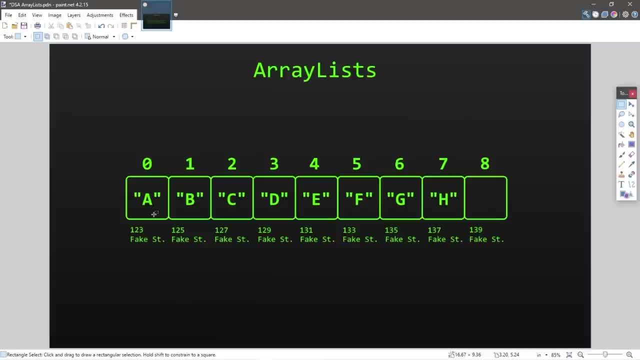 In this demonstration I'm storing letters of the alphabet. Suppose that the first element of my array has a memory address of 123 fake street. Obviously, these are not real memory addresses, but this is how I like to think about things. If this was a memory address, then the next element in my array may have an address of. 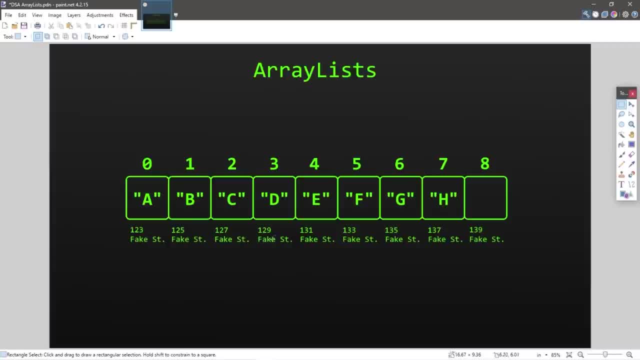 125 fake street, then 127 fake street, 129 fake street, and then you just continue on in that pattern. Now, arrays are fantastic at randomly accessing elements because they have an index, but they're not so great at inserting or deleting elements, especially when those elements are closer. 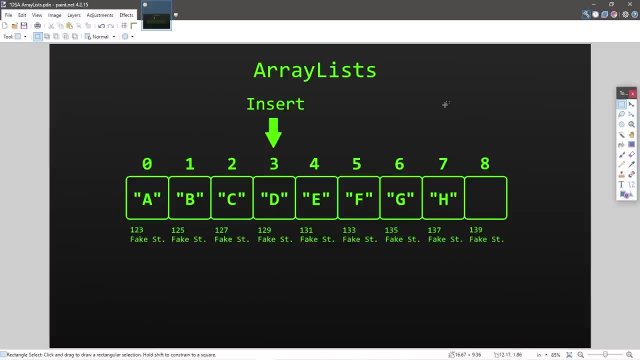 to the beginning of the array. Here's an example. Suppose I need to insert a new element at index 3.. Since this element is already occupied with a value, I would need to shift my elements to the right in order to accommodate room for this new element. so the process of shifting. 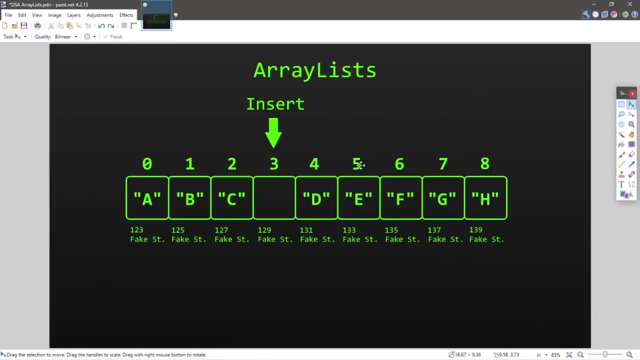 is cumbersome. But once this element is empty, then I can insert a new value. So it's not that big of a deal if I have a small dataset. but imagine if I had 1 million elements. I would need to shift my data up to that many times depending on the location of the insertion. 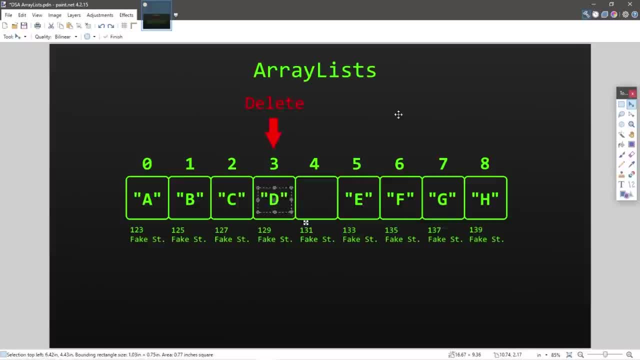 As with deletion as well, we would shift our elements to the left to close the gap. You're probably thinking, dude, why are you talking about arrays in a video about linked lists? Well, where arrays have difficulty inserting and deleting, linked lists actually have the 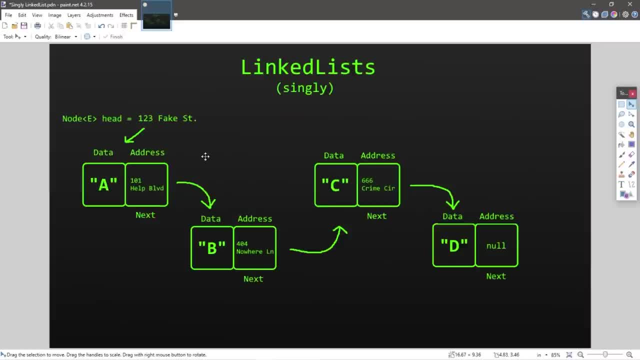 advantage. Here's a representation of a linked list. A linked list is made up of a long chain of nodes. Each node contains two parts: some data that we need to store and an address to the next node in line, also referred to as a pointer. 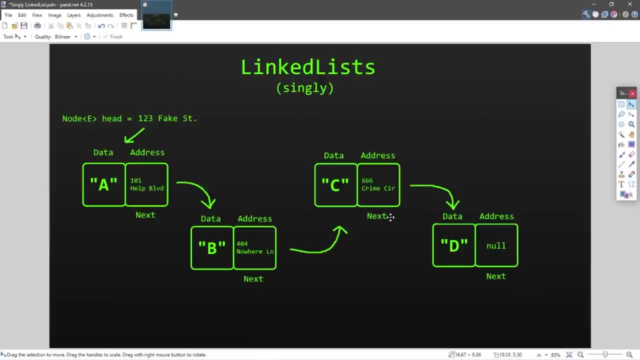 Linked lists do not have an index the same way that arrays do, But each node contains an address to where the next node is located. So these nodes are non-contiguous. They can really be anywhere within your computer's memory. If our initial node has a memory address of 123 Fake Street, like our array example, then 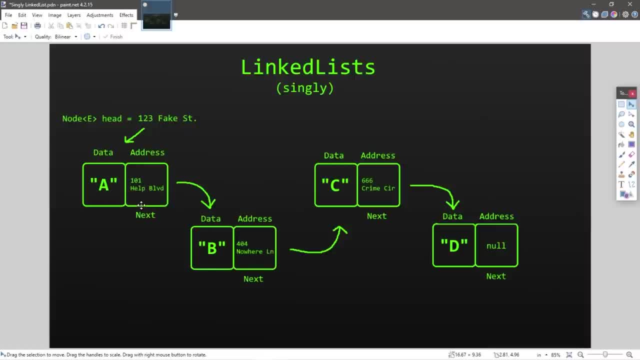 the next node in our linked list could have a memory address of maybe 101 Help Boulevard, and another could be 404, Nowhere Lane, then 666 Crime Circle. Each node knows where the next node resides. I imagine this as if we're following a code. 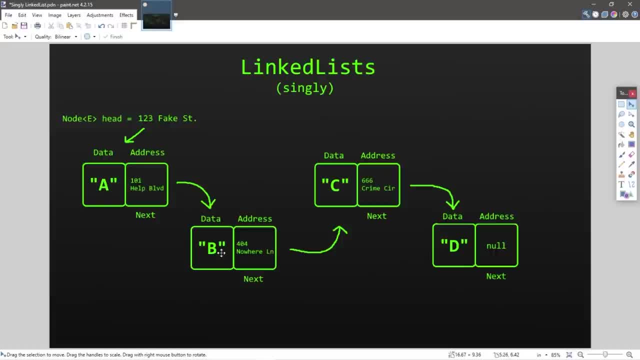 I imagine this as if we're following a scavenger hunt or a series of clues to find the end of the linked list, the tail. Each node has an address, a clue as to where the next node is. We begin at the head and work our way towards the tail, following each clue, each memory. 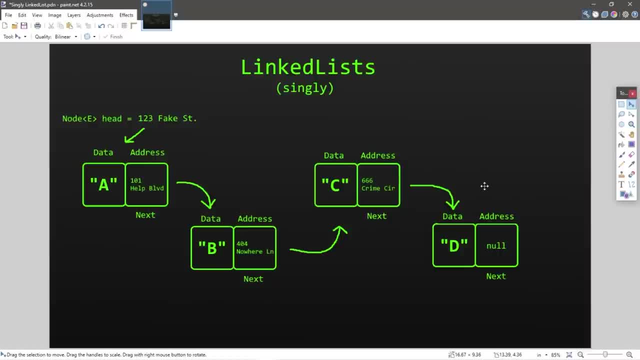 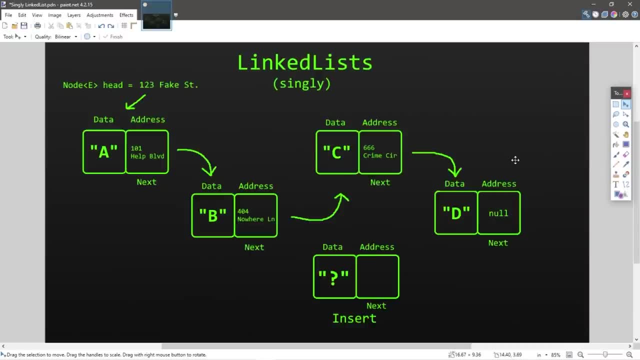 address found in each node. Then we know when we reach the end of our linked list. when we check that address, our pointer, and it has a value of null, That means we're at the tail, we're at the end of our linked list. 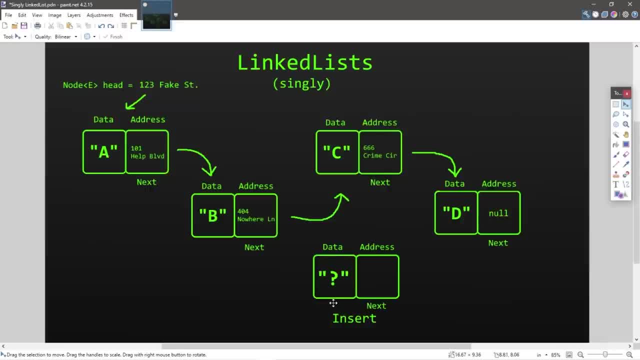 Inserting a node is easy in a linked list. There's no shifting of elements involved. Wherever we need to place a new node, we take the address stored in the previous node and assign the address of our new node with the address from the previous node, so that 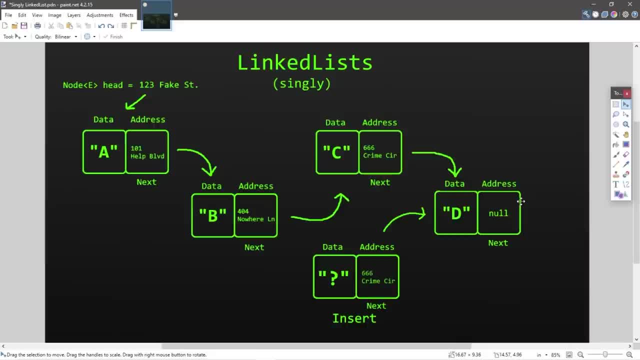 our new node is pointing to the next node in line, Then we can take and replace the address in the previous node with an address that points to our new node. It's as simple as that and we're completing our chain simply by inserting a node at a. 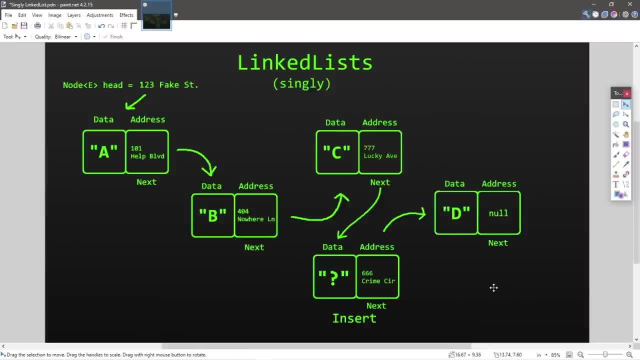 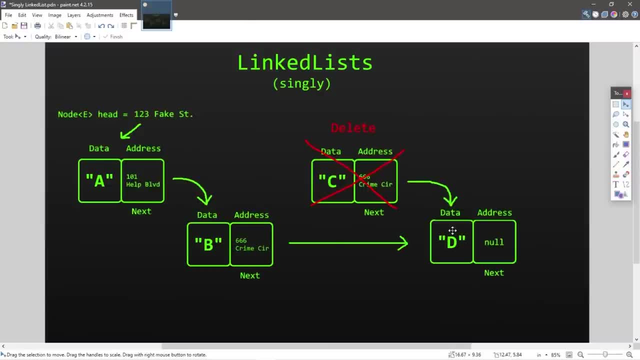 given location. There's only a few steps involved, no shifting of elements required. Deleting nodes are easy too. Wherever we need to delete a node, We have the previous node point instead to the next node in line. Again, no shifting of elements is necessary. 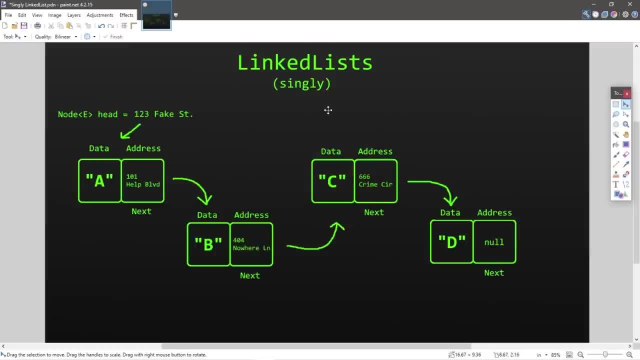 Now this is where linked lists tend to be inferior to arrays. They are bad at searching. We can randomly access an element of an array because we have an index With a linked list. that is not the case. To locate an element, we need to begin at the head and work our way towards the tail. 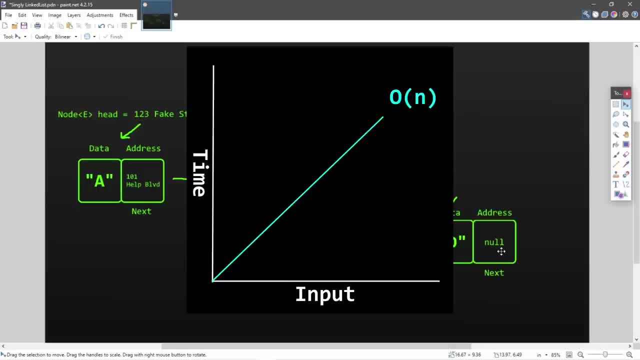 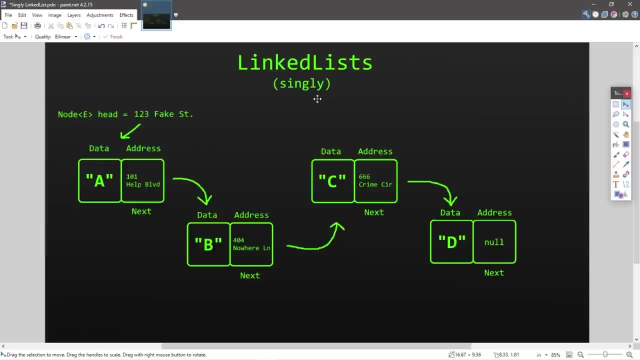 until we find the element that we are looking for. This itself takes time. In fact it would take linear time, but making the insertion or deletion of a node is constant. This variation of a linked list is a singly linked list. There are single links to each node. 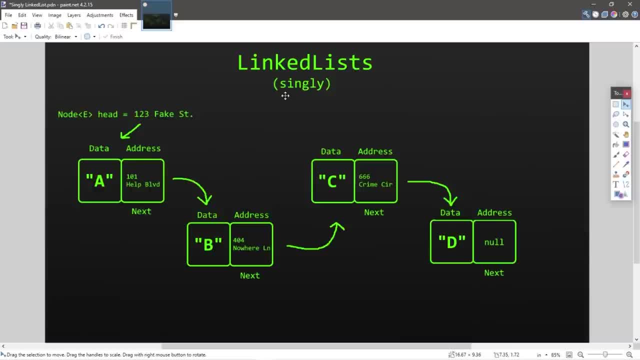 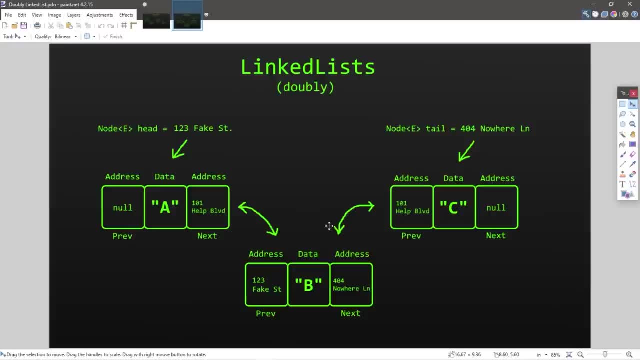 However, there's another variation called a doubly linked list. A doubly linked list requires even more memory to store two addresses in each node, not just one, which is the case with a singly linked list. One address for the next node and another for the previous node in our chain. 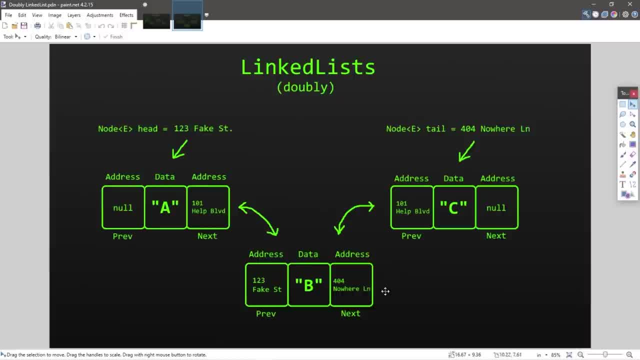 The benefit of a doubly linked list is that we can traverse our doubly linked list from head to tail or from tail to head in reverse. That's a good thing. Everyone knows where the next and previous node is. But the downside is that a doubly linked list uses even more memory than a singly linked. 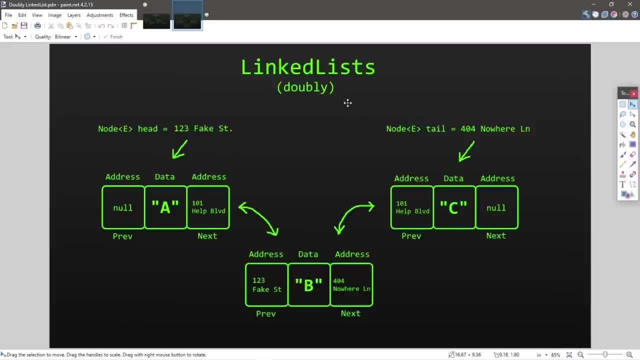 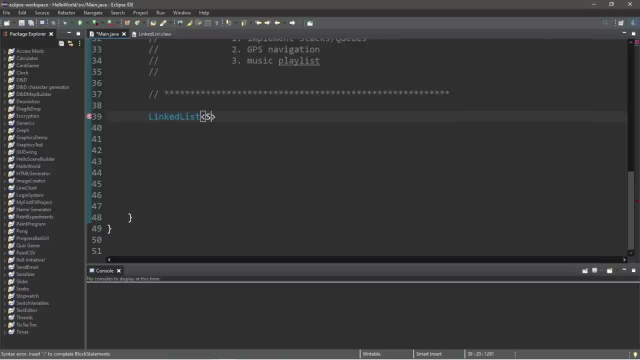 list. So how about we create a linked list in real life? now? Let's do it. All right, ladies and gentlemen. with all of that out of the way, let's create a linked list. Linked List List: the data type of the objects we'll be storing within this linked list: just strings. 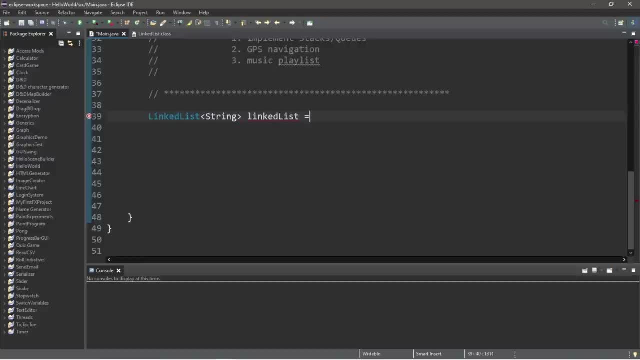 because they're easy, and I will name this linked list linked list. Linked list equals new linked list And list the data type. again, We are storing strings. Add a constructor- Boom, You got yourself a linked list. Now, if I was to take my cursor and hover over my linked list declaration, there's a. 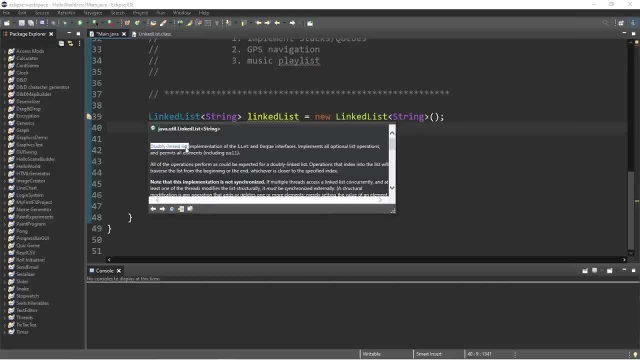 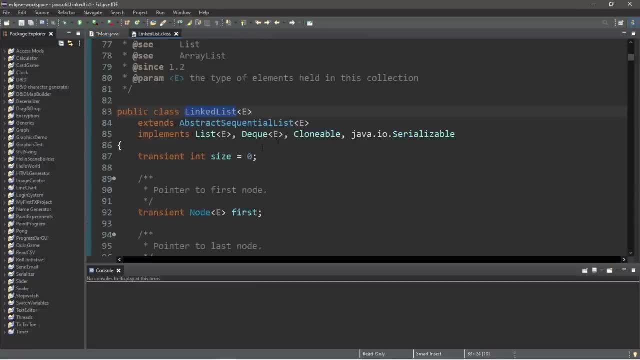 note here that says this is a doubly linked list. Each node knows where the previous and next nodes are. Now, if we head to the linked list class itself, there's a few things I need to mention here. Our linked list stores the memory location of our first and last nodes. 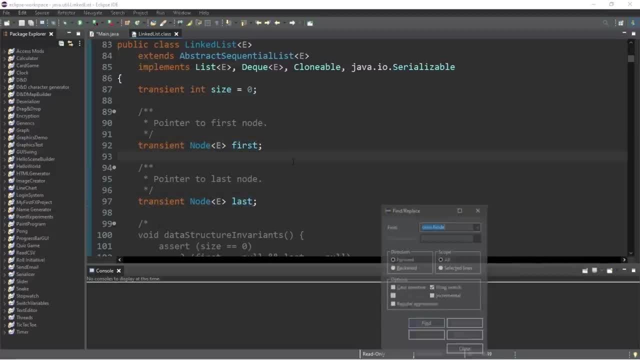 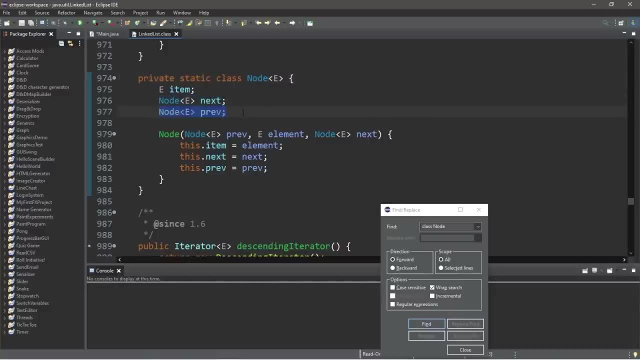 These are effectively the head and the tail of our linked list And there's also an inner class named node. Each node This is the memory address of the next and previous nodes within this linked list. Now taking a look at our linked list class definition. our linked list class implements: 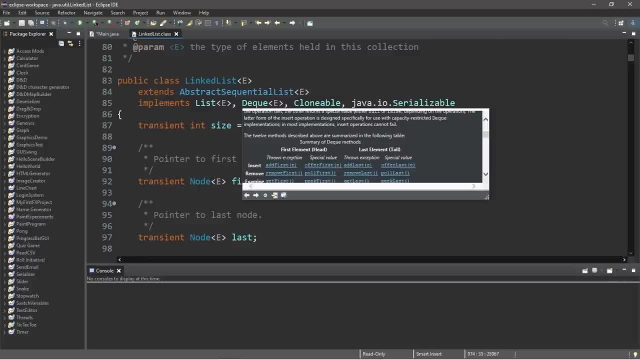 the deck interface, And a deck is more or less a double-ended queue. So with the deck interface we implement 12 additional methods. So here's just a few of them So we can add to the head, add to the tail, remove the head, remove the tail. peek at 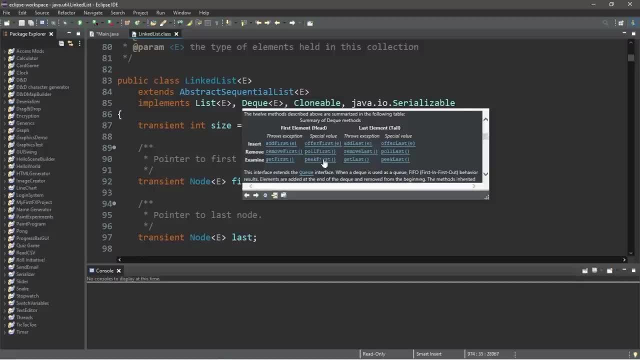 the head, peek at the tail, Some will throw exceptions, Some will return a special value. So you can use any combination of these, really, And not only do we have these 12 methods, but we can treat our linked list as either: 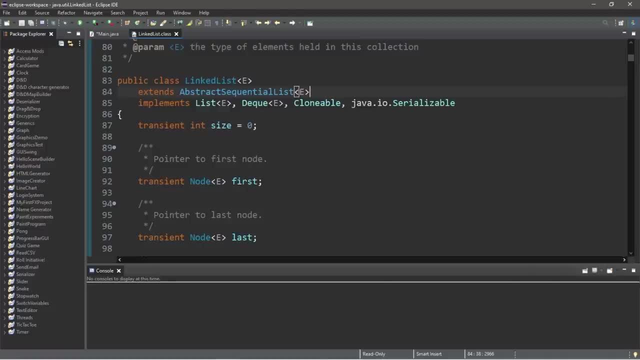 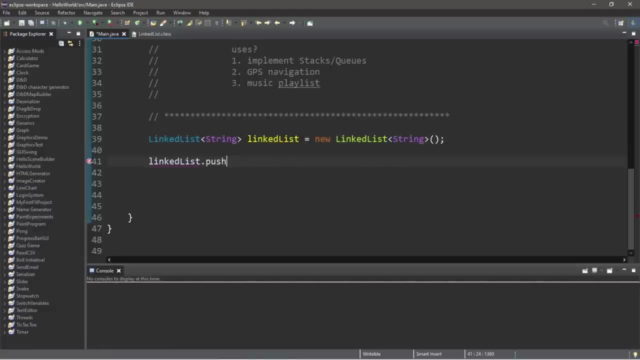 a stack or a queue, We can push, we can pop, we can pull and we can offer. So just to demonstrate, let's first treat our linked list as a stack. So linked lists do have a push method as well. If we need to push an element onto our linked list as if it were a stack, 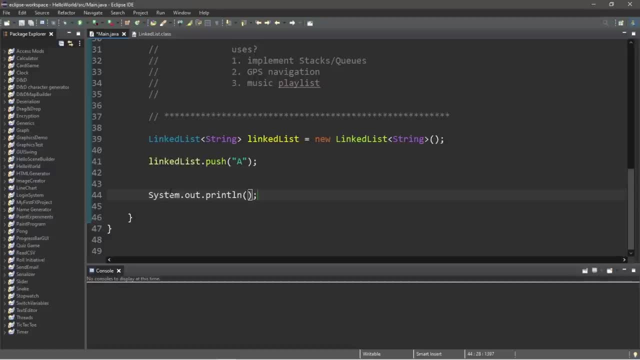 So let's push the letter A and then I will display my linked list with a println statement: Systemoutprintln Linked list. And of course, we have the letter A. So let's push another letter onto our stack. What about B? 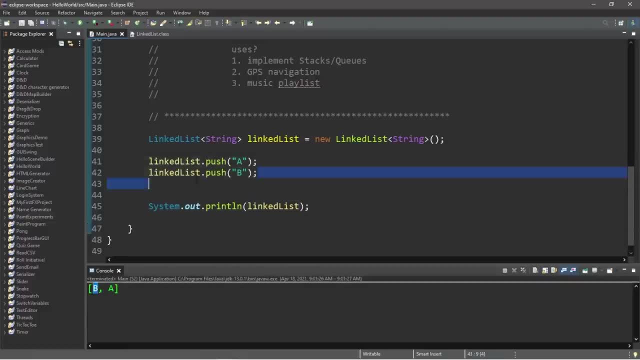 So at the bottom of our linked list we have A and then on top we have B. Let's add a couple more letters. Let's represent a typical grading scale. We have C, D and F, A, B, C, D, F. Notice that I'm intentionally leaving out E- We're. 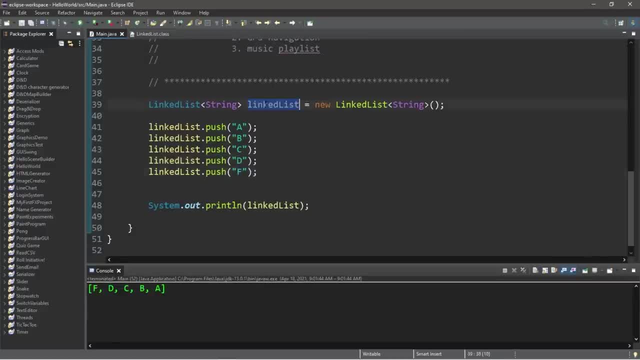 going to insert that later. So within our linked list that's behaving as a stack. we have F on top, then D, C, B and A. We're going to do a pop method as well: Linked listpop- And this will pop the top of my linked list. 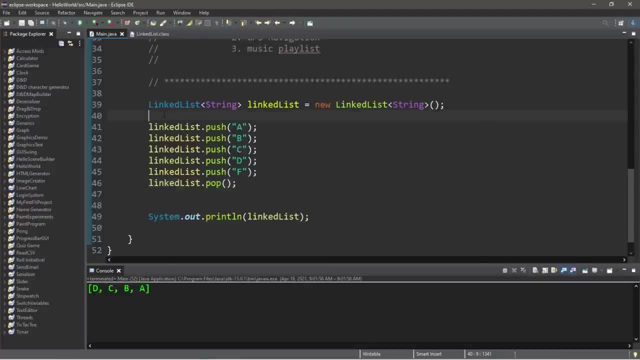 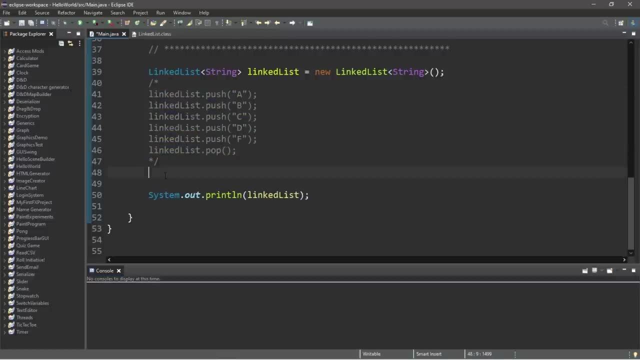 So F should no longer be here. It's D, C, B and A, So we can treat a linked list as a stack. We can also treat it as a queue as well, And just to save some time, I'm going to copy these lines of code. 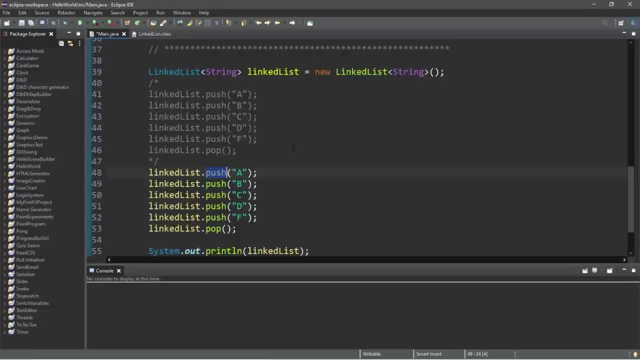 To add an element to a queue. we do not use push, We use offer, So linked listoffer, And we will keep the order, So I'm not going to pop it quite yet. So we have A, B, C, D, F. A is at the head, F is at the tail. 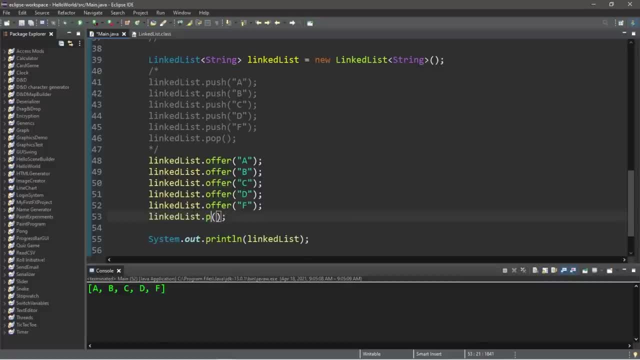 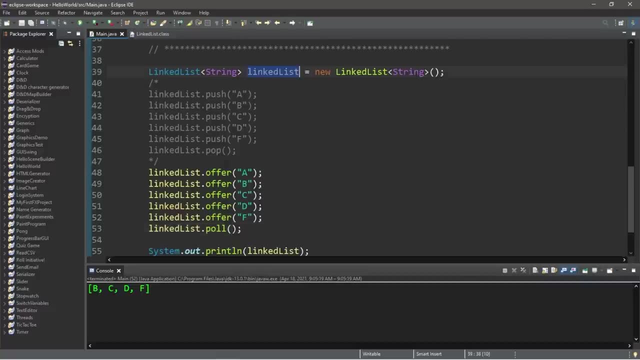 And to remove the head of our queue. we do not use pop, We use pull, And A is no longer in here. We have B, C, D, F, So you can use a linked list to mimic a stack or a queue. 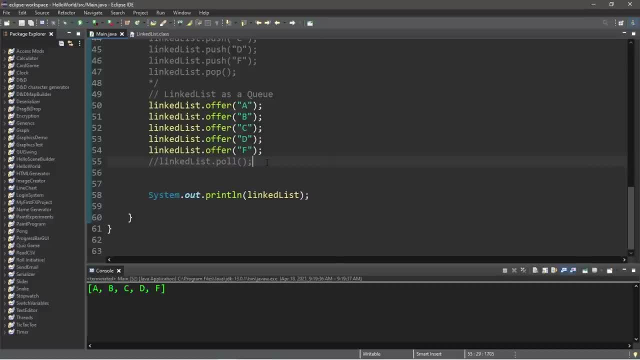 Before we move on to the next section, I'm going to get rid of this pull method, So we have a typical grading scale: A, B, C, D, F. Where linked lists are really good is the insertion and deletion of nodes. 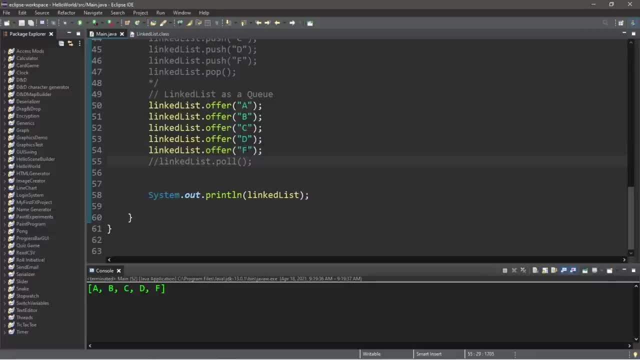 Let's say for this example I need to add a node between D and F that contains the letter E. So that's really easy to do with a linked list. We would type the name of our linked list, dot, add list and index like 4, and our object: 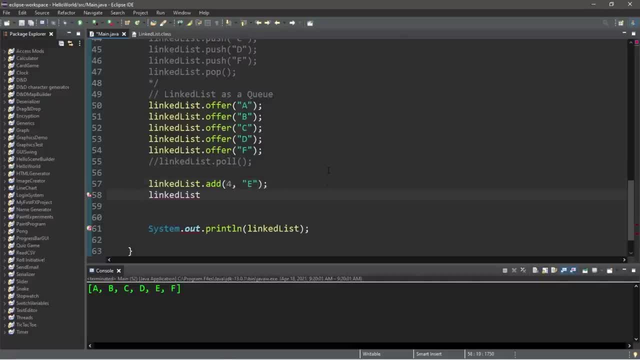 E And then to remove a node we would type the name of our linked list, dot remove, then list the object E. So E should no longer be within my linked list. So where linked lists tend to have an advantage over arrays and array lists is the insertion. 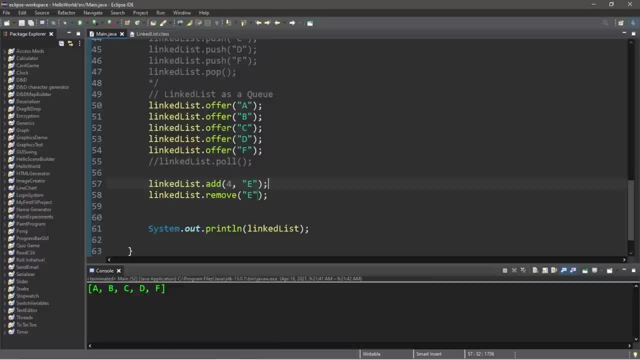 and deletion of nodes. However, there's one catch to this: With a linked list, we still need to traverse the entire linked list to find where we need to go. Unlike with arrays and array lists, there's no random access to a linked list. 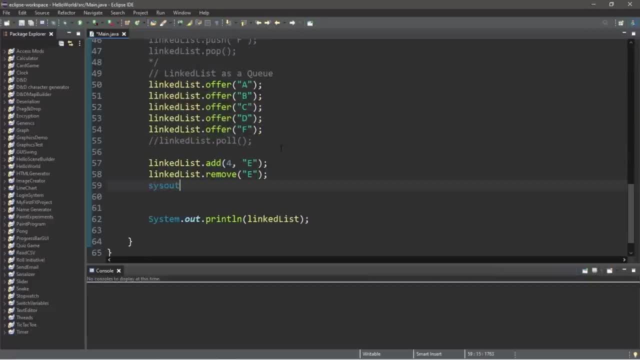 Searching for an element is fairly straightforward too, So within a println statement I'm going to use the index of method of a linked list. Linked list dot index of. let's look for F, So that would be at index 4.. 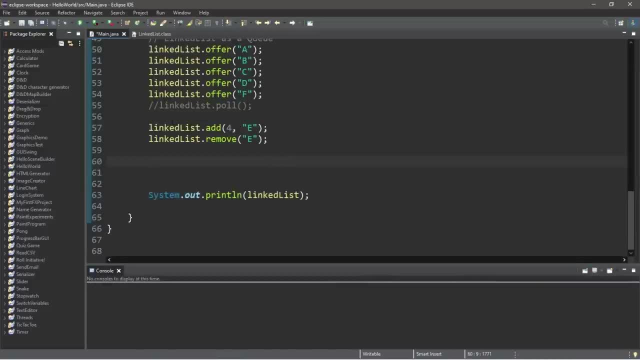 And before we wrap things up here, here's a few methods that we can use. Here's a few methods related to linked lists that you might be interested in. We can peek at the head or the tail node of our linked list. So within a println statement I'm going to print linked list dot and then use the peek. 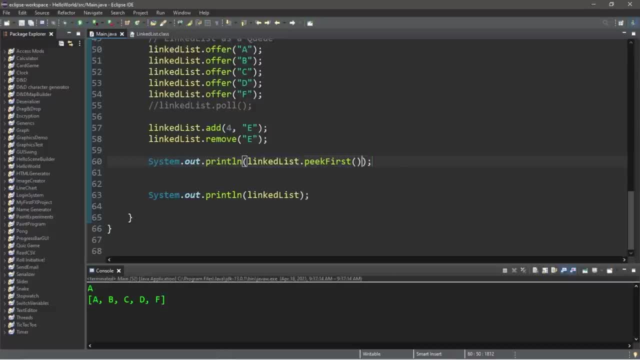 first method. So the first node within my linked list contains the letter A, So we can peek last as well. Linked list dot peek last. And the last node of my linked list contains the letter F. We can add new nodes at the head. 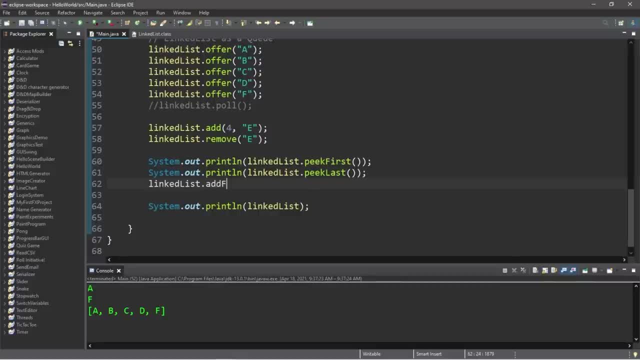 or the tail of our linked list by using the add first method for the head. So maybe I need to add maybe zero, because I don't really know what comes before A in the alphabet. So zero would be a good bet, I guess. 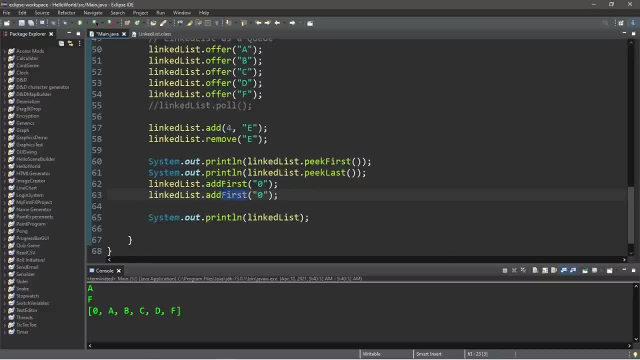 Or we could add to the tail by using add last, And after F comes G, And we now have G at the tail of our linked list. We can remove first and remove last. You can also store them within a variable too. Let's say, string first equals linked list, dot remove first. 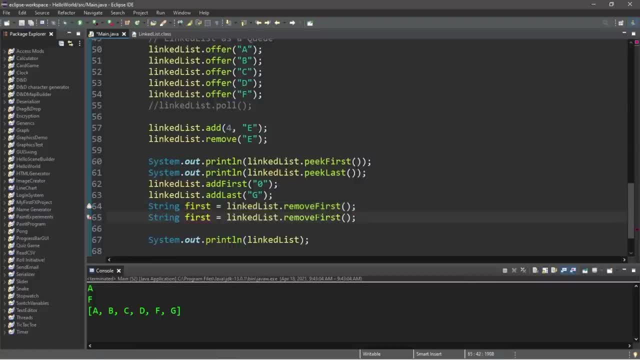 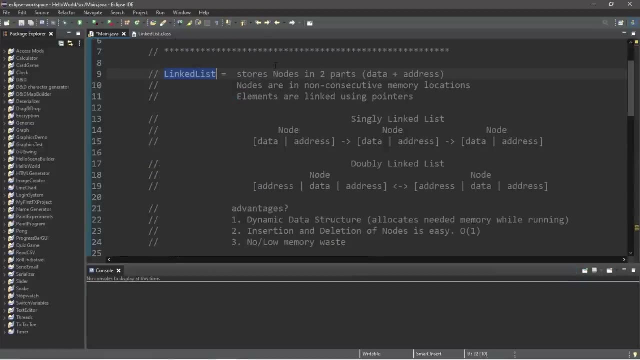 Then to remove the last node, we could just use: remove last, then, And let's store this within a different variable: remove last. So yeah, those are a few useful methods related to linked lists. In conclusion, everybody, a linked list is a data structure that stores a series of nodes. 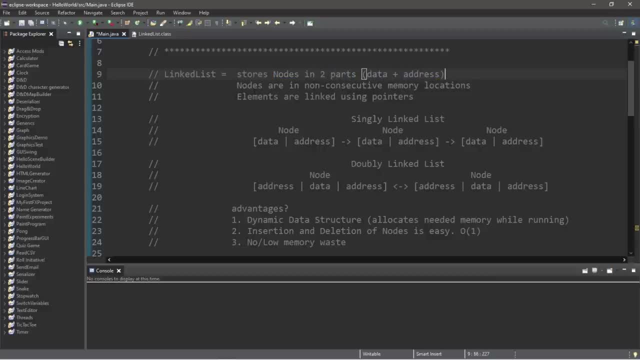 Each node contains two parts: Some data And an address. Nodes are stored in non-consecutive memory locations. Each node can be really anywhere within your computer's memory And elements are linked via these pointers. They contain an address for where the next node is. 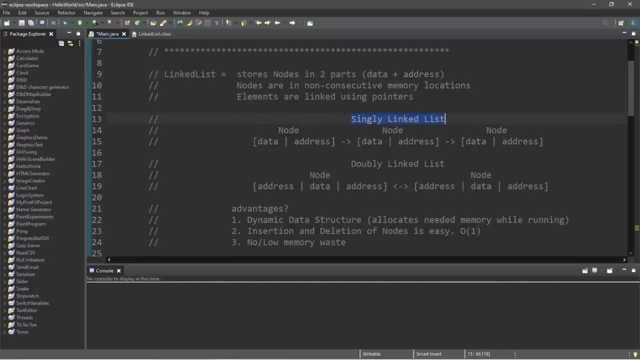 We've discussed two varieties of linked lists: a singly linked list as well as a doubly linked list. With a singly linked list, each node is made up of two parts: some data and an address. To traverse a singly linked list, we would begin at the head node and use the address. 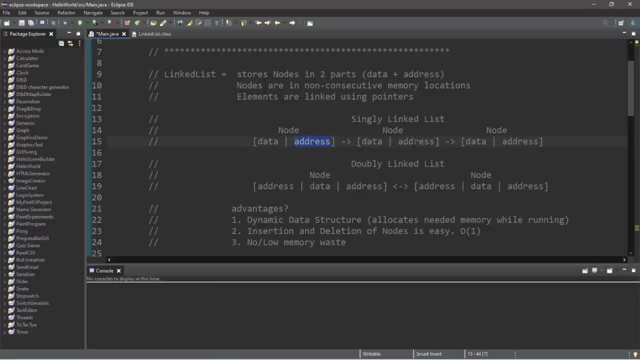 as a sort of clue to find where the next node is located within our computer's memory, With a doubly linked list. each node is made up of three parts: some data and two addresses- one address for the next node and another address for the previous node- and it behaves. 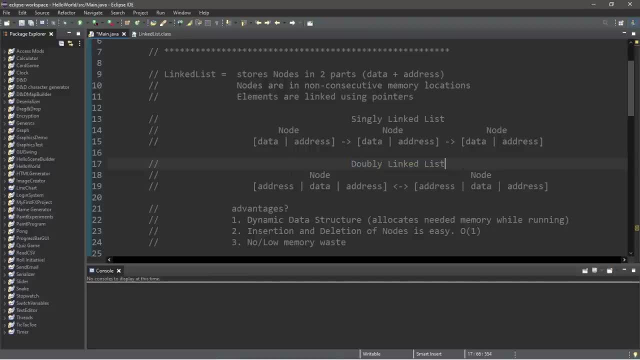 the same way And to traverse a doubly linked list. we could begin at the head and work our way towards the tail, Or we could begin at the tail and work our way towards the head, depending on which way is closer to where we need to be within our linked list. 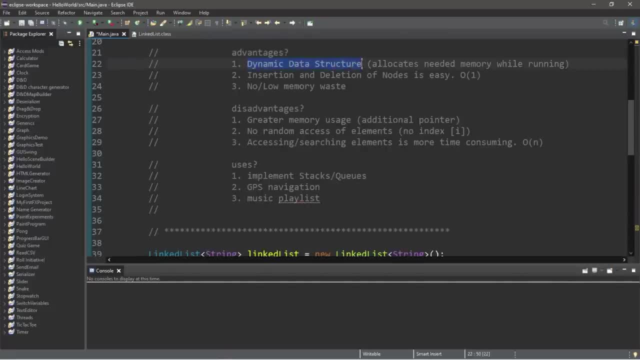 What are some of the advantages of a linked list? One: they're a dynamic data structure. They can allocate needed memory while our program is currently running. Two: insertion and deletion of nodes is really easy. If you're familiar with big O notation, this would be in constant time. 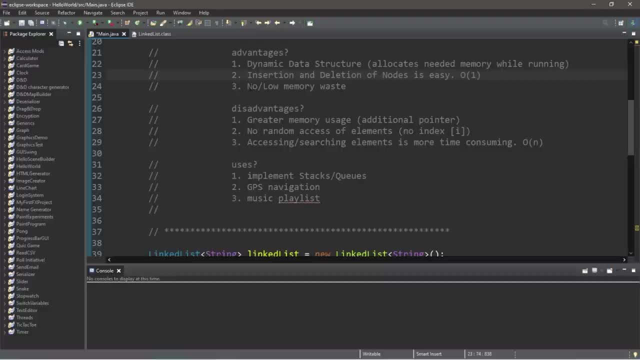 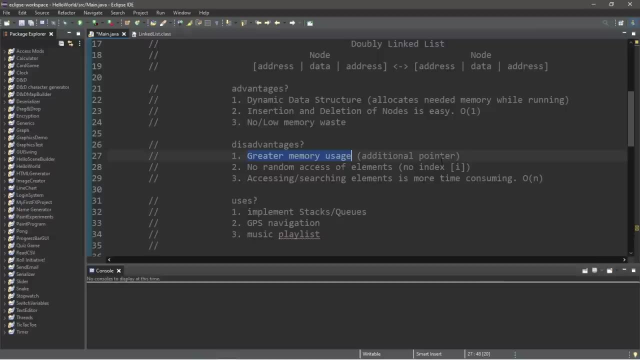 There's only a few steps, regardless of the size of our data set. And three, there is no too low memory waste. What are some disadvantages? One: there is greater memory usage because we have to store an additional pointer. Each node also stores the address for where the next node is located. 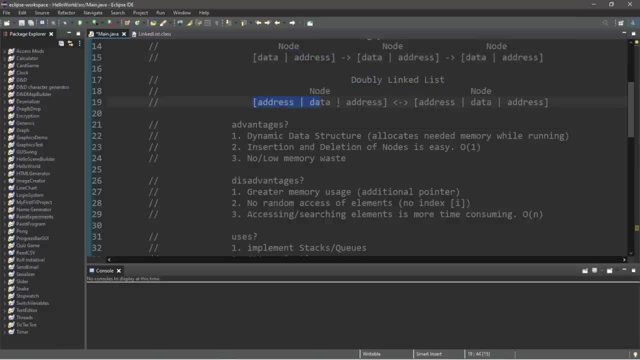 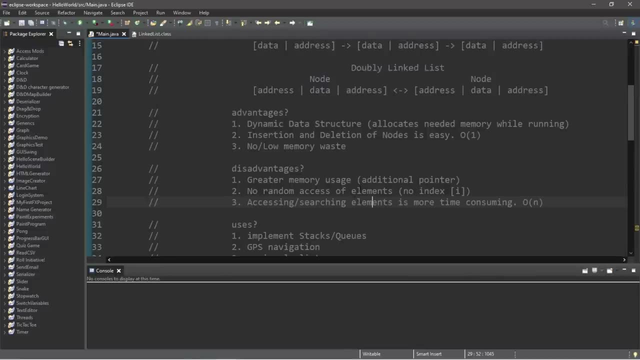 And even more. there is no too low memory waste, Even more so with a doubly linked list. This will use a lot more memory because we need two addresses for each node, Now two. there's no random access of elements within a linked list. 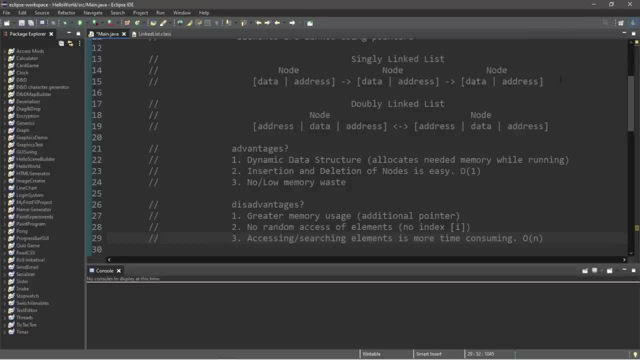 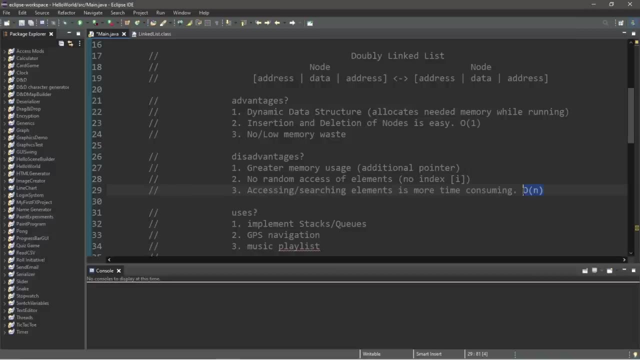 To find an element, we need to begin at one end and work our way towards the other end. And three: accessing and searching of elements is more time consuming. This is done in linear time. This is where arrays and array lists have an advantage. 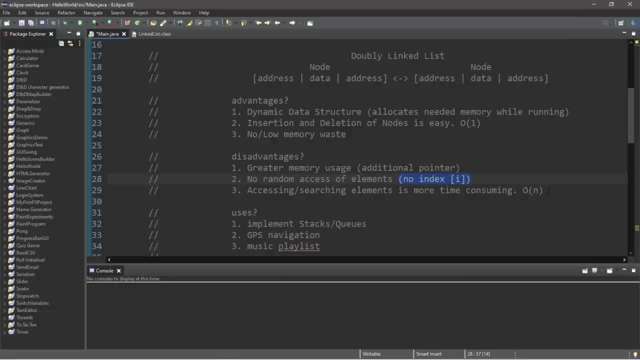 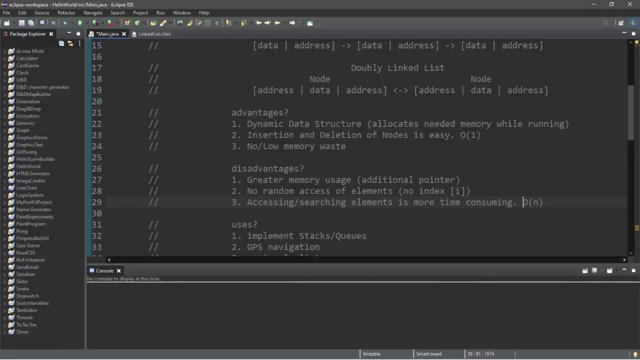 Since they use indexing, they can randomly access an element of an array or an array list. With a linked list, we have to manually traverse the entire linked list to get to a particular index, since we don't have random access. Now, what are some uses of linked lists? 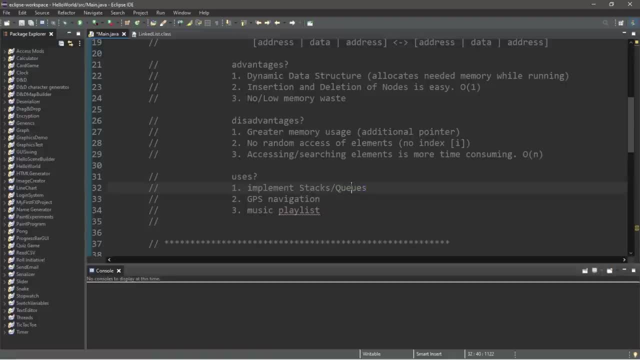 One, they could implement stacks or queues. If you need a stack or queue for anything, you could also use a linked list. Two, maybe GPS navigation. So let's say you have a starting position and a final destination. Each step or stop along the way is kind of like a node. 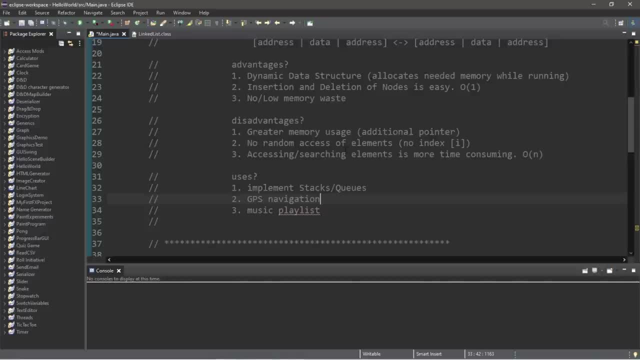 And if you need to take a detour, you can easily change, insert or delete a node and recalculate how to use it. Three: what about a music playlist? So each song within a playlist might not necessarily be next to each other within your computer's. 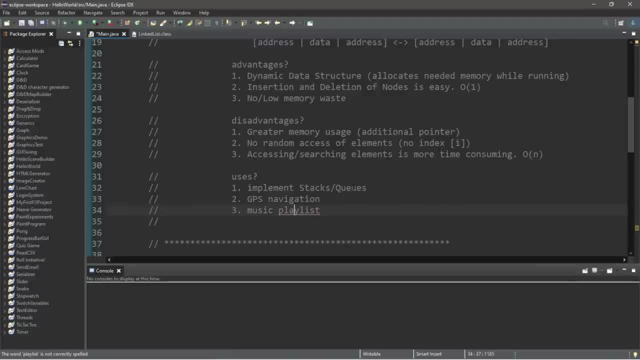 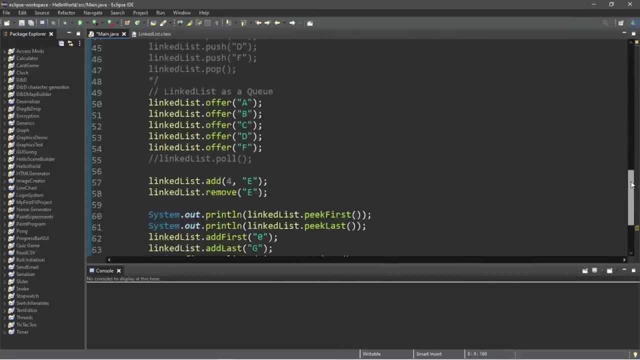 memory. You want your playlist to follow a certain order of songs, So that could be another use of a linked list. So those are linked lists. If you would like a copy of all my notes here and my code, I will post this to the comments. 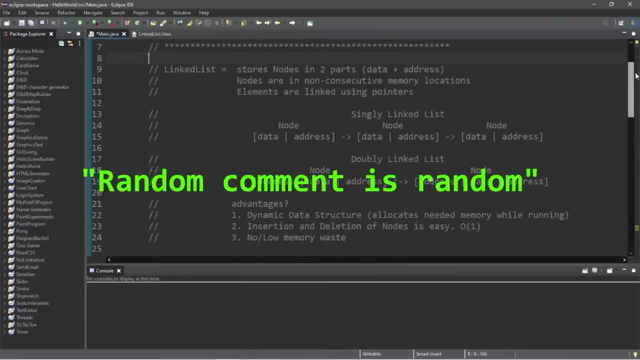 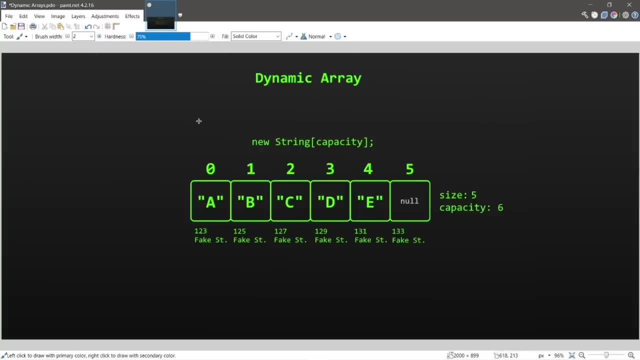 section down below. If you can give this video a thumbs up, drop a random comment down below and well, yeah, those are linked lists in. what the heck is it? What the heck is a dynamic array? A dynamic array is an array with a resizable capacity. 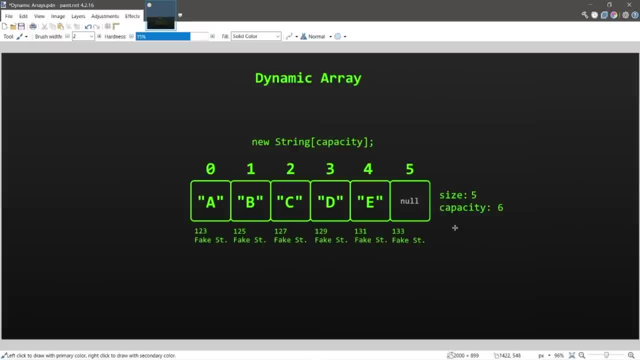 If we need extra room for elements, we can increase the capacity, which we cannot normally do with a standard, typical fixed-size array. Dynamic arrays are also known as ArrayList in Java, Vectors in C++, Arrays in JavaScript and Lists in Python. 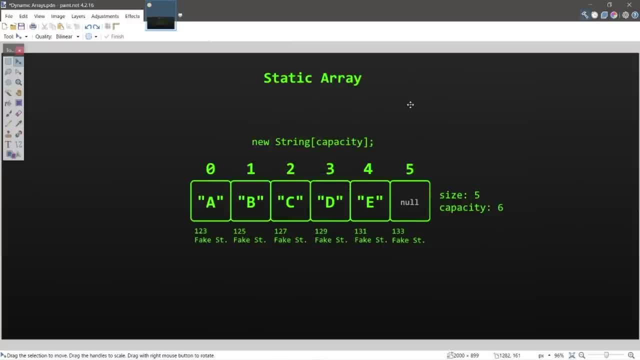 Here's an example of a static array, and then we'll take a look at a dynamic array. A static array has a fixed capacity. We determine that capacity at compile time And we can't change it later. normally, In this example I have a static array with a capacity of six elements and a size of five. 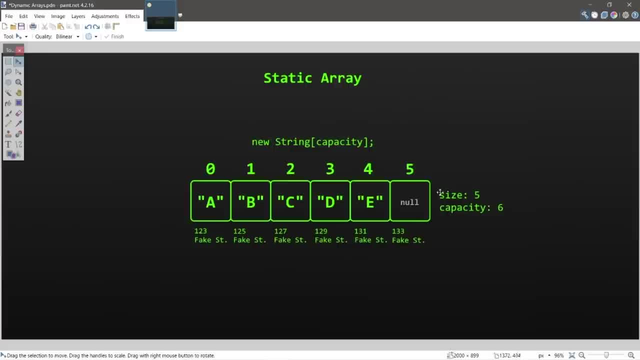 elements that are currently occupied. The last element is open, so it's null. Each element has a memory address. Obviously, these are not real memory addresses, but this is how I like to think about things. Imagine that all of these memory addresses are houses and they're all next to each other. 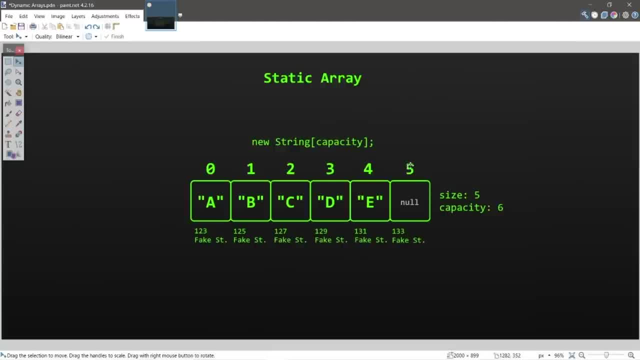 Now accessing an element is easy because we have index numbers to work with. We can randomly access an element in O constant time. The size of our dataset doesn't matter. However, searching for a stored value still takes time because we need to begin at index. 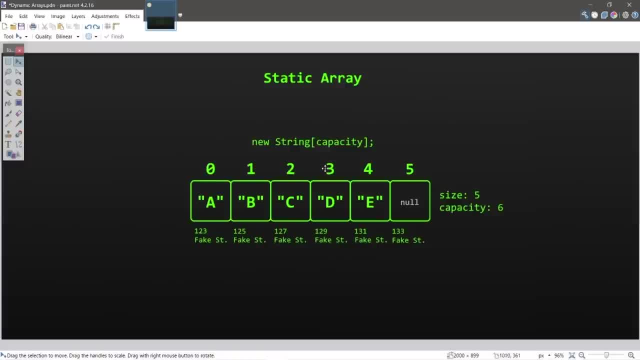 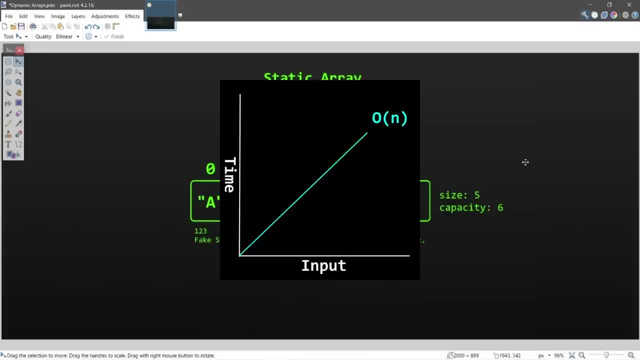 zero and iterate over our array until we reach our value or the end, in case we don't find it. This is done in O linear time. The larger the dataset, the time to finish will increase linearly And in the case of inserting or deleting that takes linear time unless done at the 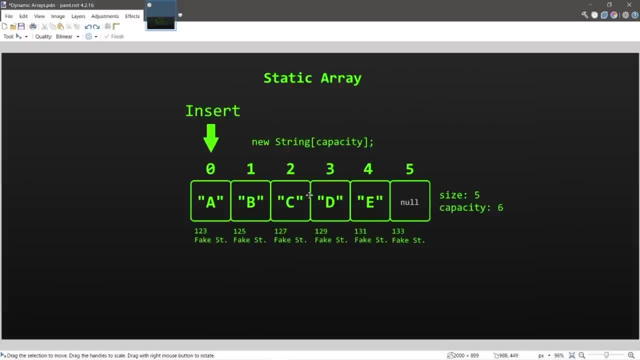 end, No shifting of elements is required. However, the closer we need to insert or delete to index zero, we need to shift all elements that follow. This is done in order to make room for insertion or close any gaps in the case of deletion. 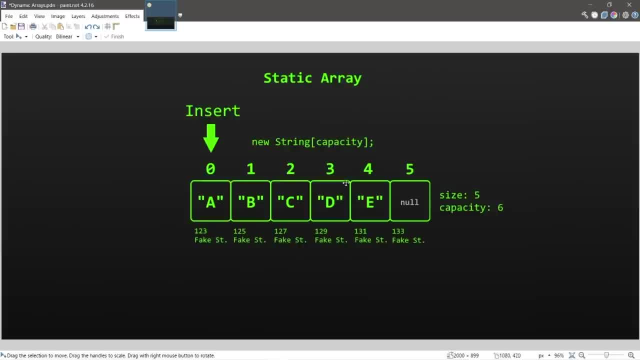 So if I need to insert a value at, let's say, index zero, I have to shift all elements to the right by one to make room for this insertion, And then we can insert a value. Now, currently, with our static array, we're at capacity. 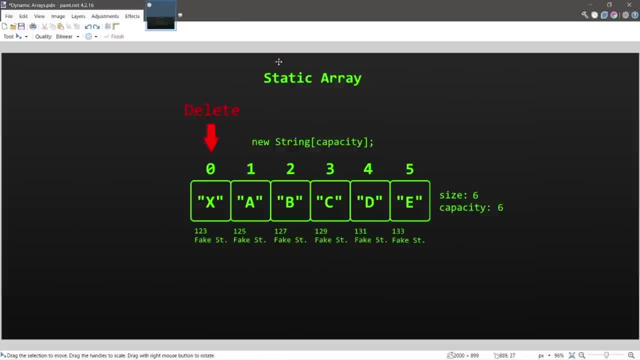 Our array is full. Our size is equal to our capacity. Then, in the case of deleting an element, we need to shift all elements that follow after this index where we're making the deletion, And shift everything once to the left. So that would look like this: 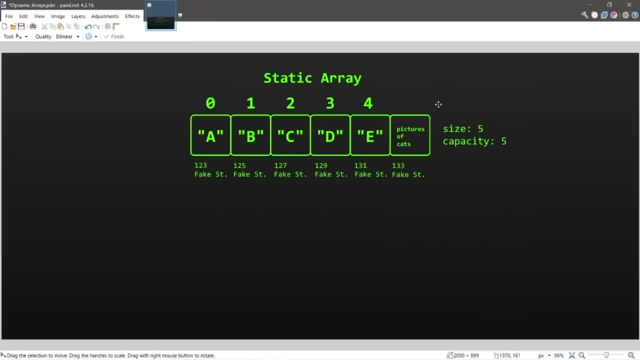 And our size is back to five. So there is one element that is open. A major disadvantage of static arrays is that they have a fixed capacity. We can't increase the capacity once the size of the elements reaches capacity. In this separate example, I have an array with a capacity of five elements and a size. 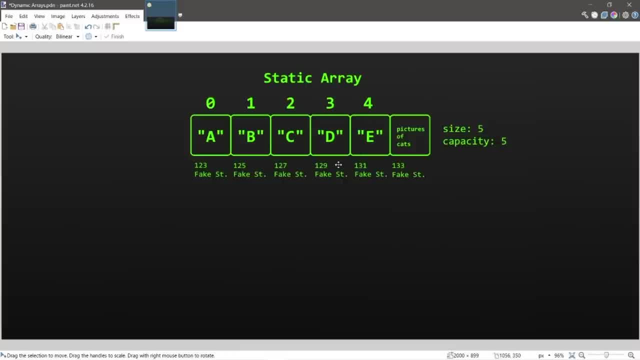 of five elements and it's completely full. I can't decrease the capacity because the next memory block contains the same number of elements. The next memory block contains, I don't know, pictures of cats or something You do, you, I guess. 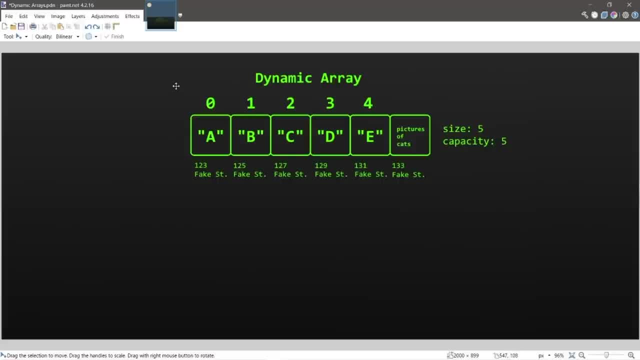 A dynamic array has its own inner static array with a fixed size. Once the inner static array of our dynamic array reaches capacity, our dynamic array will declare and instantiate a new array with an increased capacity. Usually, the amount that we increase the capacity by really varies depending on the programming. 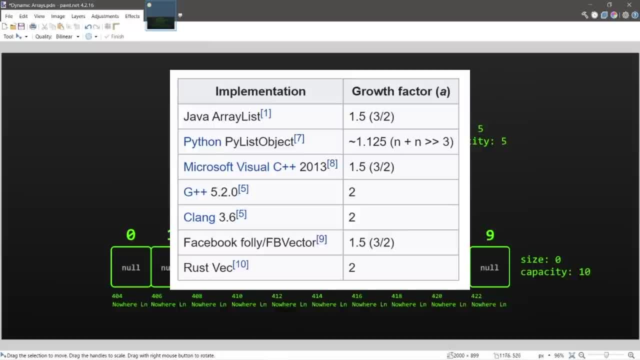 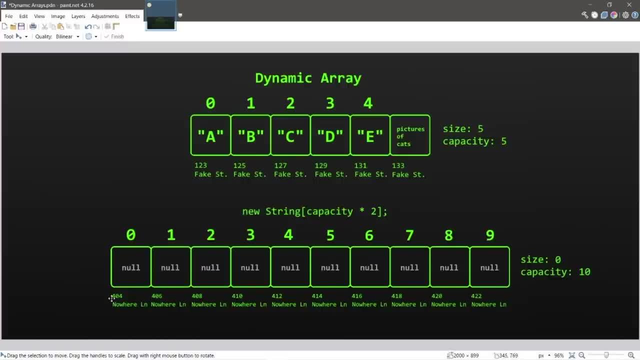 language. It's usually between 1.5 and two. I just picked capacity times two for extra emphasis. So what we'll do now? We'll copy the elements over to our new array, and these have different memory addresses than our original array. 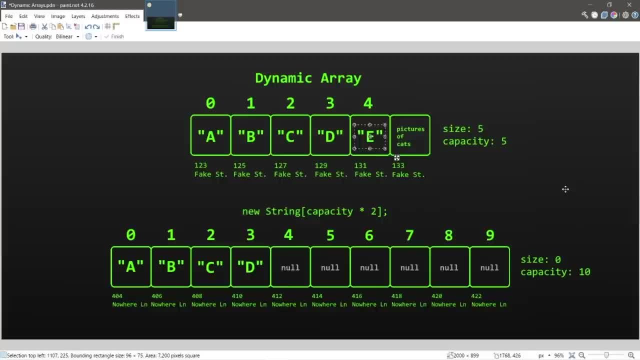 So that would look something like this: We now have a new array with double the capacity, but, like I said, it really depends on the language that you're working with. It's usually between 1.5 and two. This array has a size of five elements that are full and a total capacity of 10.. 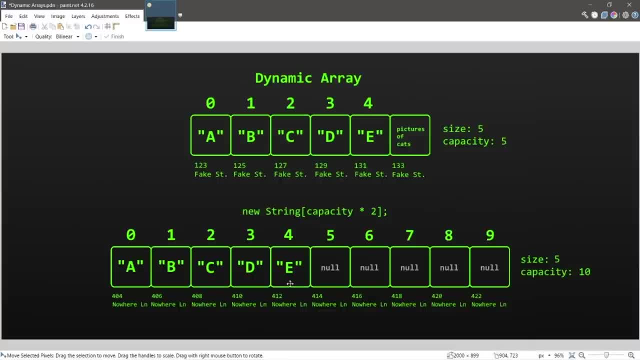 Then if you need to shrink the capacity, like if you're not using a lot of elements, you can always just do the reverse process of what we did to increase it. Now, with this new inner array, the insertion and deletion of elements is really the same. 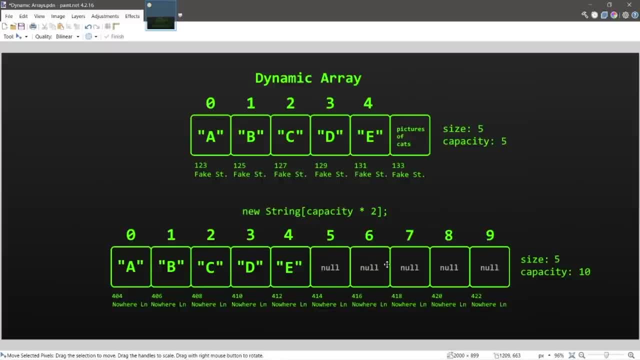 as a static array, So you just shift all the elements to the right by one to insert a new element, or shift all the elements to the left to delete an element. What are some of the advantages of dynamic arrays? One: there is random access of elements that is done in O of one constant time. 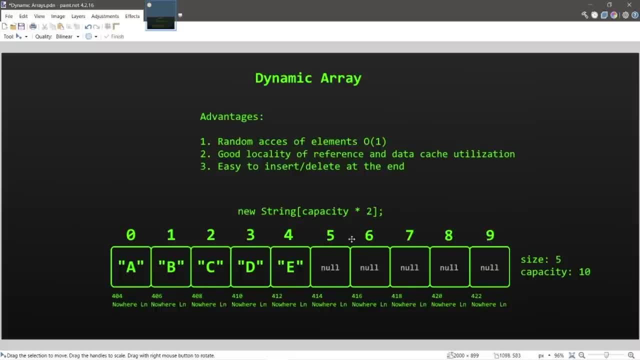 We can randomly access an element by an index number and retrieve the value. Two, There is good locality of reference and data cache utilization because all of these memory addresses are contiguous- They're right next to each other, Unlike with linked lists. you have to jump around a lot because all of the memory addresses 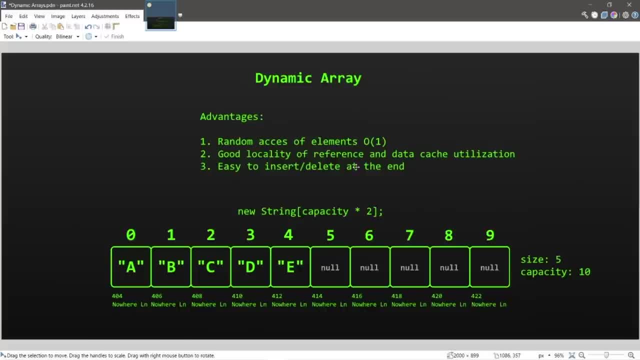 are kind of random. And three: it's easy to insert and delete elements at the end because there's no shifting of elements required. And for the disadvantages: a dynamic array wastes more memory than a linked list. because we need to increase the capacity to accommodate more elements if we need the extra room and 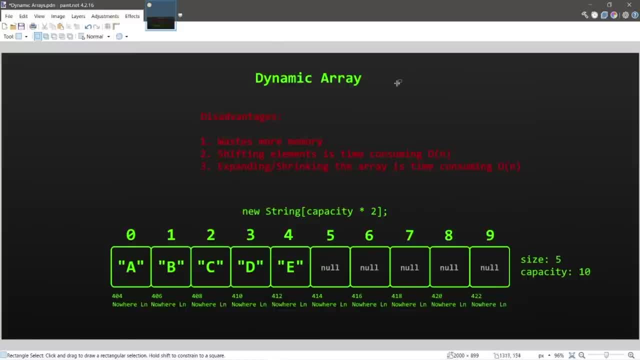 we may not necessarily need all of this extra room, So a dynamic array wastes more memory than a linked list. Two: Shifting of elements is time consuming. The closer we need to insert or delete, closer to index zero we have to shift all elements. 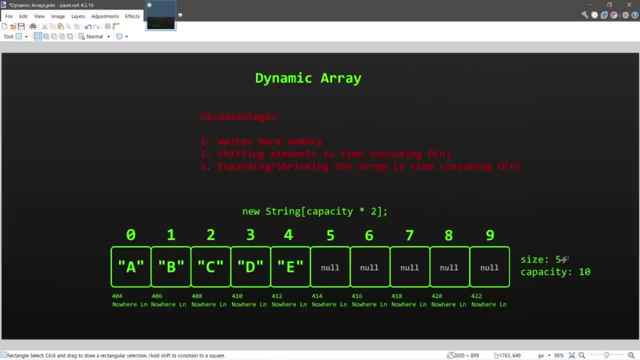 that follow afterwards- to the right in case of an insertion or to the left in case of a deletion, And three: Expanding or shrinking the array is time consuming because we have to copy all of the elements over to a new array with a different capacity. 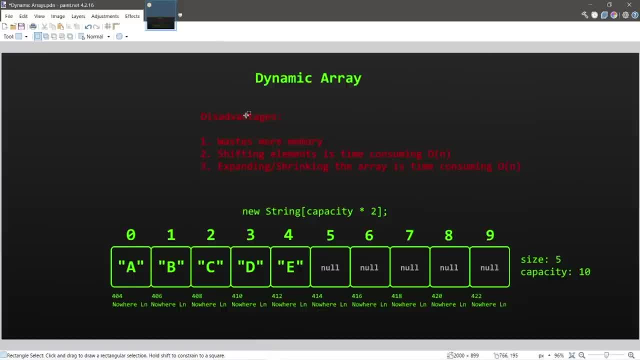 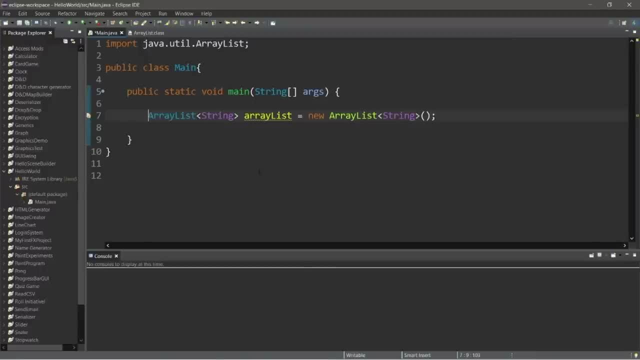 So that's one of the advantages of dynamic arrays And that's the basics of dynamic arrays. Let's create our own dynamic array for practice. Alright, welcome back. We're going to create our own dynamic array using Java. In the future, if you ever do need a dynamic array, you might as well just use an array. 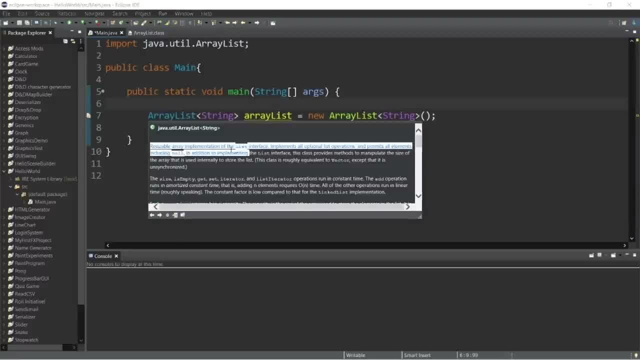 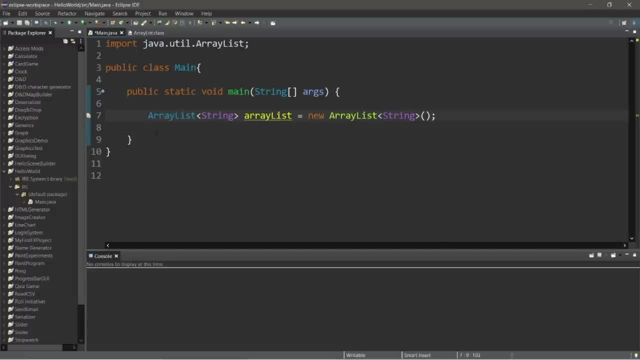 list. According to the description, it's a resizable array implementation of the list interface and it's prebuilt, so you might as well use it. I thought we would create our own dynamic array, just for learning purposes and practice. But let's take a look at the ArrayList class. 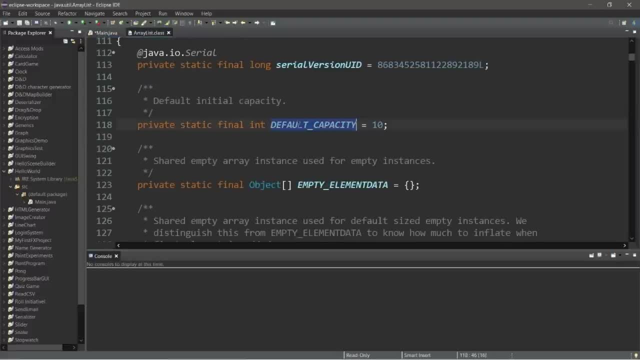 Within this class. there are a few things that we can do. First, we need to create a dynamic array. In this class there are a few defined members. There is a default capacity set to 10.. There are overloaded constructors within this ArrayList class. 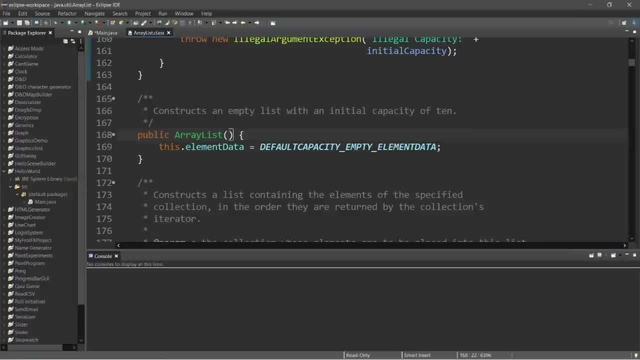 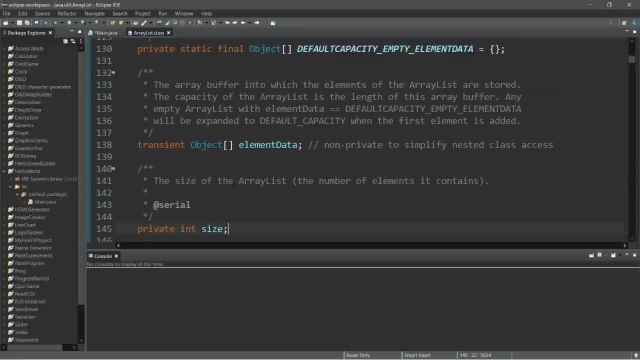 We can set our own initial capacity or we can use the default by not passing in an initial capacity. There is a size to keep track of how many elements are filled within our ArrayList, And our ArrayList does have its own inner static fixed size array. 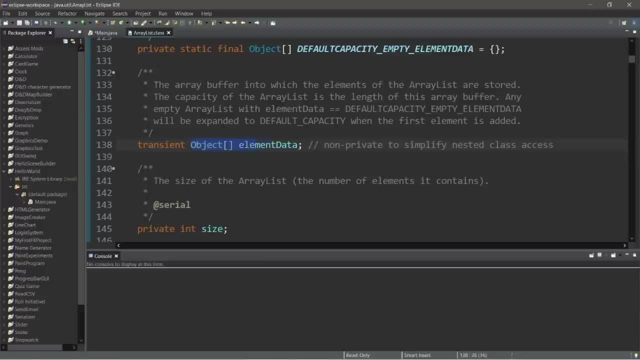 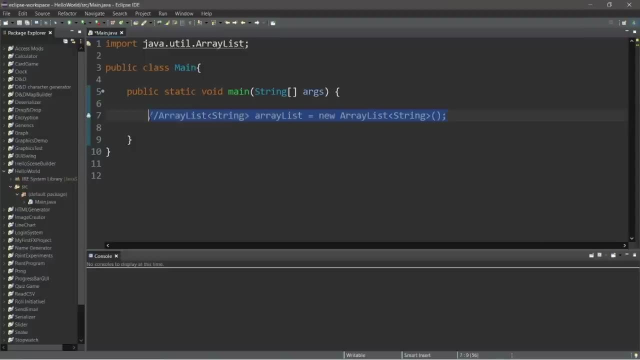 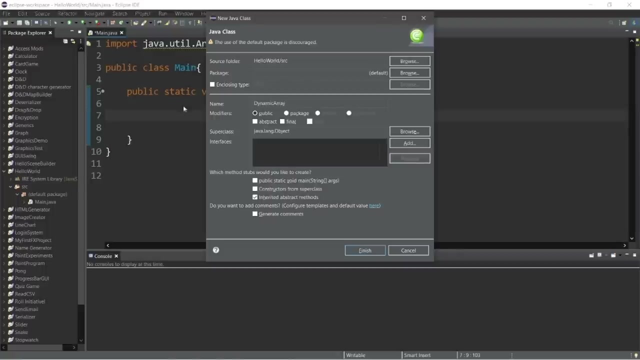 And if we ever need to expand the size of this array, we just copy the elements over to a new inner array. So let's begin. Let's create a new class named dynamic array and I'll get rid of this. So file new class and this will be named dynamic array. 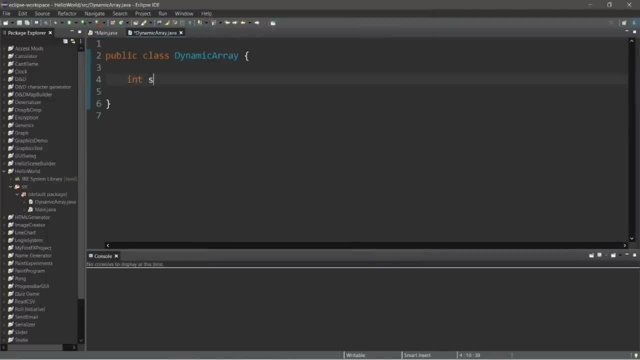 Then finish. Okay, let's declare a few members. Let's create int size, int capacity. this will be the initial capacity. I'll set this to 10, but feel free to pick whatever value that you want, As well as an array of objects named array. 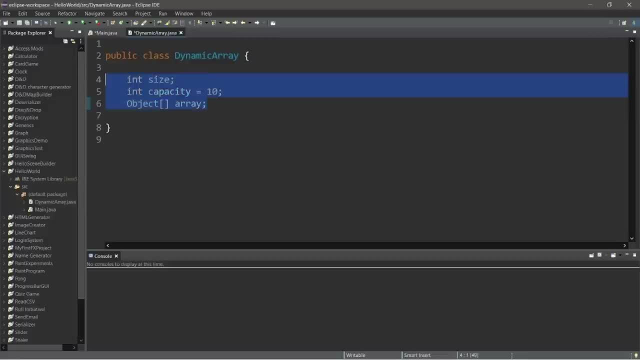 I will declare this, but not yet, in std, So you can make these private. however, I think that'll make our code a little more complex and difficult to understand, although it'd be more secure. I'm just going to use the default visibility for these members here. 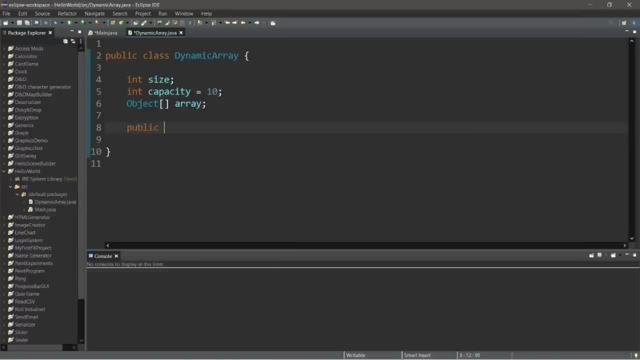 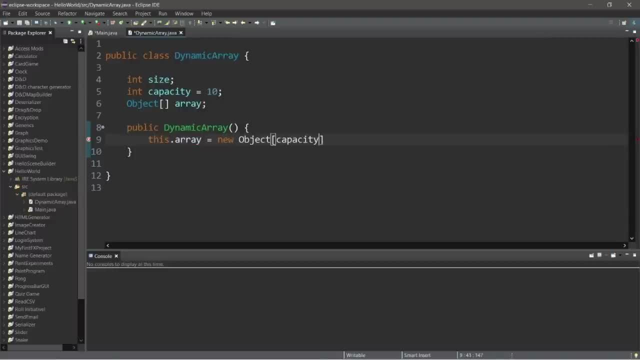 This dot array equals new. This dot array equals new- I'm going to make this- are of objects with a capacity, of whatever capacity the default is. So it's going to be 10 by default And we'll create an overloaded constructor just in case the user passes in their own. 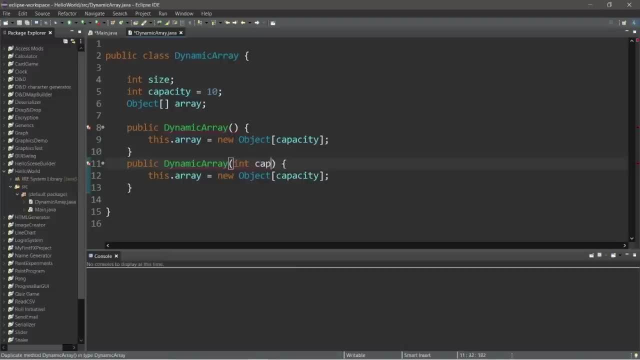 capacity they would like to set, So int capacity. this dot capacity equals whatever capacity that we pass in. Ok, let's instantiate a new dynamic array: DYNAMIC- Spell it right: Dynamic array. I'll call this dynamic array. with a lowercase d equals new. 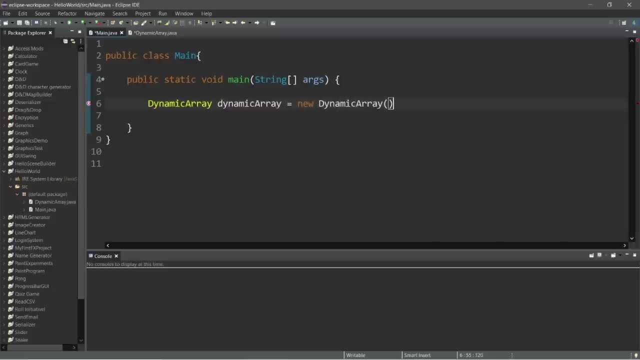 dynamic array. So I'm not going to pass in an initial capacity And let's print whatever the capacity is of our dynamic array: Dynamic array, dot capacity, And this should be 10.. Okay, now let's pass in maybe a capacity of five, And this should be five. Yep, cool, So it seems like that. 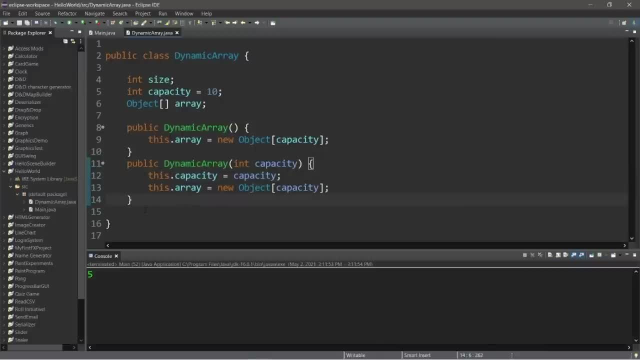 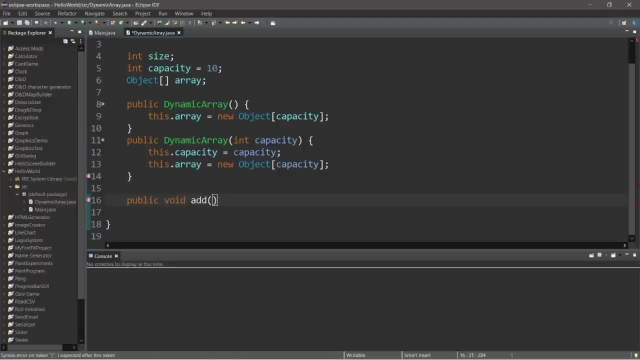 works. All right, let's head back to our dynamic array and declare all of the methods that we'll need. Let's create an add method- Public void add, And there will be one parameter of object data. Next method: insert: Public void insert. 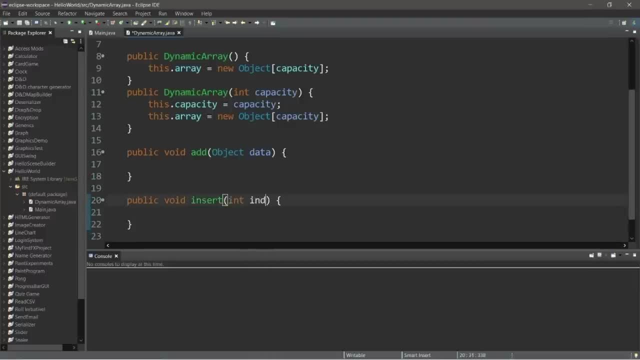 The two parameters of object data. The two parameters are: int- index object data. Okay, next method: we have delete Public void. delete. There is one parameter of object data. Then we have search Public int. we're going to return an index search. 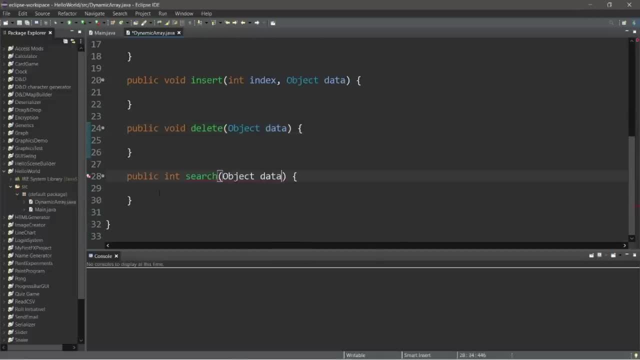 And we will need Object data And let's return negative one for now. Then we have private void grow to expand the size of our array. Private void shrink. Then we'll need an. is empty. method Public. we will return a. boolean value is empty And we might as well fill this in right now. So we're going to need an. 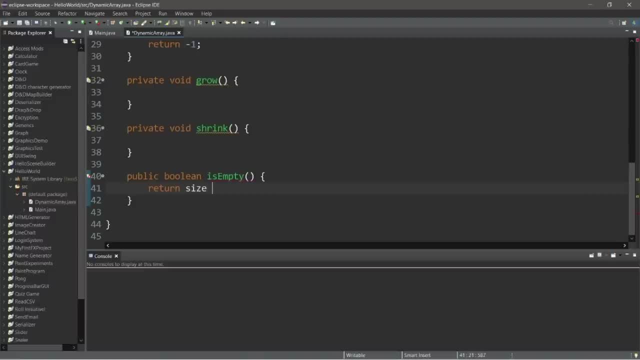 add method right away, because there's only one line: Return size is equal to zero. If our size is anything but zero, we will return false. And lastly, to string: Public string to string And I need to type in something. I'm just going to return null for the time being, until we return. 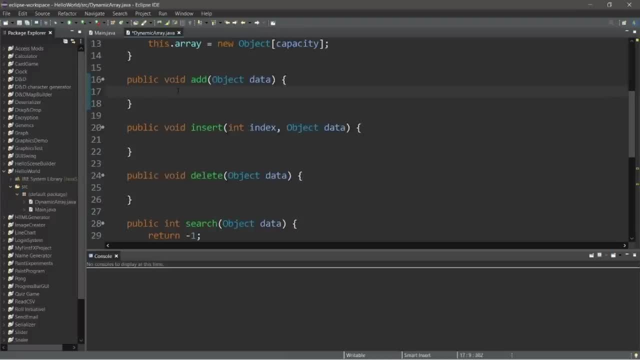 something. Okay, let's begin by filling in the add method. First, we'll want to check to see if we're at capacity. We're going to need to type in something. We're going to need to type in something. If our size is greater than or equal to our capacity, then we better call the grow method to. 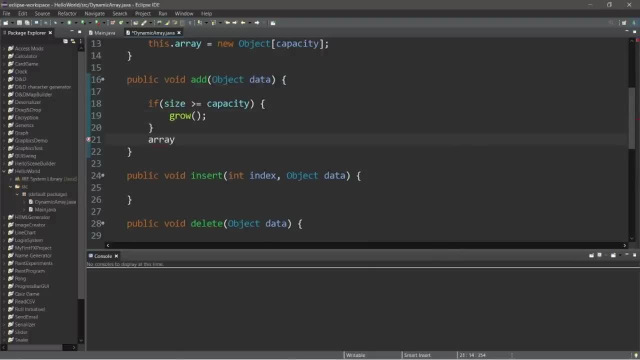 expand the size of our array. So if there is room, we will take our array at index of size. that should be the end of our array, equals data. Then we will increase our size by one. Now let's head all the way down to the toString method to display the elements of this array, And we just need to. 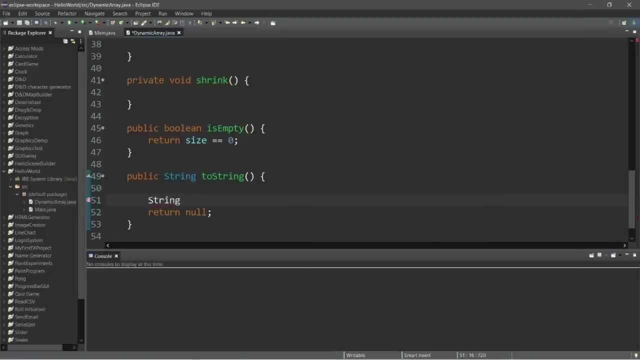 iterate over these. Let's declare a local variable of string, String, string- And I will set this equal to an empty string And we will fill in the elements when we iterate over it. So let's iterate over the elements of our array. So let's create a for loop for int, i equals zero, And then I will continue this for. 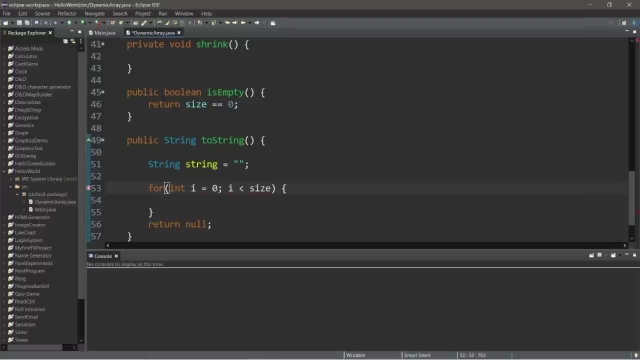 loop as long as i is less than our size. You can do capacity too if you want to see the entire array. But let's begin with size And I will increment our index i by one. So I'm going to take our string and append it. String plus. 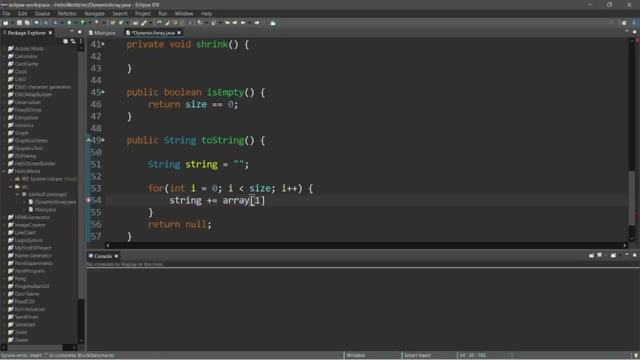 equals our array at index of i, that's one i plus maybe I'll add a comma, then a space. Then we should return our string string. Okay, this isn't perfect yet, but let's at least test it. Let's head. 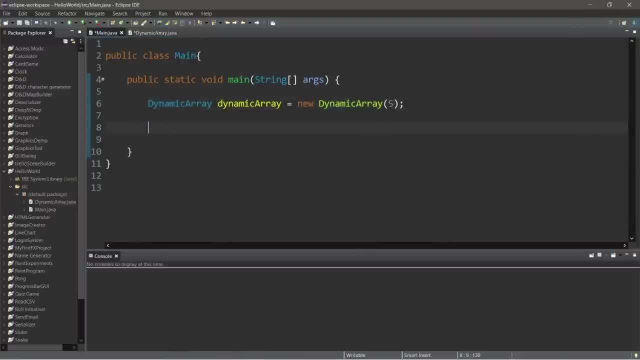 back to our main Java file and add a few elements to our array using the add to string method. So let's use the default capacity of 10. So we don't necessarily need to pass in anything. So to add to our array we can use dynamic array dot and we declared an add method at the top. 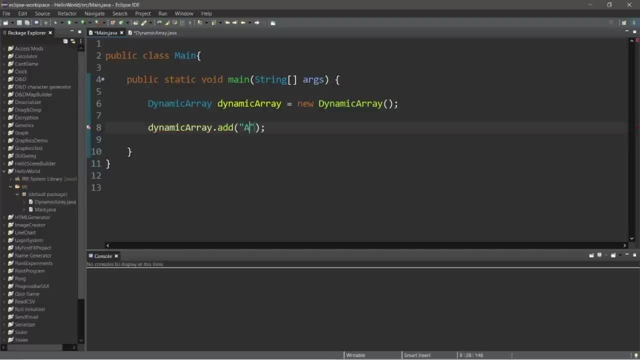 So let's add maybe some letters. I will add the letter a, then b, then c. That should be good. So a, b and c, And then let's call the to string method, systemoutprintln, And with the to string method we only have to type in the name of what we would like to. 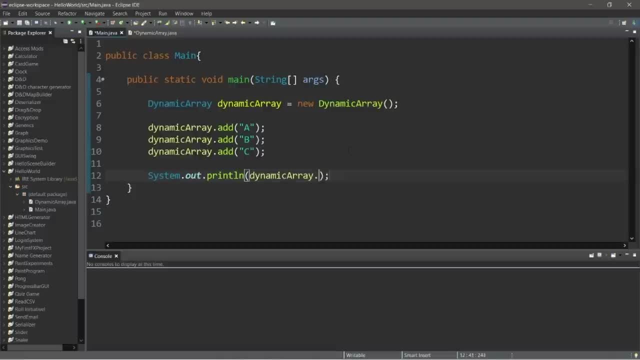 display the elements of So dynamic array and we don't necessarily need to type to string. So this should display a, b and c. Now let's format this and clean it up a little bit, Like I would like to get rid of the last comma here and maybe enclose all of these elements within a set. 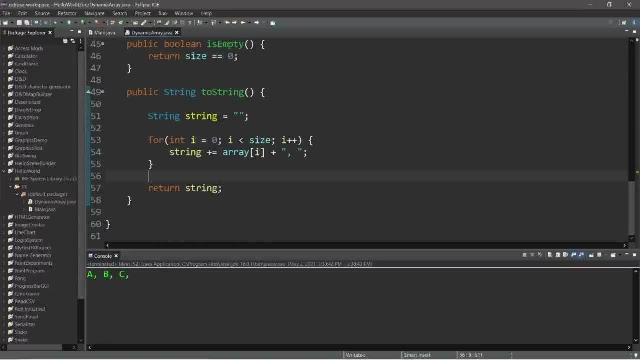 of square brackets. So this is what we can do within the to string method. So after the for loop, let's check to see if our string does not equal an empty string. If that is the case, if there are elements to display, 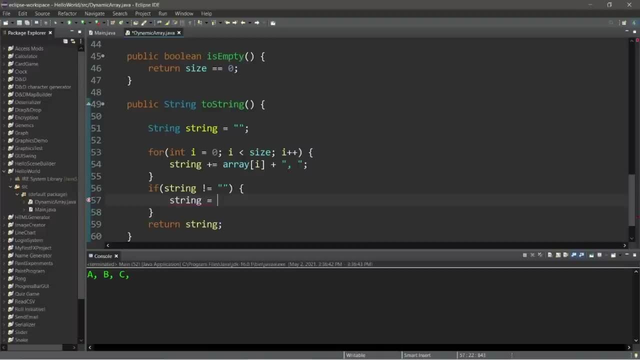 let's take our string, Then I'm going to create a substring and get rid of these last two characters, the comma and the space. So string equals string dot substring And the length is going to be beginning at index zero And I will continue this until string dot. 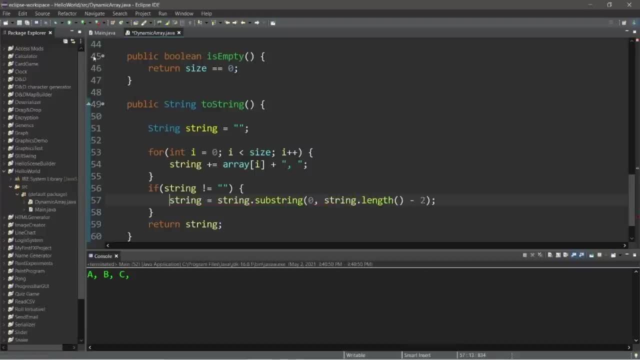 length method Minus two. Then, after running this one more time, the comma and space at the end should no longer be there because we created a substring to end at the last element. Then let's enclose all of these elements within a set of square brackets, So I'll 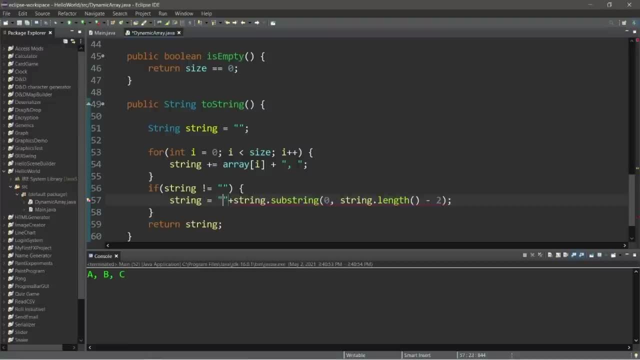 use some string concatenation, So I'll add a left square bracket And then at the end, add a right square bracket, And then these should be within square brackets now, And that looks a lot better. Now, what if our string is empty? Let's return just a set of square brackets using an else. 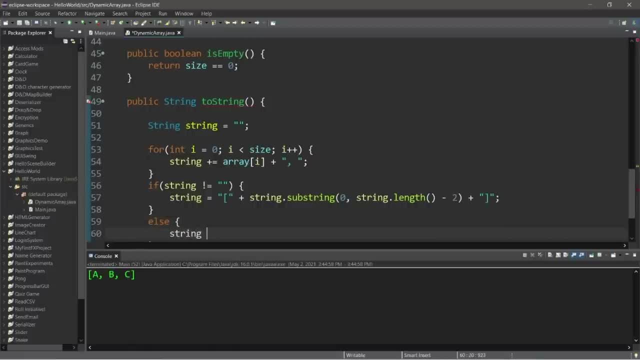 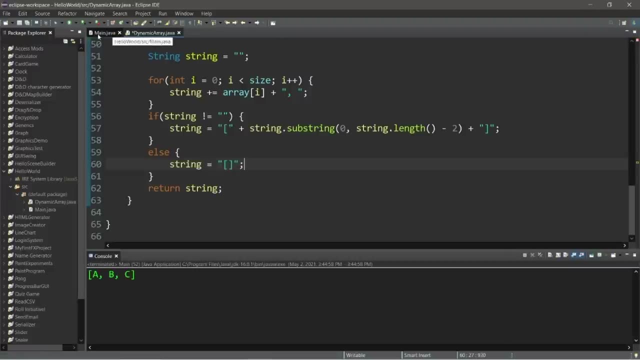 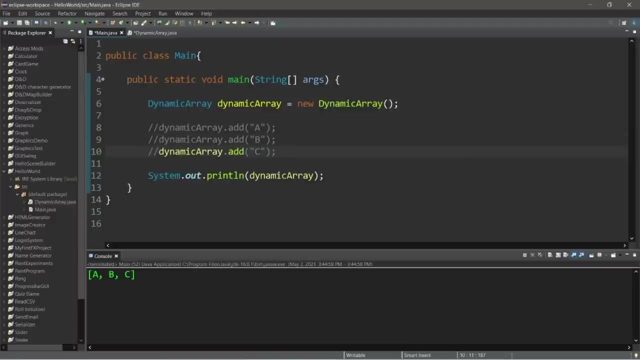 statement Else we will set our string equal to a set of square brackets, And that's it. So let's head back to our main Java file and comment these lines of code out, where we add elements to our dynamic array. So let's run this and we should have an empty set of square brackets. 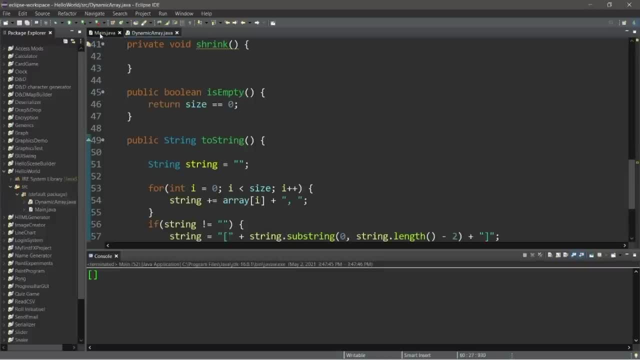 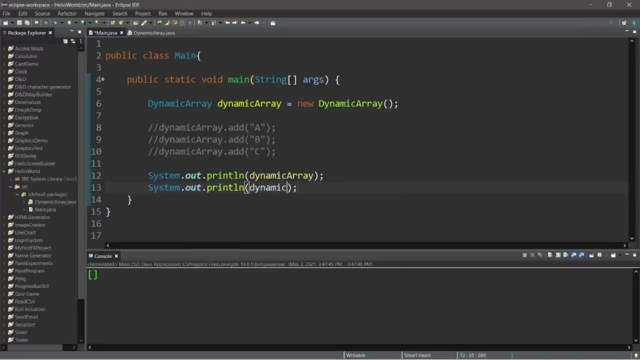 Actually, this would be a good opportunity to test our isEmpty method. So let's check that. So within a println statement systemelta println- I will take my dynamic array and use the isEmpty method. Then I'm just going to use some string concatenation. 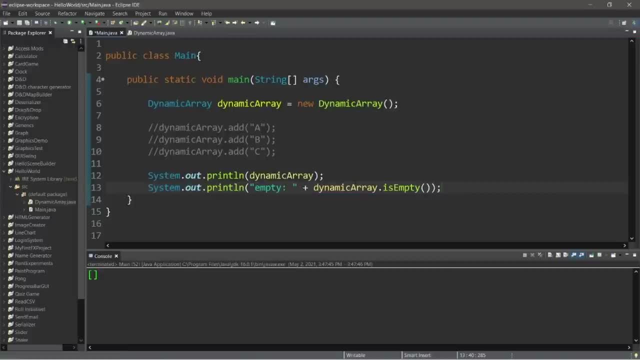 Empty colon space plus dynamic array isEmpty method And our dynamic array is currently empty. That is true, Then let's fill this with elements a, b and c, So this should iterate and display the elements of our array and let us know if our array is empty. 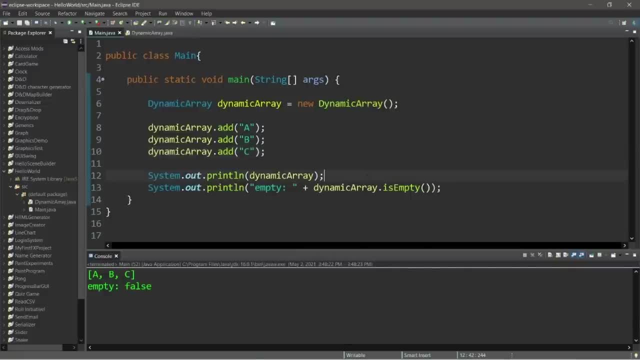 which is false. Since we're here, let's display the size and the capacity of our array too. So systemelta, println, dynamic array, dot size, And I'll use some string concatenation here too. So size, colon, space plus dynamic array dot size And the capacity as well. So capacity. 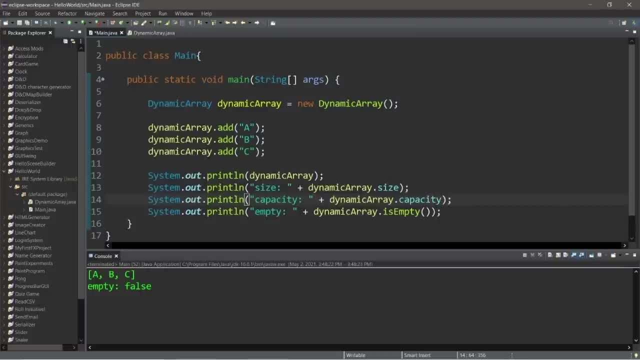 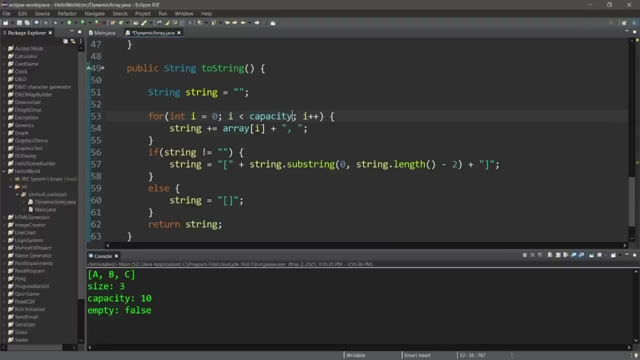 plus dynamic array, dot capacity. So this dynamic array has a size of three, three elements are filled in and a capacity of 10.. For fun, just to see the entire array, let's go to the toString method and change size to capacity, so we can see all of the elements. 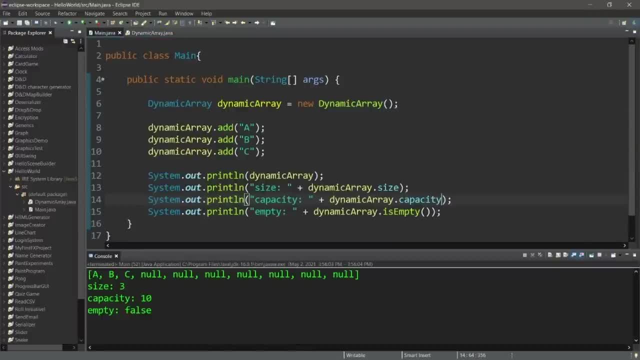 that are filled in and not filled in. So after running this, we can see our entire array at its full capacity. So we have a size of three. three elements are filled in, but we have a total capacity of 10. The rest of the elements are null. So if we were to count all, 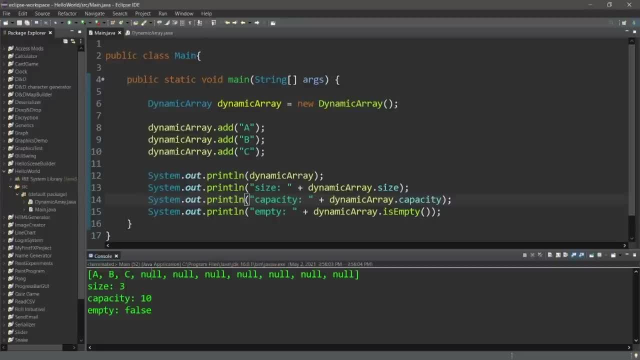 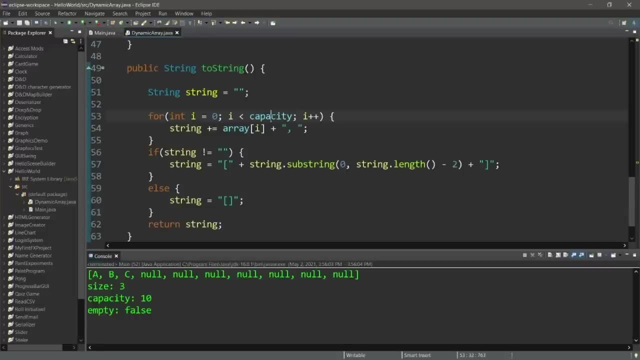 of these, they should be 10.. So we have 1,, 2,, 3,, 4,, 5,, 6,, 7,, 8,, 9,, 10.. Nice, So you can change that back to size or you can keep it as capacity. I'll just keep it as capacity for teaching purposes. 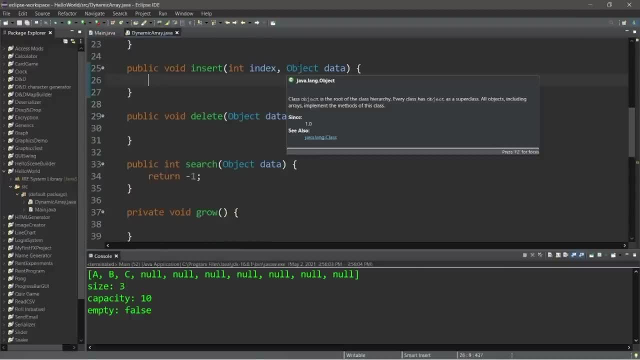 Now let's fill in the insert method. There's not a whole lot left to do. First, let's check to see if our size is greater than or equal to our capacity. If so, then we'll need to grow our array. If that is the case, call the grow method. What we're going to do at this point is shift all of 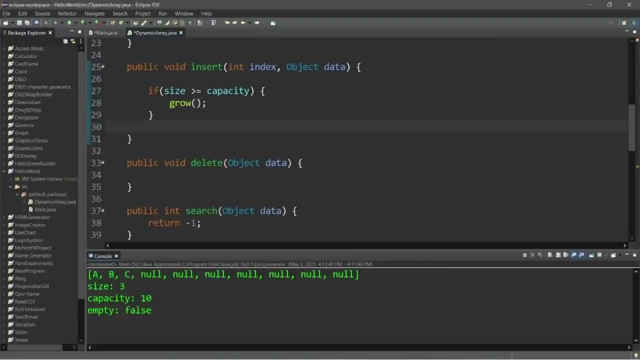 the elements that are filled in to the right in order to make room for the insertion. So let's use a for loop and iterate over our filled elements in reverse order. I will set int i our index, equal to our size, And then I will continue this as long as i is less than our index. 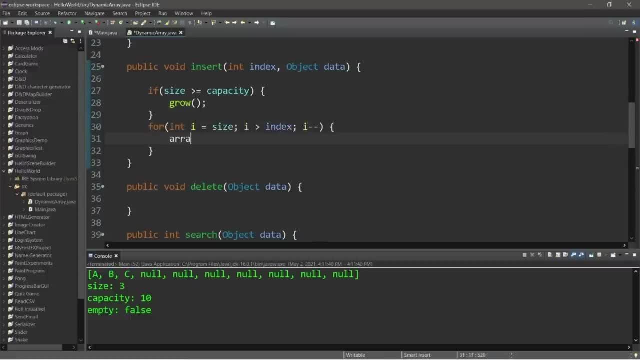 Then decrement i by 1.. So I'm going to take our array at i and set this equal to array at index of i minus 1.. This will shift all of the elements over to the right to make room for the insertion. So we will take our array at index equals whatever data we want to set. 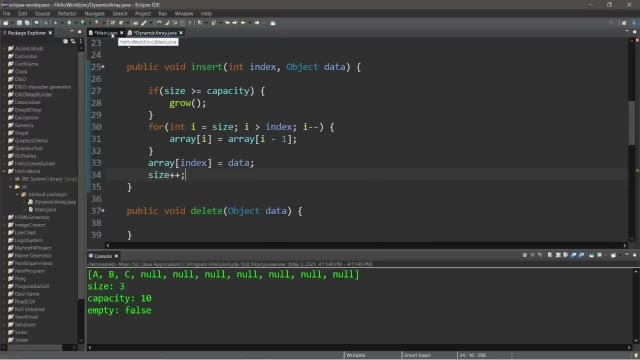 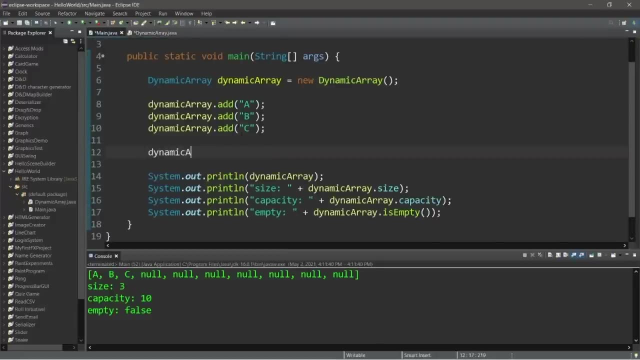 Then increase our size by 1.. So then, if we head back to our main java file, we can insert a value at a given index. So let's take our dynamic array dot, use the insert method, Let's say at index 0,. 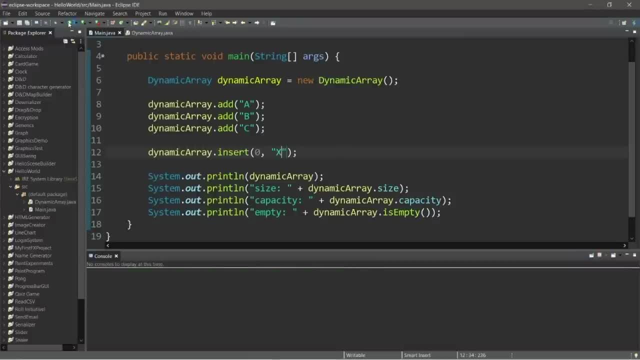 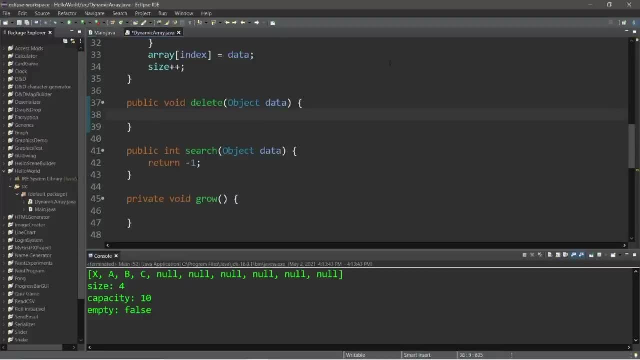 I would like to insert an x, So let's try it. Cool, we have x a, b, c, The size is now 4 and the capacity is still 10.. Now let's work on the delete method Within. here we're going to iterate. 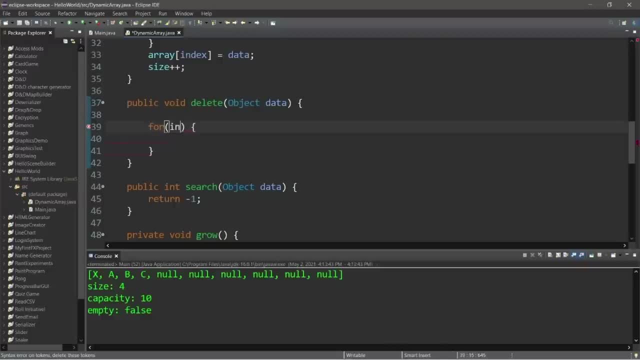 over the elements of our array beginning from left to right. So this is fairly easy. Int i equals 0.. We will continue this as long as i is less than our size And increment i by 1 after each iteration. So during each iteration we will check to see if. 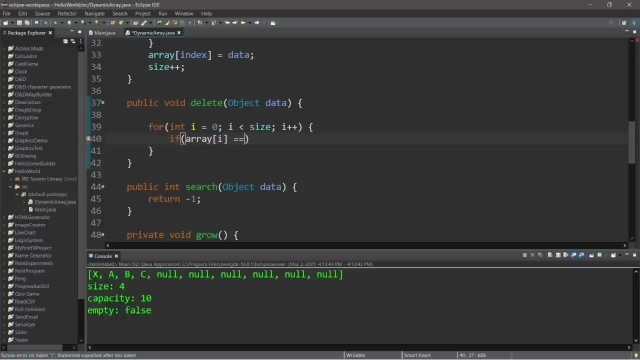 our array at index of i is equal to the data that we pass in as an argument. So if that is the case, we need to shift all of the elements to the left then. So we'll need a nested for loop for that. Then we will need an index of j, because i is already taken. We're within a nested for loop. 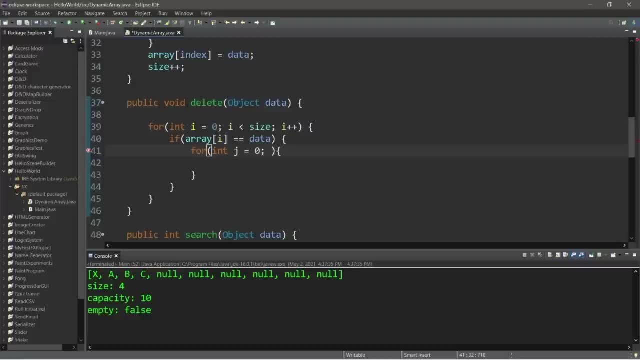 Int j equals 0.. And I will continue this nested for loop As long as j is less than our size minus i minus 1.. And then we are going to increment our index j by 1 during each iteration, So basically, wherever we make the deletion. 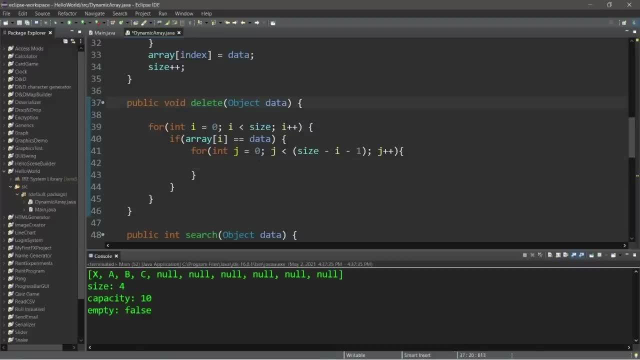 we're going to shift all of the elements afterwards one spot to the left. So we will take our array at index of i plus j and set this equal to our array at index of i plus j, The same as before but add plus 1.. So that will target the next element that comes afterwards, SAfe 15. 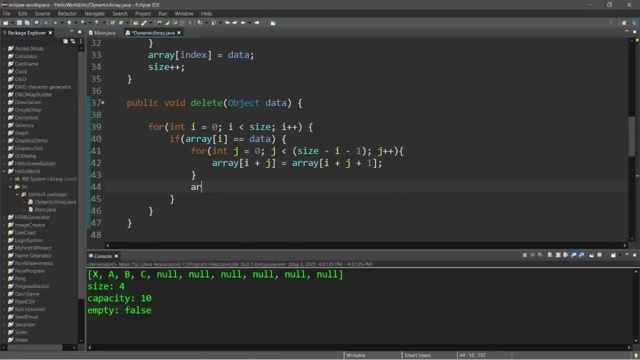 So, after we escape this for loop, we will take our array at index of s minus 1 and set this equal to null, And then we will decrement our size by 1. And actually here would be a good place to shrink our array. So let's write an if statement And check to see if our size 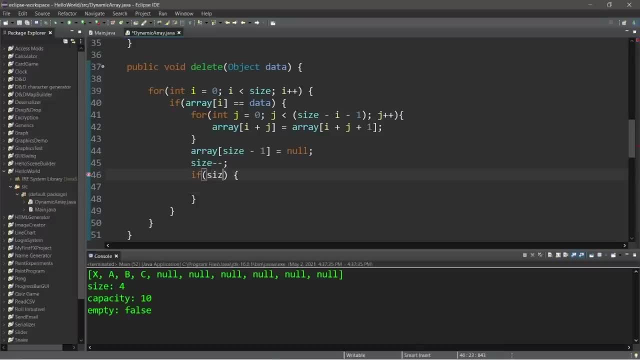 falls below a certain criteriaœ. So let's say that 5- our size- is less than or equal to a third of the capacity. so capacity divided by three. we don't want to shrink too often just because that's time consuming and then you may want to cast this as an 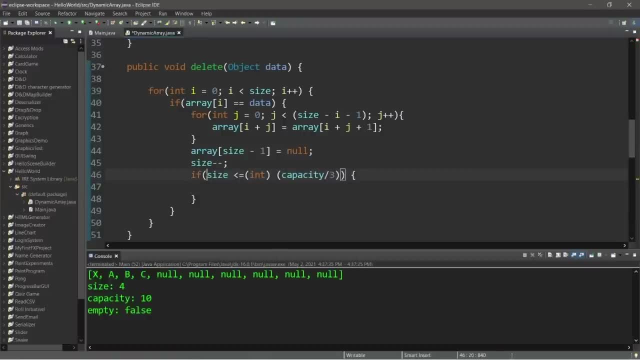 int, because it may not divide evenly. so if our size is underneath a third of the capacity, let's call the shrink method, and we will shrink our array by maybe half, but we'll get to that later. so then we want to break, to escape this for loop. then okay, let's try this then. so, after making the 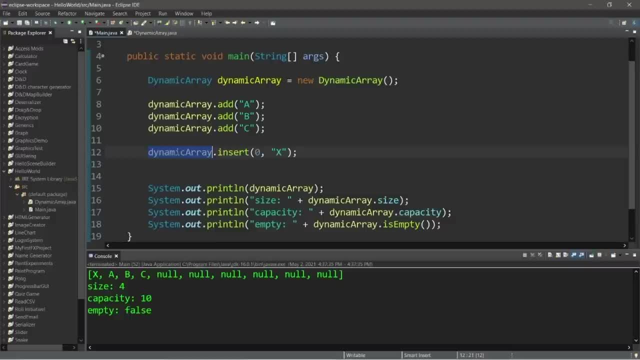 insertion. let's delete. what about a? so dynamic array dot delete and i do not need to pass in an index, just the data that i'm looking for. all right, so a is no longer in here. we have x, b and c, the size is 3 and the capacity is still 10.. all right, i promise we're almost finished. let's fill in the. 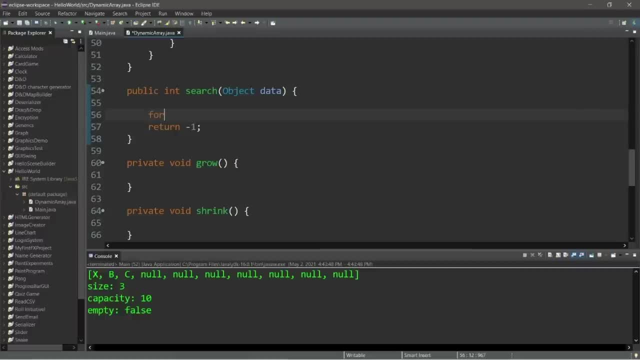 search method next, and this one is fairly short, so we just need to iterate over the elements of our array, beginning at index 0. for int i equals 0. i will continue this. as long as i is less than the size of our array, increment i by 1.. if our array at index of i is equal to the data that we're looking for, the data 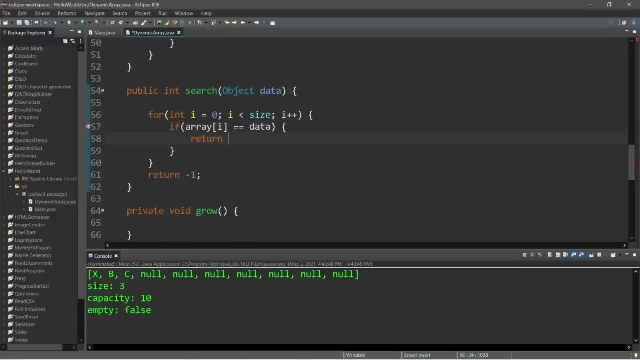 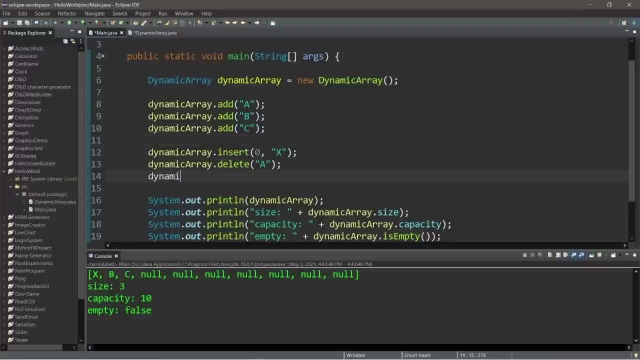 that we pass in as an argument, then we will return whatever i is our index. if we do not find it, we're return negative one. that's kind of like a sentinel value that means we did not find the value that we're looking for. okay, so let's search for maybe c dynamic array, dot search and i will pass in the 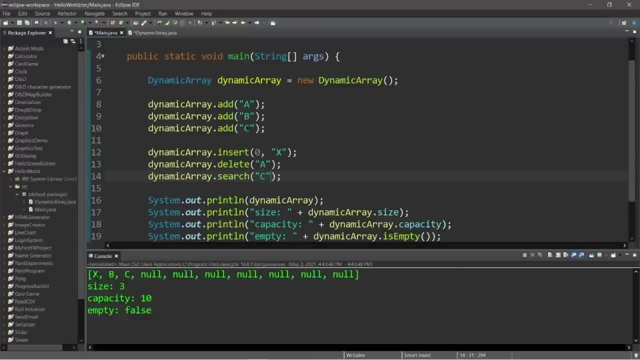 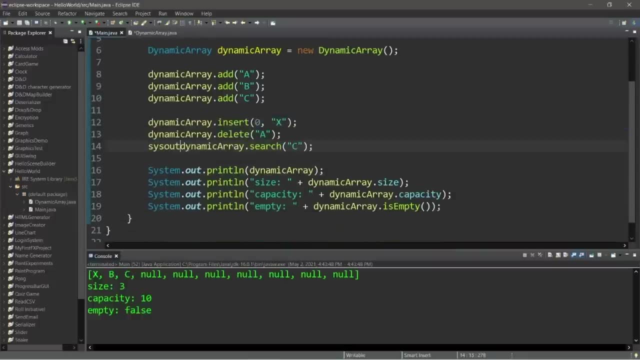 data that i'm looking for. i am looking for c, so that should be 0, 1, 2, assuming we insert and delete some values later- and then i'm going to place this within a print line statement. so dynamic array dot, and I am searching for C, And our result is that C is at index 2, 0, 1, 2.. All right, we're near. 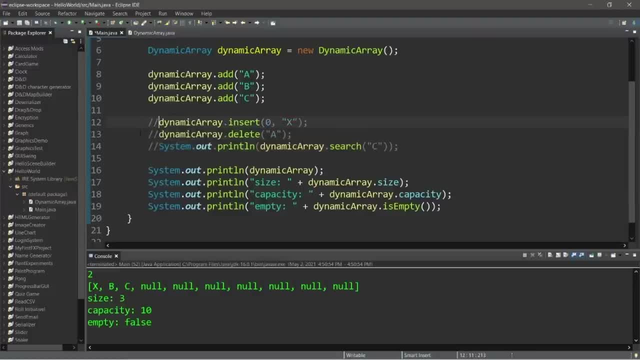 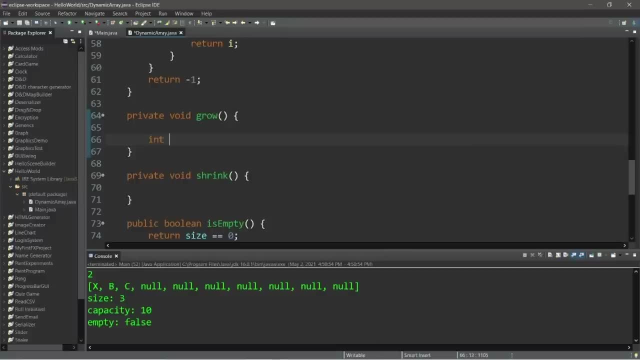 the end. Let's grow and shrink our array, and I'll turn these lines into comments. Now for the grow method. we're going to instantiate a new array, but we'll increase the capacity first. int. new capacity equals our old capacity, which is just named capacity, And let's say we want to increase. 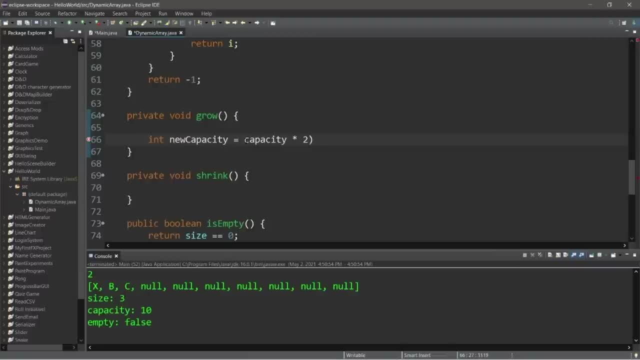 the capacity by two and then I will just cast this as an int. Okay, so after we create a new capacity, we will instantiate a new array. Then we need to copy the elements over, So we'll have an array of objects named. new array equals new array of objects with a capacity, of our new capacity. 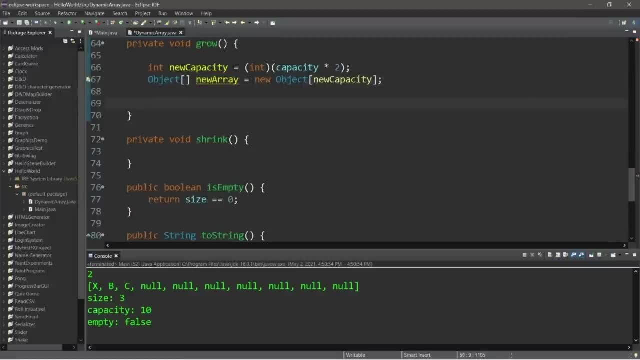 And then we need to copy the elements over to our new array and that's kind of time consuming but necessary. So we begin at index 0, for int i equals 0.. We will continue this as long as i is less than our size, And I will increment this by one after each iteration. So we will take our new array. 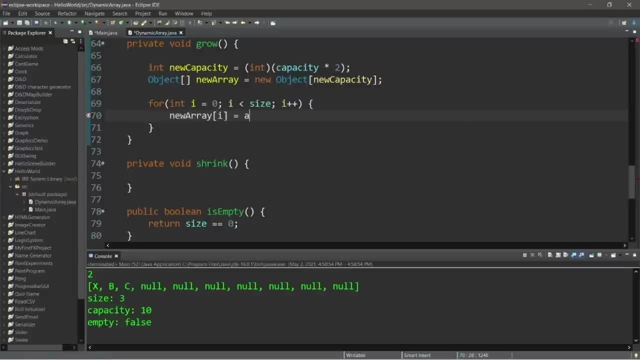 at index of i and set this to our old array, just named array, at index of i, And then we will change the capacity to whatever new capacity. Then, lastly, we will set our array to equal our new array. Then let's test it. So I'm going to 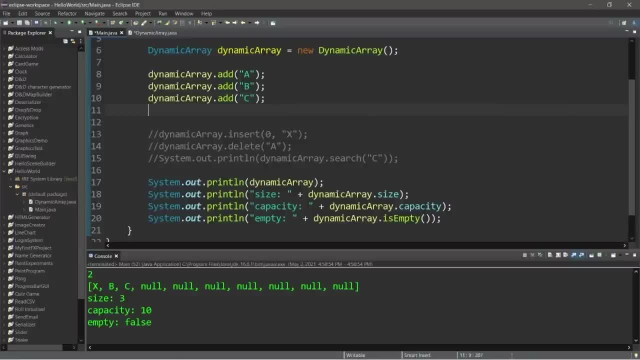 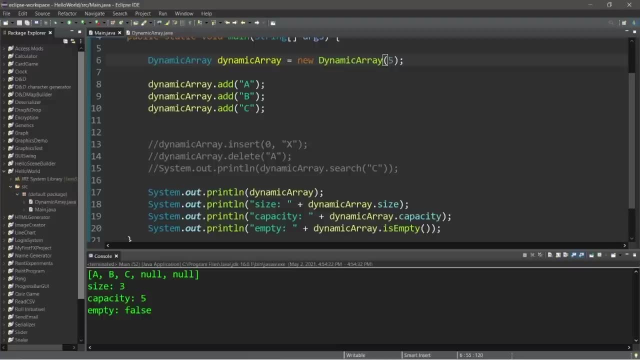 maybe add a bunch of elements. I'll keep that as a comment. So let's change the capacity of our array to 5.. I'll pass in 5 into the constructor so we have less elements to work with. So the size is. 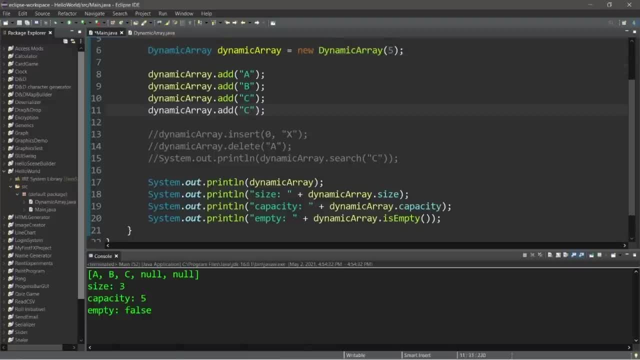 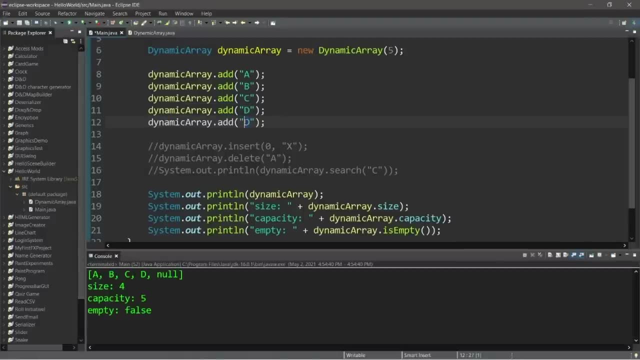 3 and the capacity is 5.. I'm going to add another element. Let's try d. So size 4,, capacity 5.. Let's add e. Okay, so currently our array is full. Now let's try to increase the size past the. 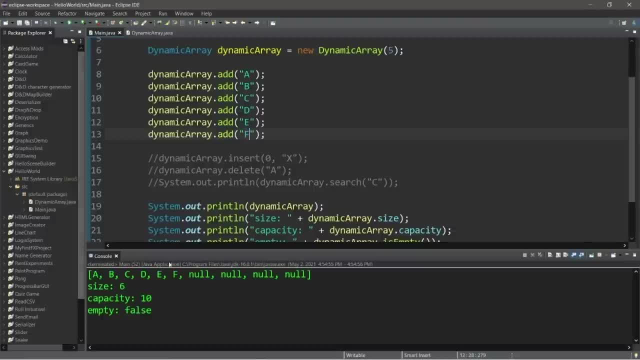 capacity. So I will add f and this should increase and grow the size of our array. So we have a capacity of 10 now and we have a bunch of empty elements And lastly, we just need to shrink this array. And this next part is super simple. for the shrink method, Copy everything from the grow. 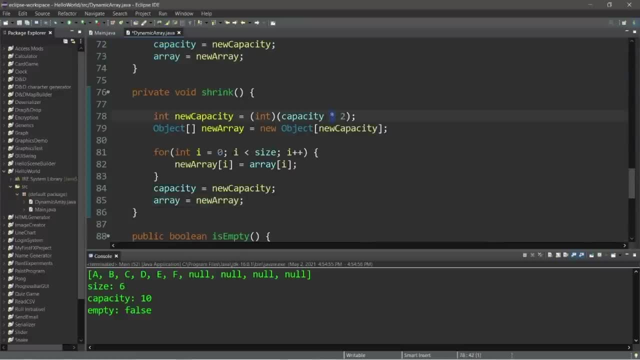 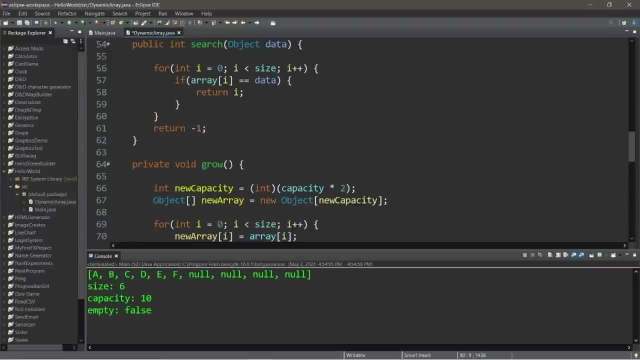 method and paste it within the shrink method. So let's add a new component, Let's add a new component method, but change capacity times two to capacity divided by two. now we will call the shrink method automatically when the size falls below a third of the capacity. that means we have a lot of wasted. 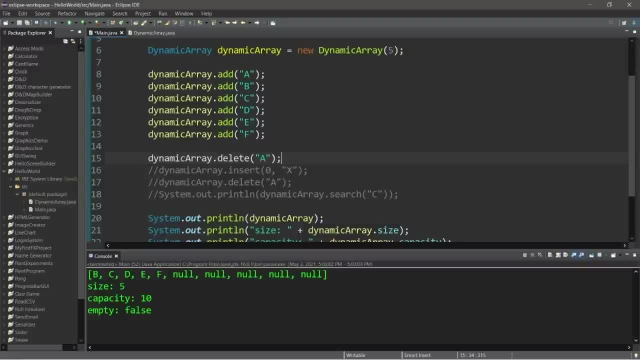 memory. now let's begin deleting elements. so i will type dynamic array dot, delete a, then maybe b, so when the size is a third of the capacity, that's when it should shrink. so we're not there yet. let's delete maybe one or two more times. so let's delete c, and there we go. so the size is three and the 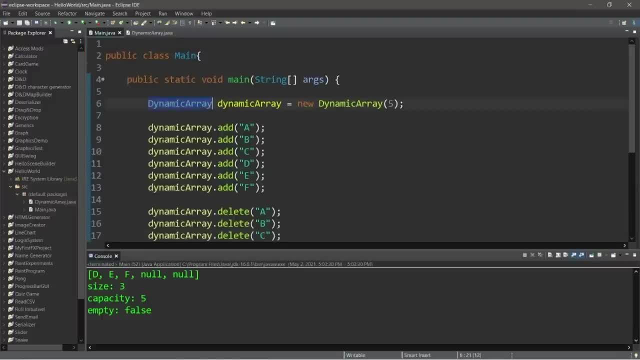 capacity is now five. well, all right, that's a very basic dynamic array. if you're using java, instead of just building your own dynamic array, you might as well just use an array list, because it's more efficient and well, it's already coded for you, but i think this was good practice for us, just to. 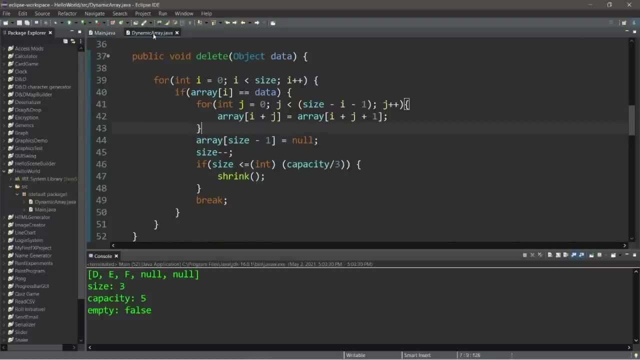 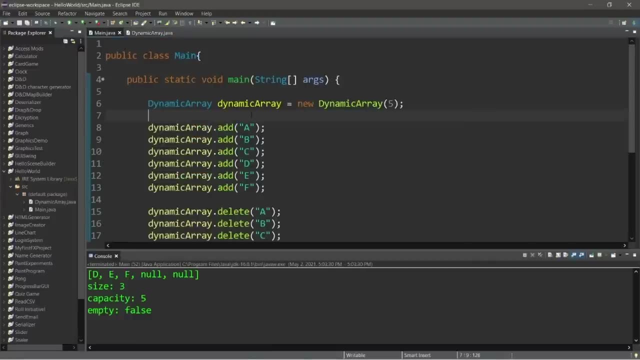 understand how dynamic arrays work. so if you would like a copy of all this code, of course i will post this to the comment section below and i'll see you in the next video. if you made it all the way to the end, please give this video a thumbs up. a random comment down below. 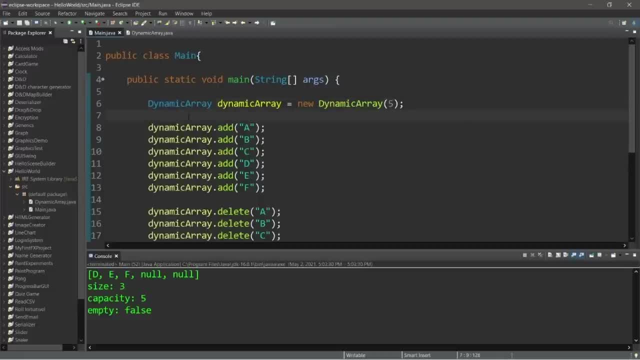 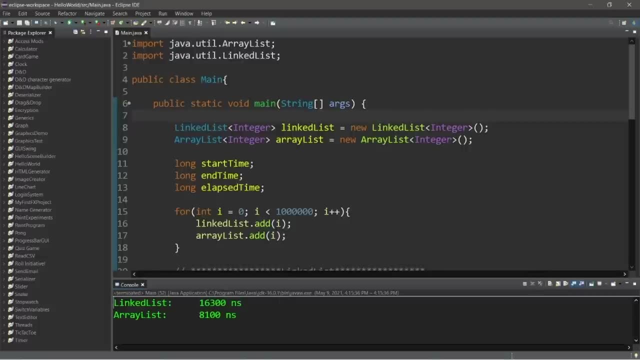 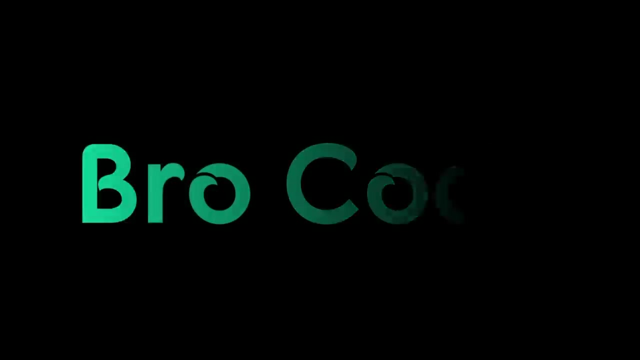 and well, yeah, those are dynamic arrays. and well, computer science. hey, what's going on? everybody, it's your bro, hope you're doing well. and in this video we're going to run some tests on both array lists and linked lists in java. so sit back, relax and enjoy the show. all right, let's begin, we'll. 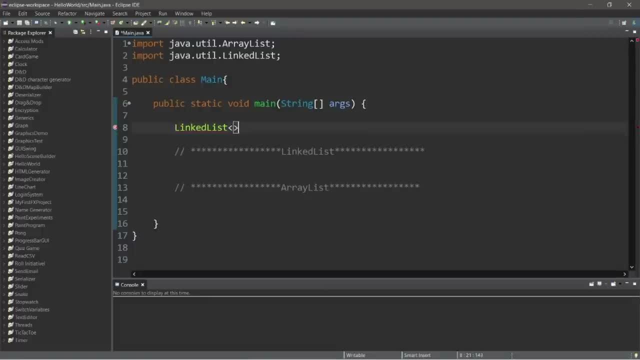 need both a linked list and an array list. so linked list- the data type will be integers and we'll name this. linked list equals new linked list. again, the data type is integer. add a constructor. boom, we got ourselves a linked list and now we'll need an array list. change linked to array. 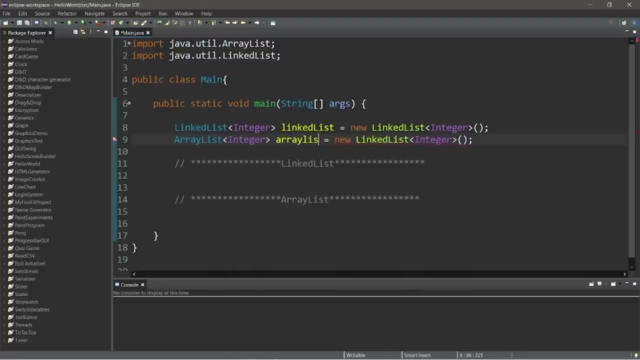 this will be named array list. make sure to pay attention. the capitalization equals new array list and we'll need to keep track of the time. we'll need a start time, end time and elapse time and these will be of the long data type. we'll be working on that in a little bit, but i'll see you in the next video. 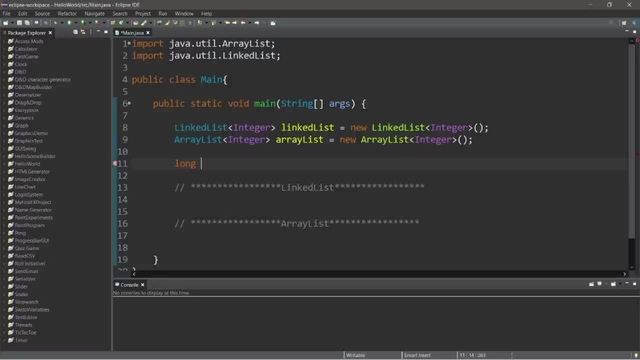 working with nanoseconds. so a long is preferable to an int. a long is really just a really long integer. think of it that way. so we have start time, end time and elapse time. okay, and now we'll need to populate both our linked list and our array list, and we can do. 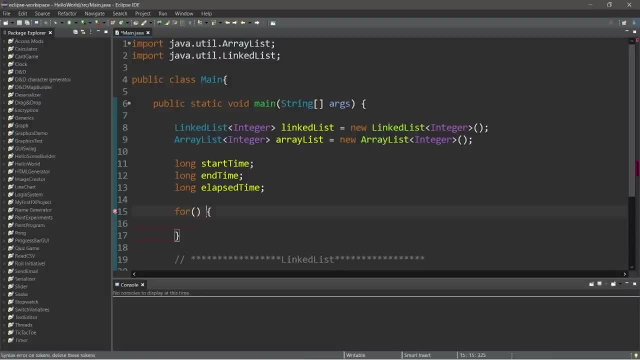 that with a for loop we'll need a large sample size, maybe one million elements. that'll be good. so int i equals zero. we'll continue this as long as i is less than a million, and i believe that's about a million. yeah, we're good. okay then. 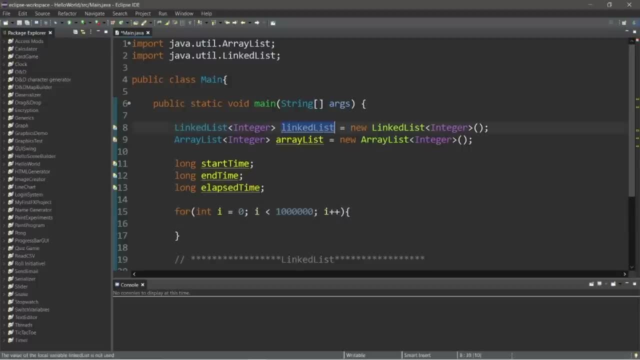 increment i by one during each iteration. so i'm going to add i to both my linked list and my array list. so we can add primitives, because java has an auto boxing feature. so even though these are integer objects, we can still add primitives, and be sure to add to our array list as well. 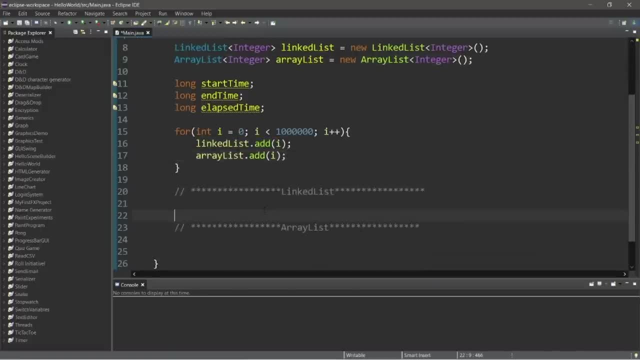 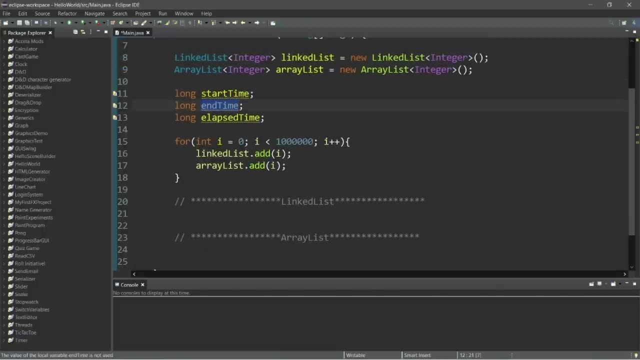 so array list, dot. add i. okay, let's move on now. we'll keep track of the time. we'll need to assign the start time of value and end time of value before and after our operation. so let's say that start time equals and we can get the current time of our jvm by using system dot nano time method. 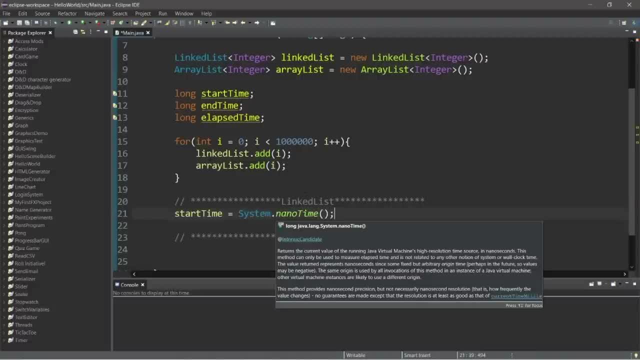 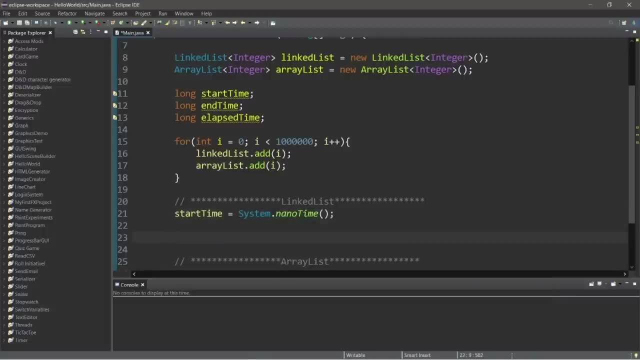 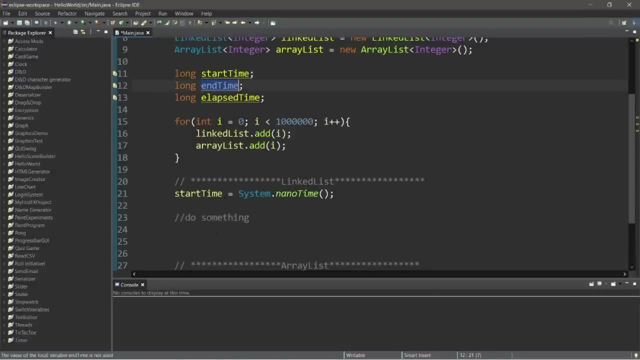 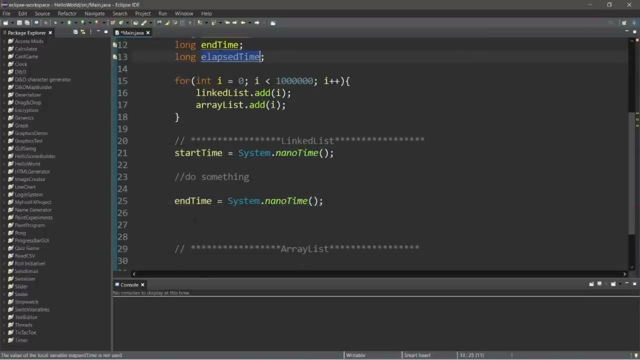 and let's take a look. so this returns the current value of the running java virtual machines time source in nanoseconds. so we will get the start time after we do something. i'll just add a note here: do something, then we will get the end time. so end time equals system dot nano time method and to calculate the elapsed time, 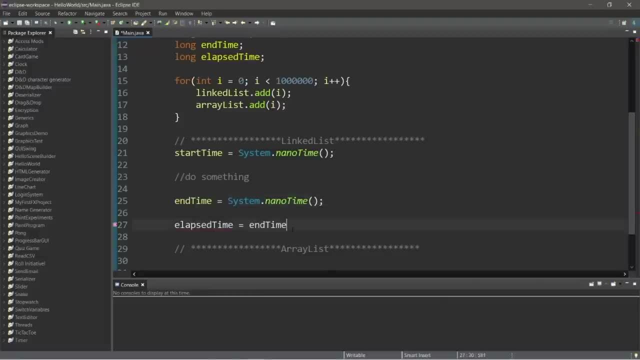 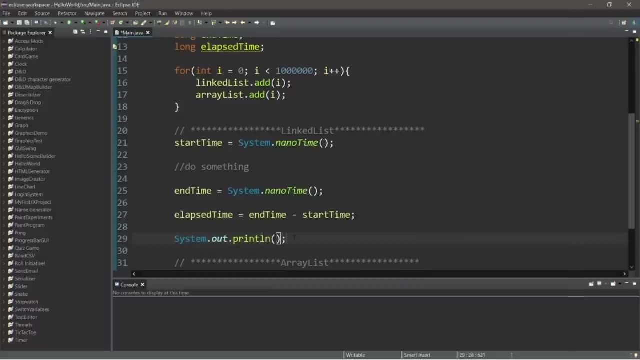 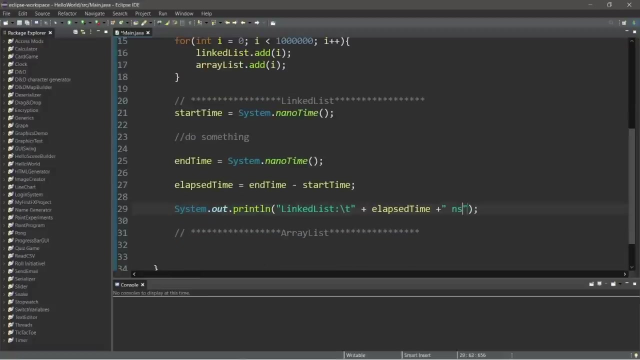 that will be. elapsed time equals end time minus start time, and then we'll probably want to display this. so let's do that systemoutprintln and let's say linked list. i'll add a tab to plus elapsed time plus ns for nanoseconds, and let's just run this to test it. so this portion of code really took. 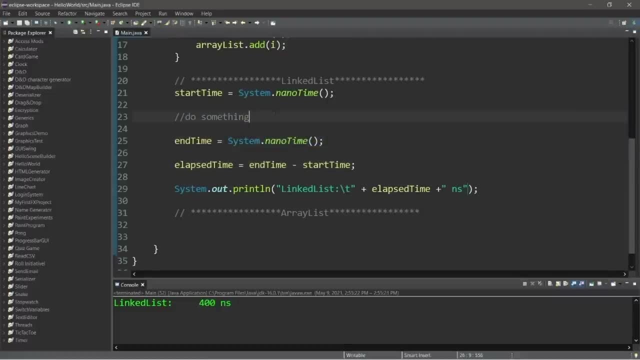 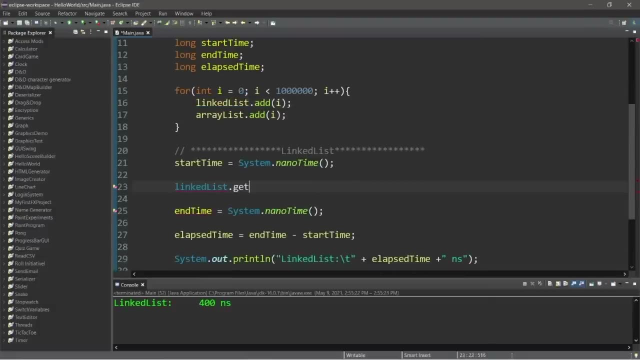 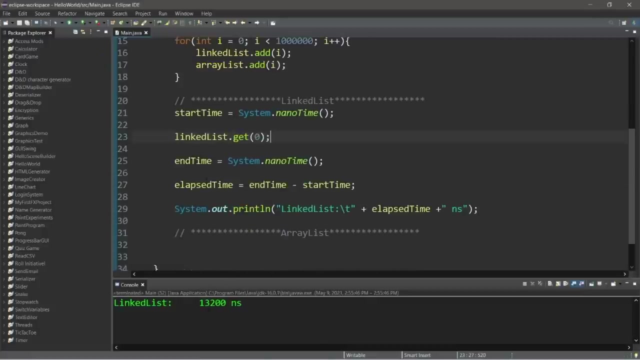 right between here, took 400 nanoseconds. okay, let's actually do something now. so let's get the first element within our linked list: linked list dot. get zero and let's see how long this takes. okay, 13,200 nanoseconds. now with an array list, let's copy everything that we have for our 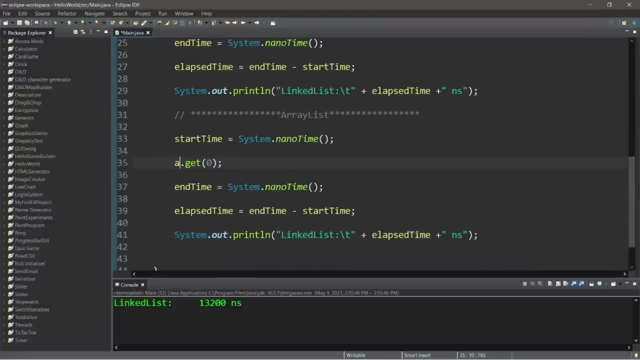 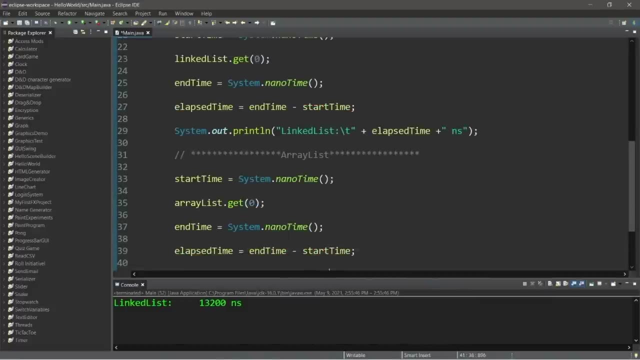 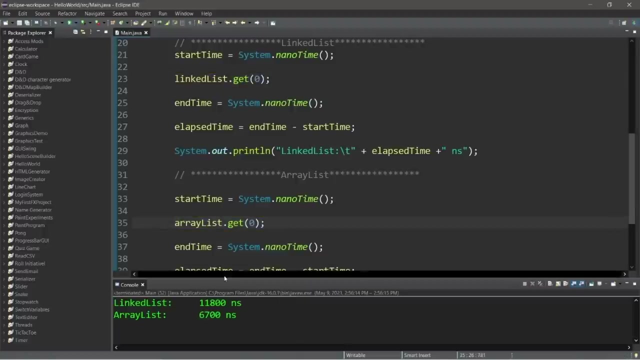 linked list and change linked list to array list and be sure to do that here as well- array list and let's compare these. so we are getting the index of zero for both our linked list and array list and we will compare them and it appears that our array list is slightly faster. our linked list took. 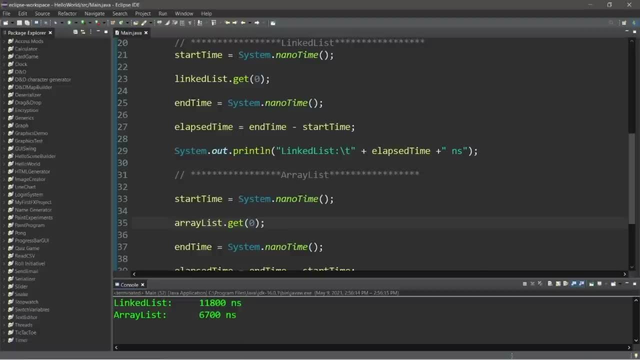 11,800 nanoseconds and our array list took 6,700. so it looks like getting the first element of our linked list is going to be the first element of our linked list and we're going to compare them to our linked list is going to be a little bit slower than our array list. this time let's get something. 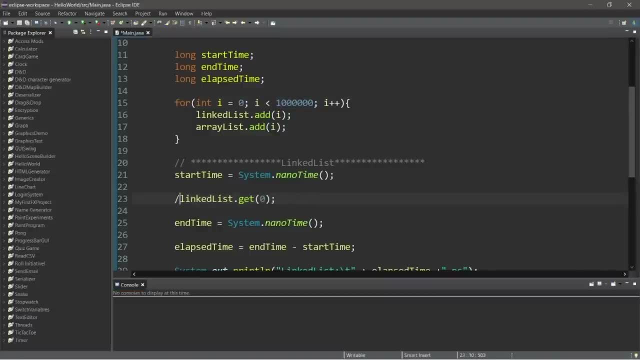 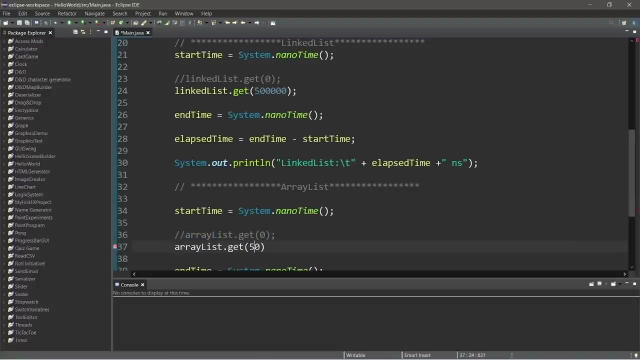 right in the middle of our linked list and array list. so i'm going to turn this line into a comment and we will get the index of 500,000- so that's right in the middle- and do the same thing with array list as well. so arraylist dot, get 500,000 and let's see how long this takes. okay, so our 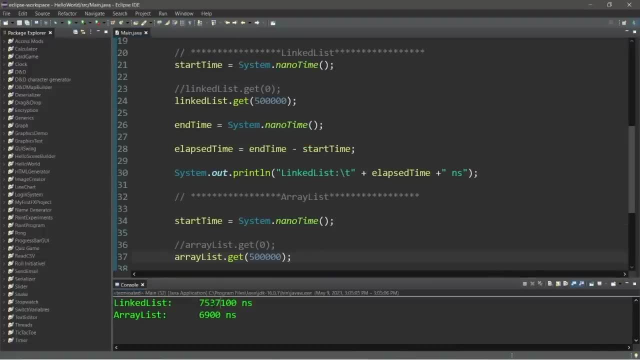 linked list took way longer than our linked list- and we're going to get the index of 500,000- than our array list. our linked list took 7.5 million nanoseconds compared to our array lists 6,900 nanoseconds. okay, so that's still way longer with a linked list. 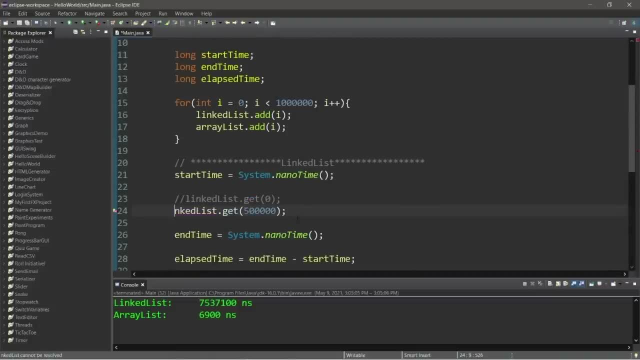 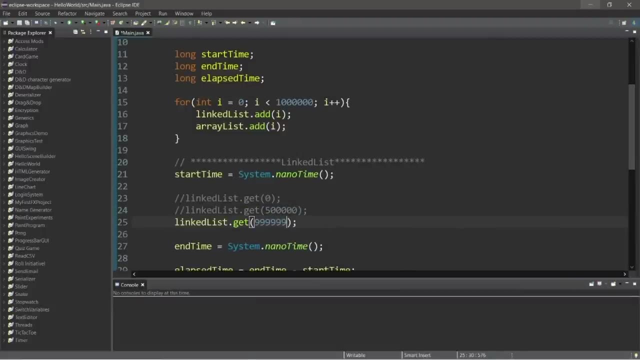 now let's try something near the end of our linked list and array list. what about the last element? linked list die get 999,999. so that is the last index in our linked list and array list. we have one million elements and this is exclusive and the first. 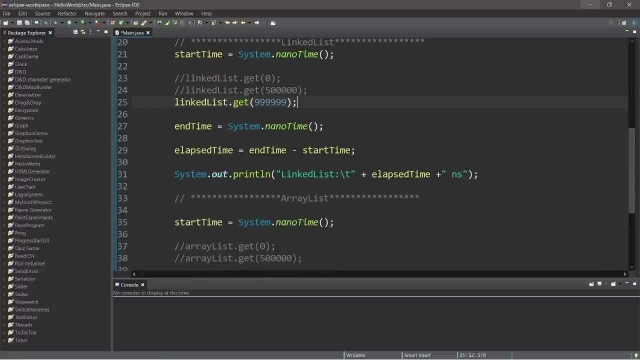 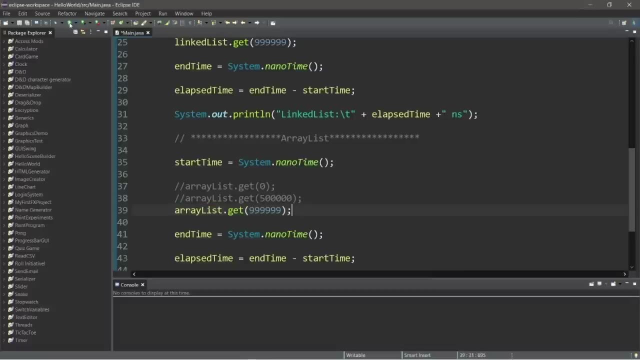 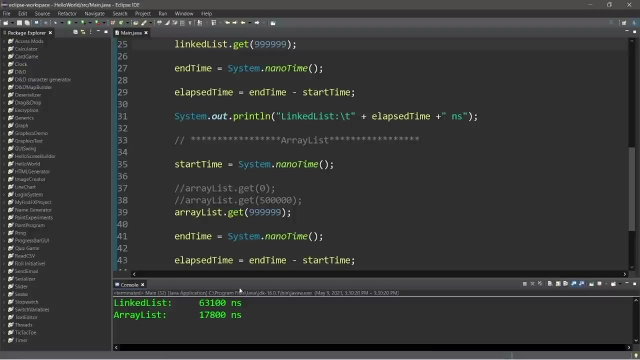 element has an index of zero. so let's do the same thing with array list. array list die, get 999,999. and here are the results: our linked list took 63,000 nanoseconds compared to our array lists 17,000. now the reason that our linked list took less time to retrieve: 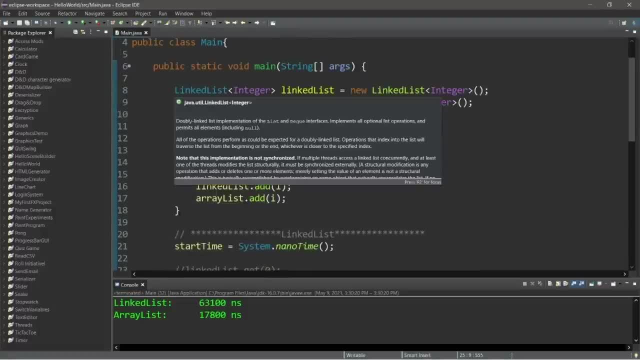 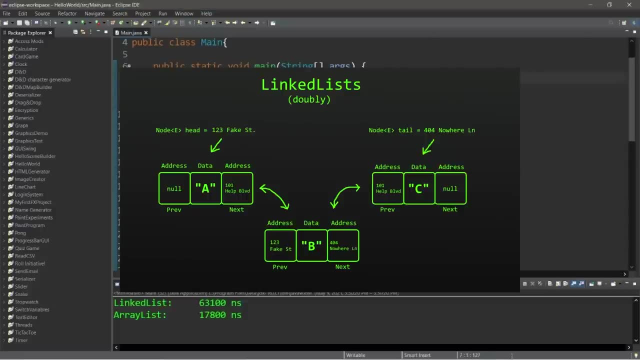 an index at the end is because this linked list is a doubly linked list, so we can begin at the head and work our way towards the tail, or begin at the tail and work our way backwards to the head. so, since this index is right at the end, 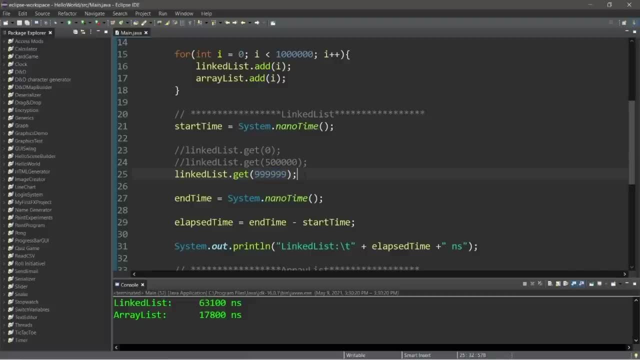 it's actually going to be very easy to retrieve this index, whereas in the middle is actually going to be the worst possible spot for a linked list, because we can start at either end, but it's still going to take the same amount of time to get to the middle. so it appears that 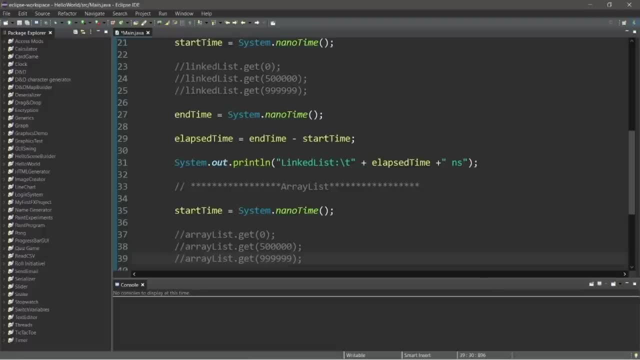 accessing an element from an array list is always faster than a linked list, and that's to be expected, because with an array list we have random axis of elements, unlike with a linked list. we have to begin at one end of our linked list and traverse our list in variousрутles, a certain to reduce the return by ก� Bigfoot. 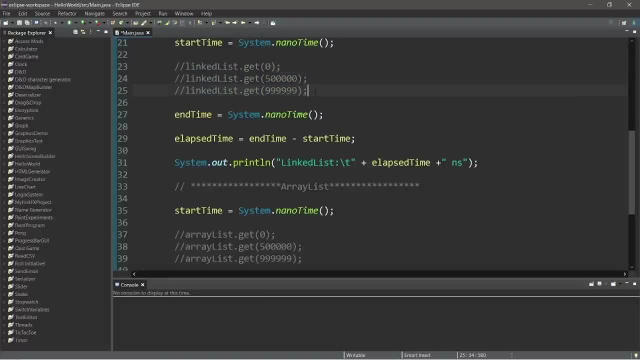 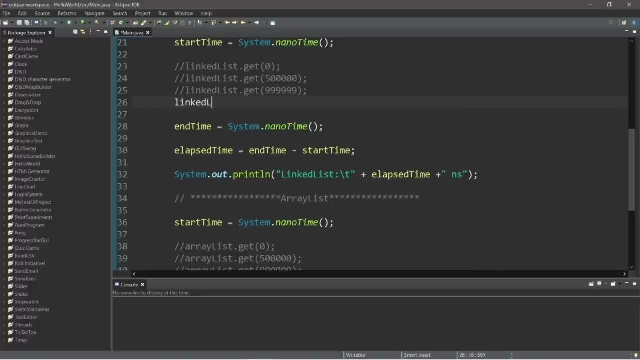 linked list until we get to the index that we're looking for. Now let's add or remove an element from our linked list and array list. Maybe just remove, because it's going to take really the same amount of time. So, linked list, dot remove And let's remove the first element. So index zero. 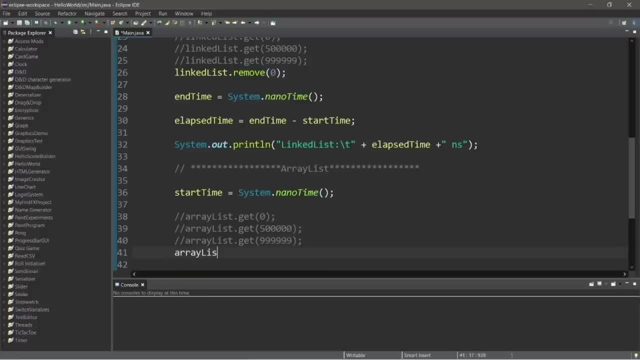 And do the same thing with array list. Array list dot. remove index zero And let's take a look again. Okay, so it appears that our linked list was actually faster this time- 17,000 nanoseconds compared to 2.2 million nanoseconds of an array list- And the reason that our array list took 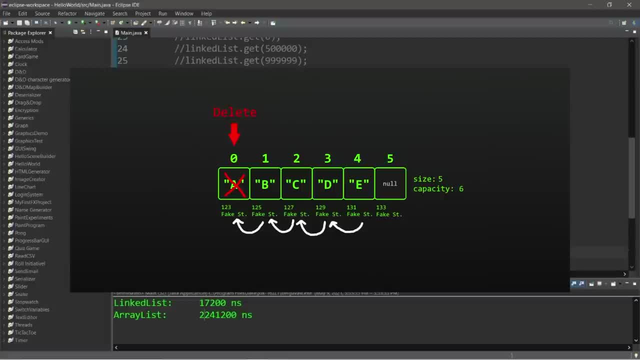 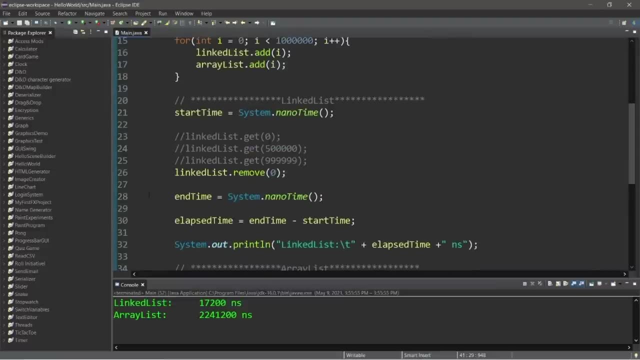 longer is because we need to shift all elements to the left after removing an element. So we had to shift 1 million elements after removing the first element. Now let's remove something near the middle. So let's remove index number 500,000.. So linked list dot remove And let's remove. 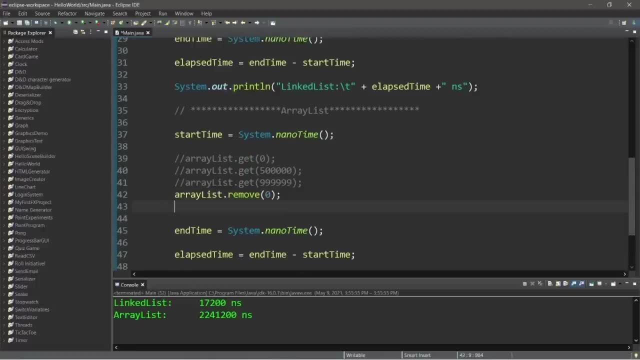 index number: 500,000.. So linked list- dot- remove 500,000.. And do the same thing with array list. Be sure to comment this line out: Array list- dot- remove 500,000.. And here are the results. So looks like our linked list took a lot longer this time, 7 million nanoseconds compared to. 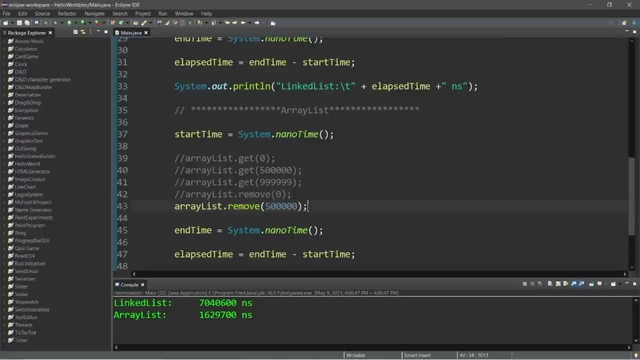 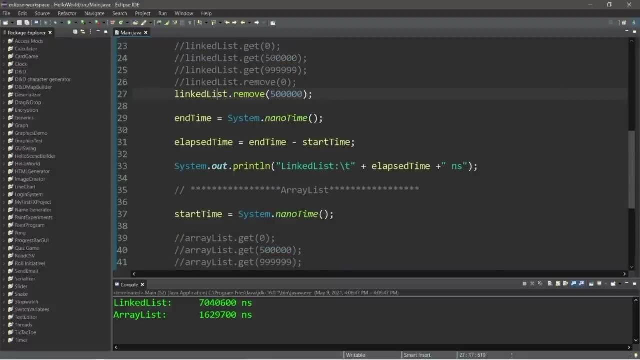 1.6 million nanoseconds for an array list. So with our array list there were less elements to shift this time because we were right in the middle. But with our linked list we still had to know that we had to shift the array list. So if we were to shift the array list we would have to 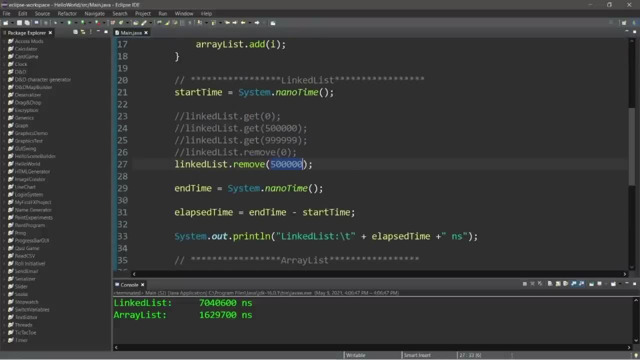 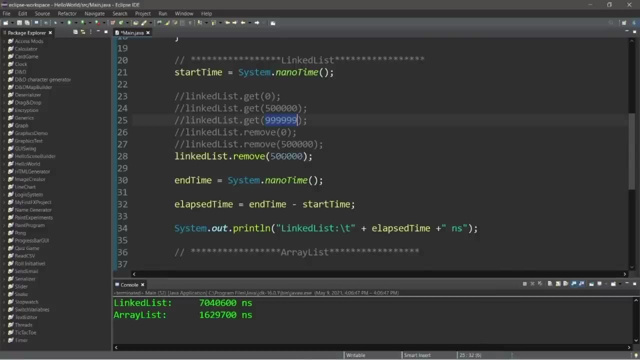 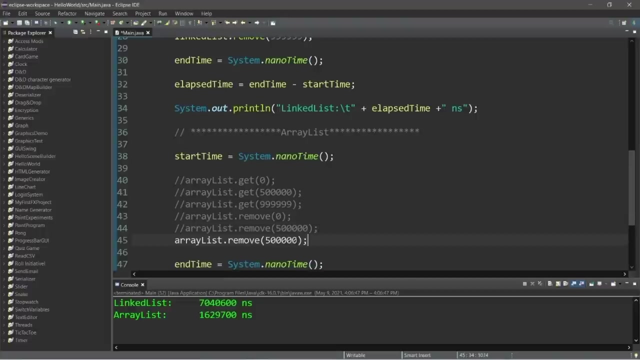 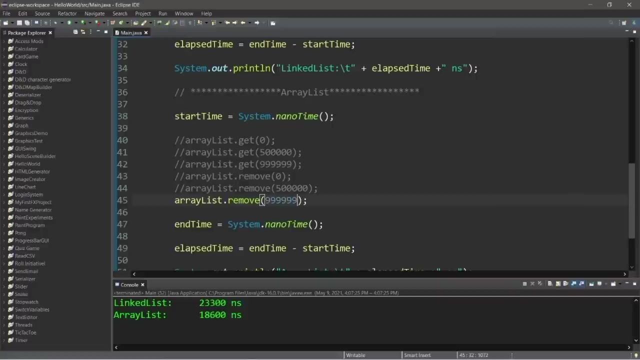 navigate to the middle to remove one of these elements. And then let's remove the element at the end of both our linked list and our array list. Linked list- dot- remove 999,999.. And do the same thing with array list. Array list- dot- remove 999,999.. And this time our linked list is just. 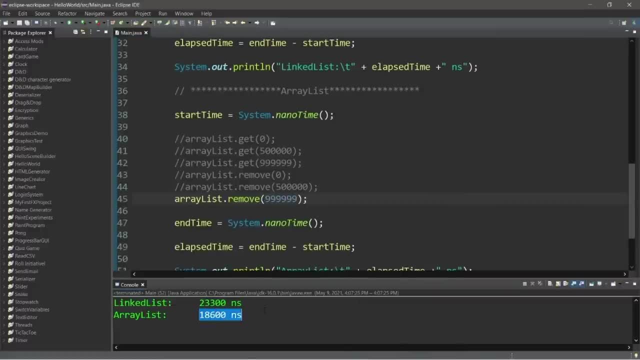 slightly slower than our array list. Adding or removing elements near the end of an array list is actually fairly easy. The closer that we insert or delete near the end, the less time it's going to take, because we have to shift less elements. And with a linked list, well, this is a doubly linked 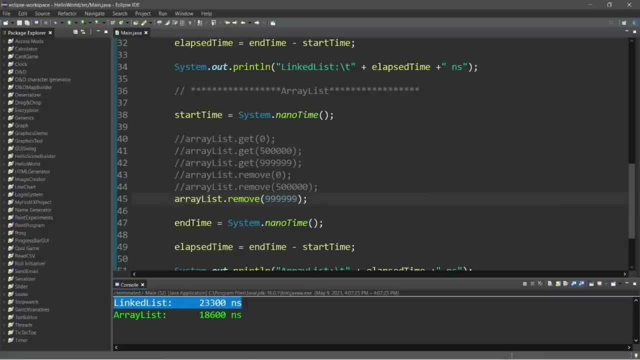 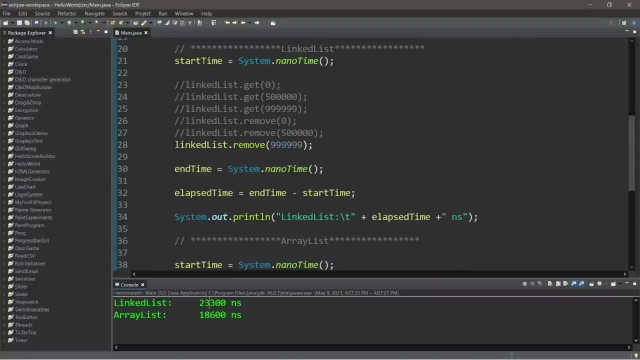 list. so accessing the last element doesn't really take too long. If it's near the middle, it's going to take forever actually. So it seems that in most situations, an array list is going to be better than a linked list. However, if you have to do a lot of inserting or deleting, 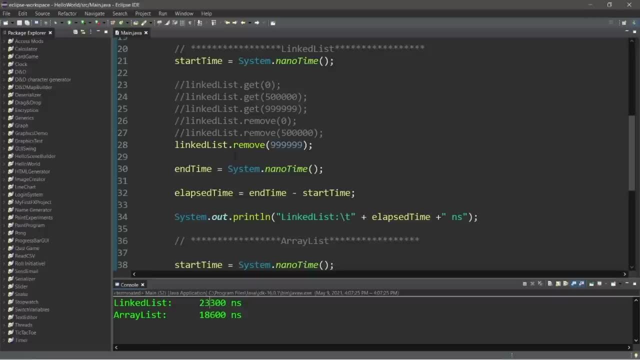 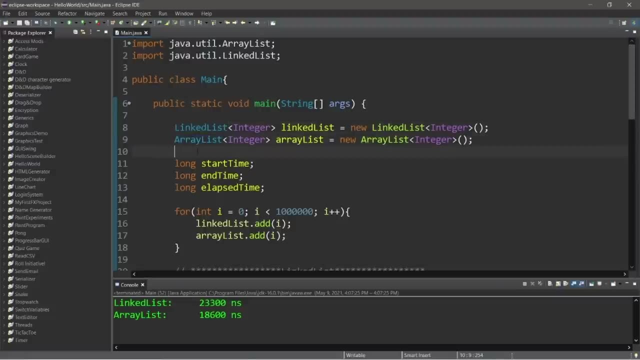 especially if it's a large data set, a linked list might be better, But it seems that in array list is going to be more flexible for most applications. So that is linked lists versus array lists. If you would like a copy of all this code, I will post this to the comments section down below. 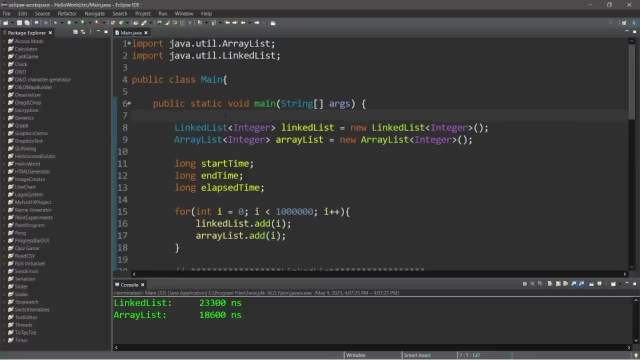 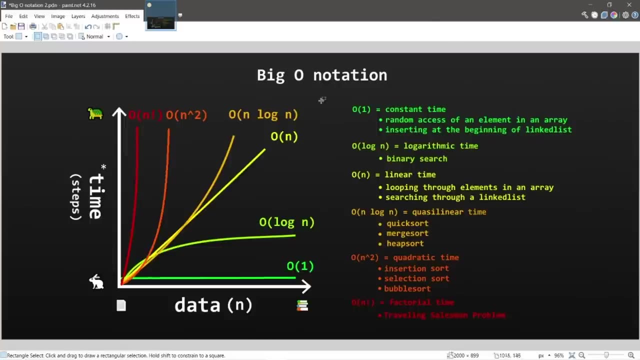 And well, yeah, that's linked lists versus array lists in computer science. Hey, what's going on? everybody, It's your bro, Hope you're doing well. And in this video I'm going to describe the very basics of big O notation in well, computer science. So sit back, relax and enjoy the show. 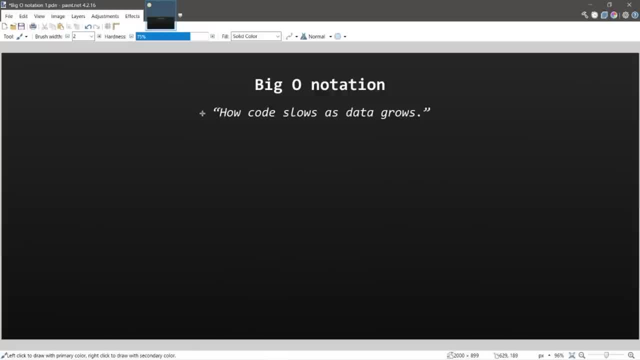 Oh yeah, big O notation. So a common phrase used with big O notation is how code slows as data grows. It describes the performance of an algorithm as the amount of data increases And really this notation is machine independent. What we're really focusing on is the number of steps to complete an 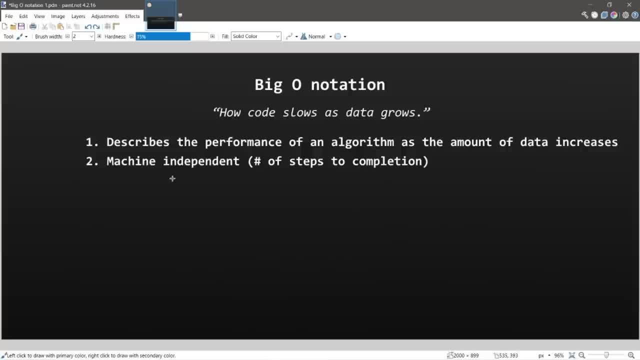 algorithm, because some machines are going to run certain algorithms faster than others. And three, we tend to ignore smaller operations. If we had some task that took n plus one, we would just reduce it to just n, because that plus one really isn't going to make a difference. 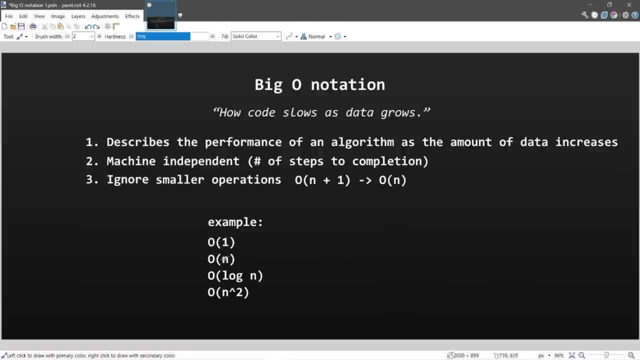 So here's a few examples of big O notation: We have o of one, o of n, o of log n and o of n squared. And n is really just the amount of data that we're passing in. It's a variable, like x, What we're. 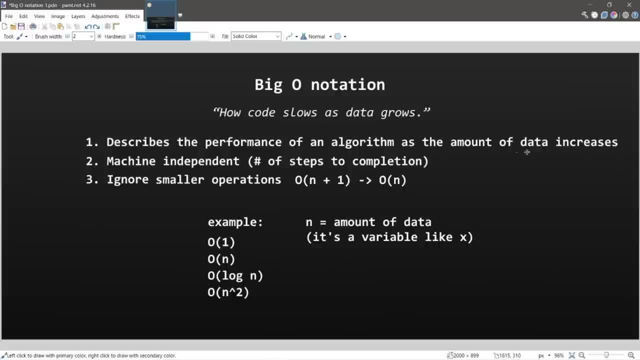 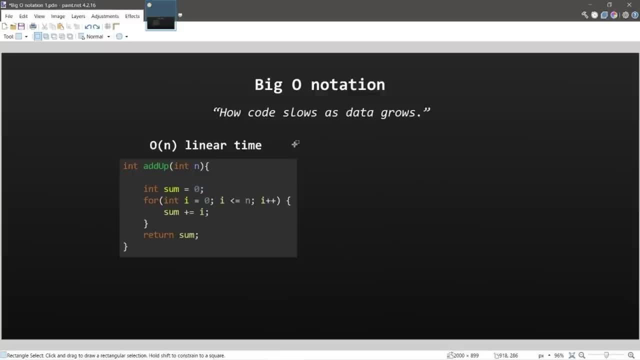 focusing on is the performance of an algorithm as the amount of dat increases, and n is a representation of the amount of data that we're passing in. Here's a more concrete example. I've a function named addUp. we will add up to a certain number, depending on what we 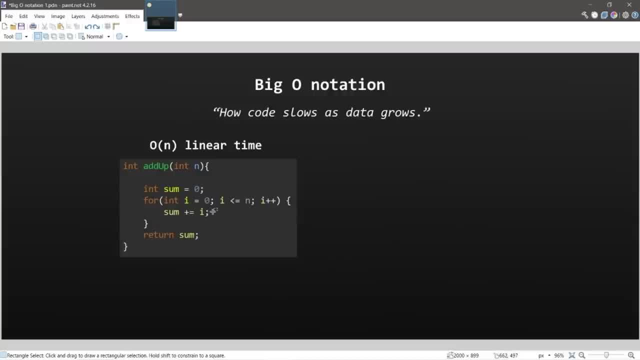 pass in as an argument. The for loop within here will iterate once up to whatever number that n is. add i to sum, then return it. What if n was a large number, like a million? Well, it's going to take just above a million steps to. 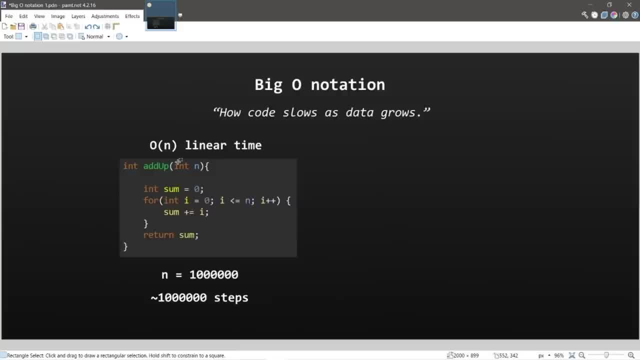 complete this function. This function is said to have a runtime complexity of O linear time. As the amount of data increases, it's going to increase the amount of steps, linearly or proportionally. Now another way in which we could write the same function is to take: sum equals n times n plus 1 divided. 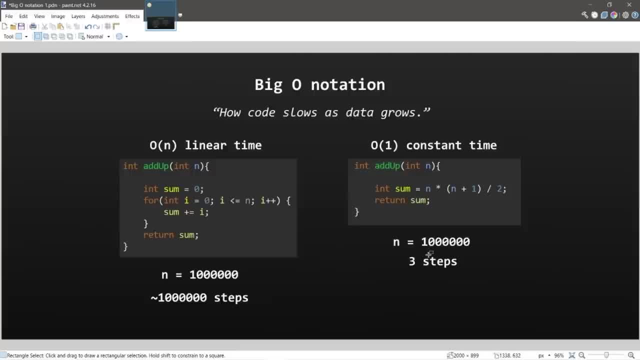 by 2. We will get the exact same sum. So if n was, let's say, a million, this is still only going to take a couple steps, Three steps, not a million steps. So this function is going to have a runtime complexity of O- The input size. 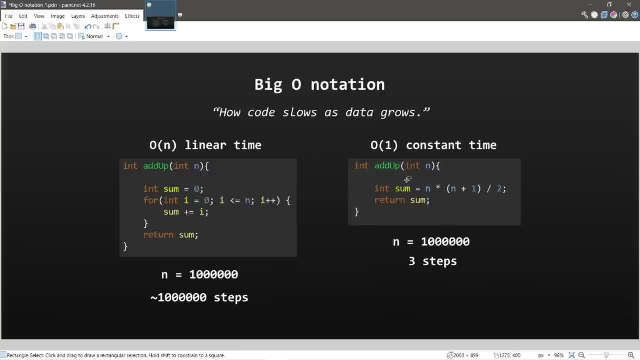 doesn't matter. The amount of data that we have really doesn't matter, It's going to be complete. So this function is way better than this previous one. Three steps is better than a million steps, And the reason that this isn't O because this takes three. 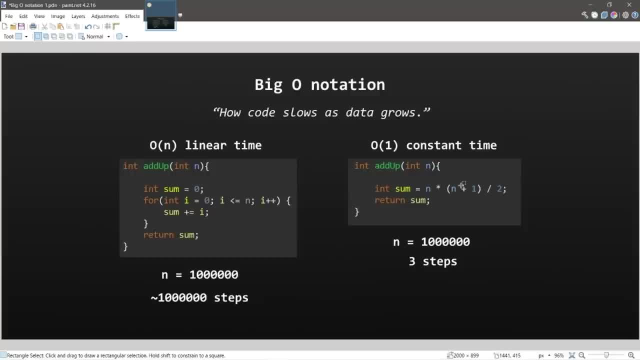 steps is that we really don't care about smaller operations. In the grand scheme of things, they really won't make much of a difference. So we would just shorten this and say that this is O constant time. The input size doesn't matter. Here's a graph that I made to represent the different runtime. 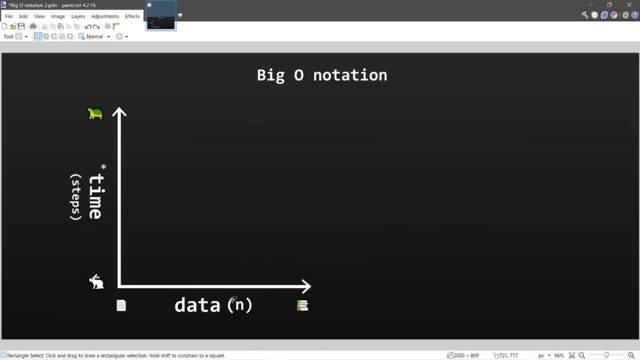 complexities. We have data on the x-axis represented by n, So data will increase as we go more to the right And we have time on the y-axis. I did add an asterisk next to time because some of these times can vary depending on. 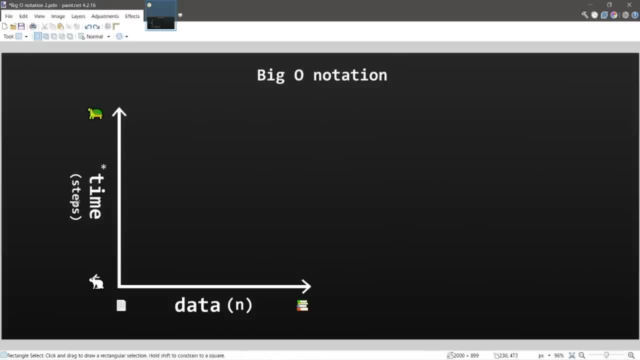 what machine you're using, So these can vary. Another way to look at this is number of steps. So as we increase on the y-axis, these algorithms are going to perform. with increasingly more time, They're going to get slower. So let's. 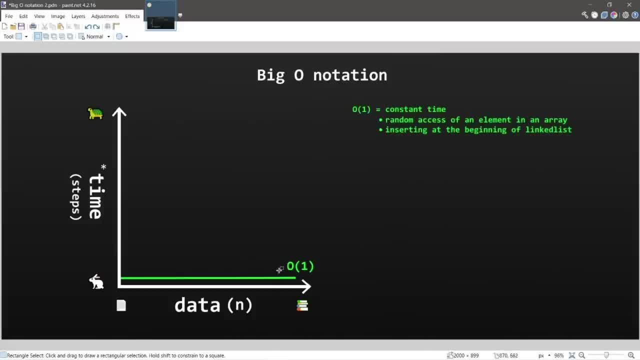 begin with O: constant time. Anything that has a runtime complexity of O will take the same amount of time, regardless of the data size. A few examples would include the random access of an element within an array and inserting at the beginning of a linked list. So O is extremely fast. Next we have O also. 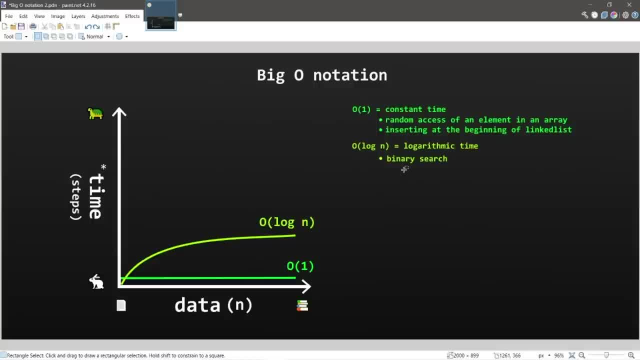 known as logarithmic time. One example is binary search. We haven't talked about this yet. We'll talk about a few of these algorithms in future videos, But anything that has a runtime complexity of O will actually take- I don't want to say less and less time. 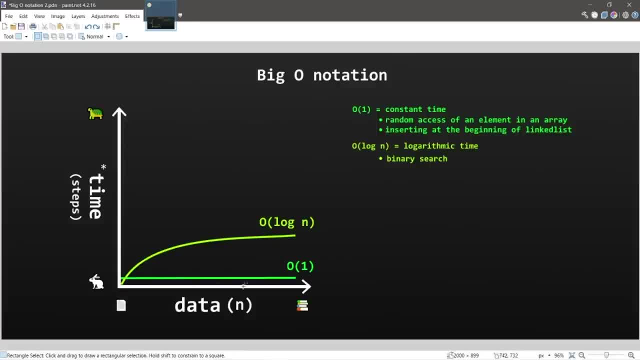 but increasingly less time to complete. So, as the data size increases, this algorithm is going to be more and more efficient compared to the early stages with a small data set. O is also known as linear time. As the amount of data increases, the time it takes to complete something. 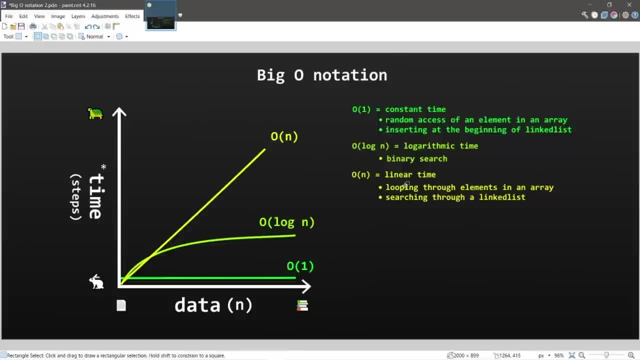 will increase proportionally. linearly, That would include looping through the elements in an array and searching through a linked list. Next, we have O, also known as quasi-linear time. This would include a quick sort, merge sort and heap sort. We'll talk about these concepts in future videos. 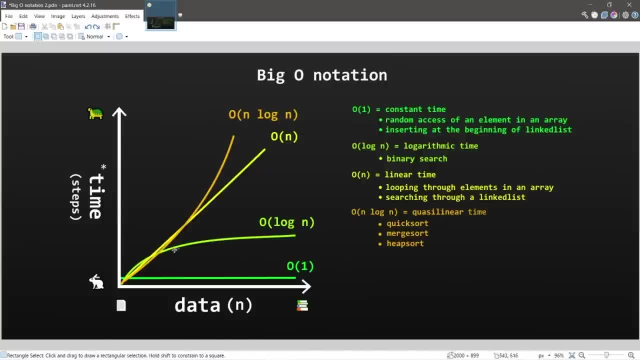 So for the most part this is very similar to linear time. unless we're working with a large data set, Then anything using O is going to start to slow down when we work with larger data sets, hence this curve here. Then we have O, also known as quadratic time A. 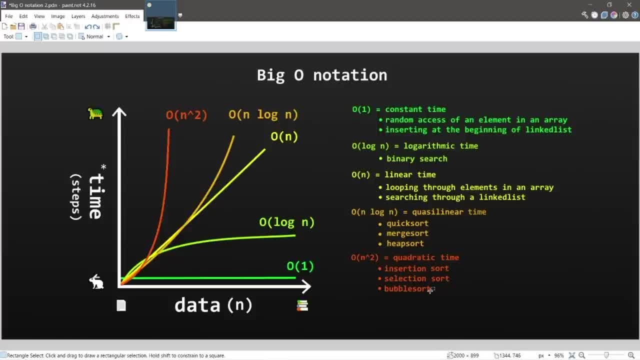 few examples would include insertion, sort, selection, sort and bubble sort. As the amount of data increases, it's going to take increasingly more and more time to complete anything that has a runtime complexity of O. So just to compare linear time and quadratic time With linear, 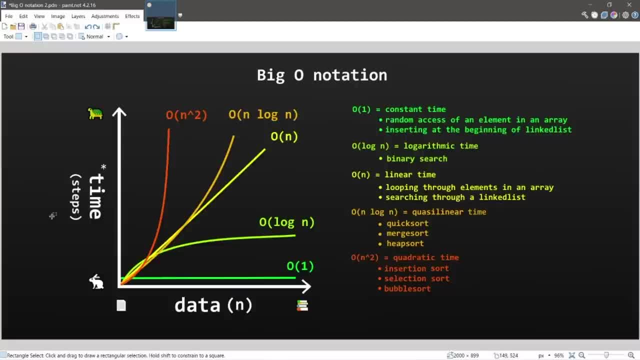 time. if our data set was a thousand, if n equals a thousand, it's going to take a thousand steps. They're proportional, they're linear. But if we were using quadratic time, if n was a thousand, then a thousand squared would be a million. So if our data set was a thousand, if we're using 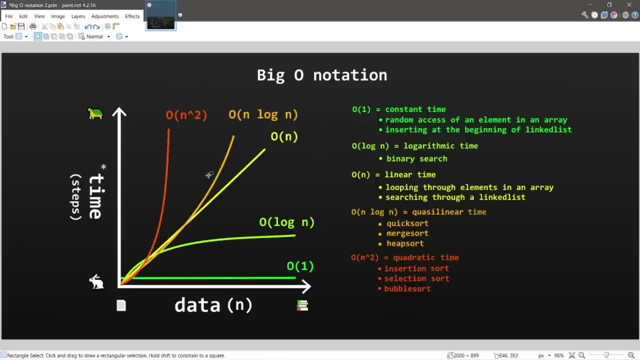 quadratic time. it's going to take a million steps Then, way more than linear time. So quadratic time is extremely slow with large data sets, But in the case of a small data set it could actually be faster, as you can see by the graph here. 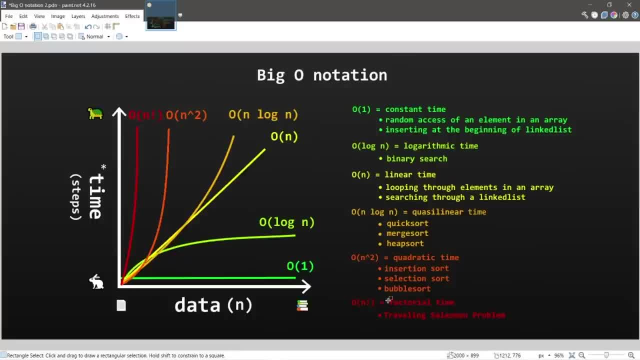 And lastly, we have O, also known as factorial time, And one place where this is used is with the traveling salesman problem, which I might discuss in a future video. So this is extremely slow. So if I had to give a letter grade to each of these runtime complexities when working with 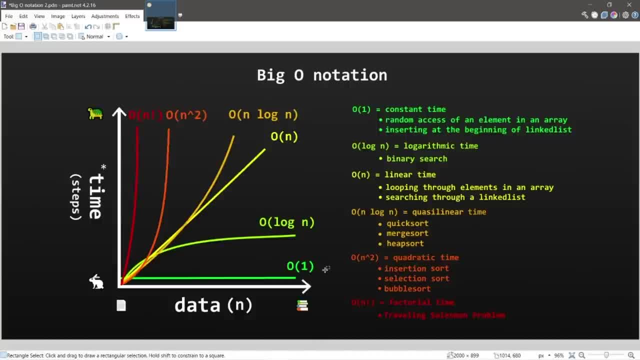 large data sets with constant time. this would be an A like an A, plus Logarithmic time would be a- B, it's pretty good. Linear time is C- it's okay. Quasi-linear time is a- D, it's just barely. 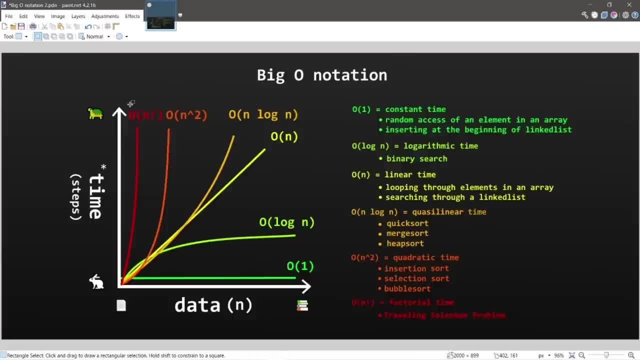 passing. Quadratic time would be an F And factorial time: well, you get expelled from school, Although some of these runtime complexities are actually faster when working with a smaller data set. So keep that in mind. Well, that's the very basics of Big O notation. It's notation used to 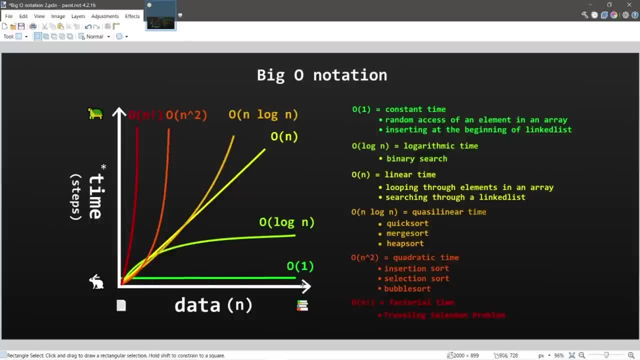 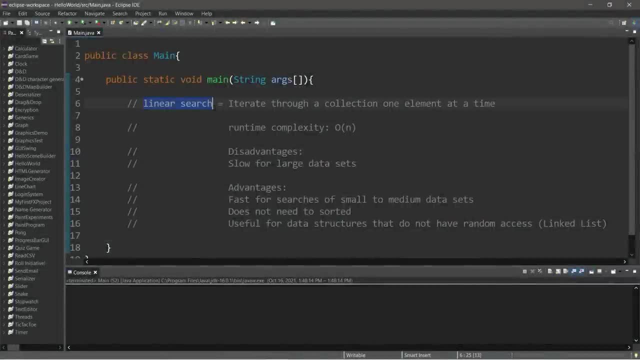 describe the performance of an algorithm as the amount of data increases. So if you can give this video a thumbs up, drop a random comment down below And well, that's Big O notation in computer science. All right, everybody. linear searches: We need to talk about linear searches. 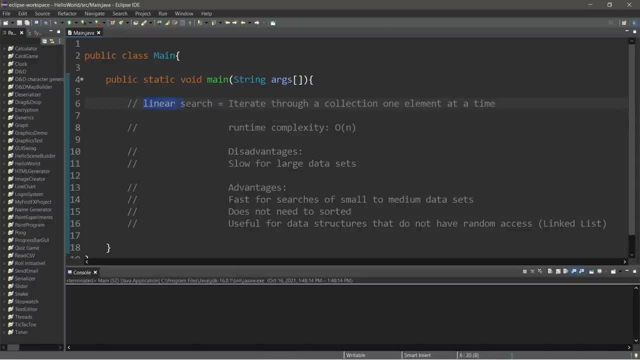 because this wouldn't be a complete course without them. With a linear search, we iterate through a collection one element at a time. The runtime complexity of a linear search is the number of steps to complete that search And so, as you can see, the larger the data set. 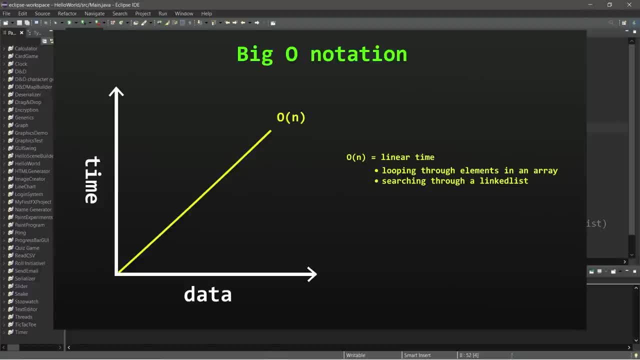 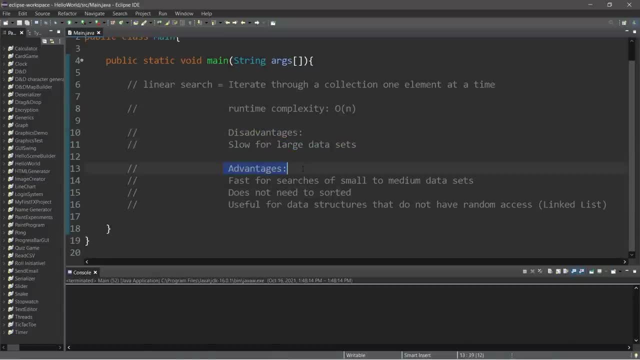 the number of steps to complete that search will increase proportionately. The disadvantages of a linear search is that they are slow for large data sets, But with the advantages they are fast for searches of small to medium-sized data sets And they don't. 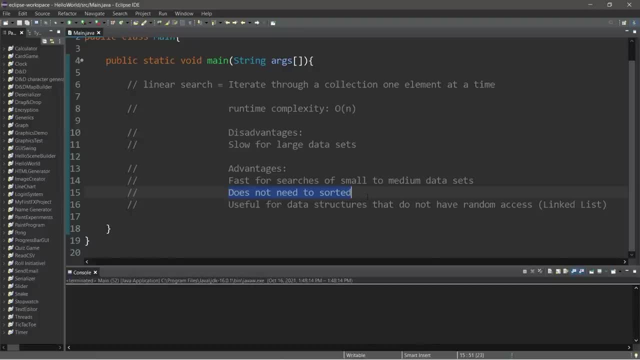 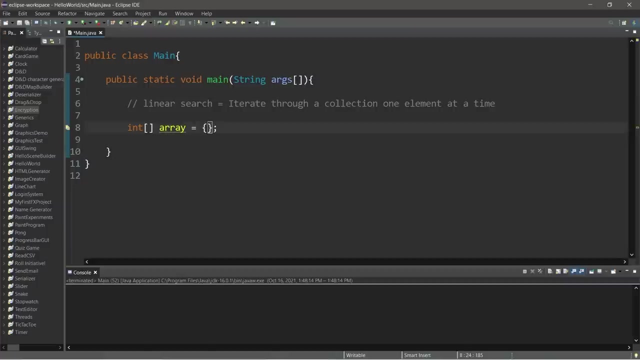 need to be sorted. That's a huge benefit over binary searches and interpolation searches, And they are useful for data structures that do not have random access, such as linked lists. So let's begin. Let's create a basic array of integers, int array- And to make up some numbers, 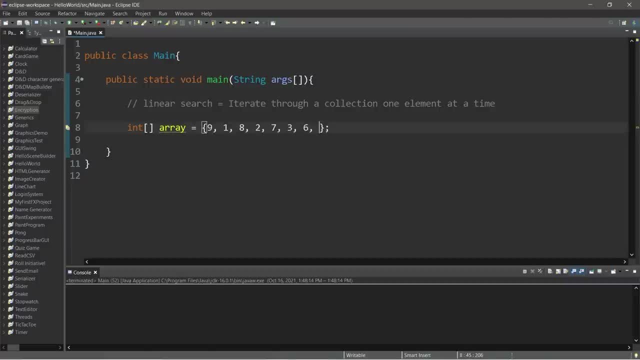 they don't necessarily need to be in order. All right then let's find an index- int index equals- And we will invoke a linear search function, which we still need to declare. We will pass in our array and some value we would like to. 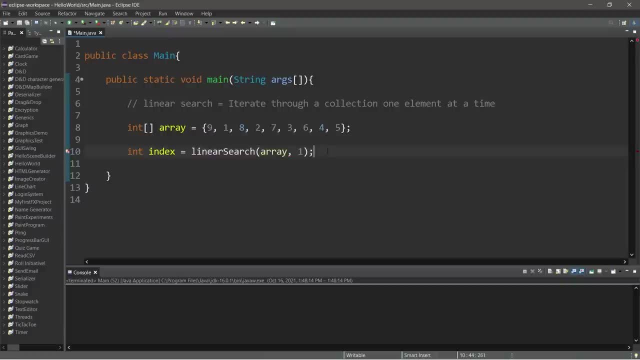 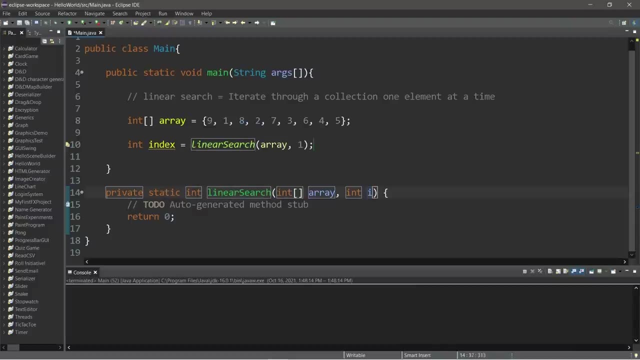 search for. Let's search for the number one, Okay, so then let's declare this function. create method: Linear search, Private, static int, linear search. So we have two parameters: an integer array and an integer. I'm going to rename i as value, so it's more descriptive. 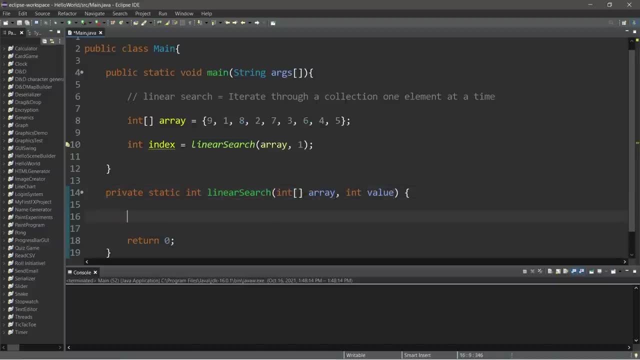 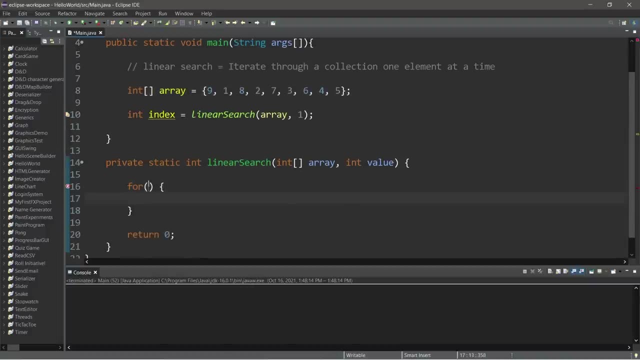 Okay, with a linear search, all we need to do is loop through our array one element at a time. So we can do that with the for loop. So let's set int i our index equal to zero. We will continue this as long as i is less than. 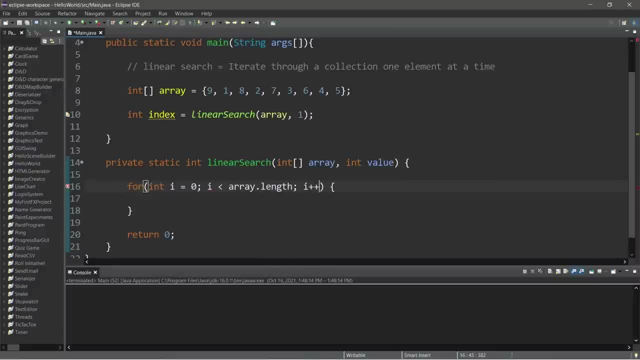 I win my first round And everything's working inside. Anything that counts out on the random types works out perfectly. All right, so I've actually found something. If I want to look for something besides the index, it goes in this browser. 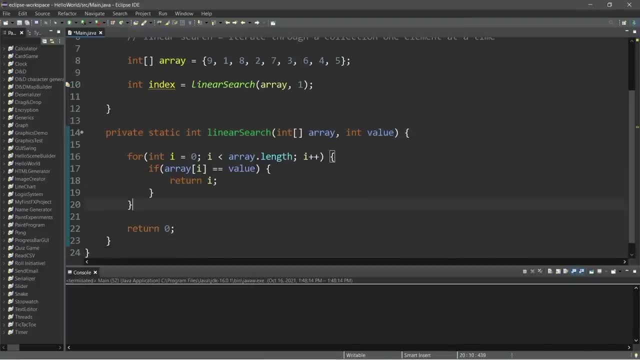 I want a star is represented, so I want to find the number one and if I want to find it, just give a second to the ID want I can export this star to this program. Okay, So it野 cave And we'll return it. 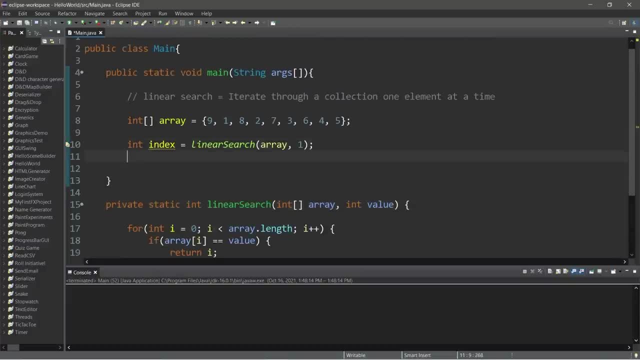 It the hard, blo nasitonow, I'm doing a good job doing it. Thank you, guys, have a great day. So back within our main function, let's check to see if the value returned does not equal negative 1. That means that we found our value. 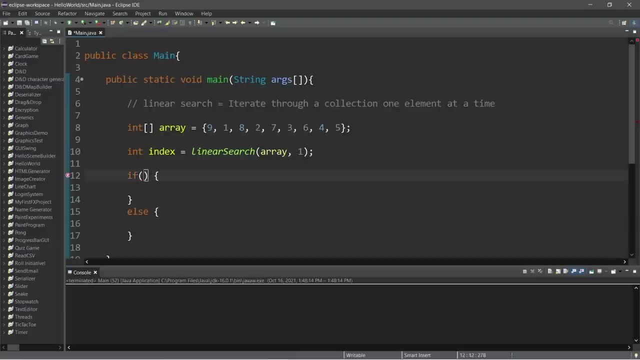 So with an if else statement, let's check to see if index does not equal negative 1. That means that we have found our element. So let's print element found at index plus index. else Let's print element not found. systemoutprintln- element not found. 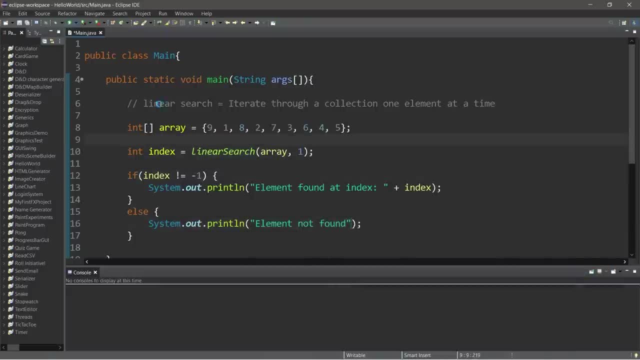 So if we're searching for the number 1, we would find that at index 1, 0, 1.. If we search for 5, that is found at index 8, 0, 1, 2, 3,, 4,, 5, 6, 7, 8.. 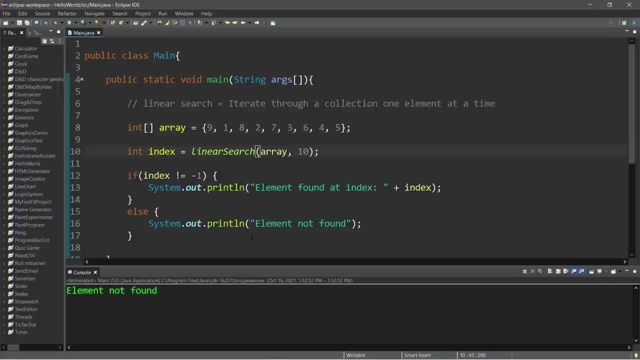 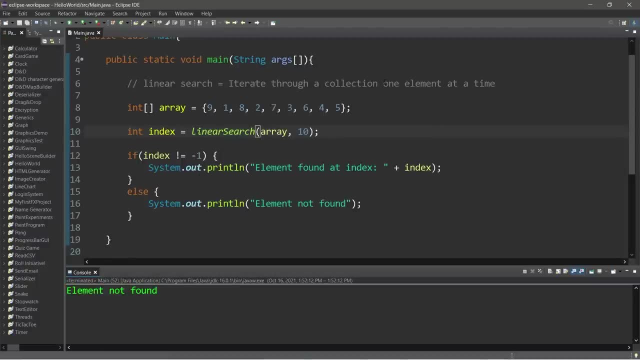 If there's some number that's not in here, like 10,, then this will print element not found. So yeah, that's the idea behind a linear search. We iterate through some collection one element at a time. It's slow for large datasets, but it's fast for small to medium datasets. 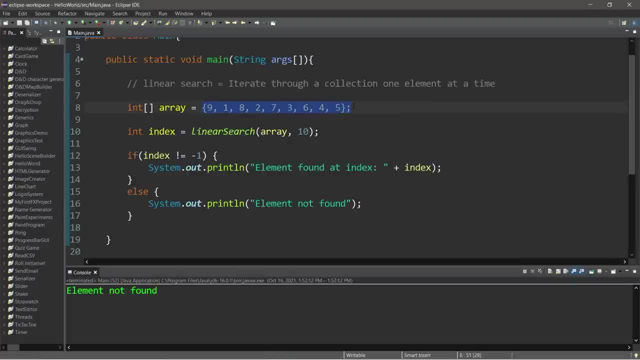 This would be a small dataset And they do not need to be sorted. That's a huge advantage. So yeah, everybody. that is a linear search. If you would like a copy of this code, I'll post this to the comments section down below. 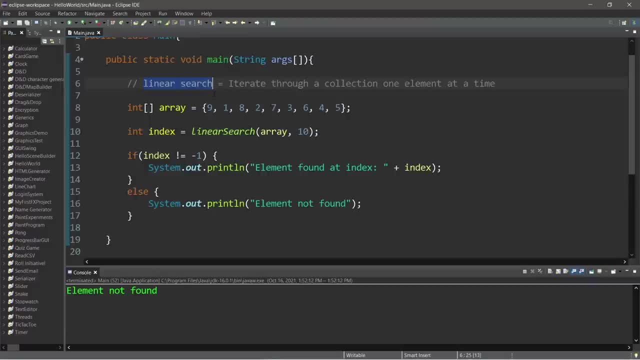 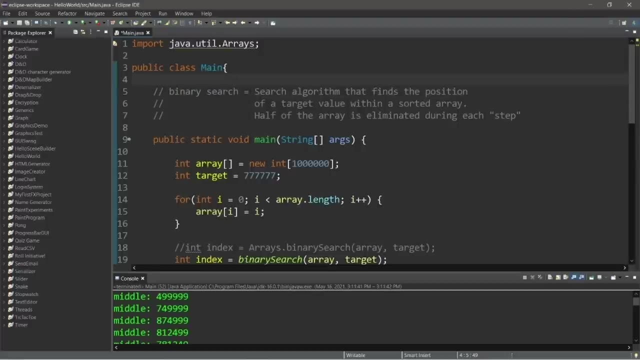 And well, yeah, that is a basic linear search in computer science, I guess. Hey everyone, It's your bro, Hope you're doing well. And in this video I'm going to explain the binary search algorithm in computer science. 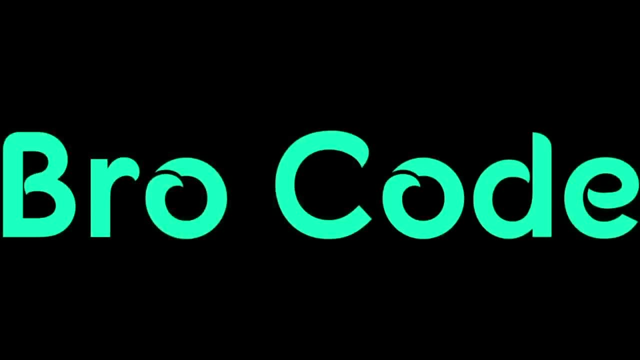 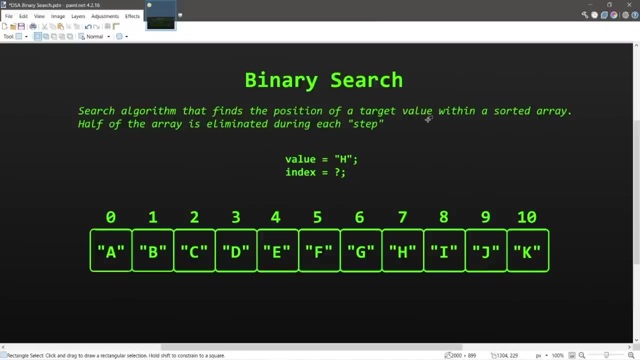 So sit back, relax and enjoy the show. All right. binary search: It's a search algorithm that finds the position of a target value within a sorted array or other collection. In order for a binary search to work, whatever we're searching through, it needs to be sorted. 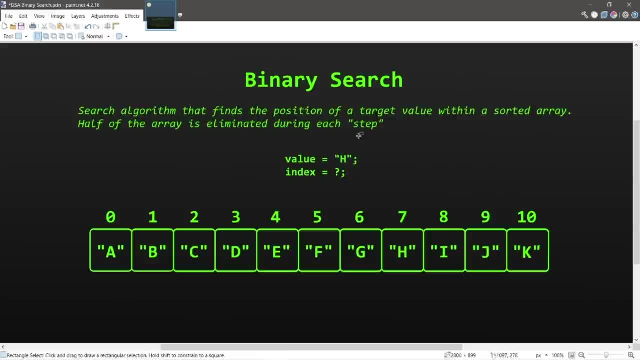 And basically what we do is we take half of the array and eliminate it during each step And we will whittle down our collection until there is only one array, And we will whittle down our collection until there is only one element remaining. In this example, I have an array of 11 elements. 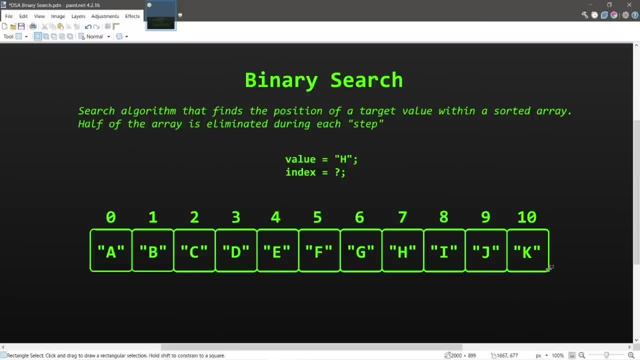 Each element contains a letter and they're all sorted alphabetically. Let's say we are looking for the letter H and I need the index. What we would do with a binary search is that we always begin in the middle. We first check to see if our target value is equal to this middle value. 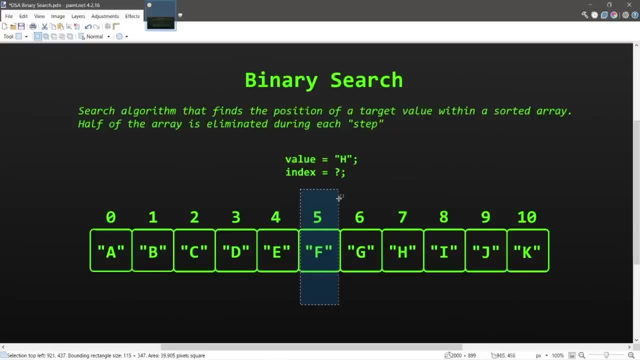 If these are equal, then we can return this index, But odds are they're probably not going to be equal on the very first turn, the very first step. So these are not equal. Then we will check to see if they are equal. 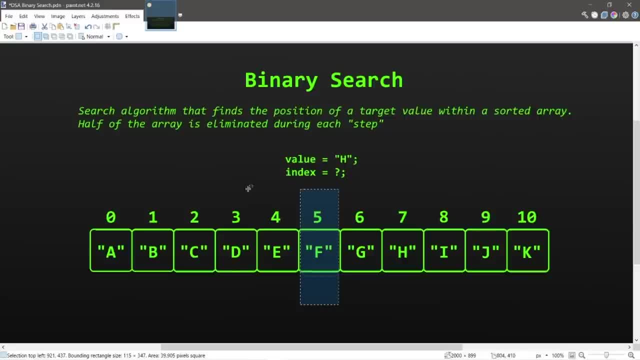 So these are not equal, Then we will check to see if they are equal. So these are not equal, Then we will check to see if they are equal, Then we will check to see if our target value is greater than or less than this middle value. 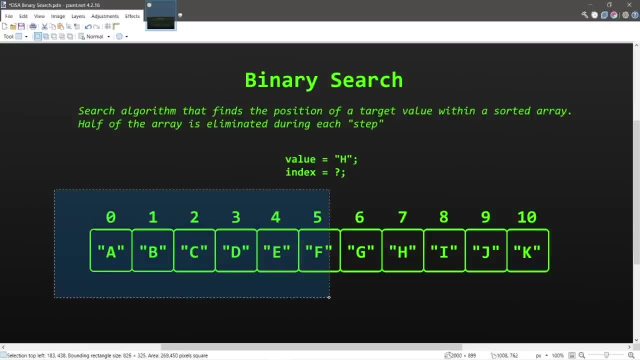 Since H is greater than F, we can disregard this entire first half of our array Because, since this is sorted, our target value could not possibly be within this first portion. And then we begin step 2, or phase 2.. It's the same process as before. 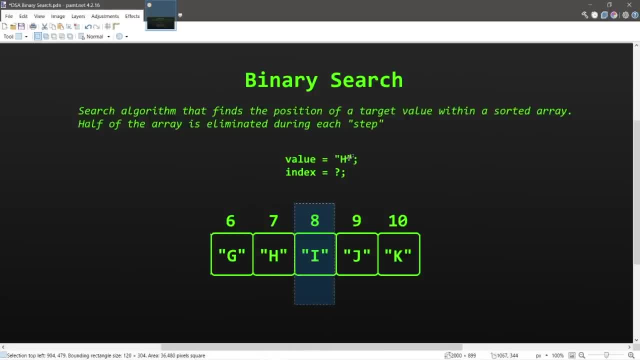 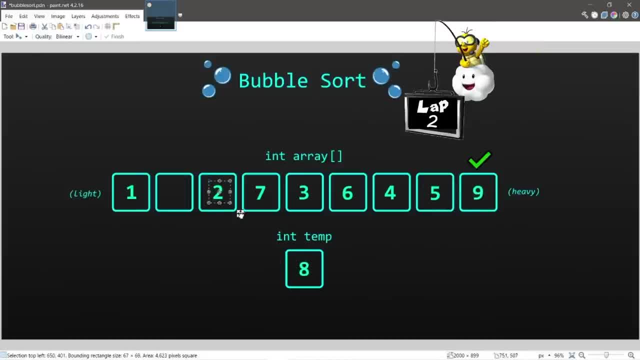 They're not Check to see if our target value is equal to the middle value. They're not Check to see if our target value is equal to the middle value. They're not Check to see if our target value is equal to the middle value. 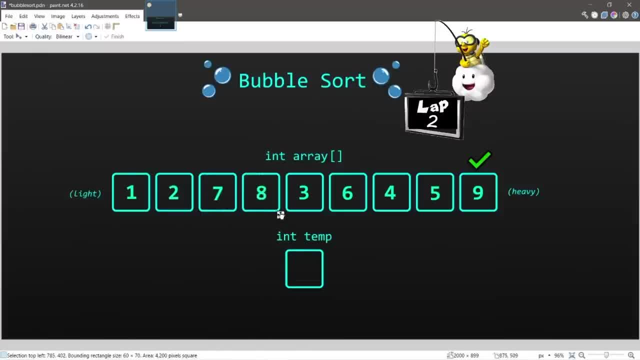 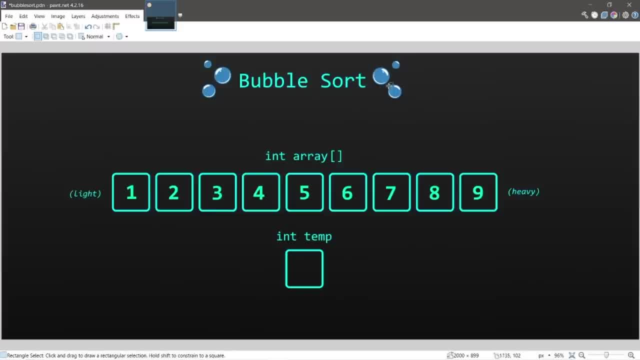 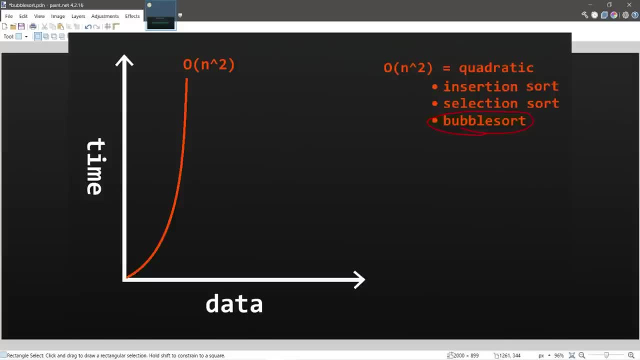 In most real world applications you'll probably use a different sorting algorithm, but this is still a good thing to learn. So the bubble sort algorithm has a runtime complexity of O of N squared. It runs in quadratic time, So the larger the dataset, the more and more inefficient that this sorting algorithm is. 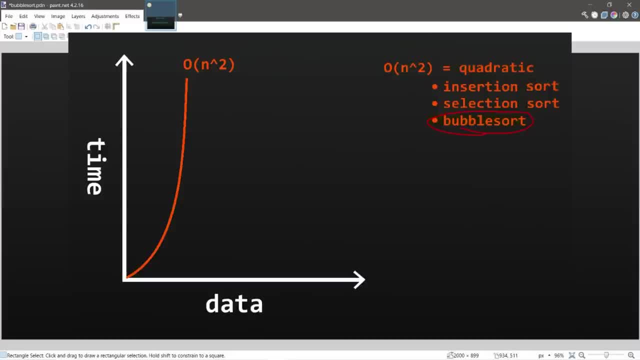 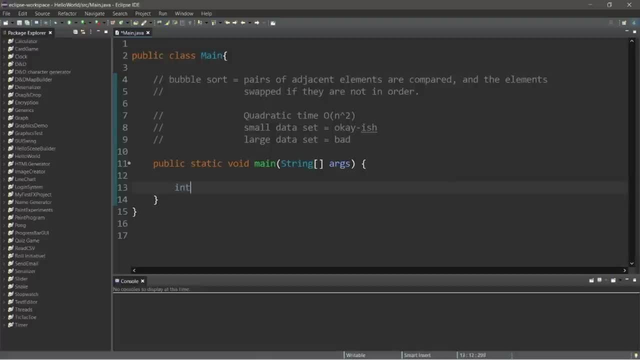 going to be With a small dataset. it's not horrible, but there's definitely better algorithms out there. So for practice, let's create our own bubble sort algorithm. Alright, let's create an array of integers and assign some random numbers. 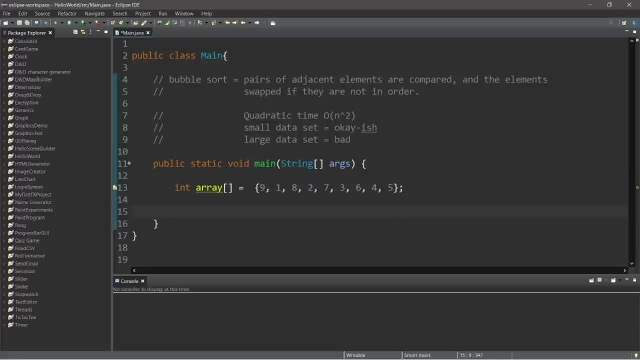 Make sure that they're not in order, because, well then, that would defeat the purpose of this program. So at the end we'll just display all the elements of this array using an enhanced for loop. For i in array we will display with a print statement, not print line, whatever i is during. 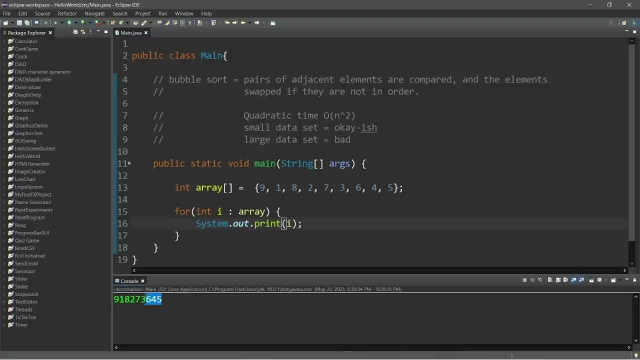 each iteration. So let's just test this. So I have all the elements in my array printed and they're currently not in order. So we'll need to declare a bubble sort method, Bubble sort, And then we will need to define this outside of our main method. 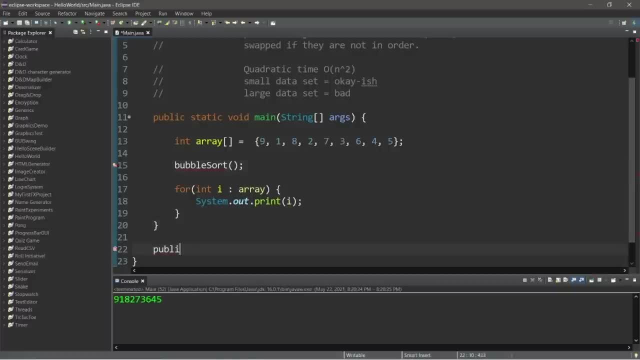 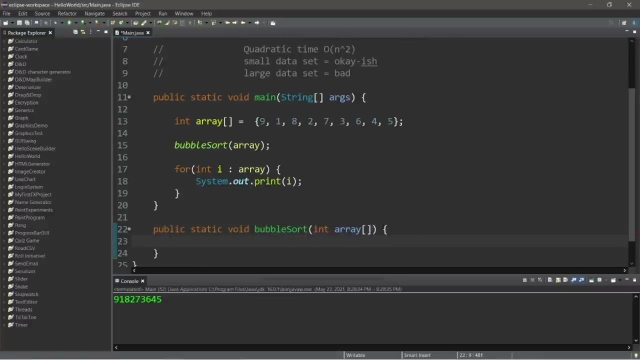 So public static void, we're not returning anything bubble sort, and then we will need to pass in an array. So that will be the argument array and we will accept int array. Okay, so this is actually really easy to write, even though the bubble sort algorithm really. 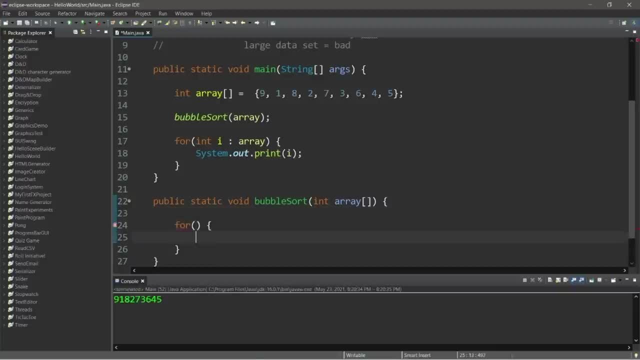 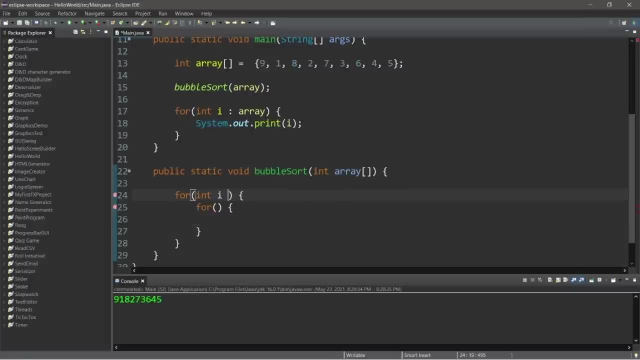 isn't too efficient, So I guess that's one benefit. So we'll need nested for loops And then the outer for loop will be int. i equals zero, i is less than arraylength minus one, i++. And let's do the same thing with the inner for loop. but we can copy what we have change. 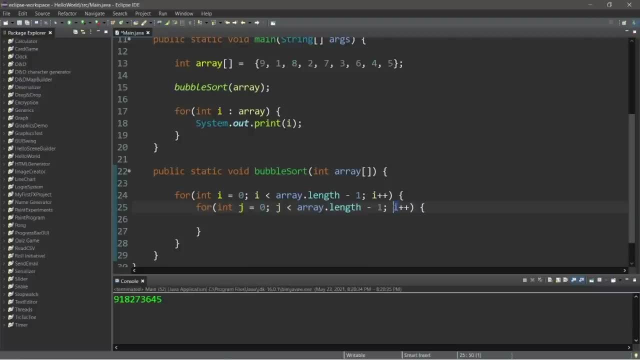 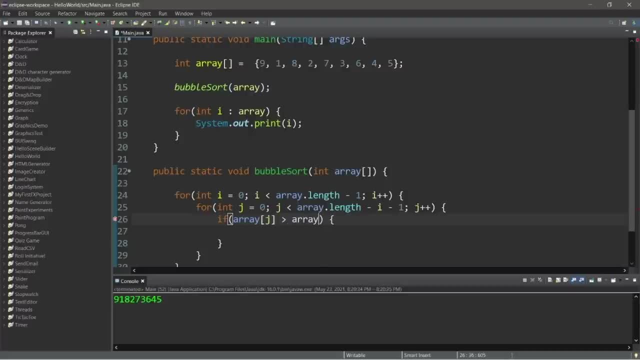 for ascending order is greater than array at index of j plus one, So that would be the next adjacent element. So if this number is greater than this one, We should switch these two elements around and we'll need the assistance of a temporary variable. 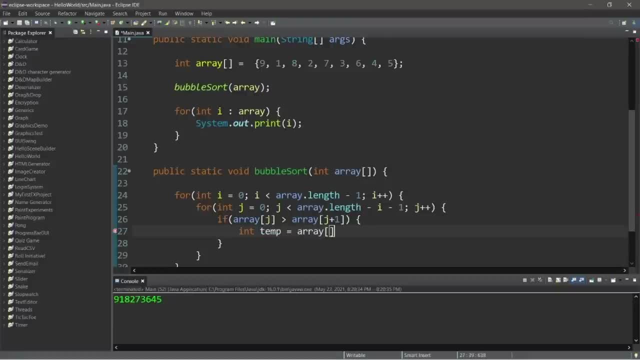 So let's declare int temp equals array at index of j. Then we will take array at index of j, set this equal to array at index of j plus one, And then, lastly, we have array at index of j plus one equals array at index of j plus. 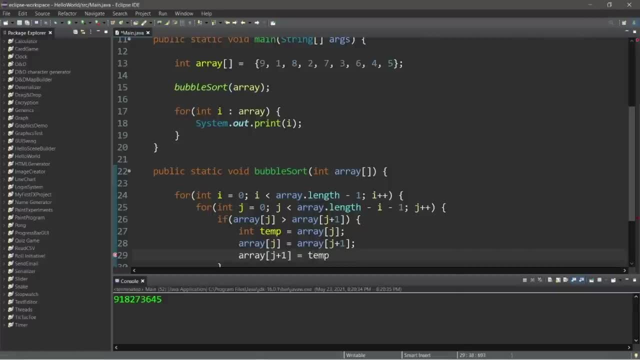 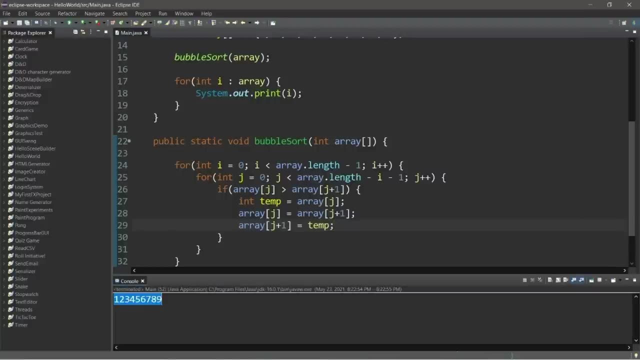 one. Then we have array at index of j plus one equals array at index of j plus one equals whatever is stored within temp And honestly, that's all there is to it. So this should sort our array and it's in ascending order. 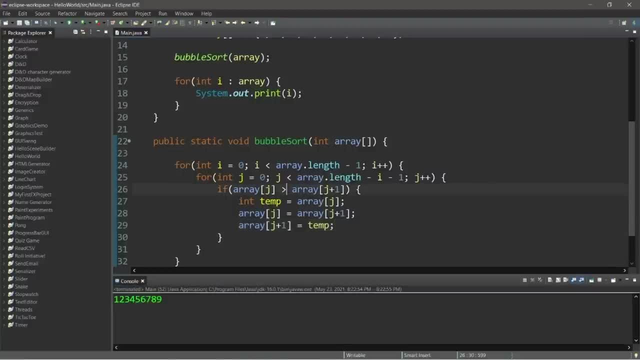 So if you need this in descending order, we would just swap this greater than sign with a less than sign, And now this is in descending order. So even though the bubble sort algorithm really isn't too efficient, it's actually extraordinarily easy to write if you just need something really simple. 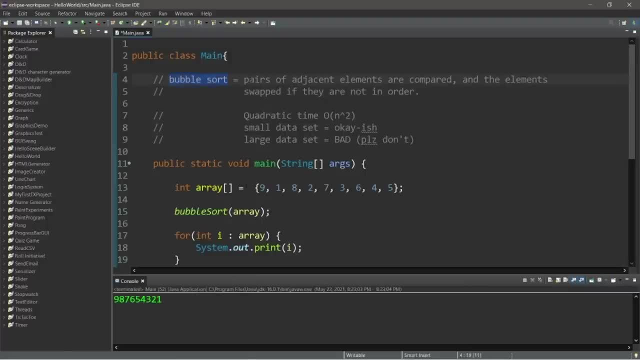 So I guess that's one benefit. All right, everybody. That's it. Thanks for watching. That is the bubble sort algorithm. It compares pairs of adjacent elements and checks to see if they're in order. If they're not, they're swapped. 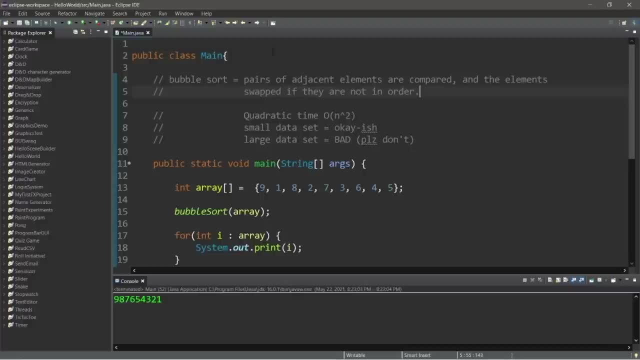 And this process will repeat once for each element in an array or other collection. So this algorithm has a runtime complexity of O of n squared, So it's okay-ish for small data sets And please do not use this for any large data sets. 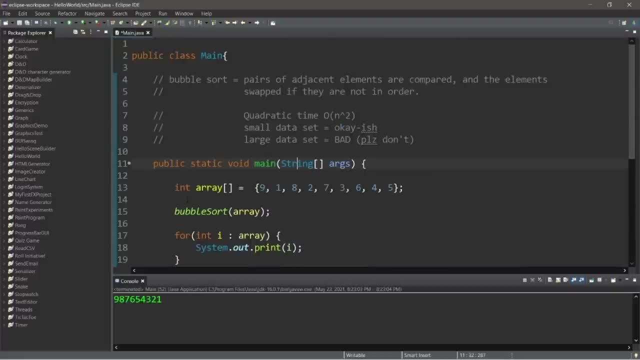 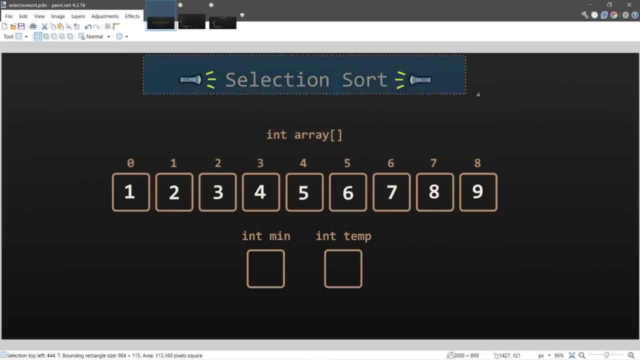 So if you would like a copy of this code, I will post this to the comment section down below. And well, that's the bubble. sort algorithm in computer science. Hey everyone, It's me again, And in this video I'm going to explain the selection sort algorithm in computer science. 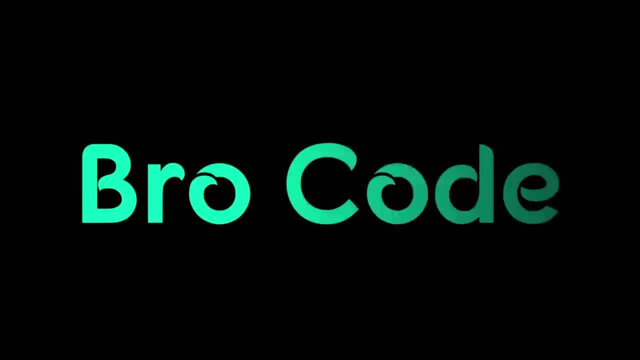 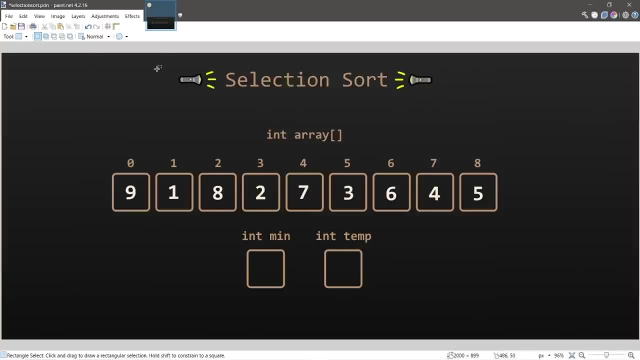 As always, sit back, relax and enjoy the show. Okay, everybody, Selection sort. Selection sort is an in-place comparison sorting algorithm that keeps track of the minimum value during each iteration And at the end of each iteration. all we do is swap variables. 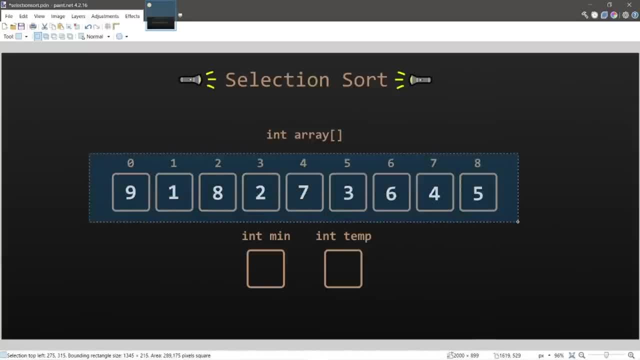 How I like to imagine this Is that let's say that our array is a bunch of different closed boxes and each box contains a number, and they're all out of order. So what we'll do is we have a flashlight too, because we're in the attic and it's really 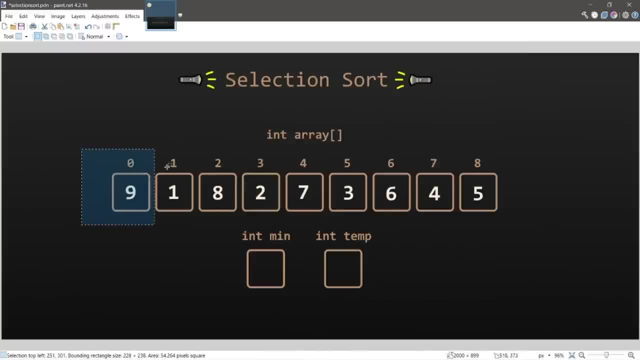 dark. So we have a flashlight. We will open each box beginning with the beginning of our array and we'll take a look at the value inside. Okay, Nine is a fairly small number, I guess, right, So we will move this value to some temporary storage. 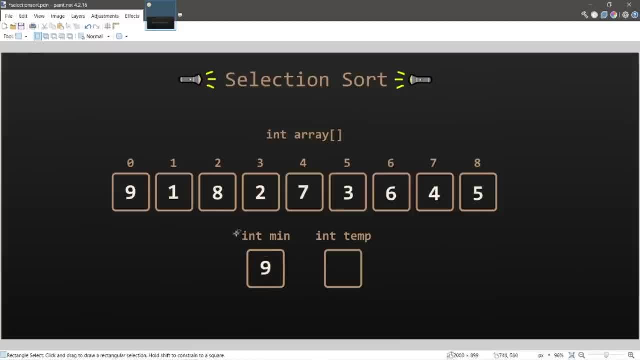 We'll keep track of the index of the minimum value. Nine: Let's open the new minimum. Let's open the next box and, holy crap, it's a one. One is a really small number, So that will be the new minimum. 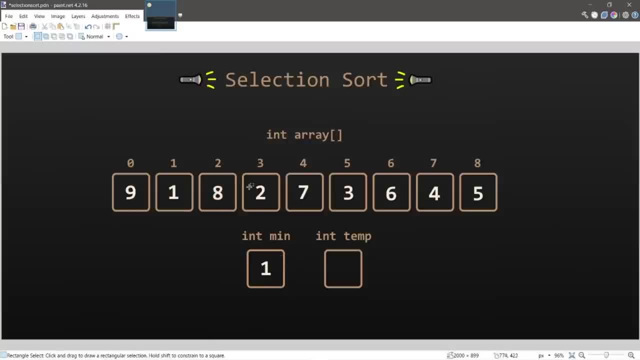 Then we'll open the next box, which is an eight. One is still less than eight. Let's move on. The next box is two, seven, three, six, four and five. One was the minimum value during this iteration and we need to move this value to the place. 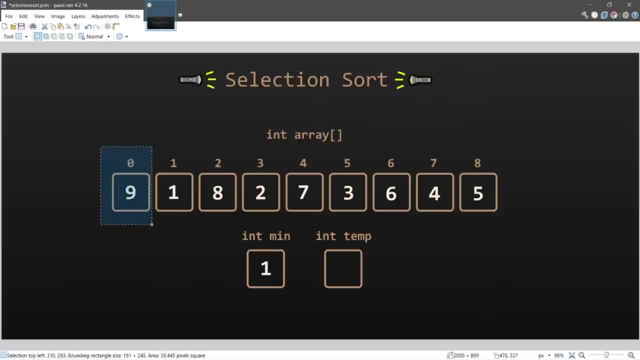 that we started during this iteration index zero. So we'll have to do some good old variable swapping. So we will take nine, Place it within some temporary storage, Then take one and place it where nine was, Then take nine and place it where one was. 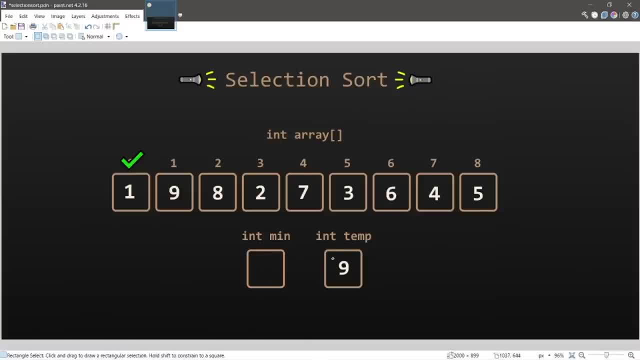 And that is the first iteration. Let's move on to iteration two and we'll clear min and temp. Okay, So this portion is done now. We're not worried about it. This is the new beginning of the next iteration. And well, nine is a low number, I guess. 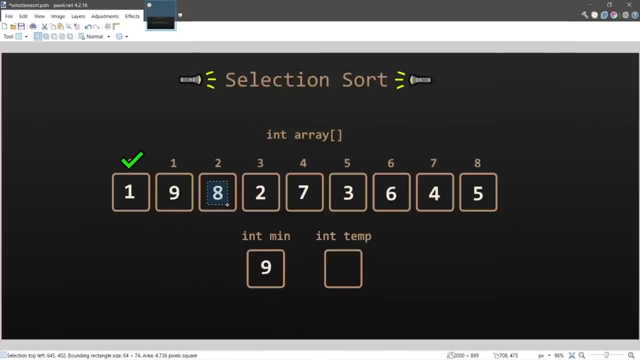 We'll move that to min. But eight is even lower than nine, So we'll move that to min. Holy crap, it's a two. Two is the new min, for sure. And then we just repeat this process over and over again. 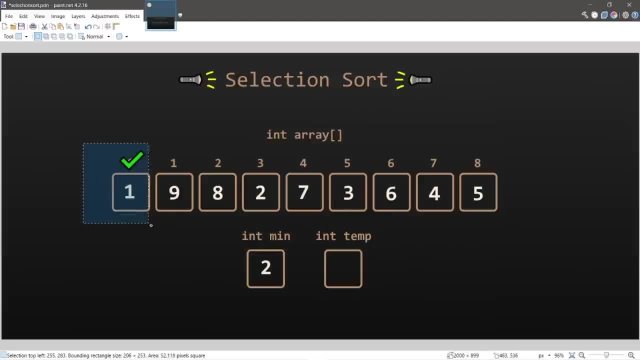 Two is the current minimum of this iteration. One was the minimum of the first iteration, but we're not concerned with that, It's already sorted. So we need to move two to where we began this iteration, at index one, And currently there's a nine in there. 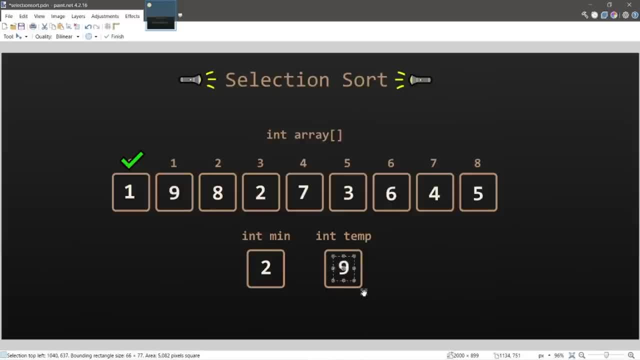 So we're going to evict this nine, Place it within some temporary shelter. Take two, place it within where we started at index one, Then take nine, place it where two was. And that is the second iteration. Now that we kind of know how this process works, I'll speed up the rest of the video. 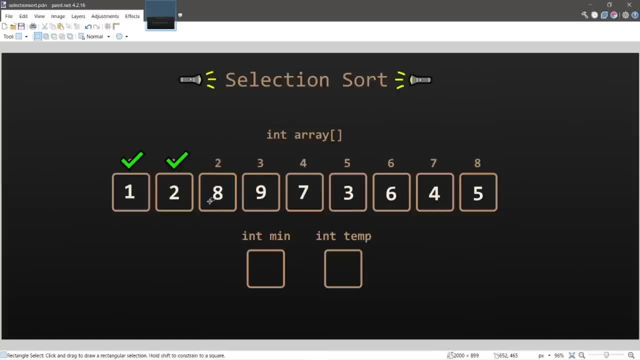 for this demonstration. So let's begin at index two. Well, we have a lot of thing to do here. Two should be up. One and two are here. One is a default, One is a free run. One is a free run. 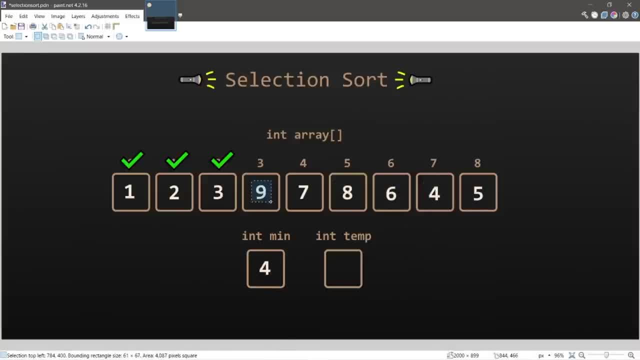 One is an in-use. Wow, Finally three, Three, Three and two. So we do that and we take a look at index one. One is a free run, One is an in-use. One is a free run, One is a free run. 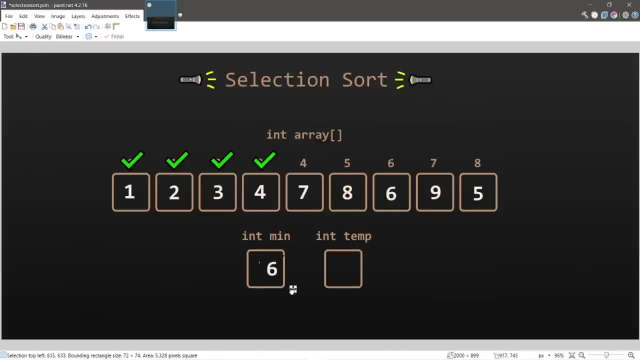 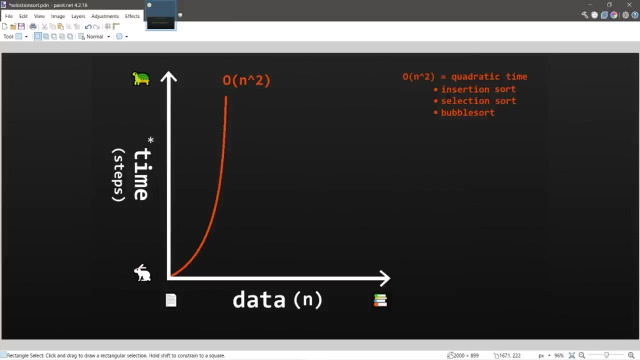 Six Five, Six, Five, Six, Six, Six Six, Thank you, And that is the Selection Sort Algorithm. The Selection Sort Algorithm has a runtime complexity of O of N squared. The larger the dataset, the more and more inefficient that using the Selection Sort Algorithm is going to be. 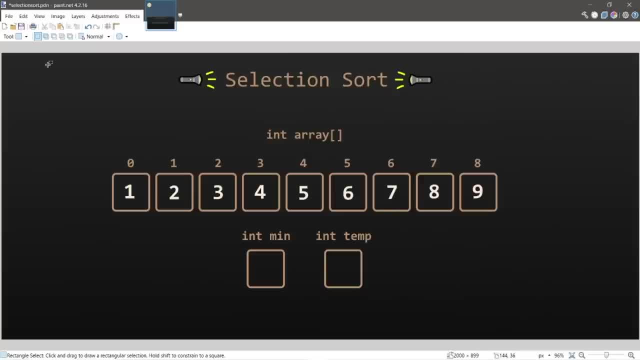 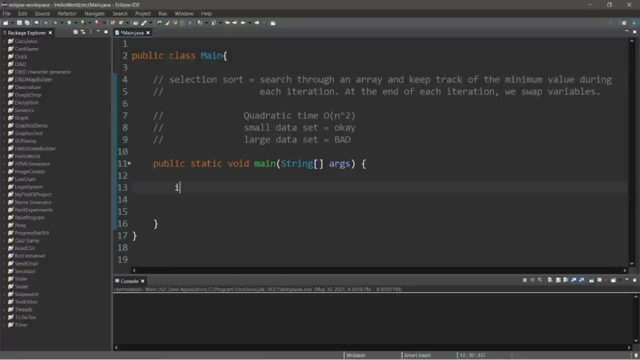 Although it's okay with smaller datasets. Now let's create our own Selection Sort Algorithm. Okay, let's implement a Selection Sort. We'll need an array or other collection to work with. Let's create an array of integers, because I want to make this as easy as possible. 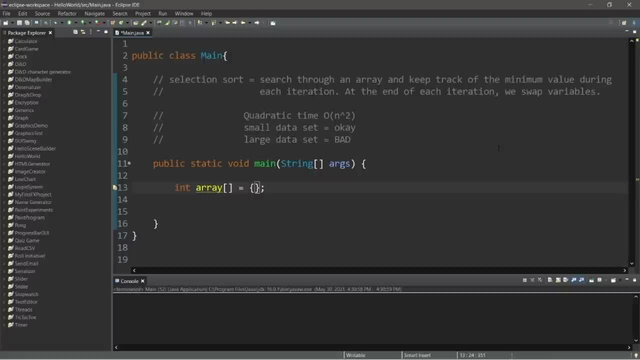 So integer array and make up some random numbers. Make sure that they're not in order. What about 8, 7, 9,, 2, 3,, 1, 5,, 4, 6, I guess? 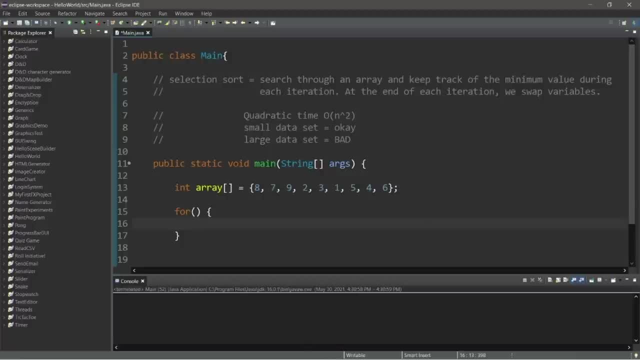 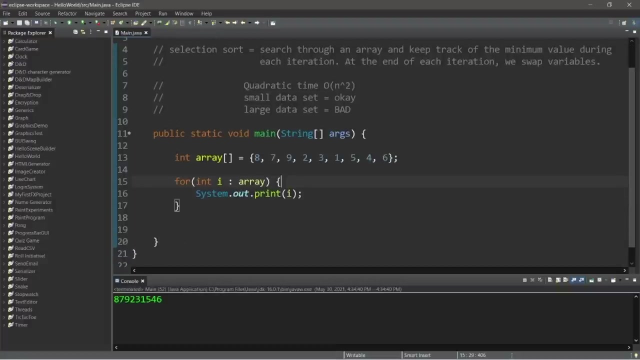 Then let's use a for each loop to iterate over The elements of this array. For int i in array, we will display each element with a print statement, Systemoutprint i. And let's run this once just to be sure that everything is working fine. 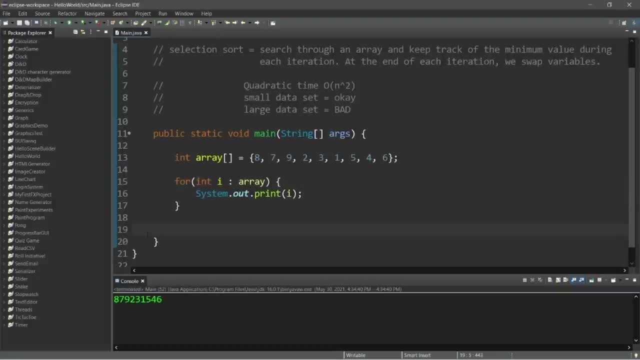 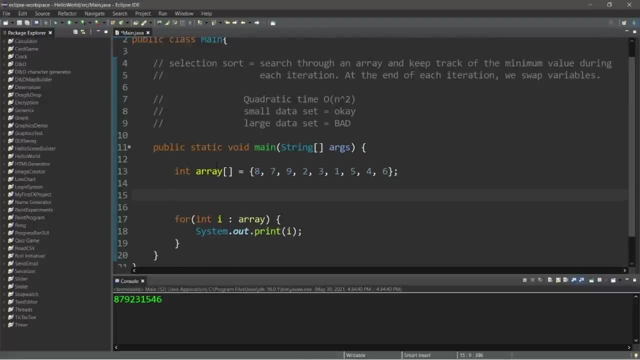 So 8,, 7,, 9,, 2,, 3,, 1,, 5,, 4, 6.. Everything is working as it should. So, before we display the elements of our array, let's invoke a Selection Sort function, which we still need to declare. 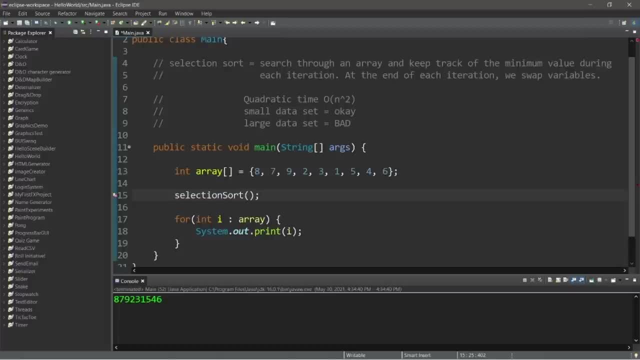 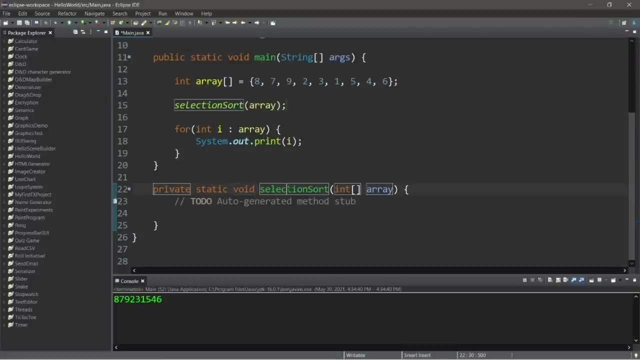 So Selection Sort And we will pass our array as an argument because, well, that's what we want to sort, right? So Selection Sort And we'll need to create this method. I will cheat and use the shortcut. So, outside of our main method, let's declare private static void. Selection Sort. 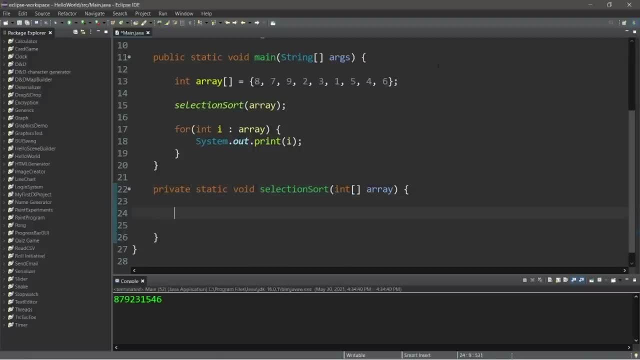 There is one parameter: an array of integers. We'll need a pair of nested loops to iterate over our array, So let's work on the outer loop, For int i equals 0.. We will continue this as long as i is less than. 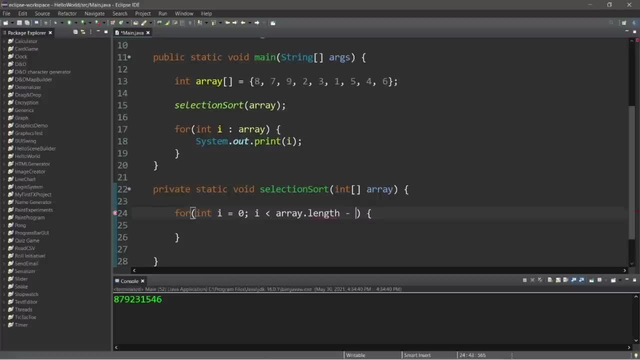 Array's length property minus 1.. Then increment i by 1 during each iteration. Then there is a nested loop within here. Change i to j, So j equals i plus 1.. j is less than array length And j plus plus. 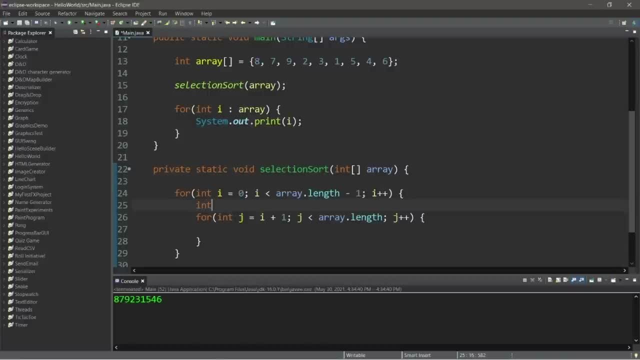 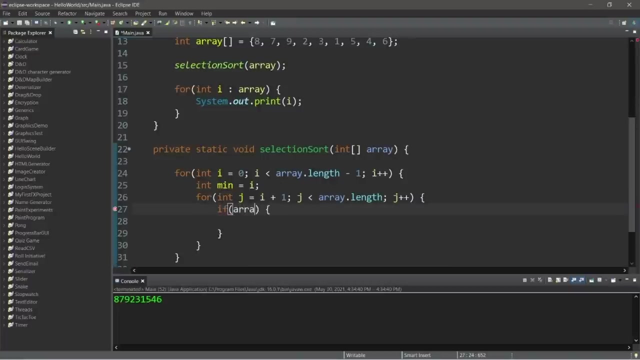 So we'll need to keep track of the minimum. So we'll do that outside of our nested loop. Int min Equals i, So that is the current minimum And within the nested for loop we will check to see if our array at index of min is greater than array at index of j. 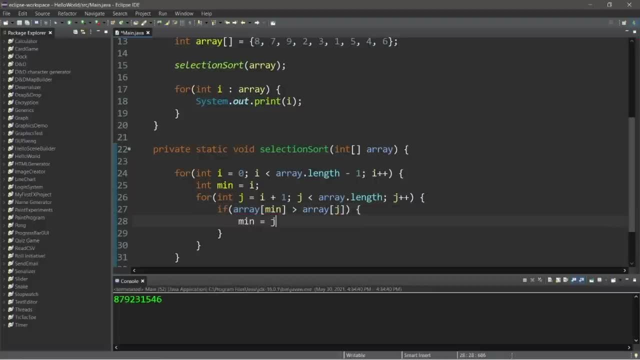 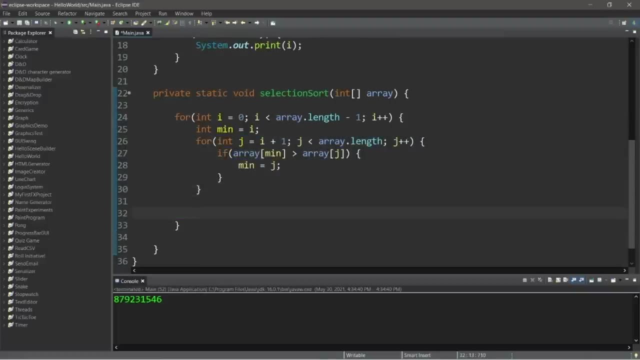 If it is, we will change our min to equal j. Then, outside of our nested loop, but within the outer loop we will do some good old variable swapping. So int temp equals array at index of i to store this element. Array at index of i equals array at index of min. 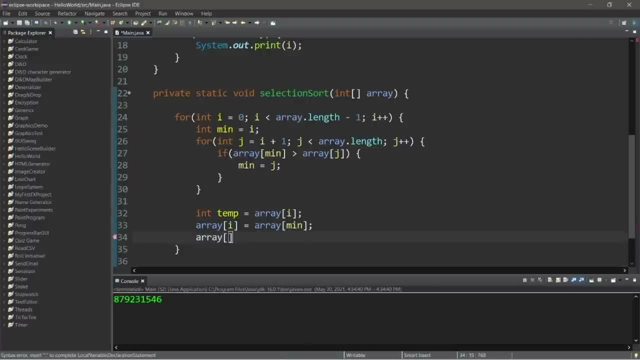 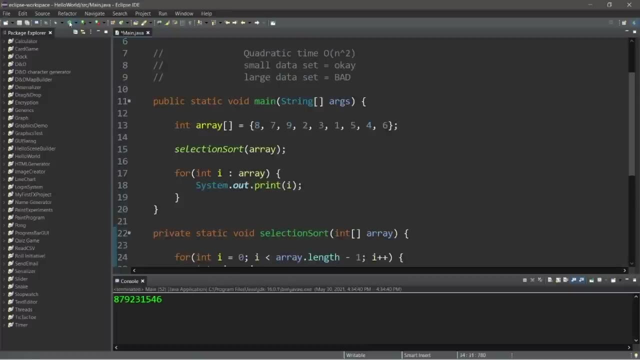 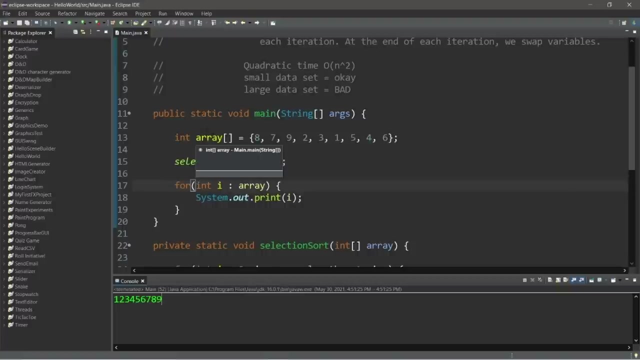 Then, lastly, array at index of min equals temp, And that's all there is to it. So, after running this program, our array is now sorted via the selection Sort Algorithm. Then, of course, if you need your array or collection sorted in descending order, 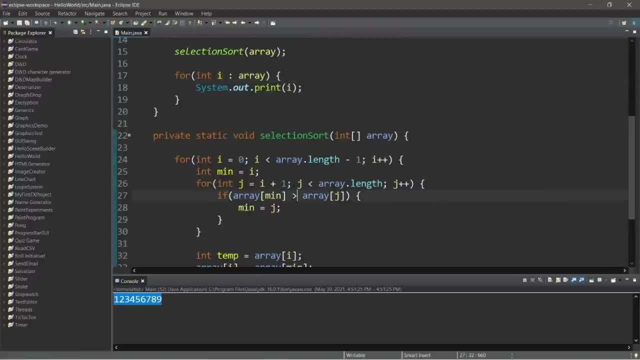 Currently, it's in ascending order. All we do is swap this greater than sign with a less than sign, And this will now be sorted in descending order, depending on what you need. Well, okay then everybody. That is the selection sort algorithm. 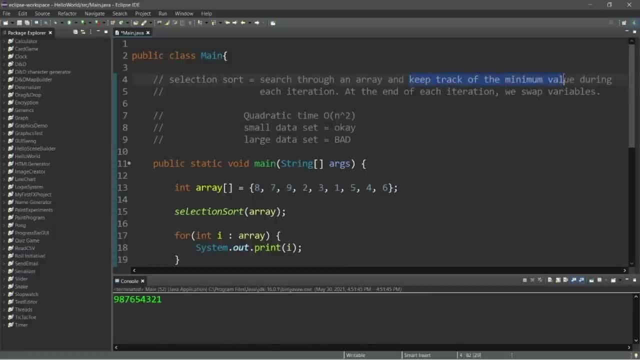 It will search through an array and keep track of the minimum value during each iteration. At the end of each iteration we swap variables And that's all there is to it. It runs in quadratic time. Big O of N squared. It's okay with small data sets. 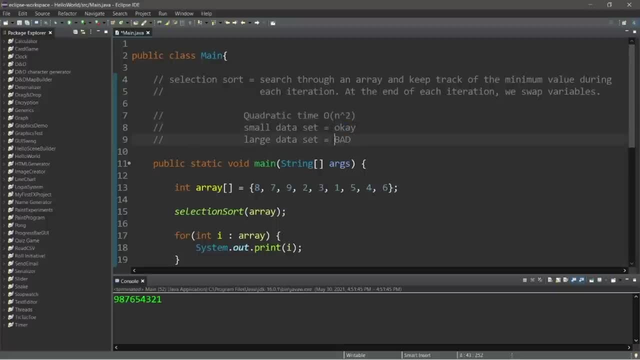 Even more so than bubble sort, And it's pretty terrible with large data sets. The larger the data set, the more and more inefficient that this selection sort algorithm is going to be. So that is the selection sort algorithm. If you learned something new, give this video a big fat thumbs up. 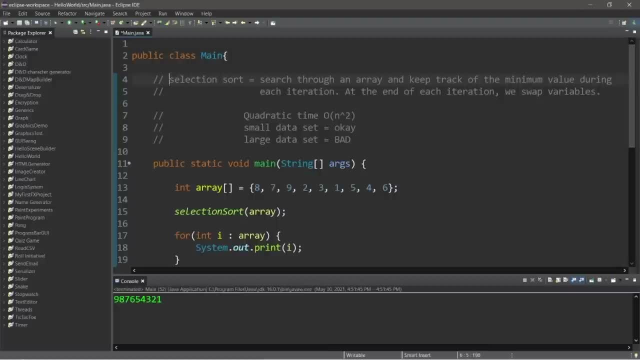 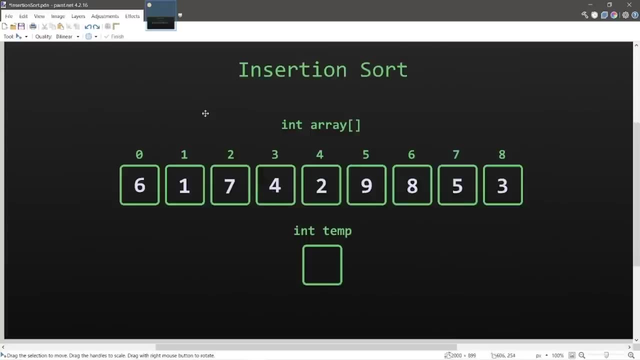 Drop a random comment down below. And well, that is the selection sort algorithm in, I guess, computer science. What's going on, people? It's Bro, Hope you're doing well, And in this video we're going to discuss the insertion sort algorithm in computer science. 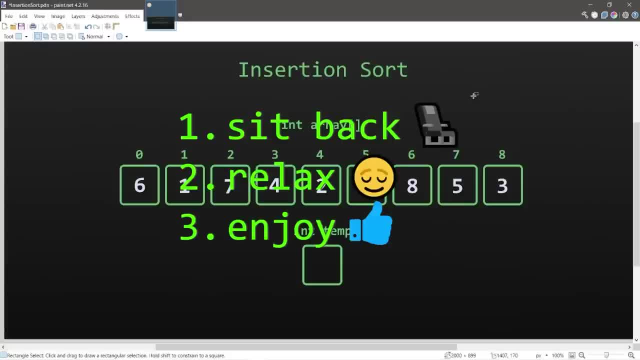 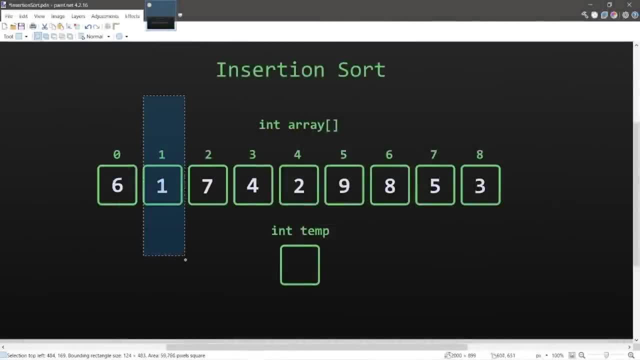 As always, sit back, relax and well, enjoy the show. Alright, everybody. insertion sort. Now, what we do with insertion sort is that we begin at index 1. We take the value found within, move it to some temporary storage, like a variable named temp, to temporarily hold it. 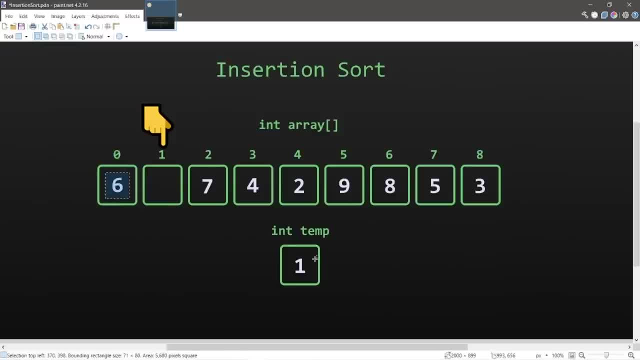 We examine elements to the left. If any elements are larger than what's within temp, we shift those elements to the right. So 6 is larger than 1.. We shift it to the right. If it's less than whatever's within temp, we stop, or until we run out of elements. 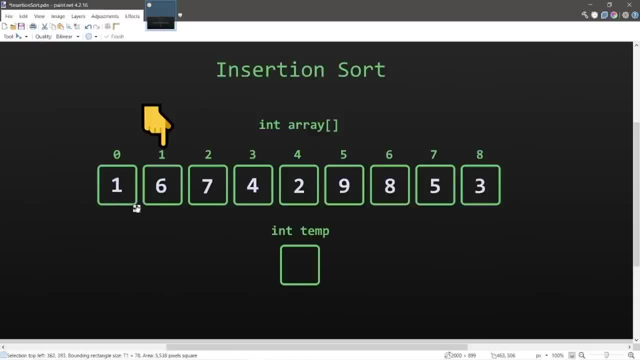 So we have run out of elements. We take this value found within temp and place it at this opening here. That was the first iteration. Let's move on to iteration 2.. Take this value, place it within temp, examine the elements to the left. 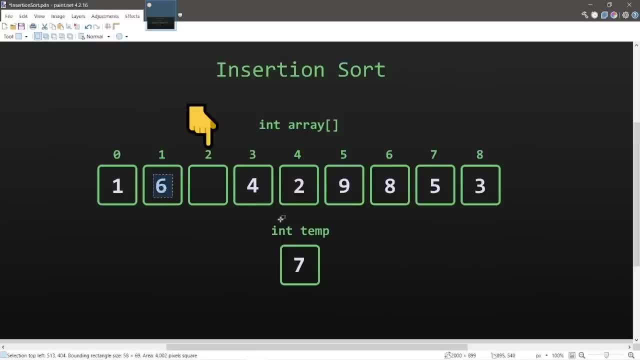 If this element is greater than temp, then we shift it to the right. It's not, so we stop here and place this value back where it came from. So that was the second iteration, Iteration 3.. Take this value, place it within temp, examine the elements to the left. 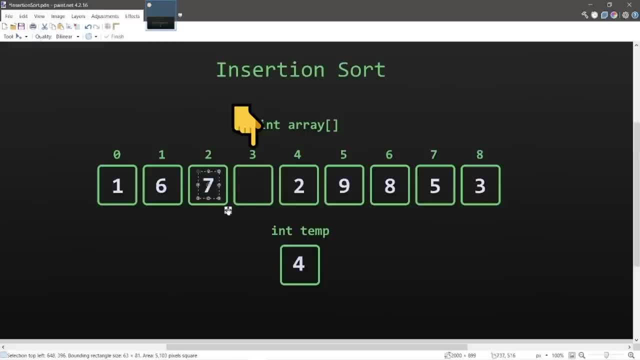 If they're greater than 4,, we shift them to the right. 7 is larger than 4, shift it to the right. 6 is larger than 4, shift it to the right. 1 is not larger than 4,. so we stop here, take whatever's within temp, this value 4, and insert it here into this opening. 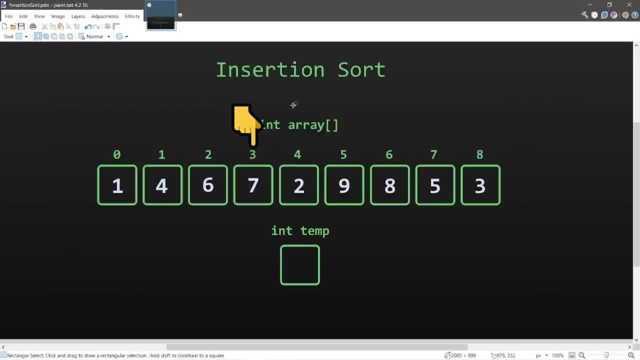 So that was the first three iterations. We repeat this process until we run out of elements, So I'll speed up the footage. So we are currently on index 1.. Index 4.. We pass this index to index 7.. Deweight 6.. 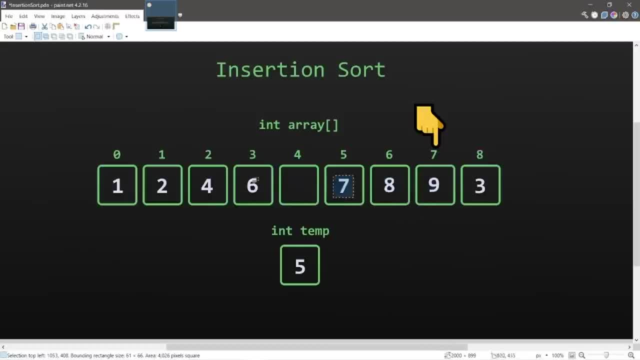 Let's try first indexing. We pass this index to index. 7. Deweight, 8. Deweight, 9. Deweight, 10.. Let's try index Ab envolv: 5. Deweight, 8. Deight, 12. Deeging, 14.. 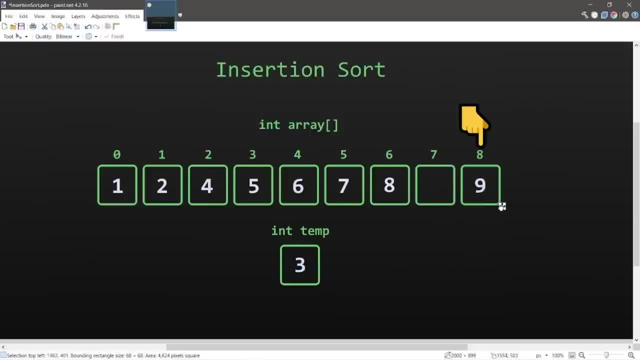 Diagonal 7. Deeging, 15. Diagonal 8. Diagnrator: 2. Deeging, 2. Agon 12. Parallel, 16. Diagonal 1. DeegGash, 15. Diagonal 3.. 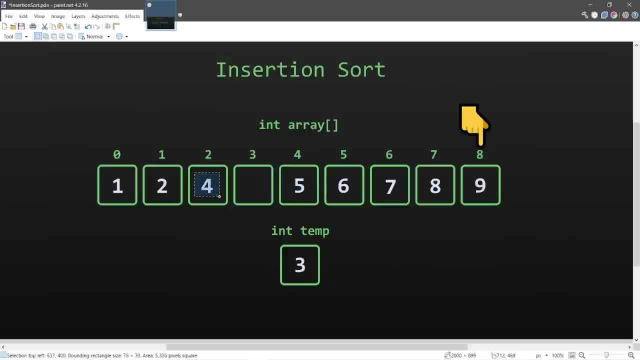 Diagonal 4.. And that is your visual representation of the insertion sort algorithm. I like to think of it like a jigsaw puzzle. We have some pieces that are connected, they fit together, and we will move whole sections of pieces together to make room for a piece that fits. So let's create our own. 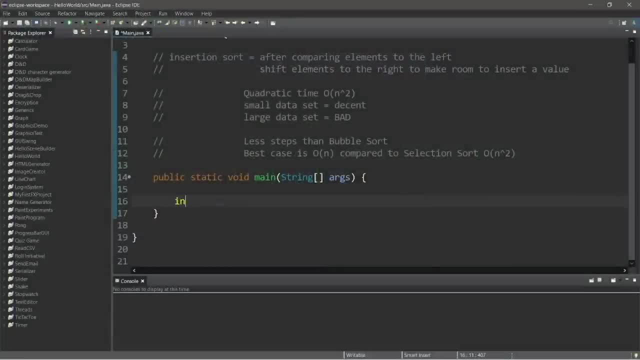 insertion: sort algorithm in Java. now We'll need to create an array. Let's create an array of integers- int array- and make up some numbers. Put whatever numbers you want within here. Maybe nine. how about a one and an eight and a two and a seven, three, six, five, four? That sounds. 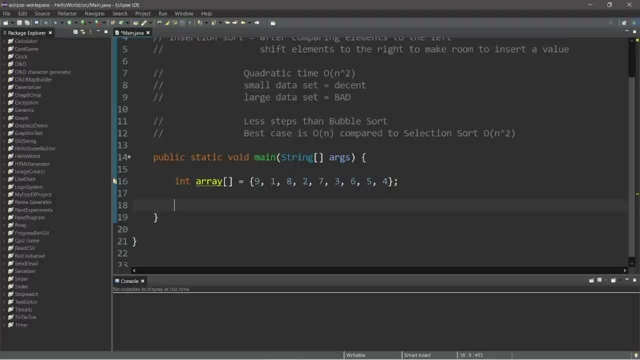 good to me. Okay, then let's display the elements of this array. We'll use a for each loop, For int i in array. we will display each element within this array with a print statement. So let me get rid of that print ln and just have print. So I will print i. I think I'm going to add. 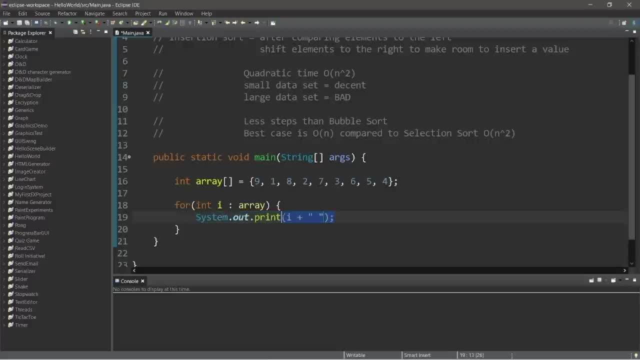 a space afterwards. I didn't do that in the previous two videos, so I think I better do that. Okay, let's just run this, just to test it: 918273654.. And before we display the elements of our array, let's invoke a function which we still need to declare, called insertion sort. So, 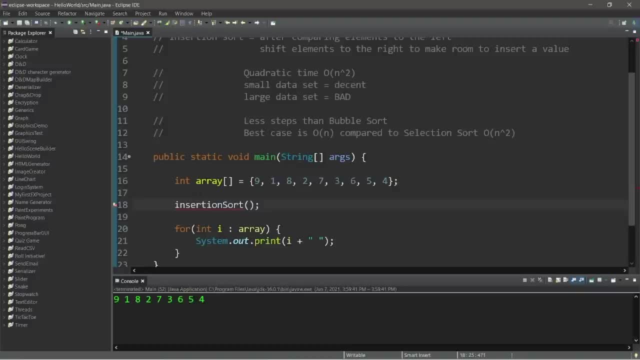 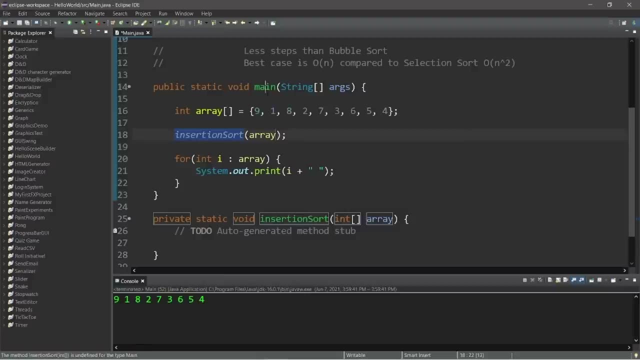 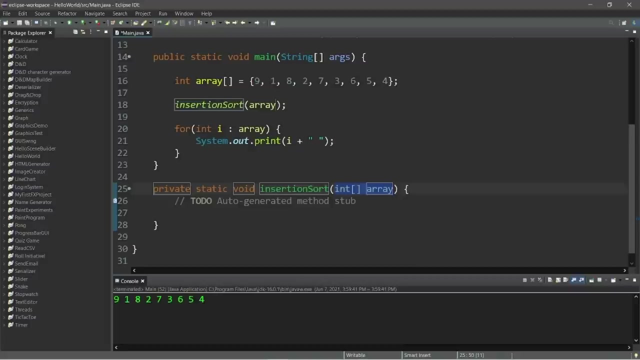 insertion sort. Then we will pass in our array as an argument and we'll need to declare this. So I'm going to cheat and create this automatically. So, outside of our main method, create a method named insertion sort- Private static void insertion sort. There is one parameter and array of integers. Okay, 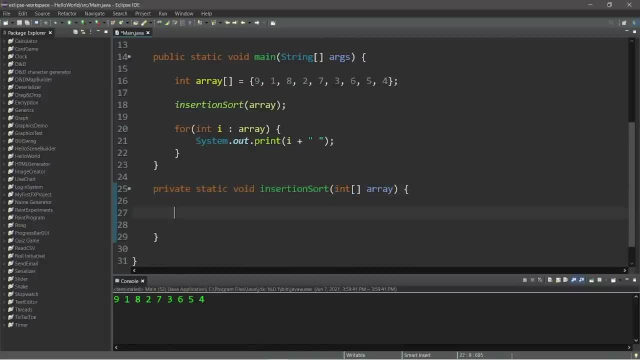 now the first thing we'll do is create a for loop to iterate over each element of our array, but it begins at one, not zero. So that would be for. then we will set int i equal one, not zero. Pay attention to that. We will continue this as long as i is less than. 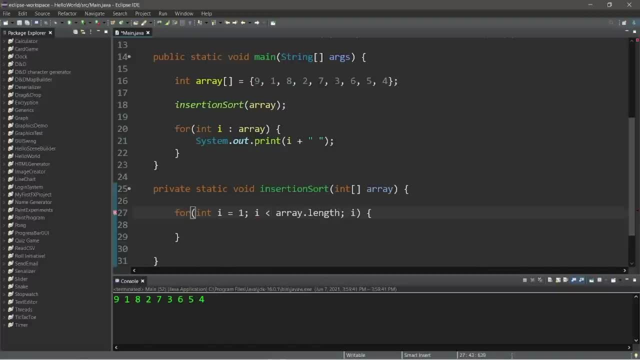 array dot length, And we will increment i by one during each iteration. Now we need to take our value found within i and place it within temp. So let's declare a temporary variable named temp. int. temp equals array at index of i, And now we'll create a variable named 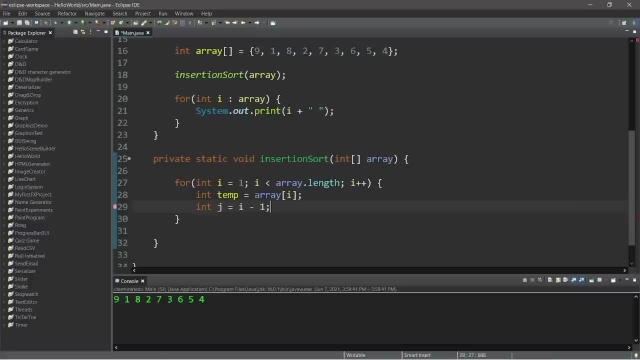 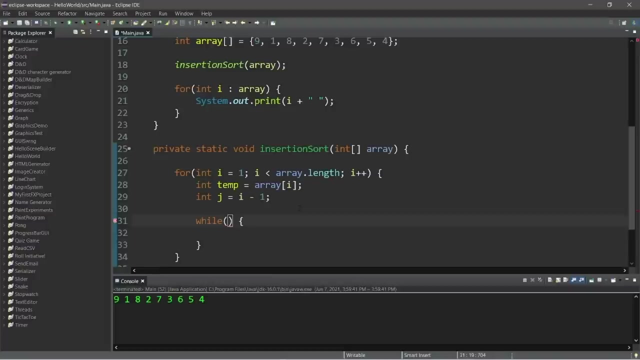 j Int. j equals i minus one, So this will keep track of what value we're comparing to the left of whatever i is. So, then, we need to create a while loop. We will continue comparing values to the left of i, And our condition is going to be: while j is greater than or equal to zero and array. 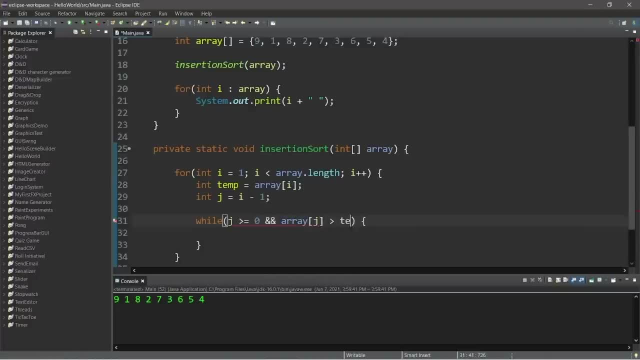 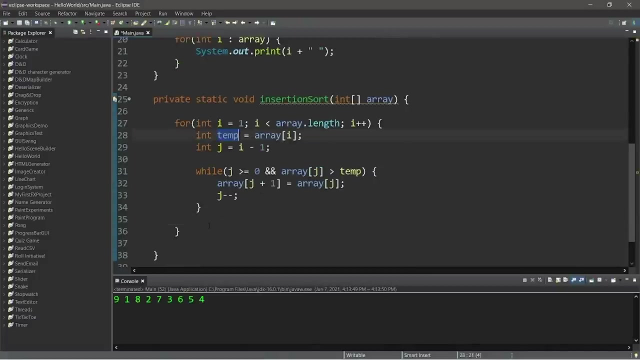 at index of j is greater than temp. So if we need to shift an element to the right, we would say array at index of j plus one equals array at index of j. So that will shift an element to the right. Then we will decrement j by one, j minus minus, And the last thing to do is to insert the value. 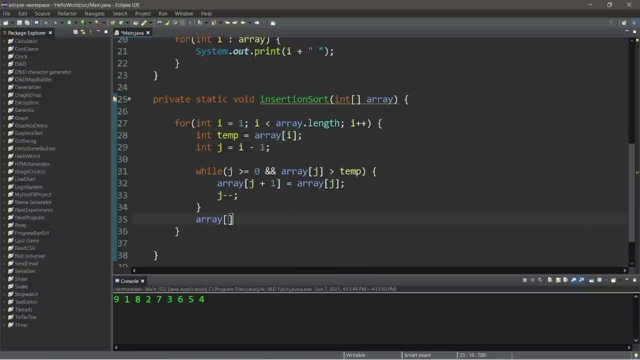 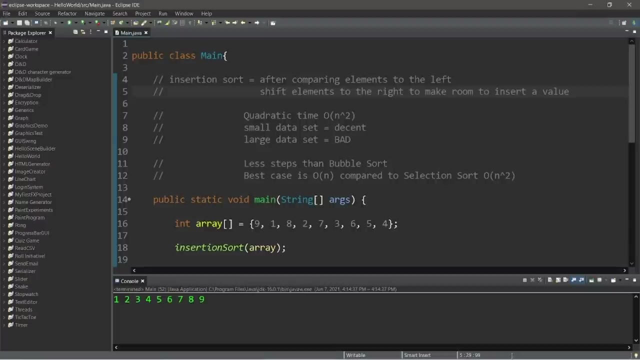 found within temp into that opening. So that would be array at index of j plus one equals temp And that's all there is to it. So let's run this booyah: one, two, three, four, five, six, seven, eight, nine. Well, people. in conclusion, the insertion sort algorithm compares: 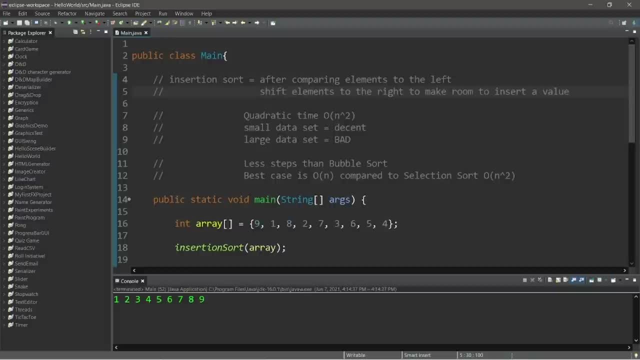 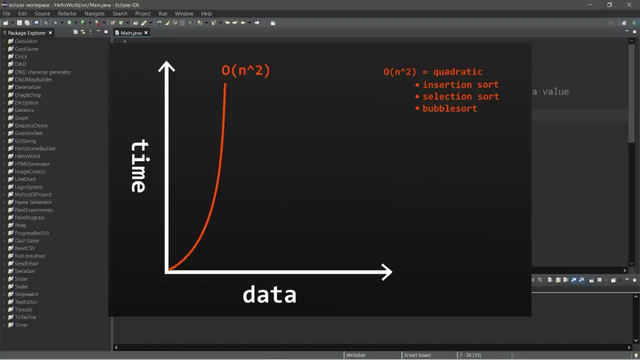 elements to the left and it will shift elements to the right to make room to insert a value. the insertion sort algorithm has a runtime complexity of big O of n squared. It runs in quadratic time. It's decent with small data sets but bad with. 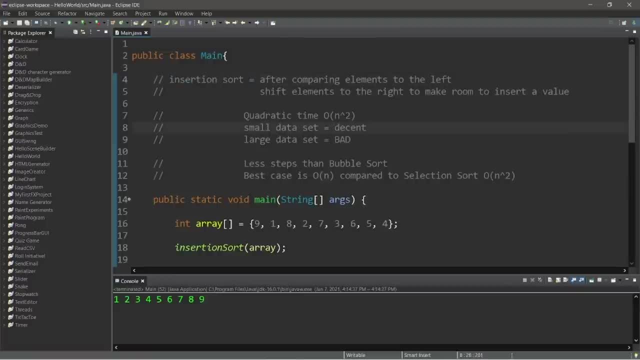 large data sets And using insertion sort tends to be preferable to both bubble sort and selection sort. It uses less steps than bubble sort and, in the best case scenario, insertion sort can run in O of n linear time, compared to selection sort, which the best case scenario is O of n squared. 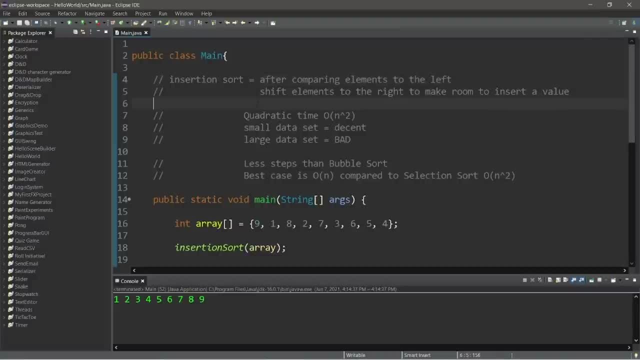 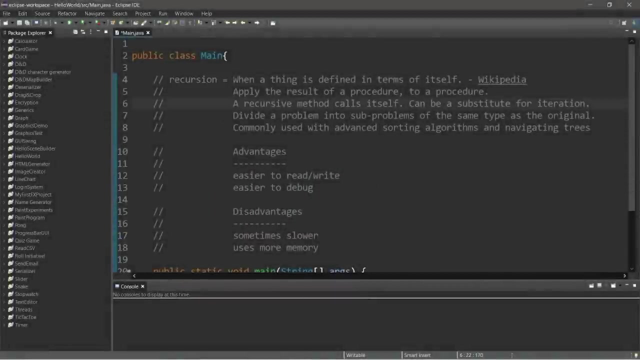 All right people. so that is the insertion sort algorithm. If you can destroy that like button, leave a random comment down below, and well yeah, that's the insertion sort algorithm in computer science. Well, howdy y'all. We're talking about recursion. Now recursion is when. 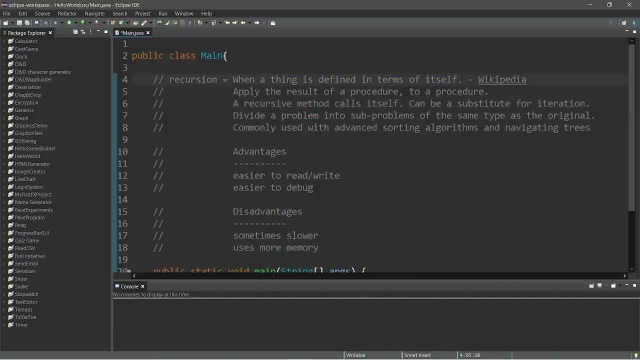 a thing is defined in terms of itself. I stole that definition from Wikipedia. Really doesn't make too much sense. A thing is defined in terms of itself. So basically, with recursion we apply the result of a procedure to a procedure. A recursive method is one that calls itself. 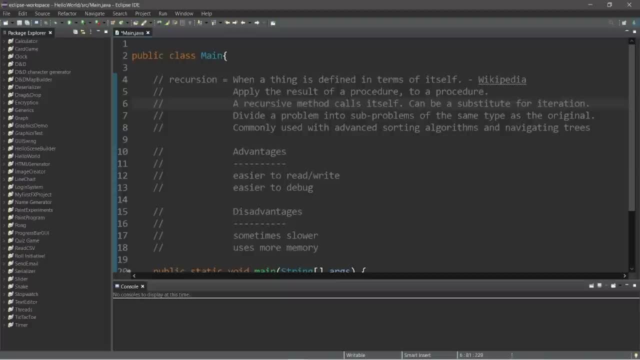 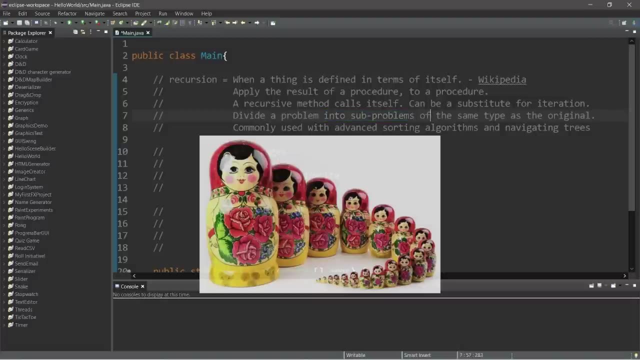 and this can be a substitute for iteration. There's a lot of overlap where you could use either recursion or iteration. With recursion, we divide a problem into sub-problems of the same type as the original, and recursion tends to be used within advanced sorting algorithms and 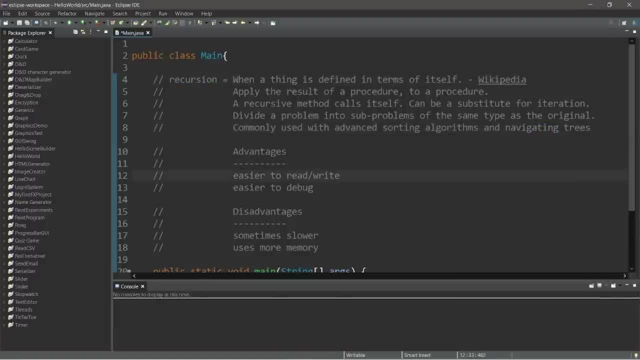 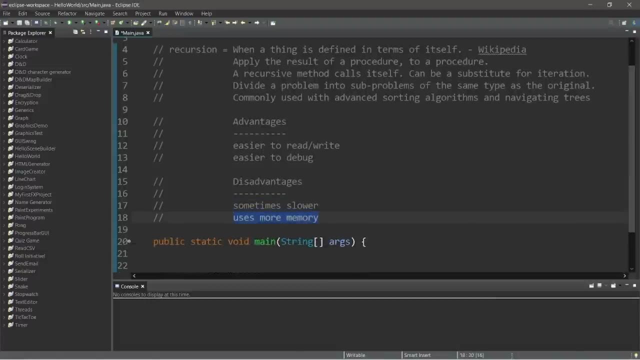 navigating trees. Some of the benefits of recursive code is that it's easier to read and write and it's easier to debug, But the disadvantages is that it's sometimes slower and uses more memory. Let's begin with a very simple example. Let's create a method to simulate walking. We'll do this both iteratively. 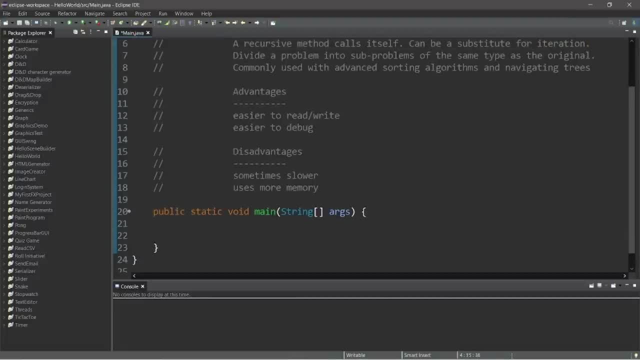 and recursively then take a look at the differences between the two. So let's write an iterative walk method. So we will need to invoke this method and then we will pass in the amount of steps that we would like to walk, like five steps, And then we'll need to declare: 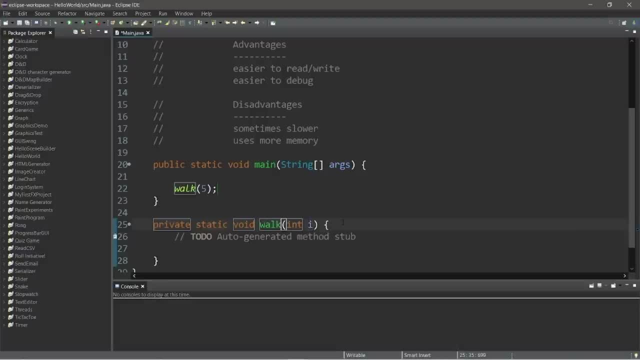 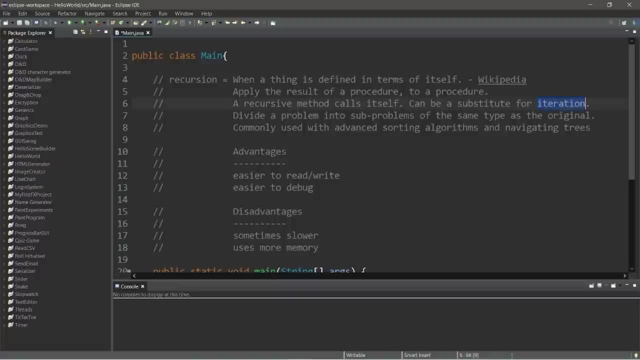 this method, Private static void walk- and I'll change i to maybe Maybe steps, just so that it's more descriptive. Now let's use an iterative approach. So iteration is the repetition of an internal process. So we can use a for loop That will repeat. 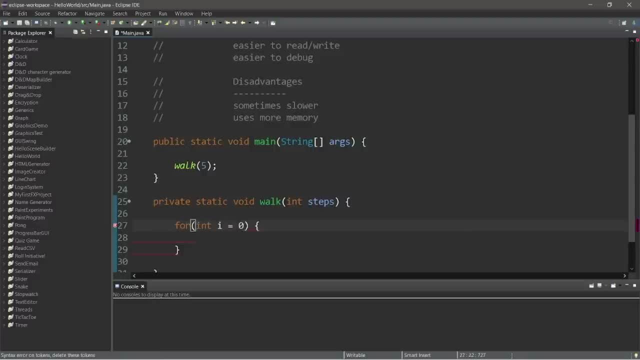 a process, And let's say that int i equals zero. We will continue this as long as i is less than steps, And then let's increment i by one during each iteration And then during each iteration, I will print: you take a step And really that's it. 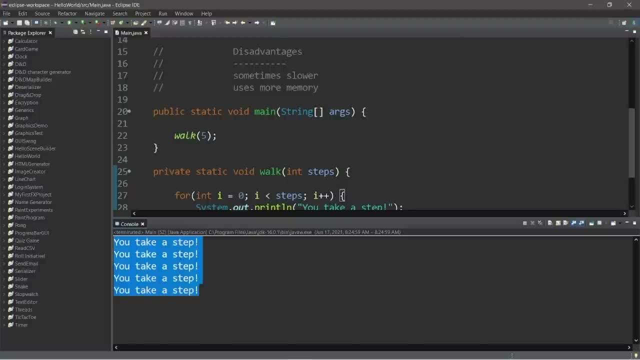 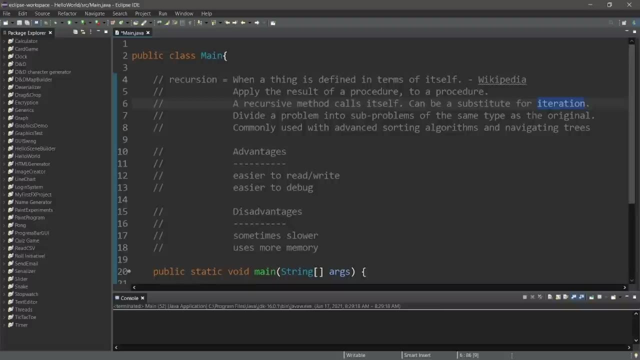 And after running this code, we have walked five steps. Now let's write the same method recursively. Recursion is the repetition of a procedure. Iteration is the repetition of a process. So with recursion we need a base case. That's what we do when we would like. 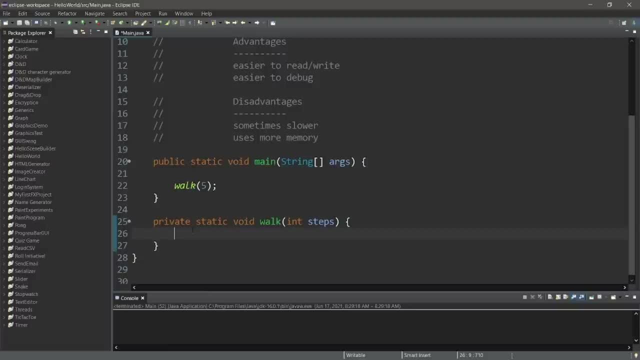 to stop And a recursive case. what do we do when we would like to continue? So our base case is going to be: if steps is less than one, then we will return, And if you have one statement within your if statement, you don't really need these curly braces. 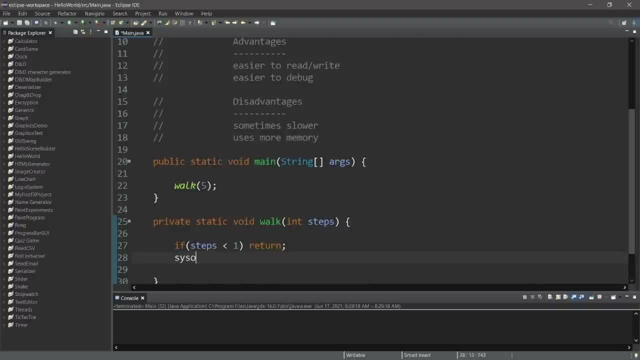 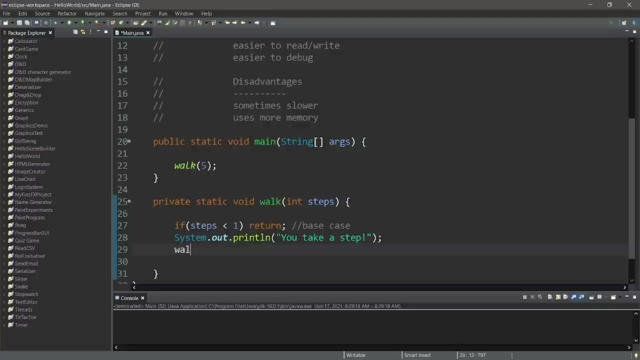 So I'm just going to omit those. All right, Then we will print. you take a step. So this is our base case. This is what we do when we would like to stop. Then our recursive case is what we're going to do. when we would like to continue, We will invoke the walk. 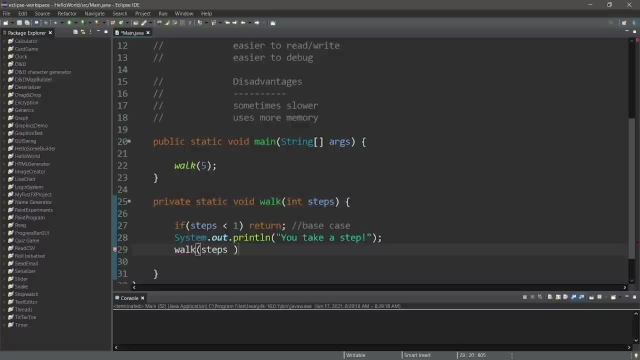 method within itself, But we will pass in steps minus one, And this is our recursive case, And this will do the same thing. However, it's just written a little bit different. Now, one thing that you should know is that programs have 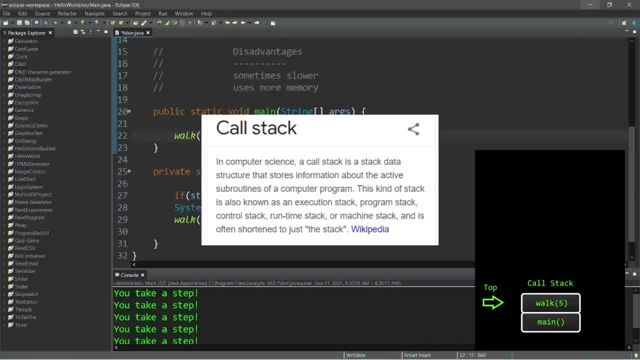 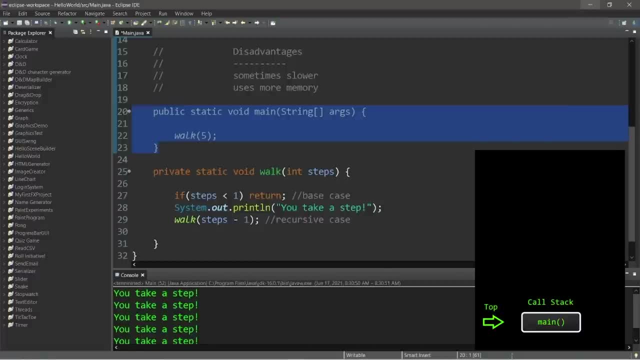 a data structure called a call stack. A call stack keeps track of the order in which our program needs to function. So with the main method, we call the main method first And that's added to the bottom of our call stack. So in order to complete our program, we have 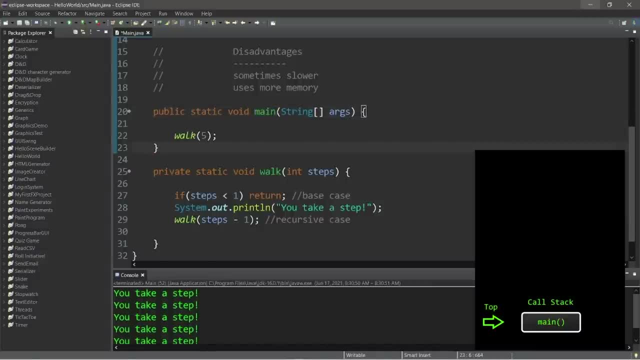 to complete the main method and get to the end of it. However, when we took an iterative approach, we invoked the walk method And that was added to the top of our stack. Remember that video on stacks. It's a LIFO data structure. Last, 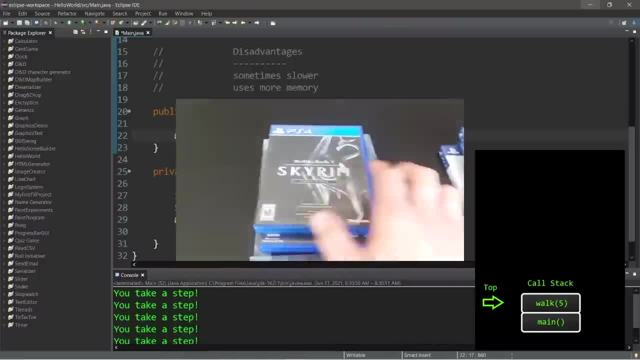 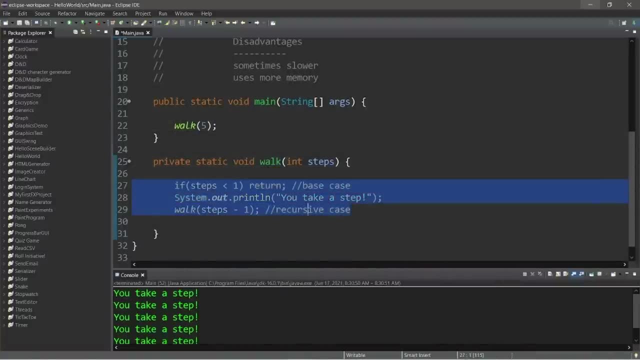 in first out. We have to take care of anything at the top of our stack first and then work our way down With a recursive approach. we're adding multiple frames onto our call stack, because one we're calling the main method, Then we're calling the walk method passing. 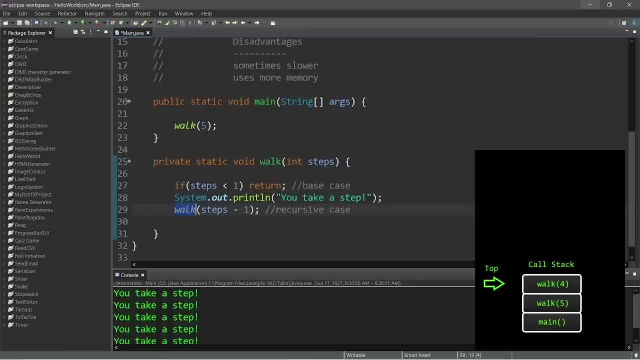 in five as an argument, Then we're calling the walk method again, Then passing in four as an argument, Then three, Then two, Then one, Then zero, Then we return, And we have to solve this in a LIFO order. Last in, first out, We begin at: 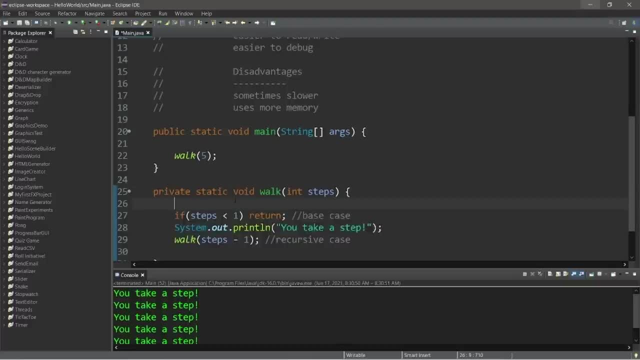 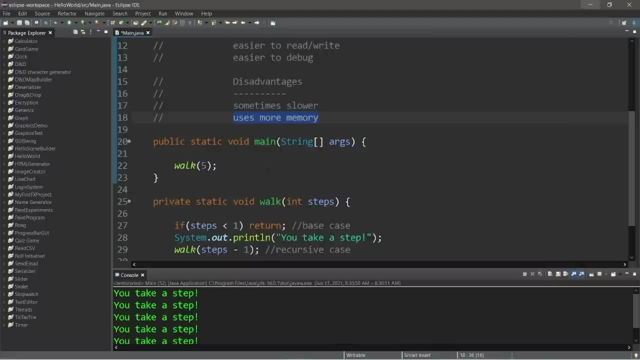 the top and remove frames from the top until we reach the end. So that's why using recursion is sometimes slower and uses more memory. We're adding more frames to the call stack. There's more methods that we have to keep track of. Now check this out. What if we take 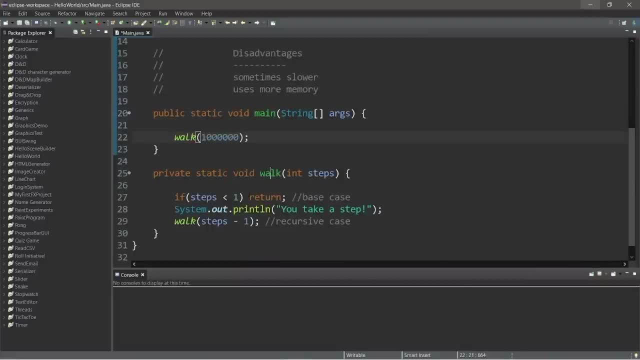 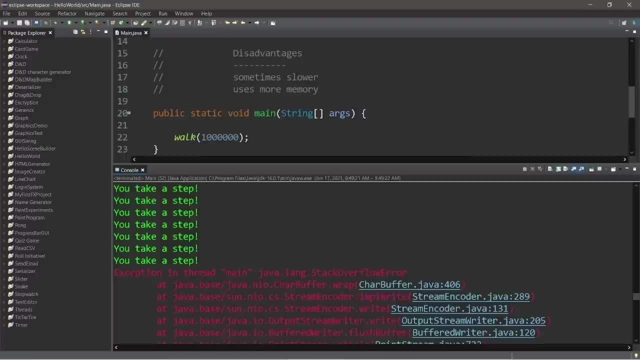 one million recursive steps. We're going to call this walk method a million times And that's going to be a problem. And we ran into an exception. Let's take a look at this. So we encountered an exception, a stack overflow error. It's kind of like that: one website. 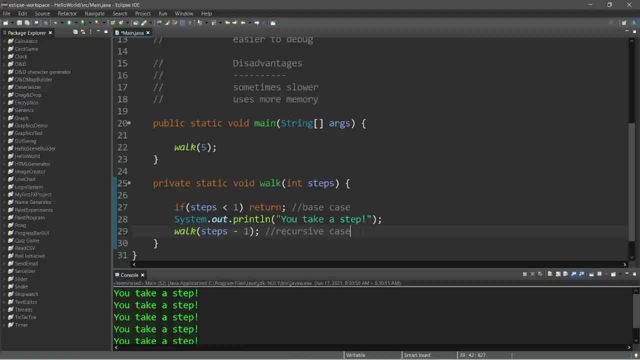 When working with recursion, it is possible to run out of memory, Although this is sometimes slower and uses more memory. recursive code tends to be easier to read and write and easier to debug. For a small method like this, I would probably stick with an iterative approach. 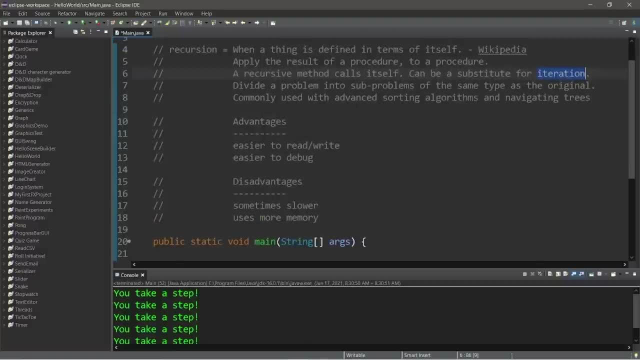 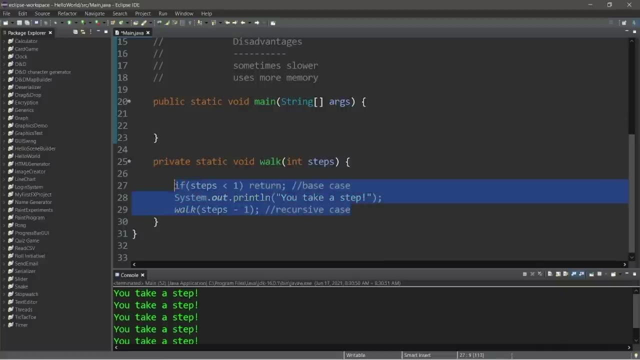 just because it already is fairly simple. But it's going to really come in handy when we get to topics on advanced sorting algorithms. So let's try something a little more complex. Let's create a program to find the factorial of a number. So let's create a factorial method. 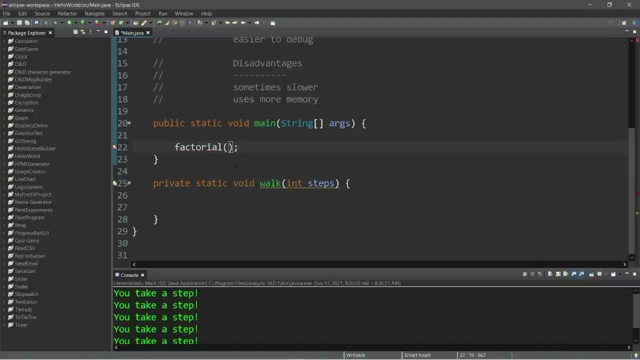 And we'll write this recursively. So let's find factorial. what about seven? and then we'll need to define this method And we no longer need our walk method. So if we're taking a recursive approach, finding the factorial of a number, let's say that i is num, So we'll 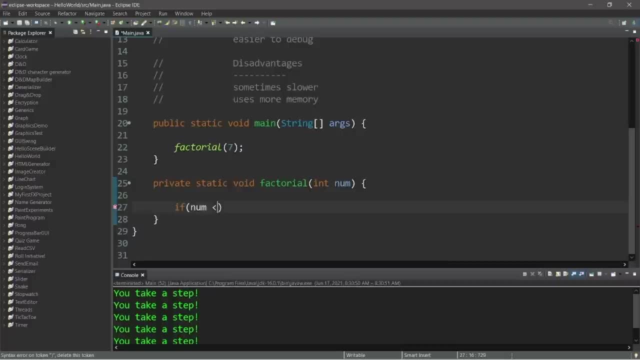 need a base case. If num is less than 1, we will return 1.. This is our base case. Then we need a recursive case. We will return num times factorial, then pass in num minus 1, and then eventually we'll hit. 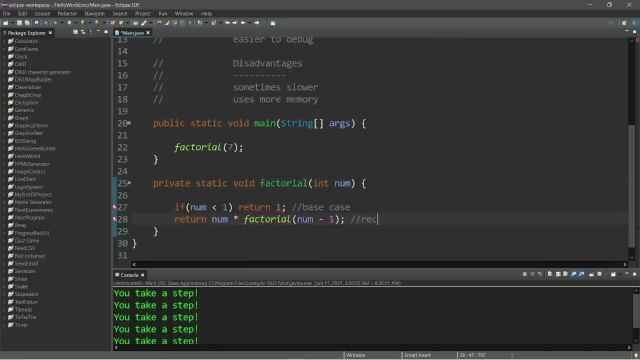 our base case, because num is going to be 0. And this is our recursive case. Oh, then change void to int, because I forgot. Okay, then let's display factorial 7 within a println statement, Factorial 7.. And the factorial of 7 is 5040.. So you can see that this was fairly easy to write. 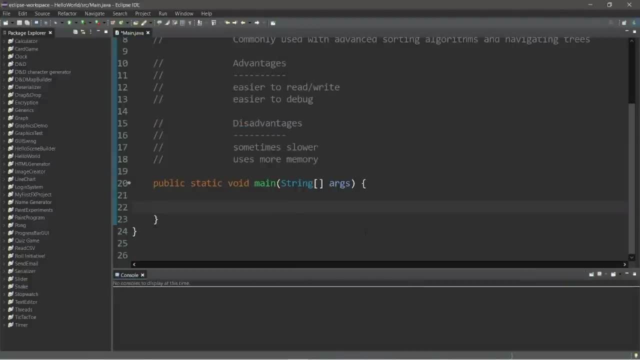 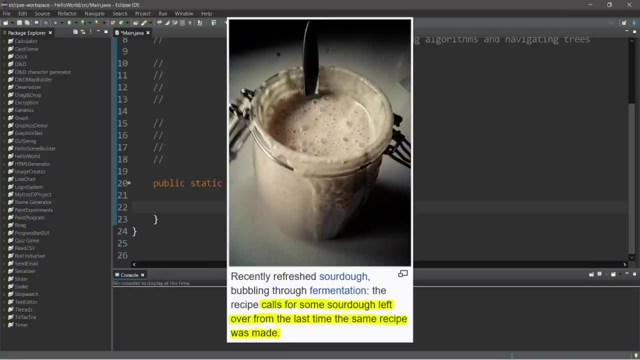 It only took two lines of code. By the way, I found a great example of recursion on its Wikipedia page, and that's by the process of creating refreshed sourdough. So the recipe calls for some sourdough left over from the last time the same recipe was made. I thought that was a fairly 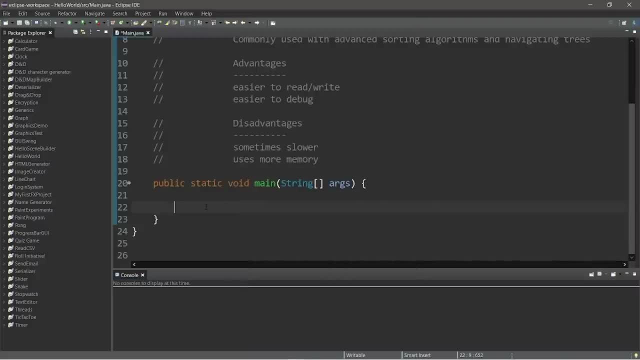 descriptive example of recursion. Let's move on to level 3.. Let's create a recursive method to find a base raised to a given power. Let's create a power method and we need a base and an exponent. Let's find 2 to the power of 8, and then we'll need to define this method: Private, static, Let's. 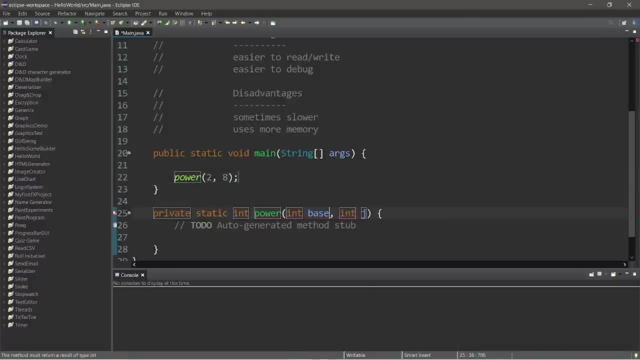 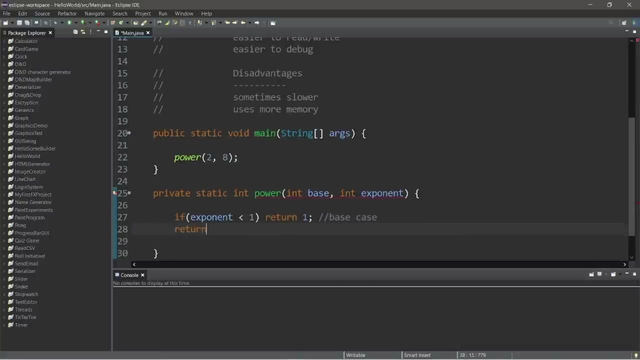 change void to int. i to base and j to exponent. We need a base case and a recursive case. The base case will be: if exponent is less than 1, we will return 1.. This is our base case. Our recursive case will be return. 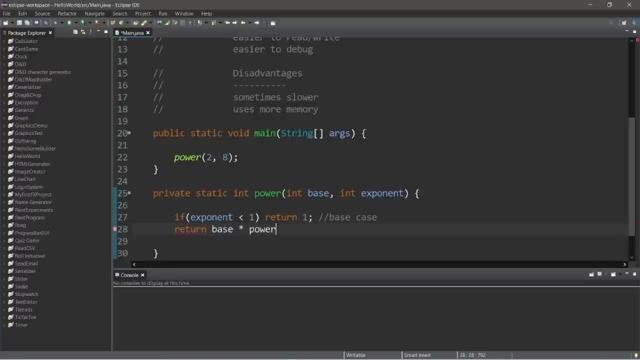 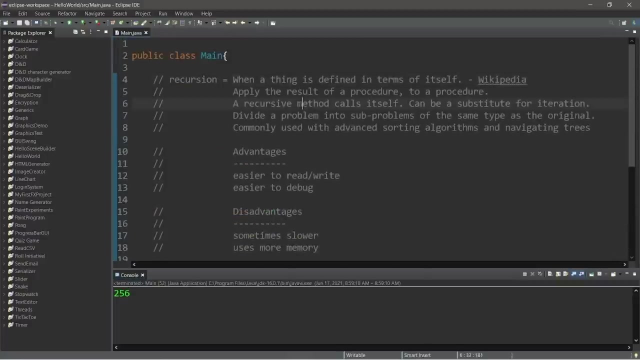 base times. invoke the power method, And then we will need to display the result Systemoutprintln 2 to the power of 8, which is 256.. All right, everybody. so that's recursion. It's when a thing is defined in terms of itself. 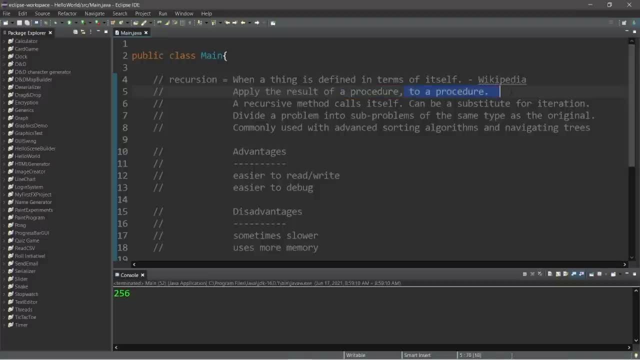 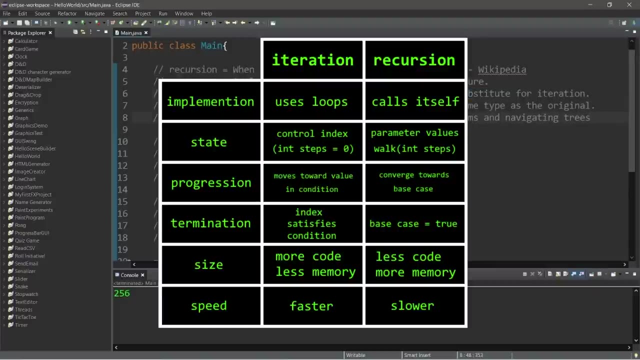 We apply the result Procedure to a procedure and a recursive method is one that calls itself, And this can be a substitute for iteration. We divide a problem into subproblems of the same type as the original, and recursion is commonly used within advanced sorting algorithms and navigating trees. Some of the advantages is: 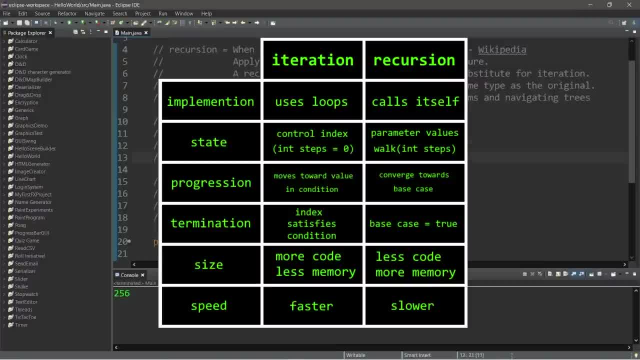 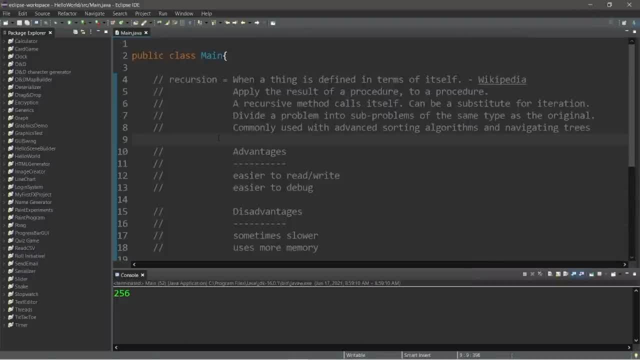 that recursive code is easier to read and write and easier to debug. However, it's sometimes slower and uses more memory. So, yeah, that is recursion. If you learned something new, be sure to smash that like button. Leave a random comment down below. 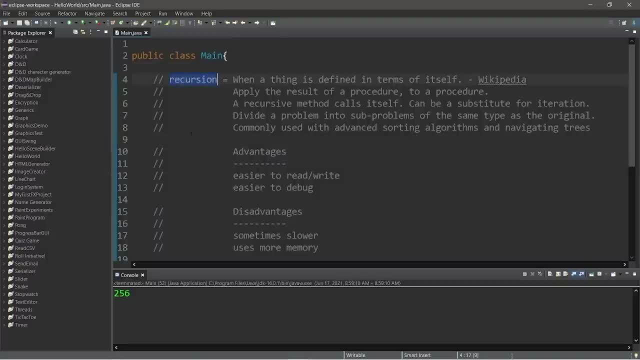 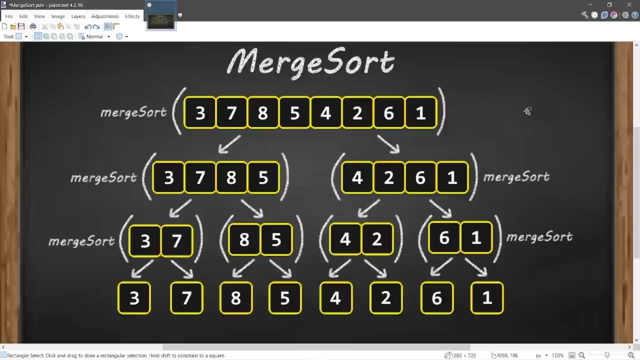 And well, yeah, that's recursion in computer science. Hey, what's going on? everybody, It's your bro, Hope you're doing well, And in this video we're going to discuss the merge sort algorithm and computer science. So sit back, relax and enjoy. 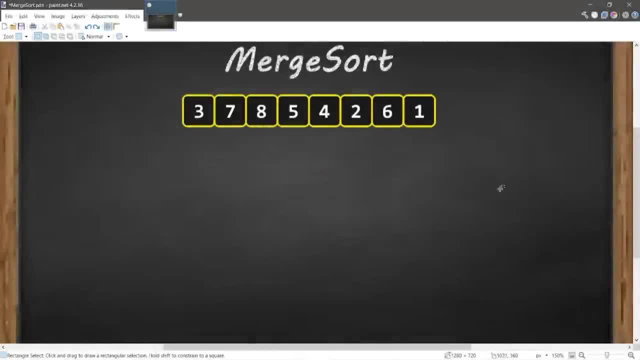 the show. All right, what's going on? people merge sort. merge sort is a divide and conquer algorithm. Basically, what we do is that we will pass an array as an argument To a merge sort function. this function is going to divide our array into. we have a left array. 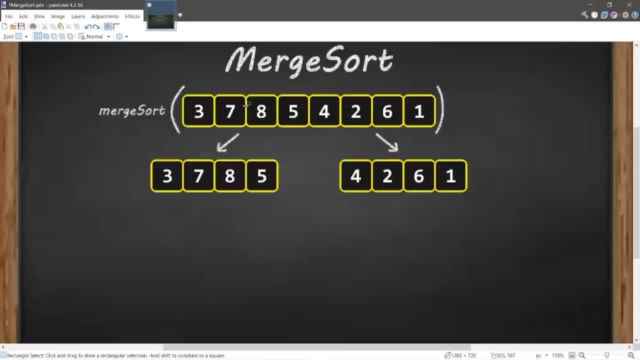 and a right array. these will be sub arrays and we will copy the elements over from our original array to our two new sub arrays. And merge sort is a recursive function, So at the end of merge sort we will call merge sort again and pass in our sub arrays that we create And again the merge sort. 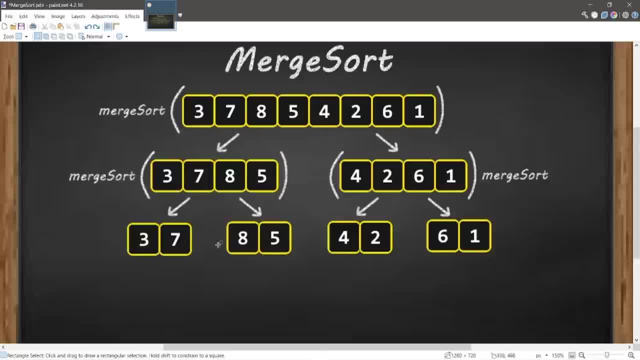 function is going to divide our arrays into by creating a two new sub arrays and then copy the elements over. And we will stop when our arrays only have a size of one, And that's where sorting, then merging, come in, And with the process of merging and sorting we will create a second. 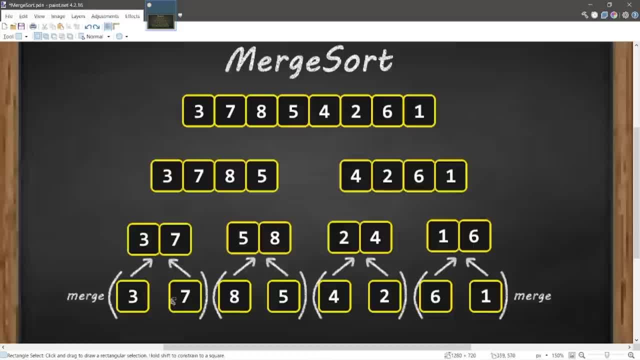 helper function named merge. merge will accept a total of three arguments: our left sub array, our right sub array and the original sub array in which these elements came from. Merge is going to take these elements and put them back into their original array in which they came from, in order. 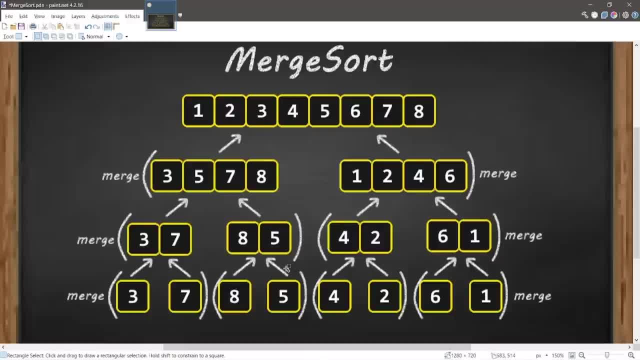 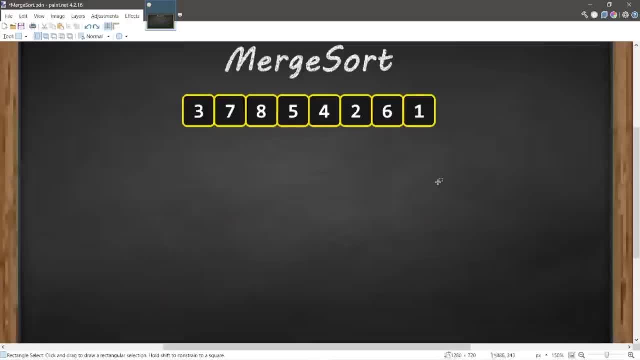 And we will do the same thing here, And we will do the same thing here, And we will do the same thing with the next grouping of arrays until all of these elements are merged back into their original array in which they came from, all in order. Now, in practice, when we do execute this merge sort, 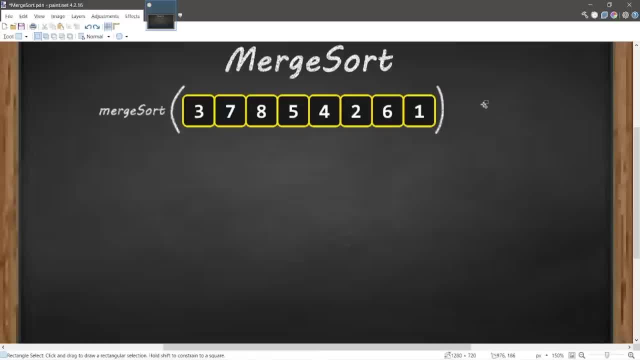 function. instead of tackling all of these sub arrays like one layer at a time, we will tackle them by one branch at a time. So it's going to look a little something like this, where we will start with the leftmost branch and then work our way towards the right. So I'll speed up the 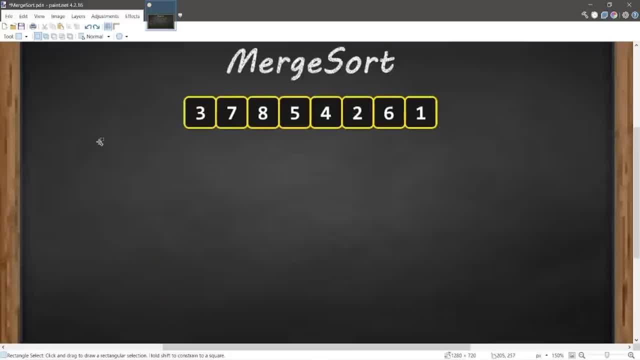 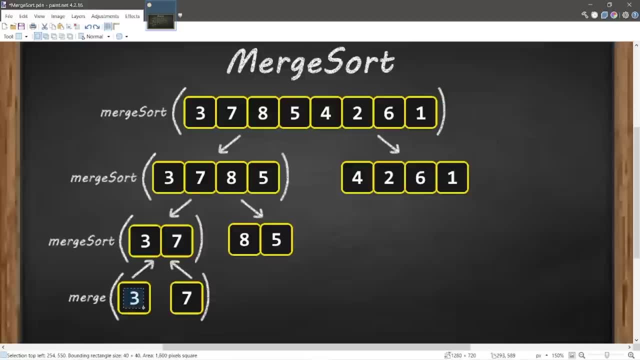 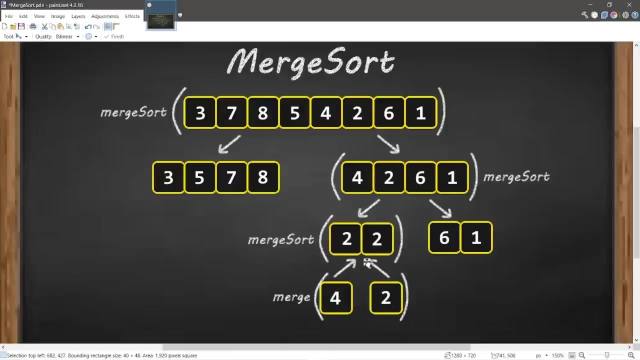 footage and just give you a rundown of what we're going to be doing here, And then we're going to speed up the footage and just give you a rundown of how this works in practice. So here we go, Thank you, Thank you. 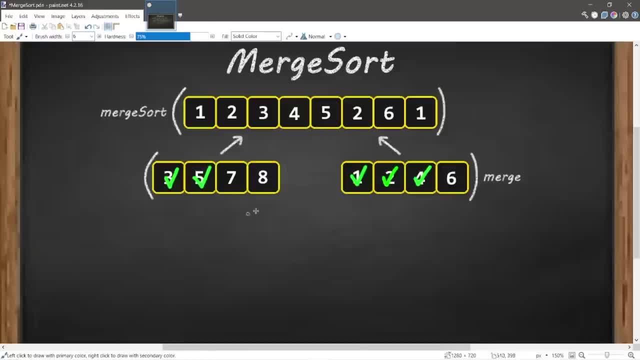 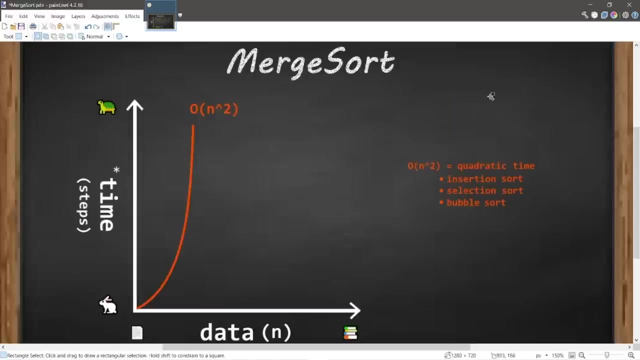 And that, ladies and gentlemen, is the MergeSort algorithm. The MergeSort algorithm has a runtime complexity of big O, of n log n. It runs in quasi-linear time, along with QuickSort and Heapsort, which we still need to talk about. 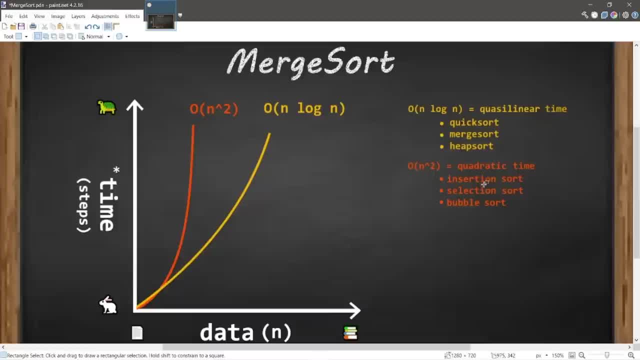 So when working with large datasets, MergeSort is faster than InsertionSort, SelectionSort and BubbleSort. But on the other hand, the MergeSort algorithm uses more space than BubbleSort, SelectionSort and InsertionSort because we need to create new subarrays to store elements. 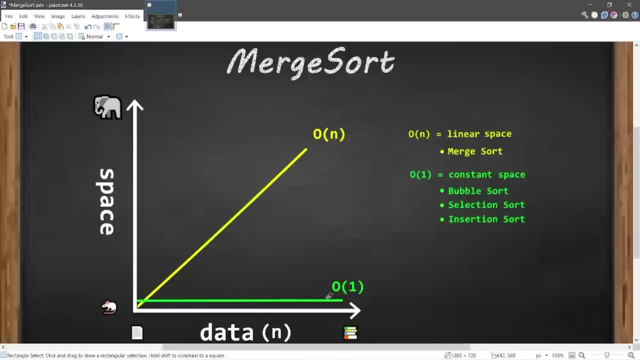 whereas BubbleSort, SelectionSort and InsertionSort can sort in place, so they use a constant amount of space to do their work, Unlike with MergeSort. Now let's move on to the hands-on portion of this video and create a MergeSort function in code. now 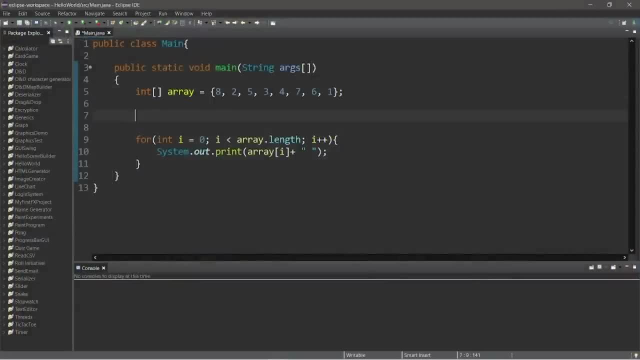 Alright, well, let's get started. We'll need an array to work with, make up some numbers, make sure that they're not in order, as well as a for loop to iterate over the elements of our array. So currently our array is not in order, but that's going to change soon. 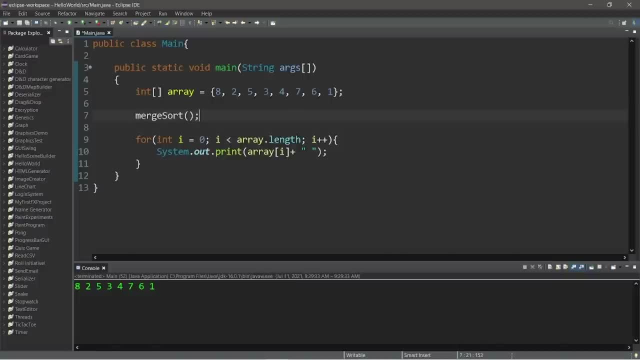 Let's invoke a MergeSort method that we still need to declare. This is going to be a recursive method and we will pass in an array, And each time that we invoke this method, we will split our array in half, create two subarrays and then copy the elements over. 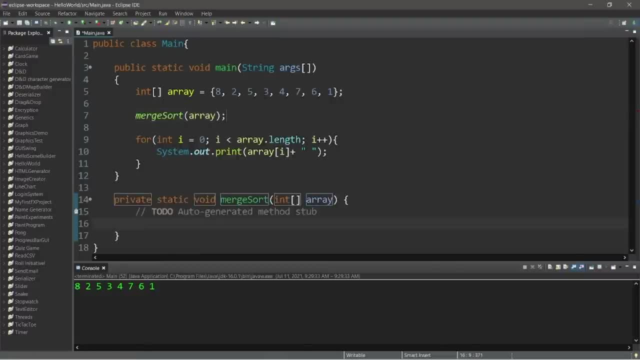 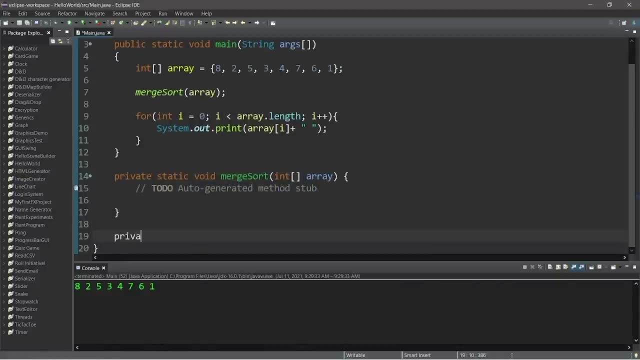 So let's create and declare this method Private static void MergeSort, and we'll need a helper method too, And we'll name this Merge. A helper method is just a method that helps another method, basically So private static void Merge. 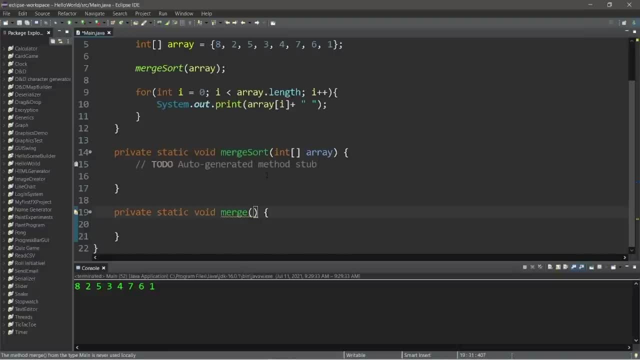 And there's going to be three parameters within our Merge method: Int leftArray, int rightArray and int array. Remember that these are arrays of integers. The first thing that we're going to do within our MergeSort method is that we need to get the length of our array. 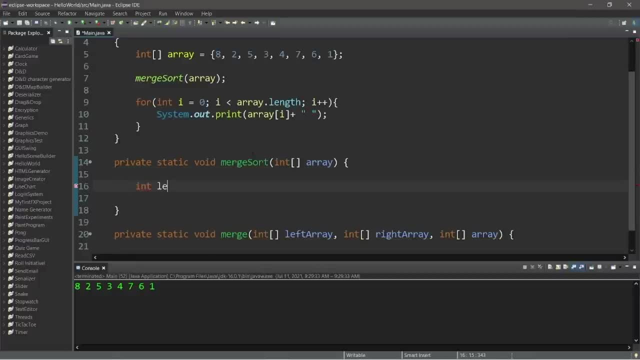 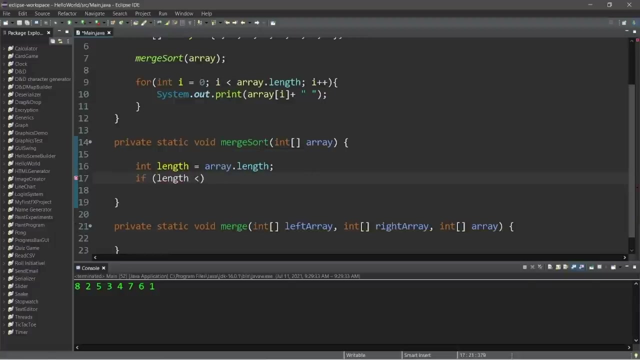 So let's cache that within a local variable named length. Int length equals arraylength, Int length equals arraylength, And we'll need a base case too. When do we stop recursion? If length is less than or equal to 1, then we shall return. 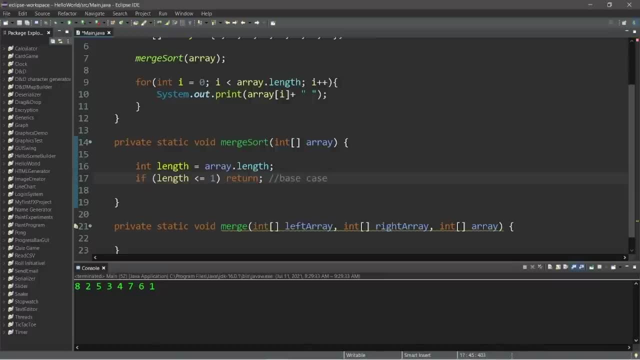 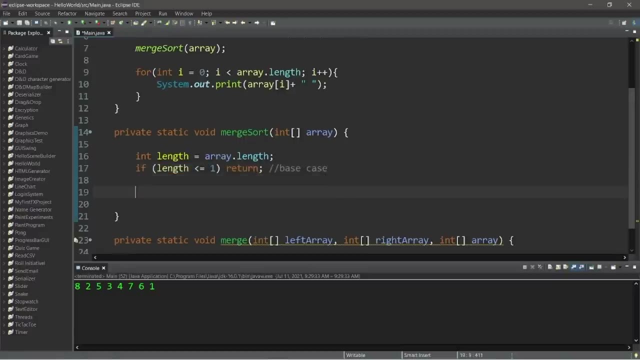 And this is our base case. Basically, with this MergeSort method, we're dividing our array in two each time. If the length is 1, there's no longer a need to divide our array further And we'll need to find the middle position of our array. 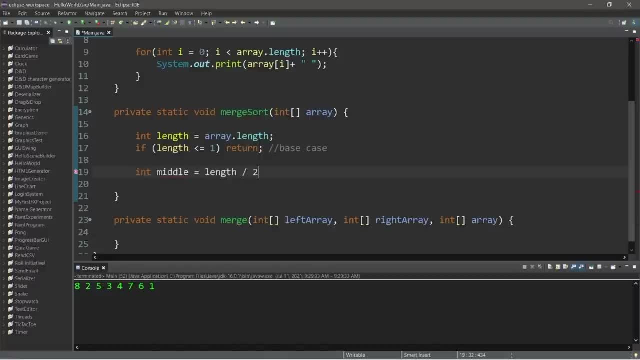 Int. middle equals length divided by 2.. And we'll create two new subarrays: Int array leftArray equals new integerArray And the size is middle. And we'll create a rightArray- IntegerArray- rightArray The size is length minus middle. 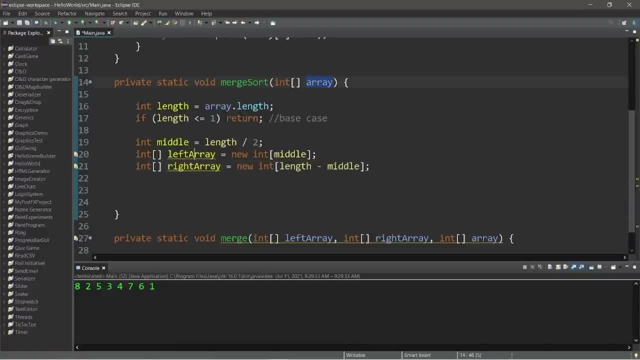 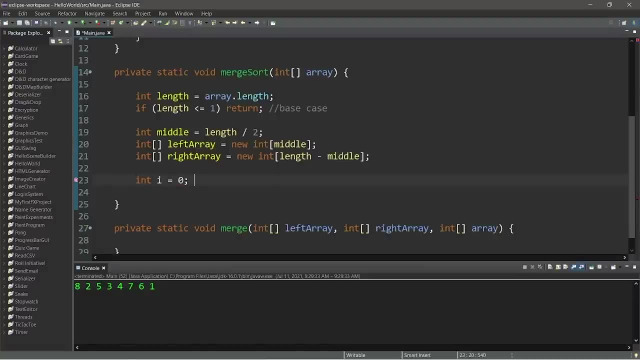 Okay, now we need to copy the elements of our original array to our left and right arrays, So we'll need two indices: Int i equals 0. This will be for our left array, And int j equals 0. And this is for our right array. 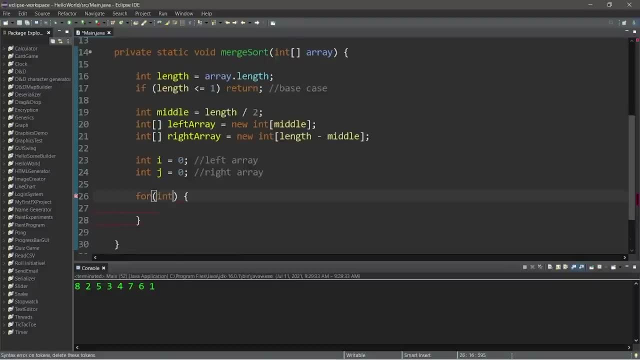 Then let's create a for loop. We don't necessarily need to declare a new index here, We can just use i. So I'm going to add a semicolon. Our condition is: i is less than Length, Then increment i by 1 during each iteration. 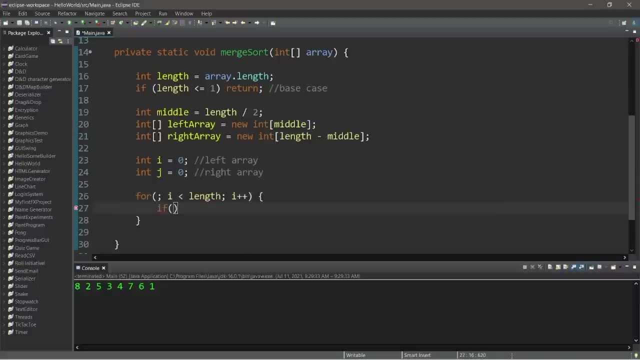 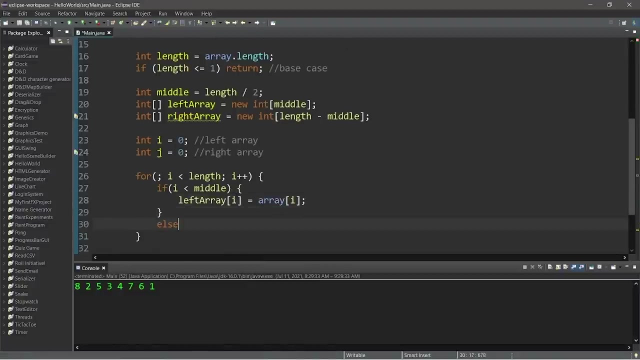 So our condition is, with an if statement, If i is less than middle, Then we will copy an element from our original array to our left array. Left array at index of i equals array at index of i, Else We will copy that element to our right array. 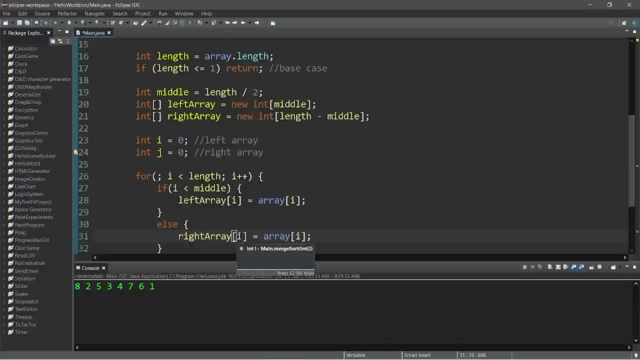 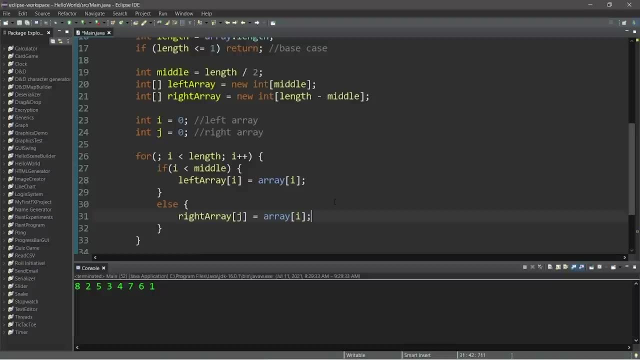 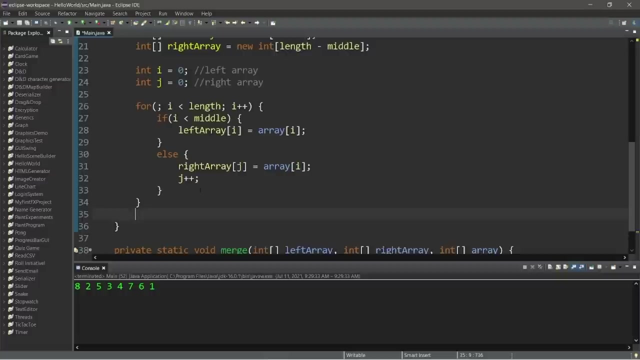 Else. Right array at index of j. Remember that this index is for the right array- Equals array at index of i. Then let's increment j by 1.. Okay, this is where recursion comes in, So outside of this for loop. 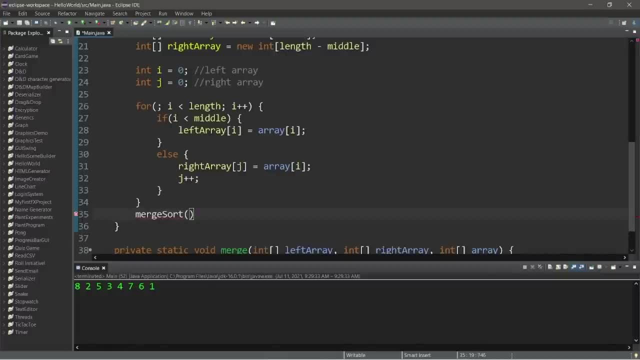 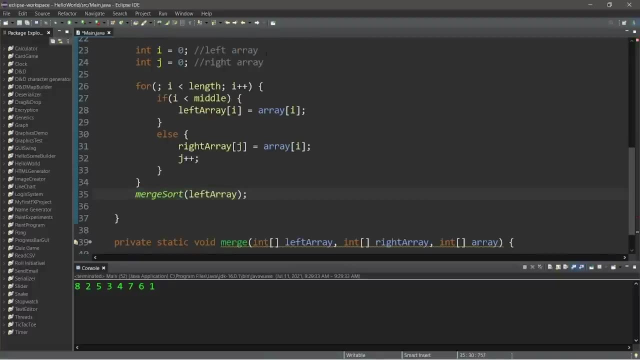 We will call merge, sort again And pass in our left array, So We'll consistently divide our array in half. We'll begin by dividing the left array, Then the right array With a separate recursive call. So left array, Then right array. 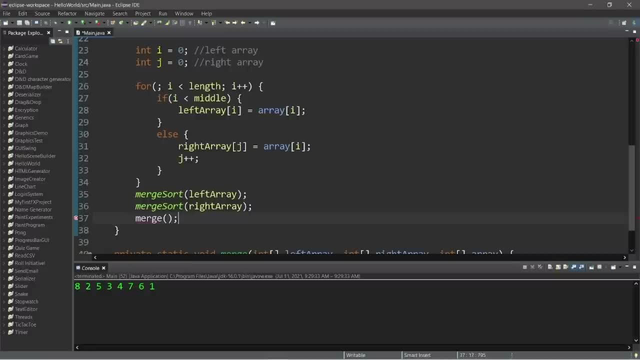 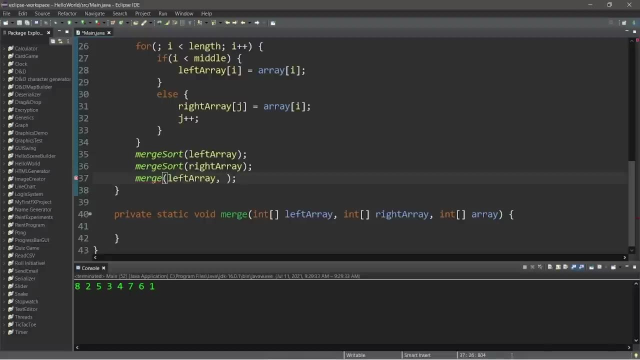 And then call merge. So with merge we have to pass in our left array, Right array And our original array, Because we'll put the elements back in order: Left array, Right array And our original array that we received as an argument. 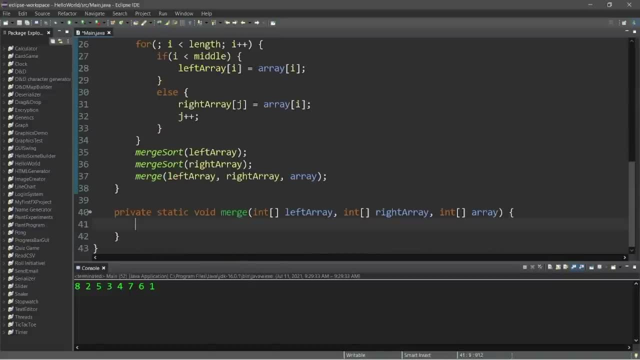 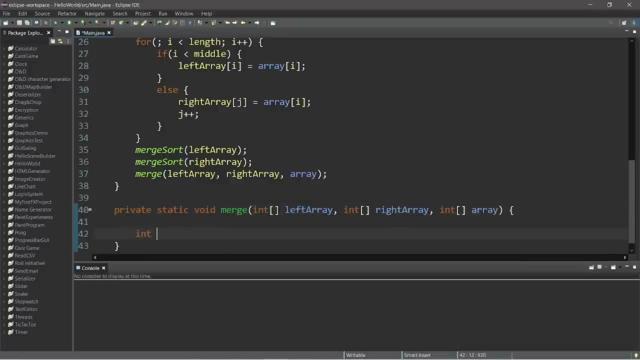 So that is it for the merge sort function. Let's work on a merge next. First thing that we're going to do within the merge method Is cache the size of our left array And right array within some local variables. Int. left size equals arraylength divided by 2.. 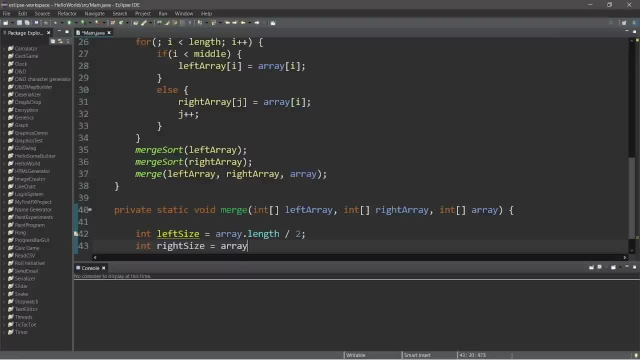 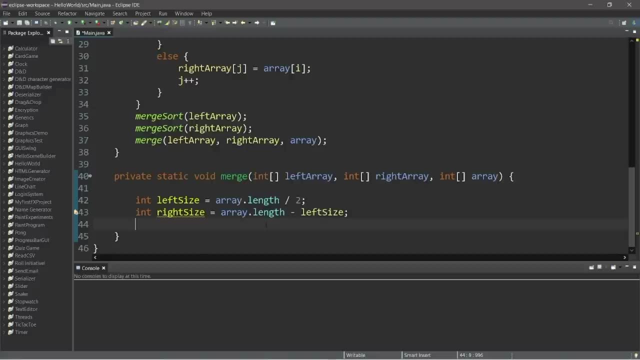 Int right size equals arraylength minus left size. And then we'll need three indices: Int i equals 0. This is for our original array To keep track of the position. L will be in charge of our left array And r will be in charge of our right array. 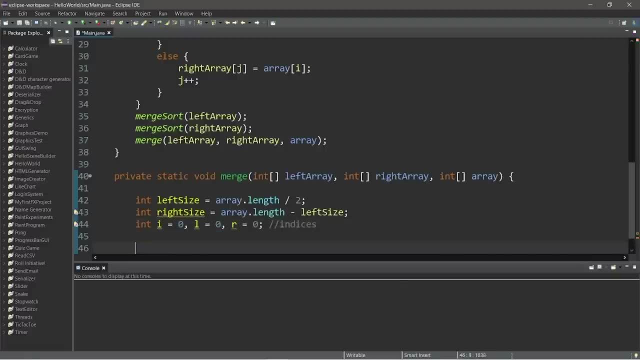 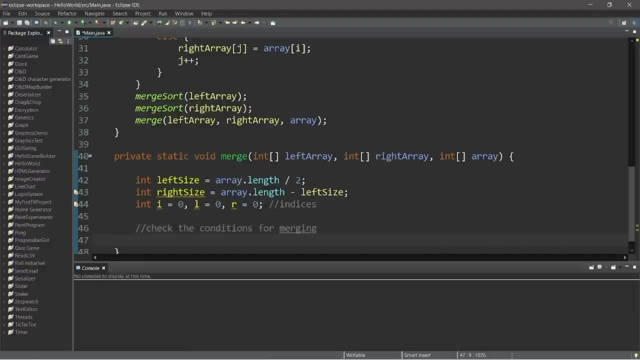 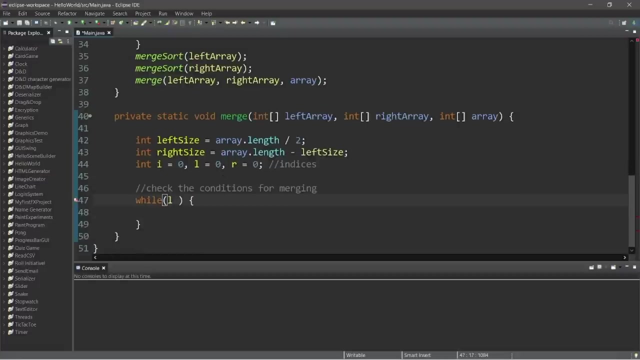 And these will be the indices that we're using. Okay, the next part. We're going to check the conditions for merging, And we can do this with a while loop. So our condition is going to be: While l is less than Less, 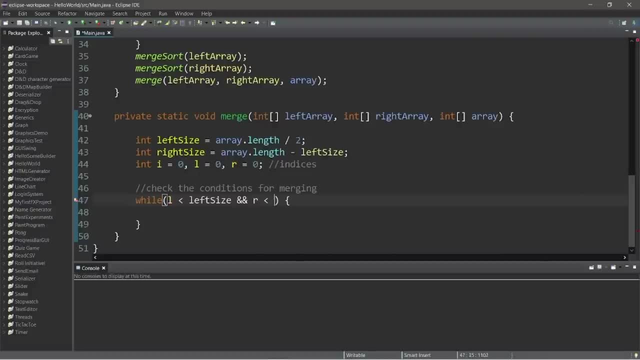 Size And r is less than Right size. So, basically, While there's elements within both our left array and right array, We will continue adding elements to our original array And we'll need to check to see which element is smaller If 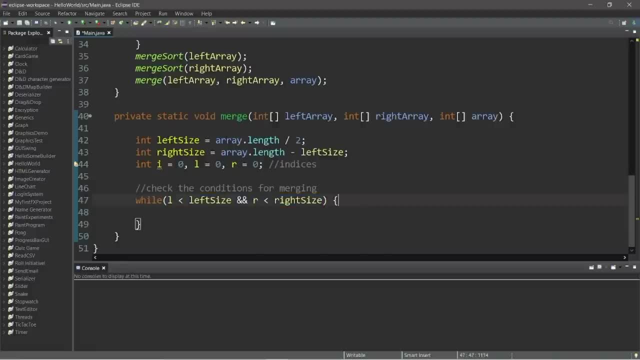 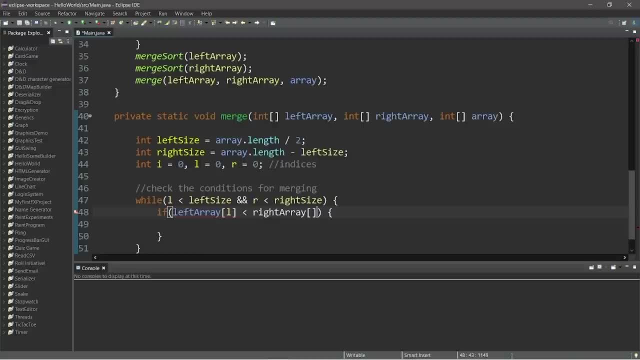 Is Less than Right array At index Of x Of r, Then we will copy the element From our left array To our original array, So basically comparing the number on the left To the right And adding whatever. 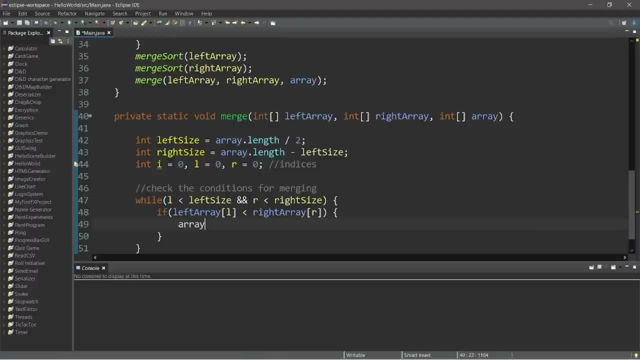 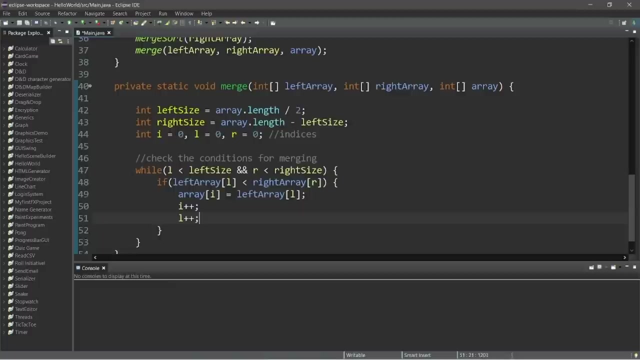 Number is smaller, Back to our original array. So array At index Of i, L Is, Or index Of i Is At index L, Then we can increment i And increment el. So if the number on the left is not smaller than the number on the right, we have to copy the element. 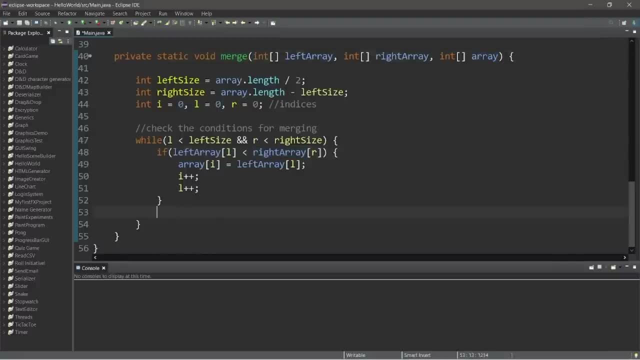 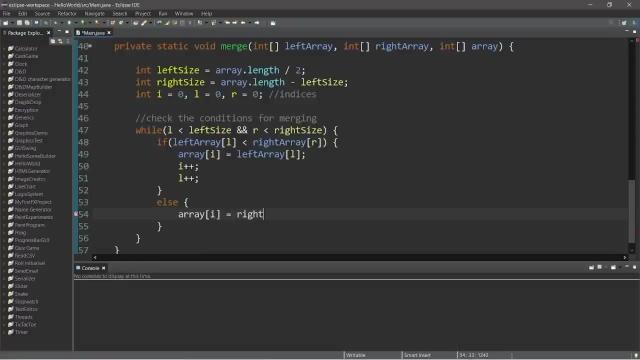 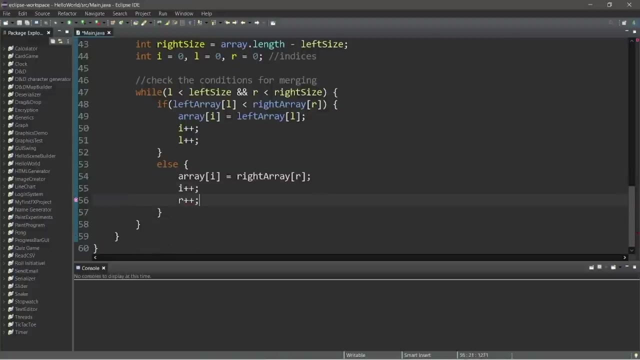 in our right array to our original array and we can use an else statement: Else array at index of i equals right array at index of r: Increment i increment r. So there's probably going to be one element remaining that we cannot compare to another element because there's only one left. 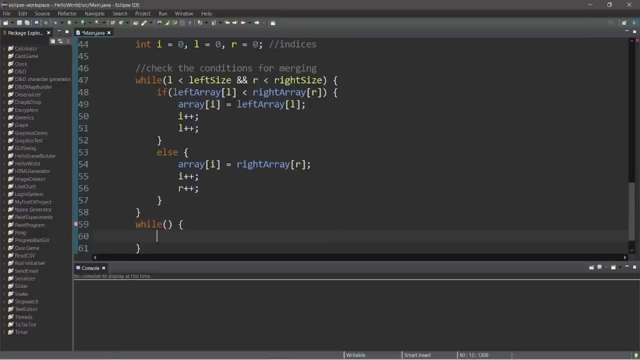 So let's write a while loop for that condition. While l is less than left size, then we will take array at index of i equals left array at index of l. Increment i increment l, Then we'll need another while loop If r is less than. 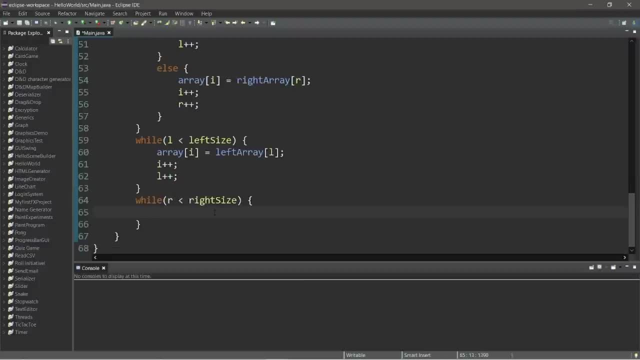 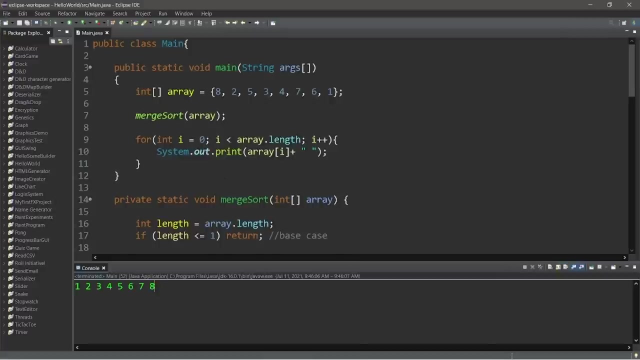 right size. we will copy the last right element over. Array at index of i equals right array at index of r. Increment i increment r, And that should be it. Let's run this And our array is now sorted. In conclusion, everybody, the merge sort algorithm recursively. 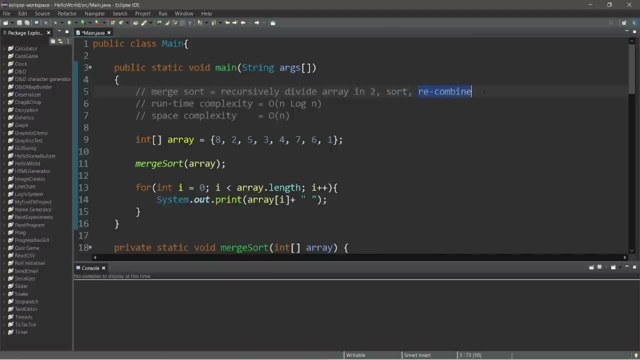 divides an array in two, Sorts them and then recombines them. The merge sort algorithm has a runtime complexity of big O of n, log n and a space complexity of big O of n. So that is the merge sort algorithm, If you. 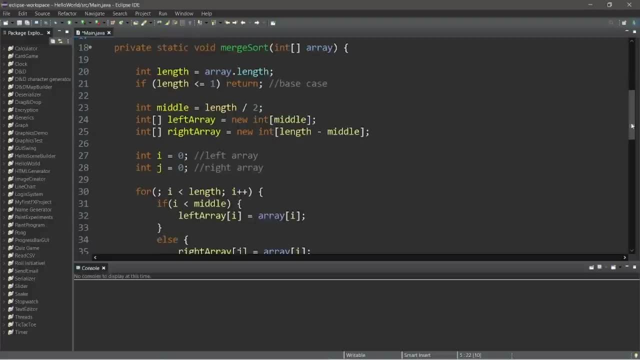 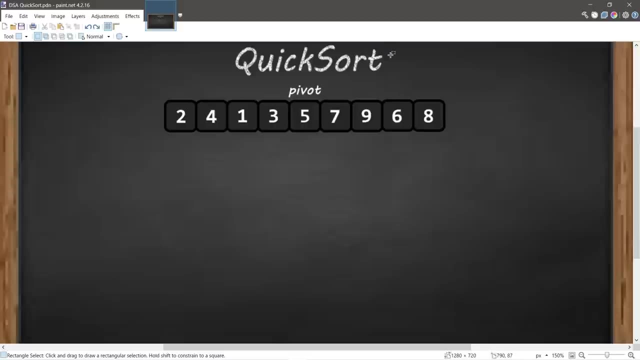 would like a copy of this code. I will post this to the comments section down below. And well, yeah, that is the merge sort algorithm in computer science. Hey, it's your bro, Hope you're doing well. And in this video I'm going to explain the quick sort algorithm in computer science. 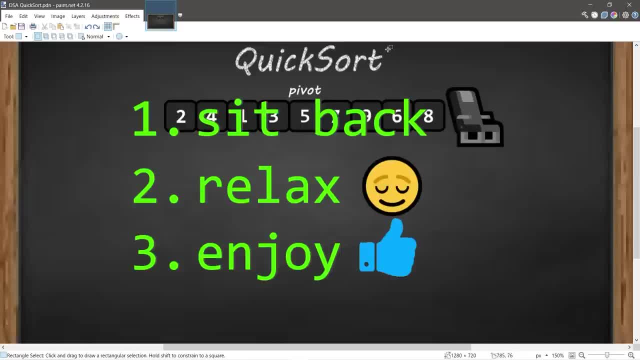 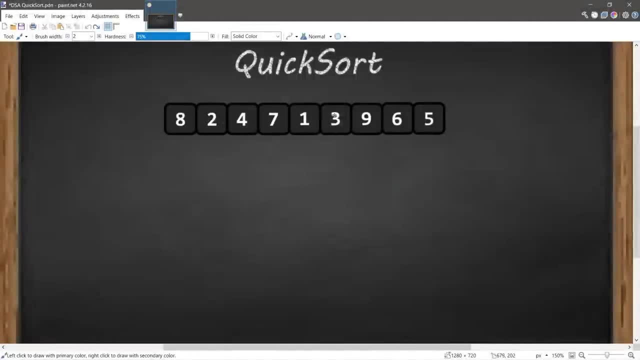 Yep, So sit back, relax and enjoy the show. All right, quick sort. Here's how quick sort is going to work. We need an array or some other type of collection. I have a simple, unordered array. What we do is that we'll pass our array. 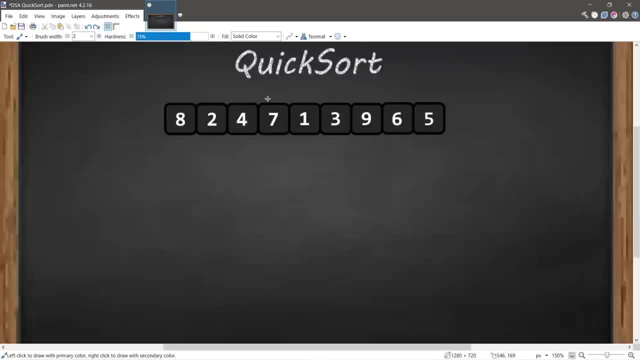 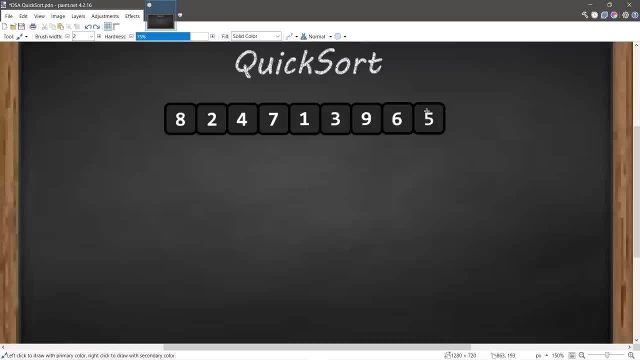 We can pick a pivot at the beginning, the middle or at the end, But with most standard quick sort algorithms we will set the pivot to be at the end of our array. What we're trying to accomplish is that we need to find the final resting place of our pivot. Where is this value going to be? 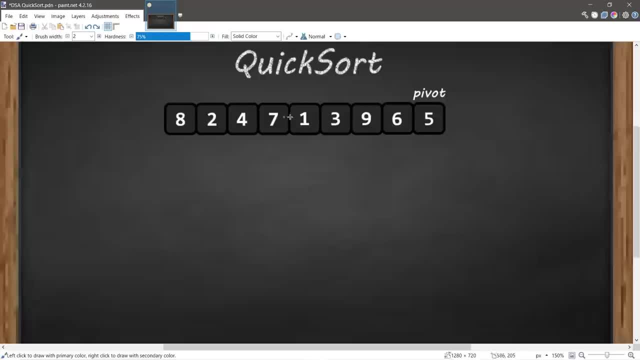 And taking a look at this, that would be right about here, But we don't know that yet. So, to find the final resting place of this value, our pivot, here's what we can do. We will declare and use two indices. 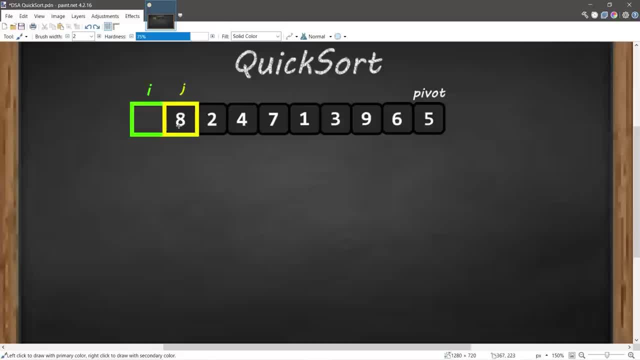 J and I. J will begin at the start of our array. I will be one less than the beginning of our array- And that's going to be important later- And we'll need the help of a temporary variable so we can swap some values. All we're doing is checking to see if the value at J is less than. 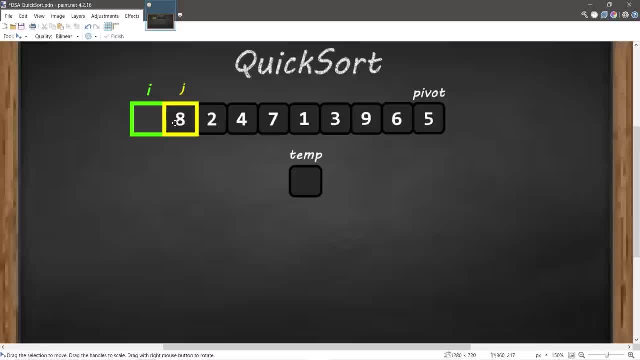 our pivot. If it's greater than our pivot or equal to our pivot, we ignore it. 8 is greater than 5.. We ignore this value And then increment J by 1.. So during that last iteration we're going to. 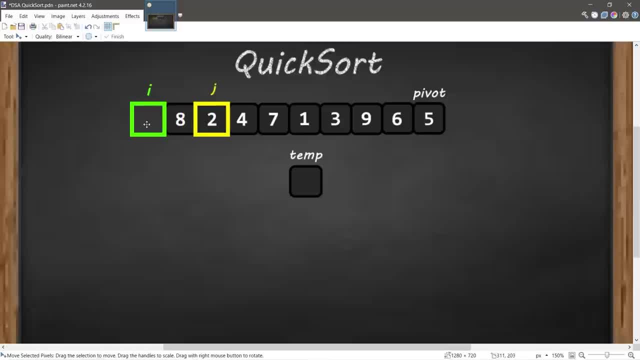 check to see if the value at J is less than our pivot. Again, we check to see if this value is less than our pivot, which it is. What we do now is increment I. Then what comes next is that we swap these two values, I and J, And we'll need the help of a temporary variable. So take the value at I. 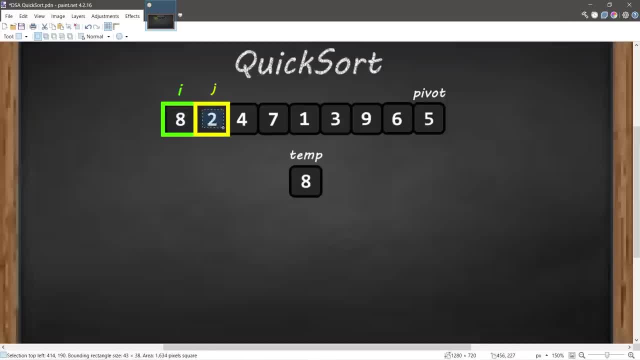 assign it to temp. Take the value at J, assign it to I. Take the value within temp, assign it to J. Then we can move on to the next iteration. Increment J: We check to see if the value at J is less than our pivot, which it is. If that is the case, we increment. I Swap these two. 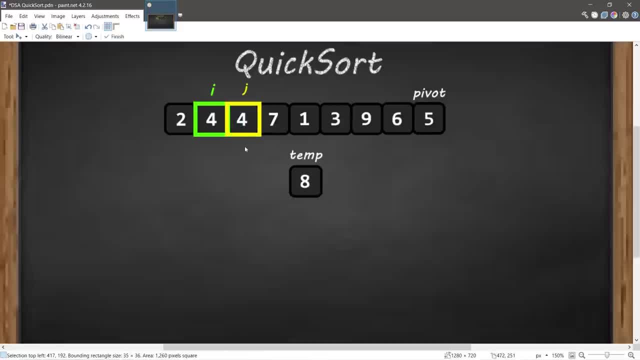 values. We'll repeat this process until J reaches our pivot. Then we can move on to the next step, Increment I. We do the same thing in the next iteration. Here's our final result And here's what we've reached. Here's our final result. 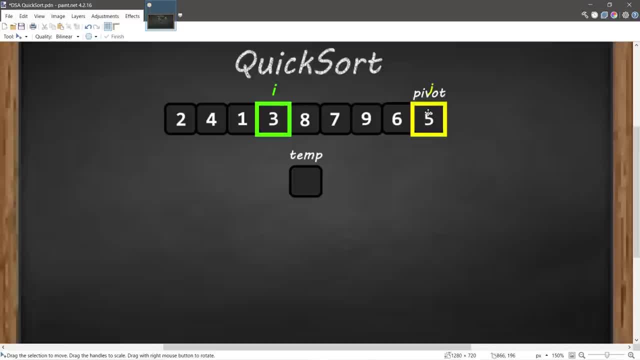 And here's our final result. step after our index j reaches our pivot, We now know where the final resting place of our pivot is going to be. It's i incremented by 1. So we will increment. i then swap the value at index of i. 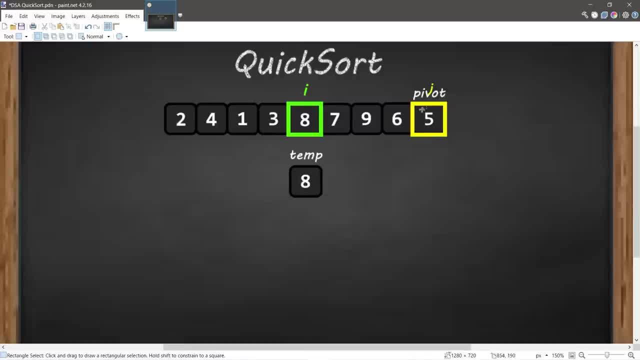 with the value at our pivot. Our pivot is now within the correct place. An easy way to tell is that all elements to the left of our pivot should be less than our pivot. but they're not necessarily going to be in order, and that's fine, They'll be organized later. All elements to the 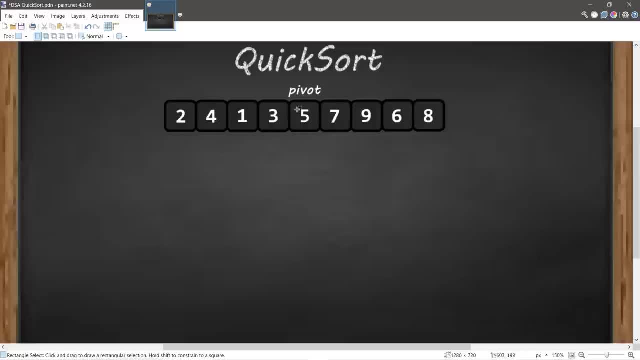 right of our pivot should be greater than or equal to our pivot And, like I said before, they probably will not be in order. The important thing is that elements to the left should be less than our pivot. Elements to the right should be greater than. That's how we know the pivot's in the correct place. 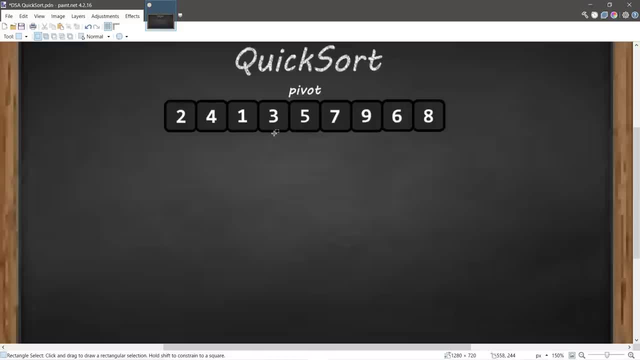 Now the next step. We're going to create two sections, two partitions. The first partition will be all the elements from the beginning of our array up until our pivot, but not including the pivot, And our second partition will be all the elements after our pivot until the end of our array. Quicksort is a recursive 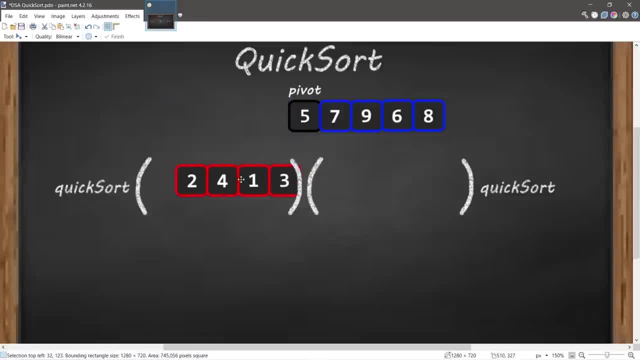 algorithm. We need to pass these partitions as arguments into the quicksort function. Remember that the quicksort algorithm is a recursive algorithm. We need to pass these partitions as arguments into the quicksort function: diversive, divide and conquer algorithm. But, unlike with merge sort, with merge sort we create new. 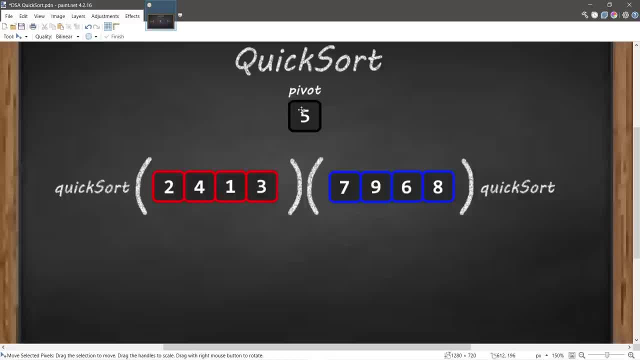 subarrays With quicksort. we will be sorting these arrays in place, but we need to keep track of the beginning and ending indices of these partitions. And then it's just a matter of repeating the same steps over again, but we're going to instead use these partitions, sections of our array I'll give. 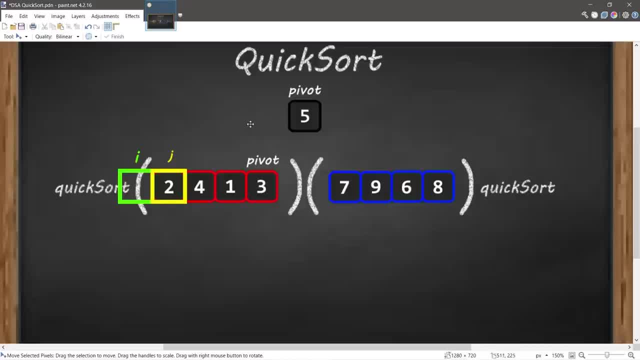 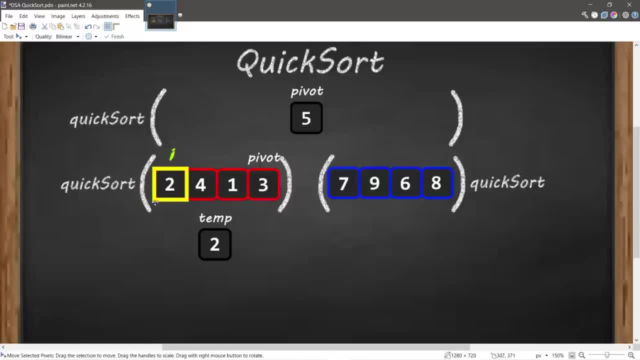 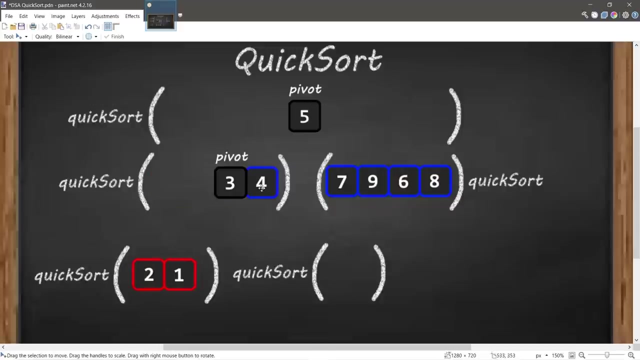 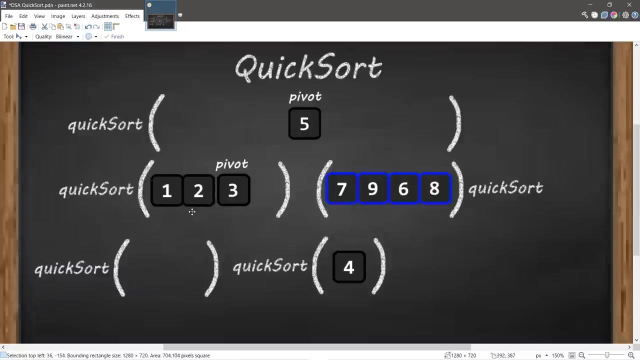 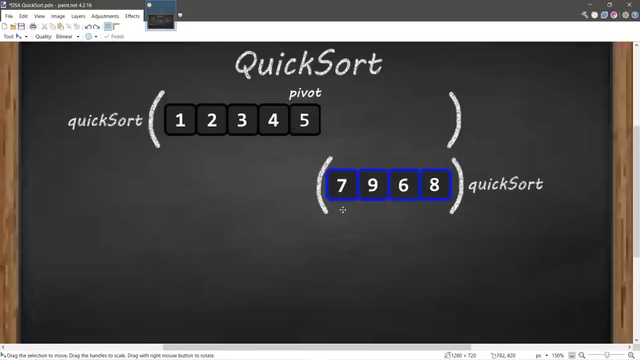 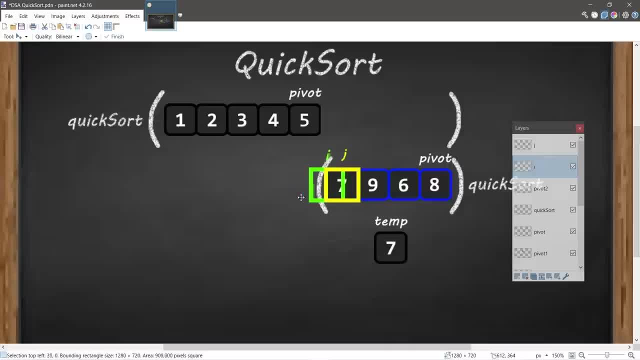 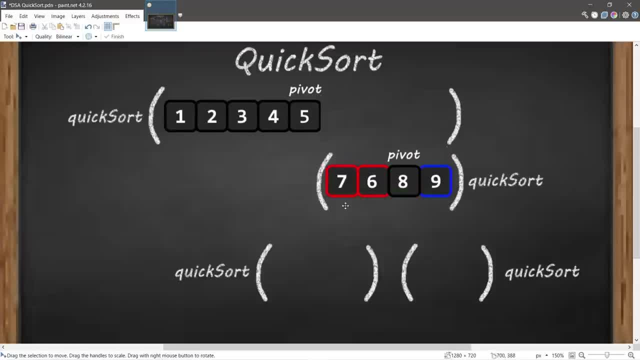 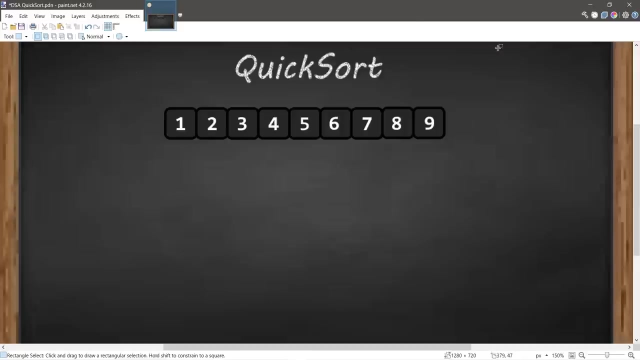 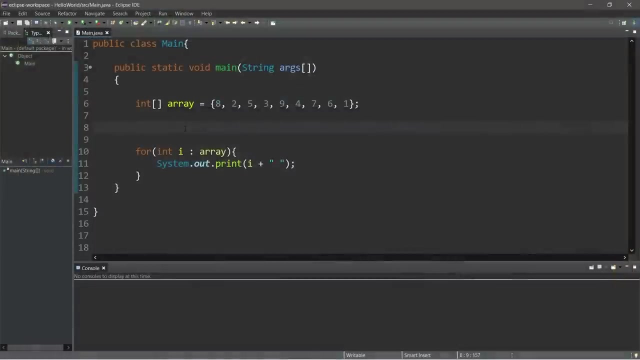 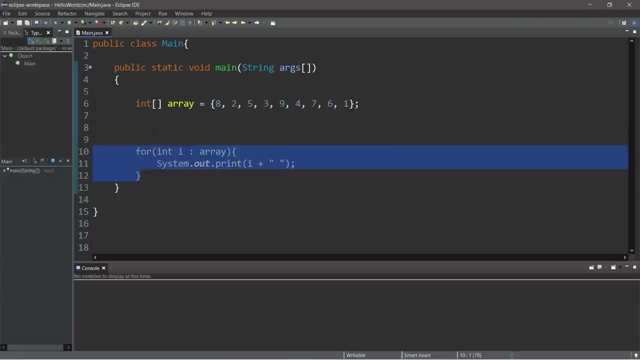 place some random numbers within that array and then some way to iterate and display the elements of your array. i'm just using a simple for each loop. so after running this, of course our array is not yet sorted. so before we display the elements of our array, let's invoke a quicksort. 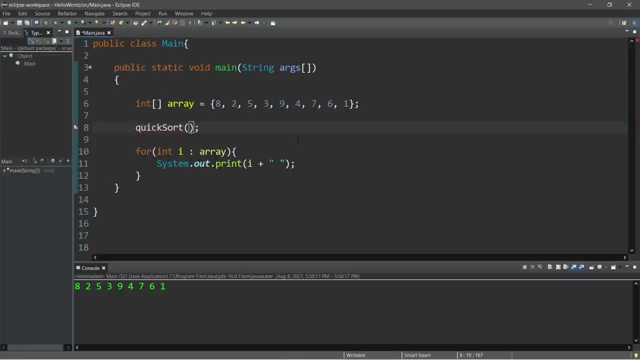 function which we still need to declare, define. there will be three arguments: our array and the beginning and ending indices of our array. so that would be zero for the beginning. then to find the ending you can just say: array dot length minus one. let's declare this function. 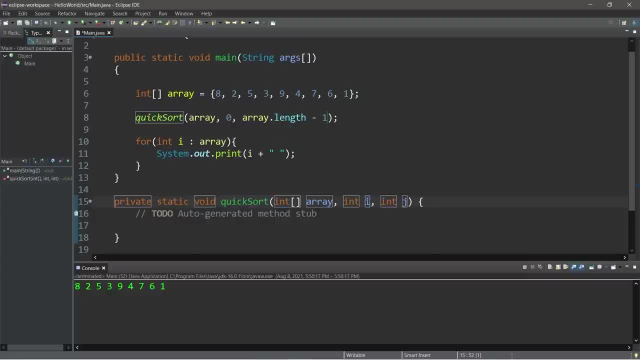 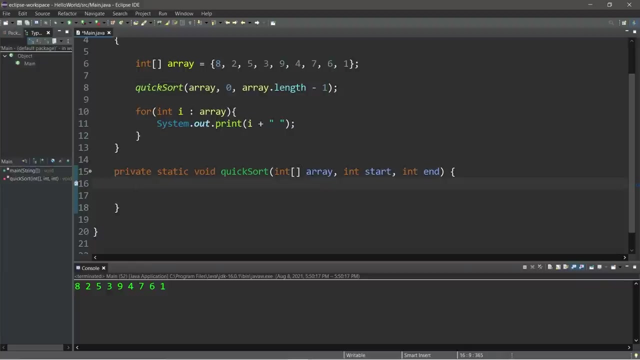 private static void, quicksort, and let's rename some of these parameters. we have our array of integers, named array, and this will be the starting index and this parameter will be the ending index. so we have indices, start and end. now the base case this will use recursion will be: 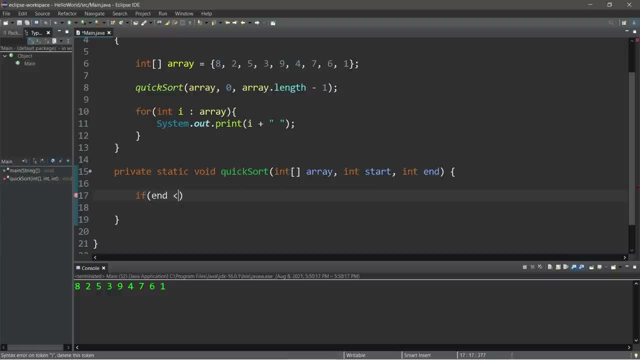 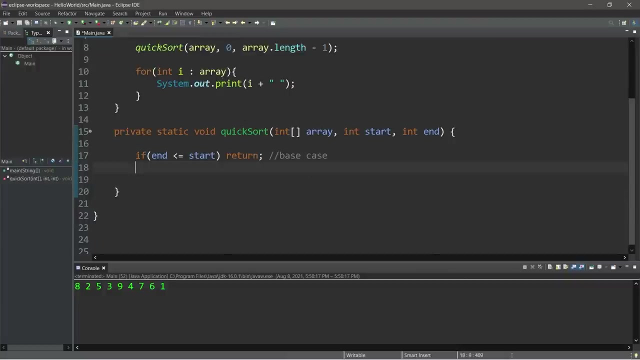 if end is less than or equal to start, then we will return, and this is our base case. eventually, we won't be able to divide our array any further, so that's when we stop and return with our quicksort function. we'll need the assistance of a helper function that we 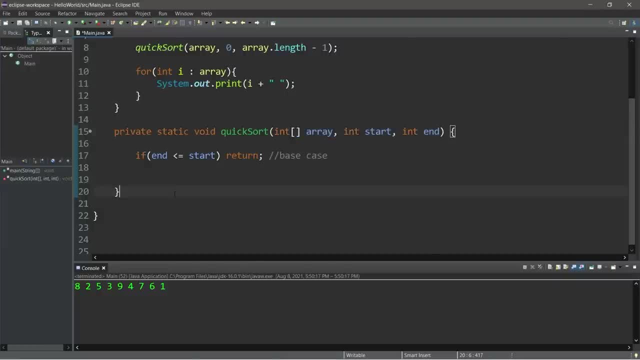 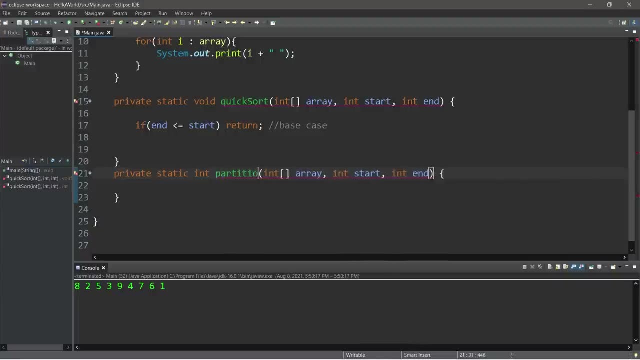 will name partition. let's copy our function declaration, paste it and make a few changes so this will return an int, the location of our pivot, and the function name will be partition and the parameters are the same at the end of our partition helper function. we'll return: 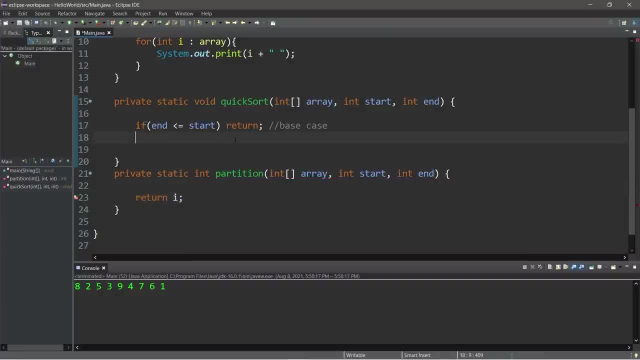 i. i will be the location of our pivot, but we'll get to that later. okay, so within our quicksort function we'll need to find the location of where to pivot- int pivot- and the partition function will be in charge of that. partition is going to sort our array and find the pivot. so all elements to 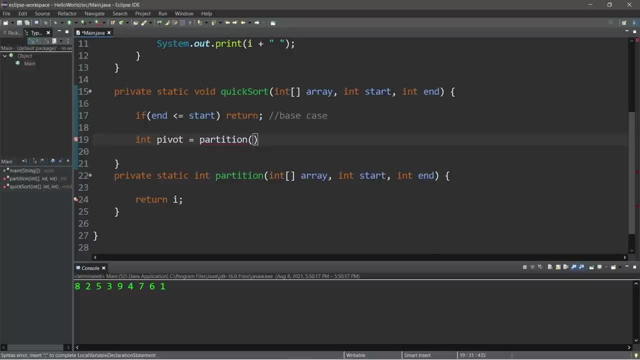 the left will be smaller than our pivot. all elements to the right will be larger, so pass in our array. we're sorting our array in place. there's no need to create any sub arrays. we'll just pass in our original array, as well as the start and end, after we figure out where our 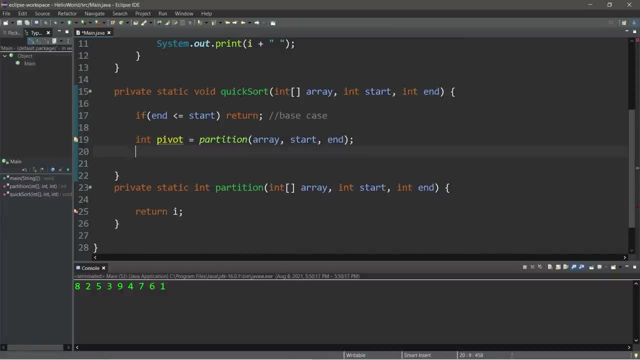 pivot's going to be. we can pass in each partition recursively back into the quicksort function. so again we will invoke quicksort, pass in our array the start of our left partition and the ending of our left partition, and that is where pivot is minus one. we do not want to. 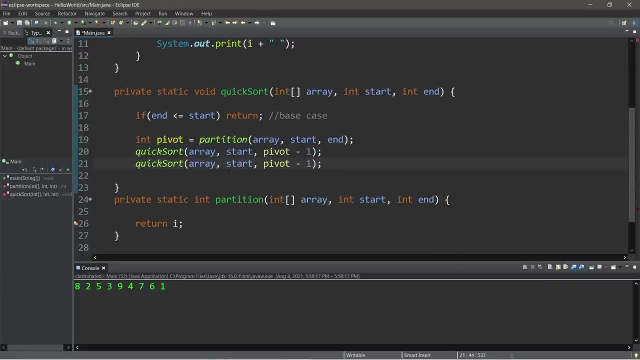 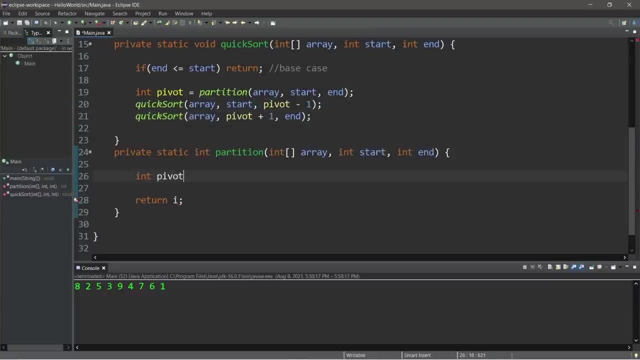 include our pivot and then we will need to use quicksort on the right partition change. start to pivot plus one, because the pivot is already in place, and then the end of our array. in this variation of the quicksort function we will say that pivot is at the end. it will always. 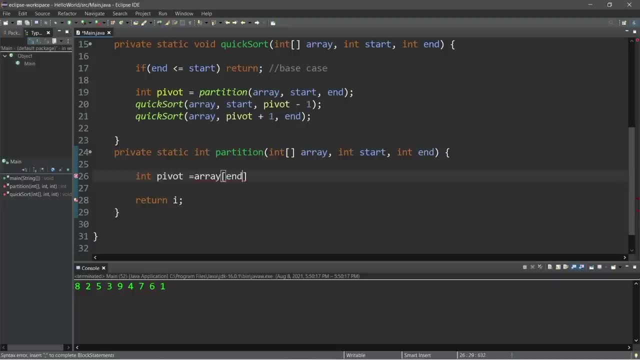 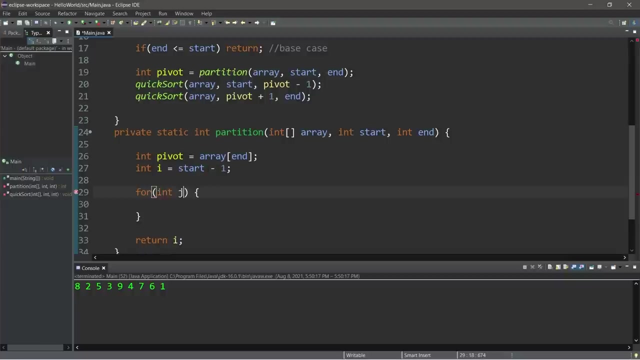 be at the end. to begin with, int pivot equals array at index of n, we'll need two indices, i and j. we'll create index i equals start minus one, and then we will iterate through our array and this way we will declare int j our second index, int j equals start, and we will continue this for loop. 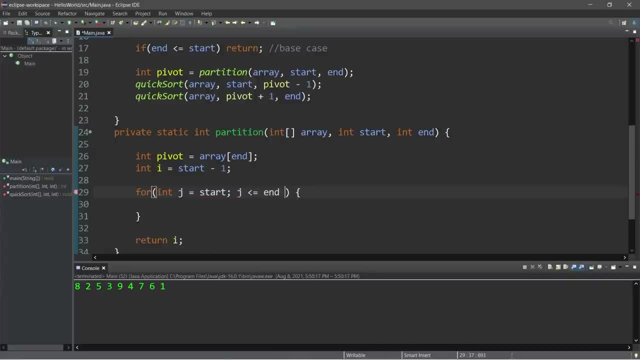 as long as j is less than or equal to the end of our array minus one, then increment j by one. what we're going to check is if array at index of j is less than our pivot. if one of these elements is less than our pivot, we want it on the left hand side of our pivot. 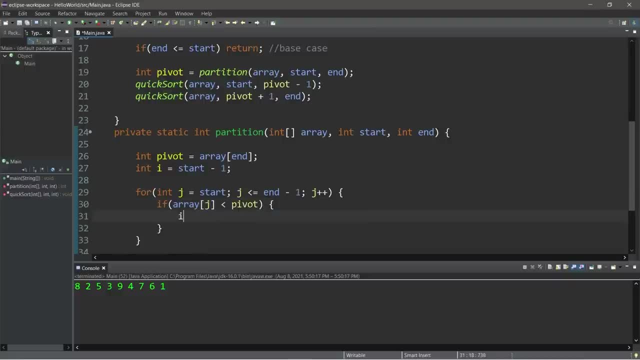 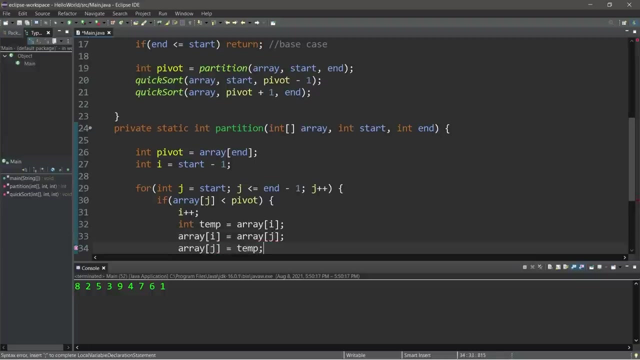 larger than our pivot should be on the right hand side. so we will increment i by one and do a basic variable swap and we'll need the help of a temporary variable. int. temp equals array at index of i. array at index of i equals array at index of j. lastly, array at index of j equals temp. 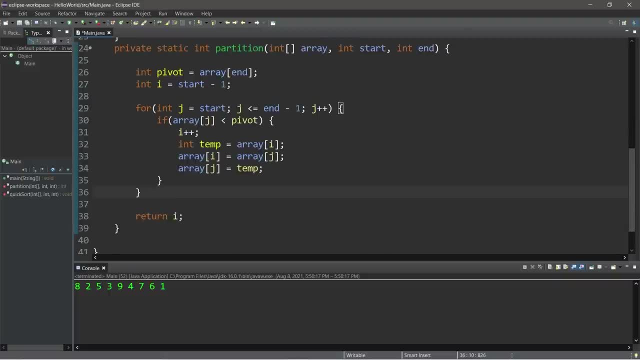 this is just a basic variable swap. once all elements that are less than our pivot are on the left hand side and all elements that are larger than our pivot are on the right hand side, what we will do now is increment i by one and then insert our pivot into its final resting place. 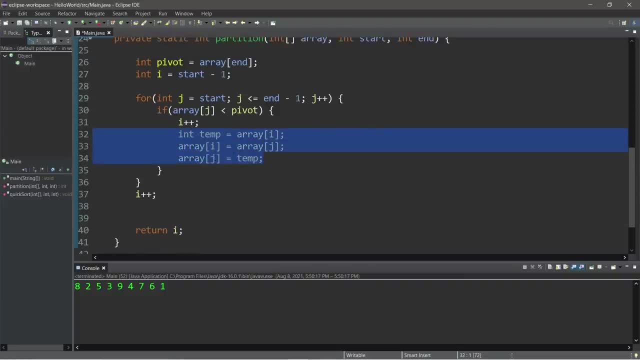 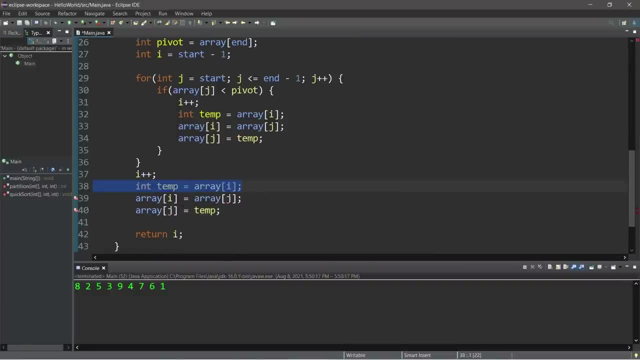 with another basic variable swap. so let's copy this code, then paste it and make a few changes. int temp equals array at index of i. that's the same. array at index of i equals array at index of end. array at index event equals temp, and that's it. and then make sure you return i at the end. 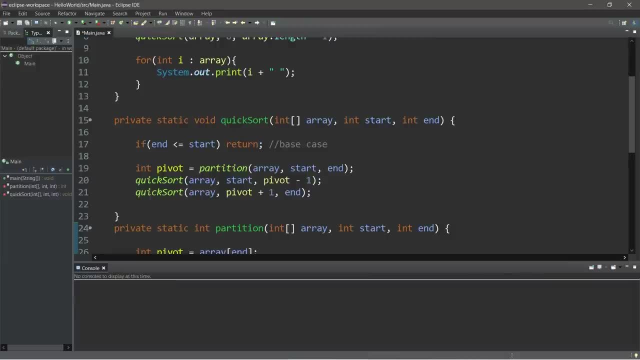 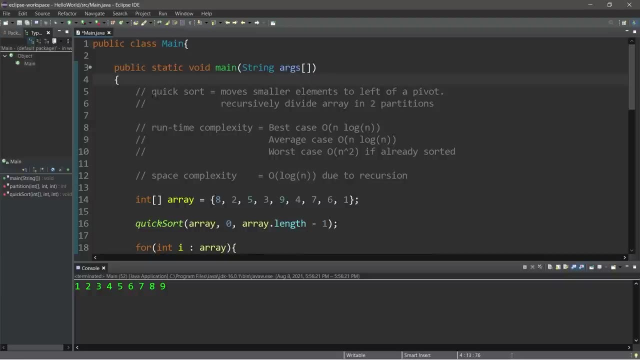 that is the location of our pivot. then, after running this, our array is now sorted via the quicksort algorithm. in conclusion, the quicksort algorithm moves smaller elements to the left of a pivot. we recursively divide our array into two partitions and pass those partitions as arguments. 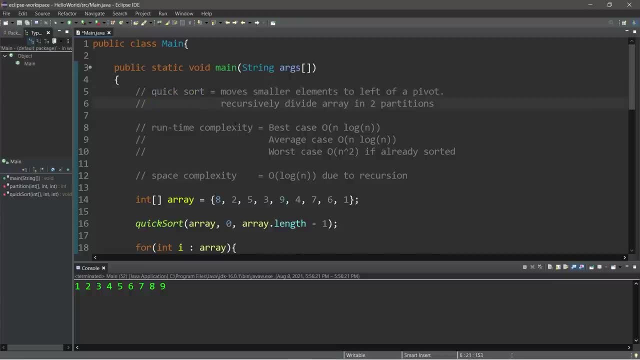 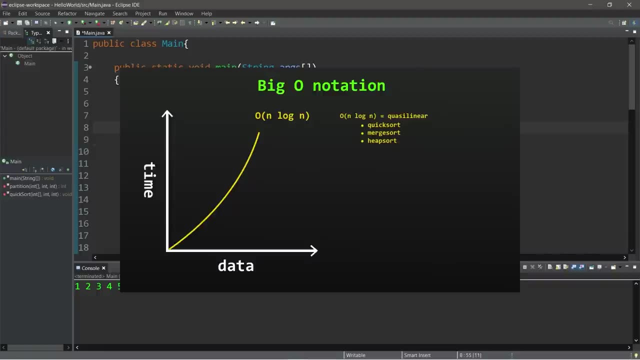 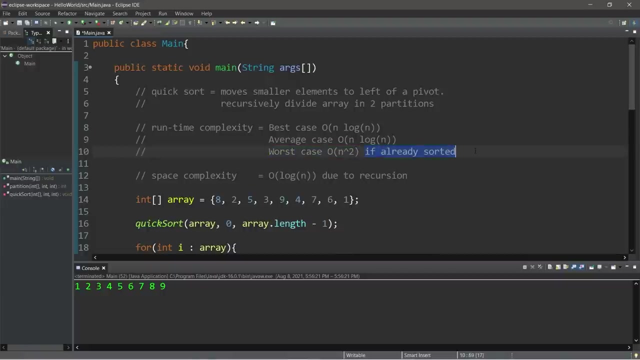 recursively into the quicksort function. the runtime complexity of the quicksort algorithm actually varies. in its best and average cases it runs in big O of n log n. however, in its worst case it can run in big O of n squared. this is rare and it occurs if the array is already sorted. 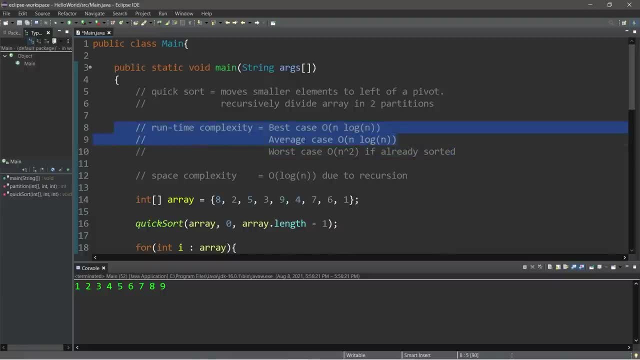 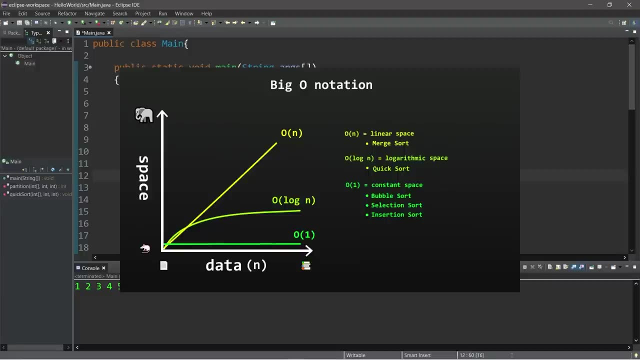 or close to being sorted, but most of the time it will run in big O of n log n and the space complexity of the quicksort algorithm is big O of log n. this is due to the fact that the array uses more space than bubble sort, selection sort and insertion sort, even though it sorts in place. 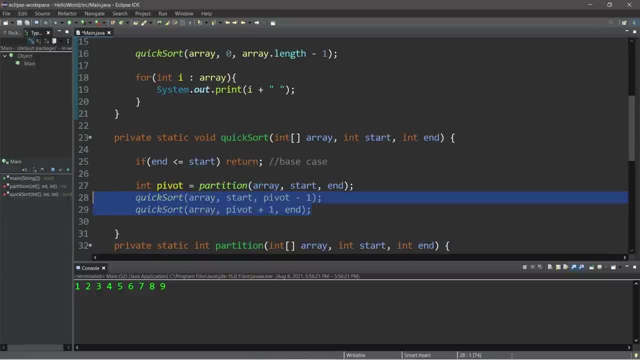 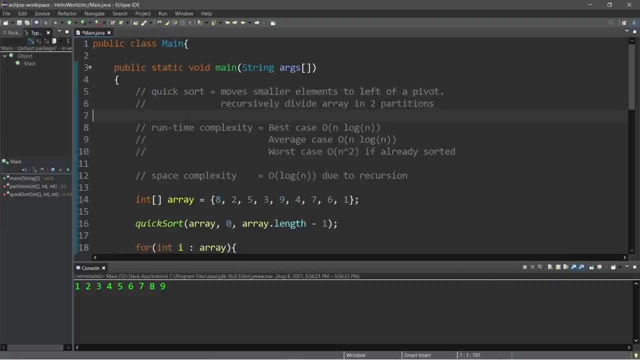 that's because the quicksort algorithm uses recursion. we're adding frames to the call stack, which takes memory. so yeah, that is the quicksort algorithm. if you found this video helpful, please be sure to smash that like button, leave a random comment down below and subscribe if you'd like to. 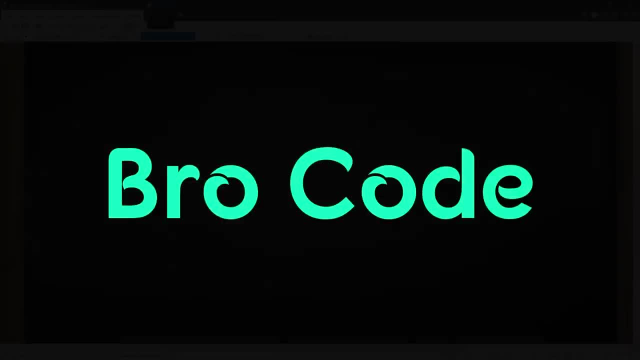 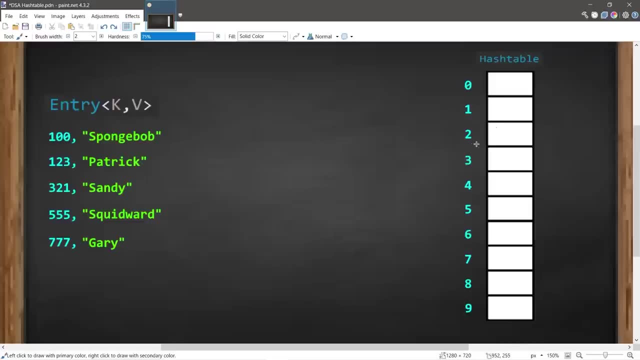 become a fellow bro. all right, what's going on? everybody hash tables. a hash table is a collection of key value pairs. each key value pair is known as an entry. we have two pieces of data: the first is the key and the second is the value. in this example, let's pretend 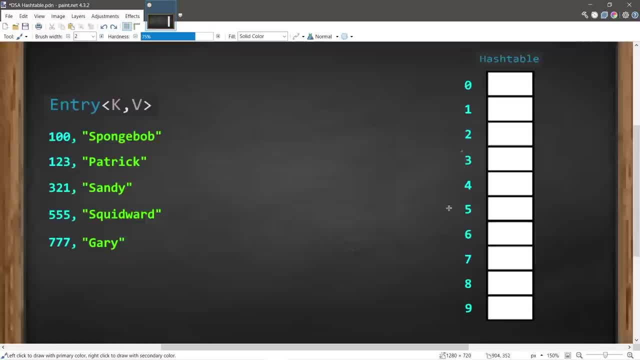 that we're a teacher and we need to create a hash table of all of our students. each student has a name and a unique student id number, but these can be of any data type that you would like. in this example, the key will be an integer and the value will be a string, so we're going to create a hash table. 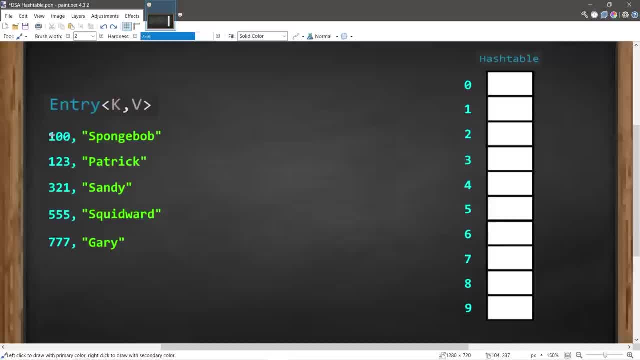 variable that's going to account for all our prove arn. Now you can actually use a smokey pen, if you want to, to wonder how the hash table成p�� hormone, vadra, doesn't vir delete an urban with bolder 1958. we have basically the gehut formula that 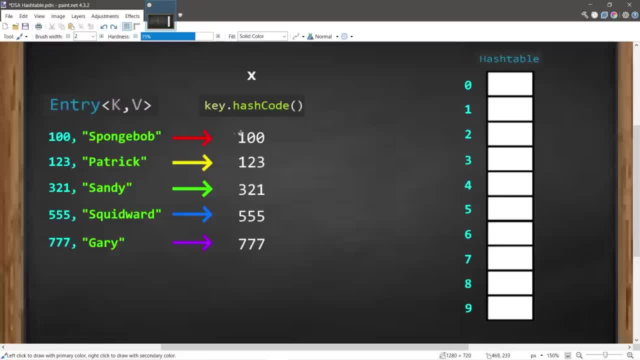 Gerstrom pushing a simple point experiment out, and then it gets out whether we should do this or that the key is entered by distance 32, SHA, oben, sarbrit, and the hash count is 0, cota 0。. So how do we know at which index to place each of these entries? Well, what w? e could do is take. each key and insert it into a hash code method. the hash code method will take a key as input, plug it into a formula and spit out an integer. this integer is known as a hash. Now, if we're finding the hash code of an, 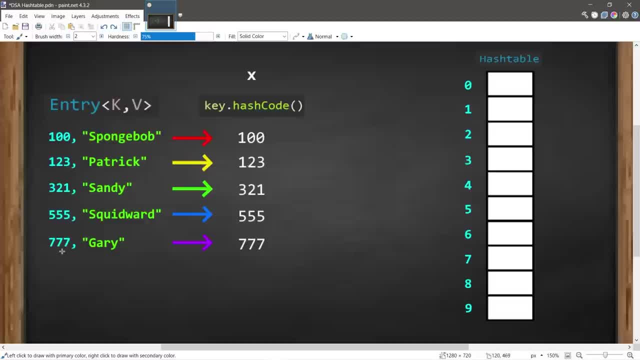 is 123, so on and so forth with the other keys. so, after finding the hash of your key, now what can we do? these numbers are way too large and the size of our hash table is only 10 elements. what we'll do next is take each of these hashes and divide each of them by the capacity, the size of our hash table. 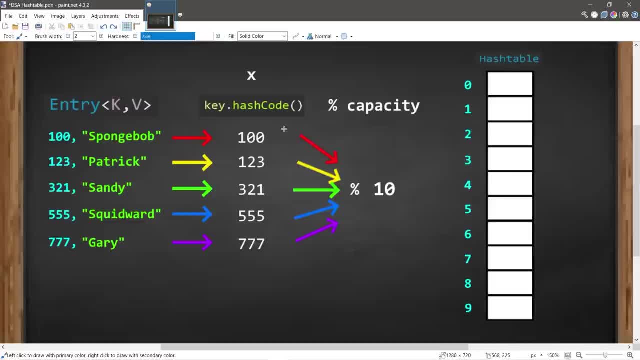 we have 10 elements. so take each hash, divide it by the capacity of our hash table, whatever the remainder is, we will use the remainder as an index and to find that we will use the modulus operator. so 100 divides by 10, evenly, the remainder is 0. so 100 modulus 10 gives us a remainder of 0. 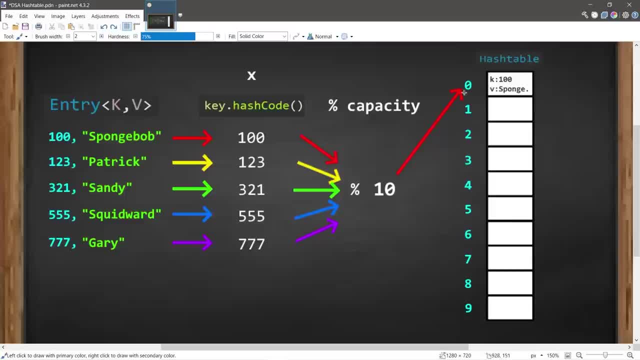 so spongebob's entry we will place at index 0 within our hash table. so the hash of patrick's key is 123, 123 modulus 10 gives us a remainder of three patrick's keyれない handle as really important and we need to be able to useatz Gabriel asenden. 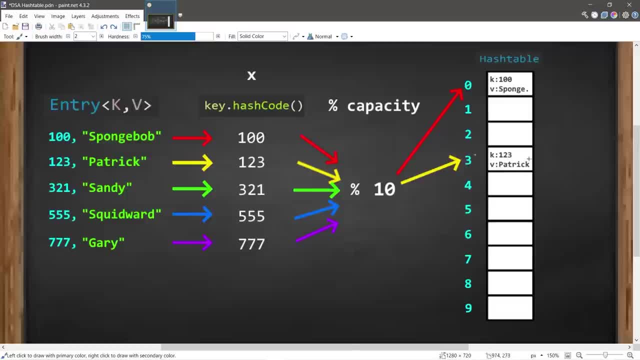 with widow. in order to annoyed cataloging, we will add key statement for these嫁y in our hash table. between the error which i just said is thearse and the error in indexつ and the shoulder key within the decimal, Patrick's entry will be inserted at index 3 of our hash table. 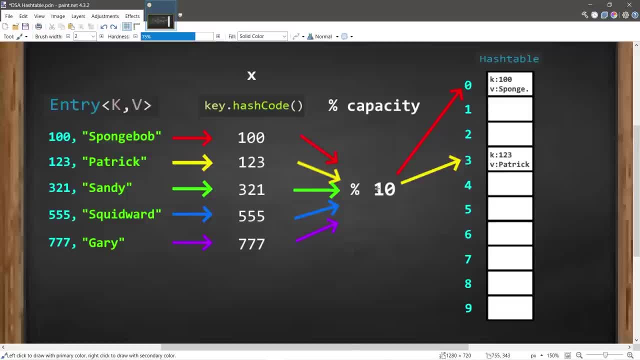 So here's a little shortcut: If you have a number modulus 10,, you can find the remainder, and that is the last digit. 321, modulus 10, will give us a remainder of 1.. Sandy's entry will be placed at index 1.. 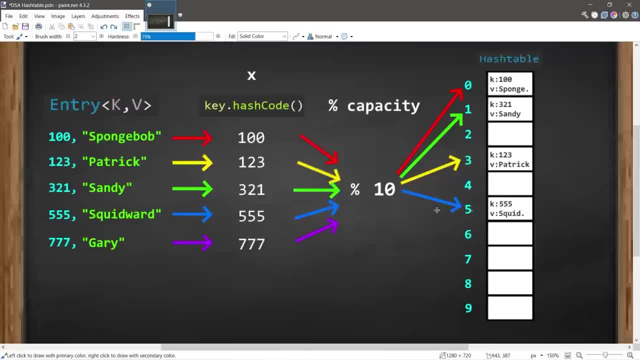 Then Squidward's entry will be placed at index 5.. 555, modulus 10, is 5.. And Gary's will be at index 7, following the same pattern. Now here's one situation. What if two hashes are calculated to be the same value? 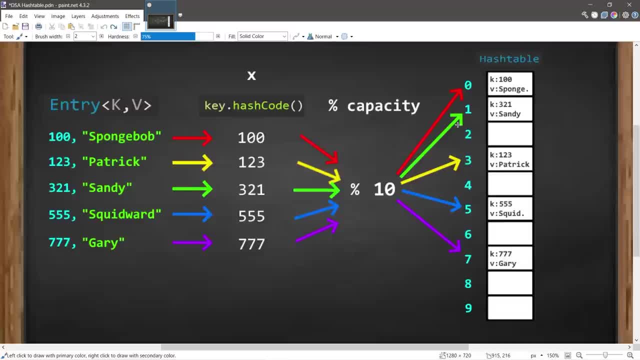 That is known as a collision, and I can best demonstrate that with a separate example. In this next example, let's say that each key is now a string, Each entry is a pair of strings. We will first need to find the hash of each of these keys. 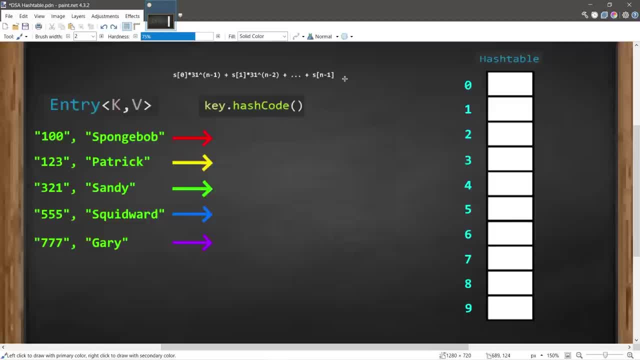 So the hash code of a string uses a different formula. Basically speaking, we're going to take the ASCII value of each hash key and we're going to take the hash key value of each hash key. We're going to take the hash key value of each character within the string and plug it into this formula. 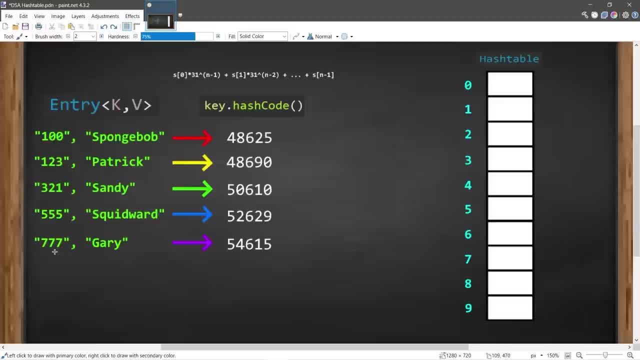 I went ahead and calculated the hash of each of these strings using this formula of the string hash code method, and the next steps are the same as before: Take each hash divided by the capacity of our hash table and find the remainder, So beginning with the first hash. 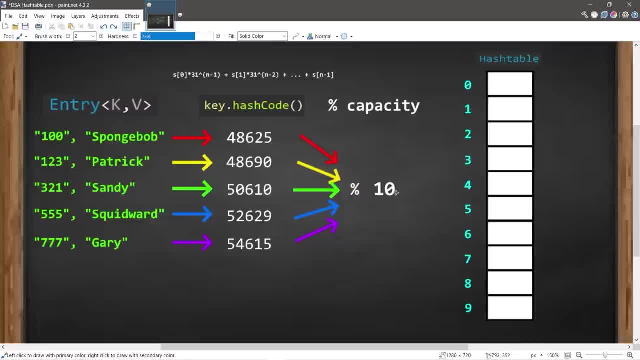 48,625, modulus 10, gives us a remainder of 5.. Spongebob's entry is now at index 5.. within our hash table Now, Patrick's will be at index 0.. Now here's Sandy's. Sandy's will also be 0. 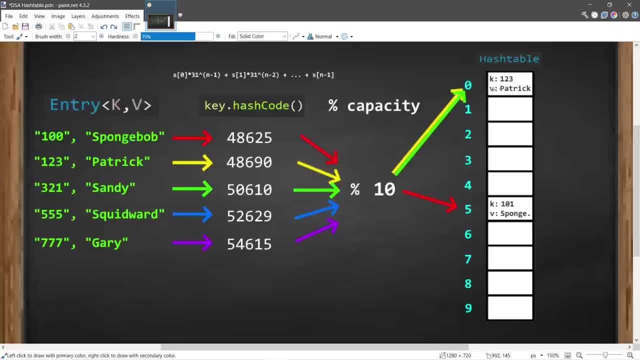 We have a collision. Both of these entries will be located at the same index, So what do we do? Each of these storage locations is also known as a bucket, And the most common resolution for a collision in a hash table is that we will turn each bucket into a linked list. 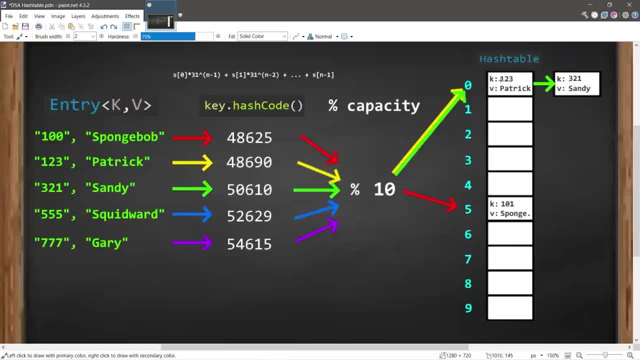 If this bucket already has an entry within the first entry, we will also add an address to the location of the next entry And keep on adding more if there's more entries within this bucket. so in this way this becomes a linked list. 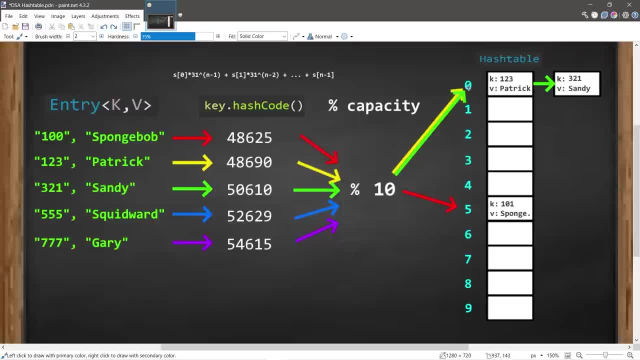 If we're looking up a key, we first go to the index in which it's located. If there's more than one entry, we will search linearly through this bucket as if it were a linked list, until we find the key that we're looking for. 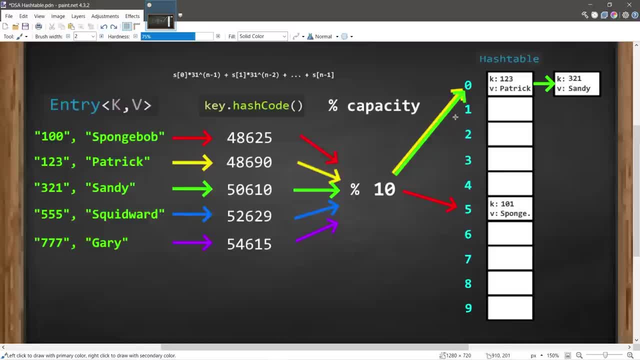 So that's the most common resolution when there is a collision, but ideally you would want each of these entries to be within their own bucket, Based on the hash of Squidward's key. Squidward's entry has an index of 9, and Gary. 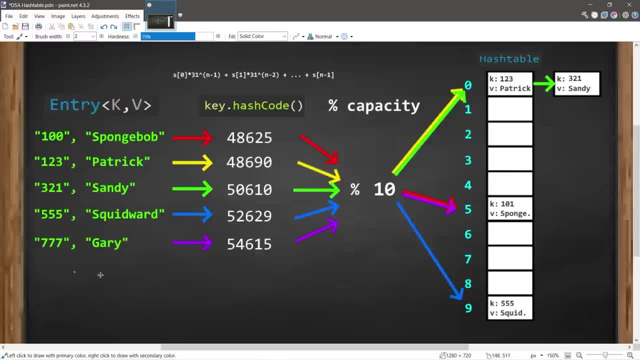 Gary has an index of 5, and there's another collision, We will add the address of Gary's location to the first entry and this bucket becomes a separate linked list. This process is known as chaining. The less collisions that there are, the more efficient that this hash table. 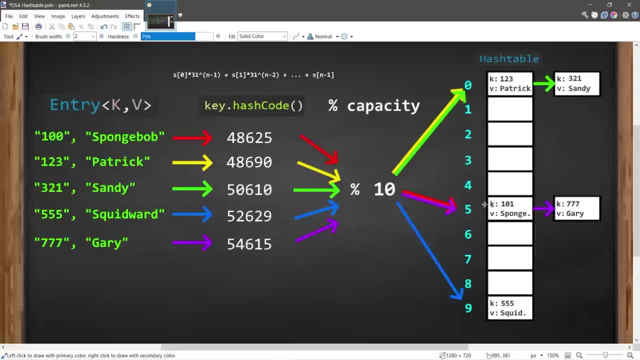 is going to look up a value. Ideally you would want each entry to have their own bucket, but collisions are possible. To reduce the number of collisions you can increase the size of the hash table, but then again the hash table is going to use up more memory then. so people usually find a. 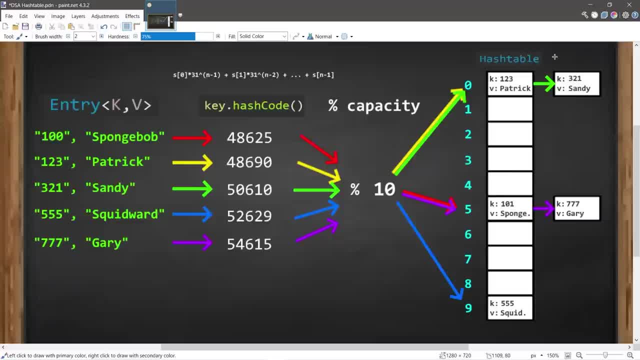 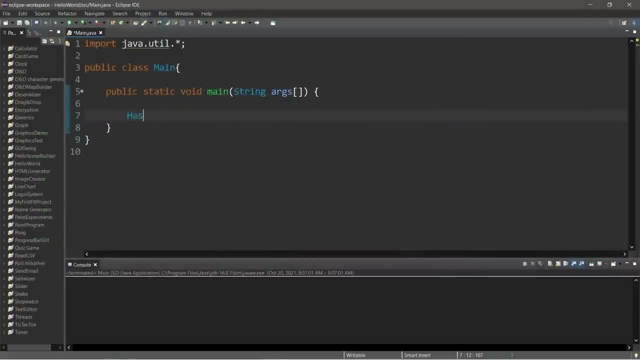 balance between the two. So, yeah, those are hash tables in theory. Let's create our own now. All right, everybody. so let's implement a hash table in Java. So we will need to declare this hash table and list the data type. 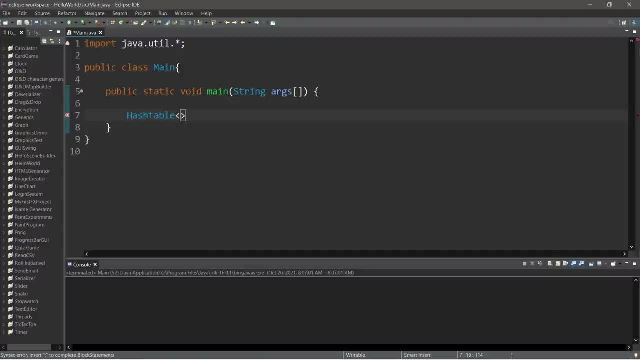 of our key value pairs. If we need to store primitive data types, we can use the appropriate wrapper class. So let's store integers and strings: Integer and string. The integers will be the keys, the strings will be the values. We'll map student ID numbers and student names. 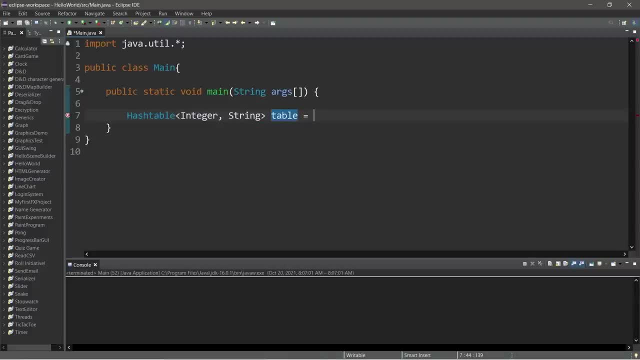 And I'll name this hash table just simply: table Equals new hash table. There we go. So, in Java, when we create a hash table, these have an initial capacity of 11 elements and a load factor of 0.75.. So once 75% of our elements are filled, 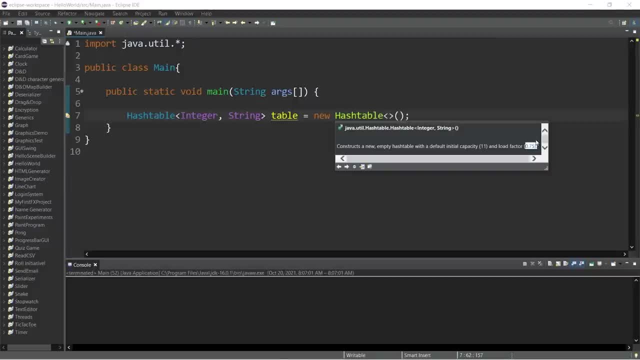 this hash table will dynamically expand to accommodate more elements. Now you can set a different capacity for your hash table: Instead of 11, let's say 10 to be consistent with our example in the previous part of this lesson, And if you would like to change the load factor. 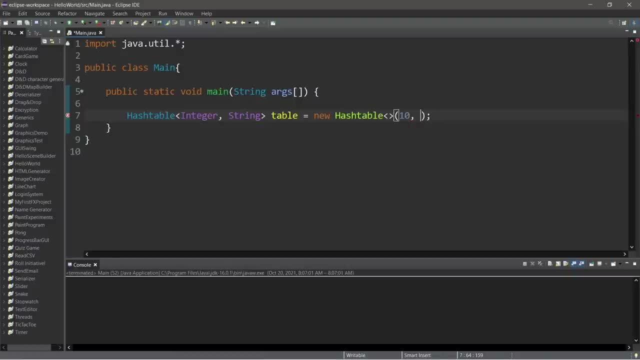 you can add that as well. Instead of 75% let's say 50%, So we would pass in a floating point number, So 0.5, then add an F at the end for floating point numbers. But in this example let's just: 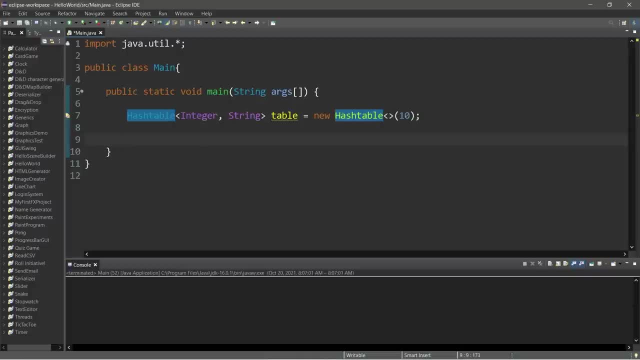 keep the load factor consistent. So let's start adding some key value pairs. To add an element to your hash table, use the put method, So tableput, And then we will pass in an integer as the key and a string as the value. So our first student is Spongebob. He has a student ID of 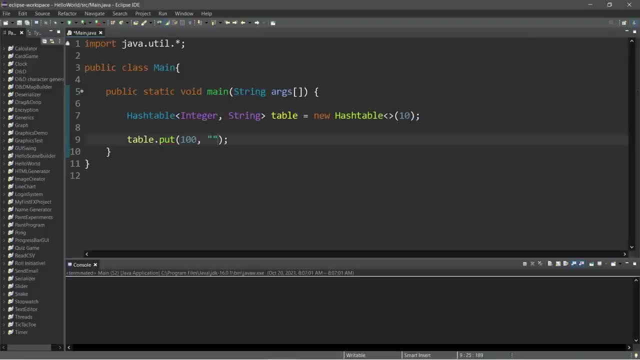 let's say 100.. And let's pass in a string for the value Spongebob. Okay, that is our first student, So let's add a couple more from the previous example. So we have Spongebob Patrick with an ID of 123.. Sandy with an ID of 321.. 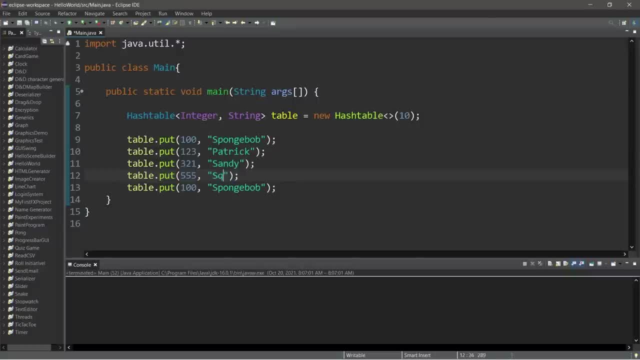 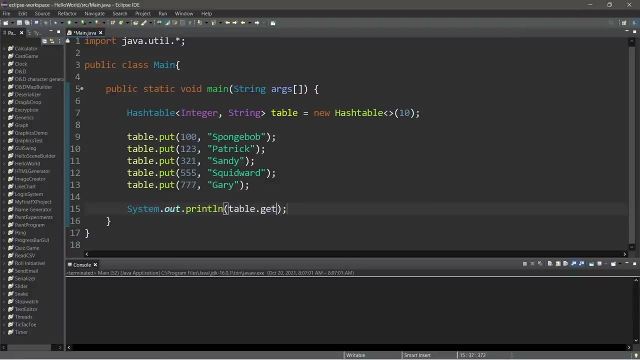 Squidward with an ID of 555. And Gary with an ID of 777.. Now, to access one of these values, you can use the get method of tables. So I'll display this within a println statement Tableget And I will pass in a key. Let's get the value at key number 100.. So this student. 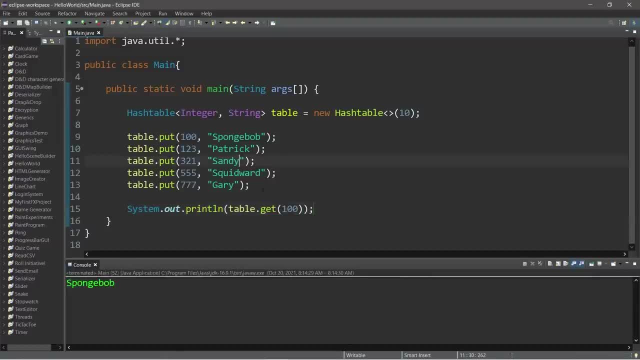 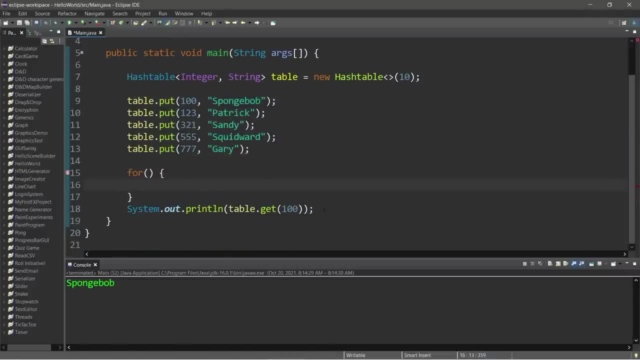 is Spongebob. How can we display all of the key value pairs of a table? Well, we could use a for loop. So I'm going to create a for loop and place this within it, So to iterate over the keys of our table. this is what we can write. We can use an enhanced for loop, So we are iterating over. 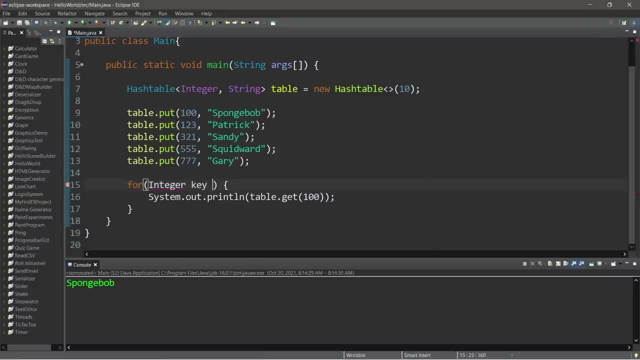 a set, So the data type is integer key colon. So to make our hash table iterable, we can get all of the keys from our table and put them within a set. A set is iterable, So we will iterate over table dot key set method. This will take all of our keys and return a set, And a set is something. 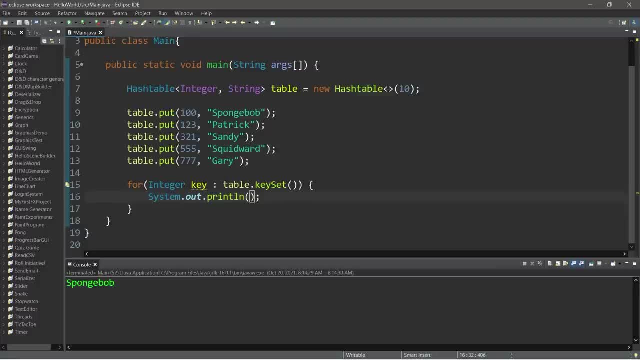 we can iterate over And within our println statement. let's print each key, key plus, then maybe I'll add a tab to separate these. Plus, table dot, get, Then pass in whatever our key is. Okay, so after running this, 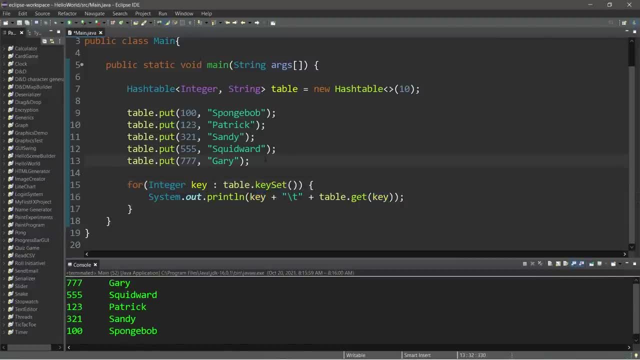 this will display all of our key value pairs And if you need to remove an entry, well, there's a remove method: Table dot remove. Then pass in a key. Let's remove Gary. So remove the entry with this key 777.. And Gary is no longer within our table, But we'll keep him in. I'll turn. 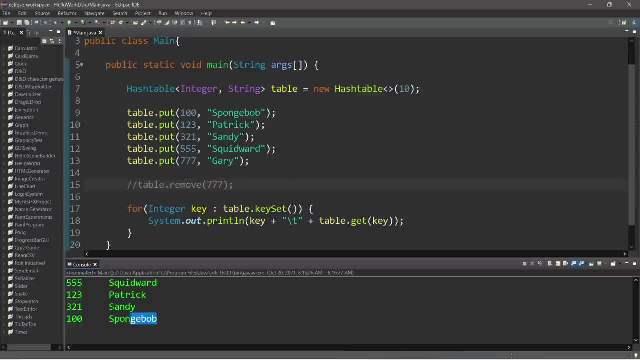 this line into a comment. Now, just to get a better understanding of where these key value pairs are being placed, let's also display each hash code for each of these elements. So preceding our key, let's display each hash code. I'll precede our key with a tab and let's display each key's. 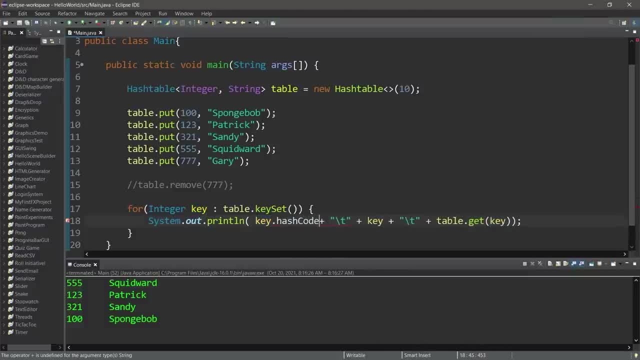 hash code: Key dot. hash code method. If we're using the hash code of integers, this will return the primitive integer value represented by the prefix cuz, like in the alphabets field. So we can integer value represented by the key that we're passing in If we're using the hash code method. 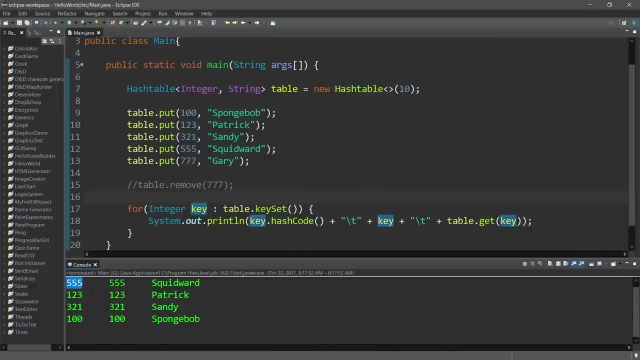 of integers. well, the hash is going to end up being the same integer, So you can see that these numbers are the same. To calculate an index we can follow the hash with modulus operator. then the size of our table. We set this to originally be 10.. So we have Gary at index 7,. 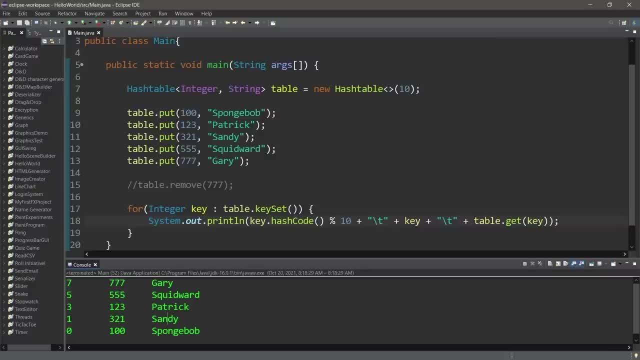 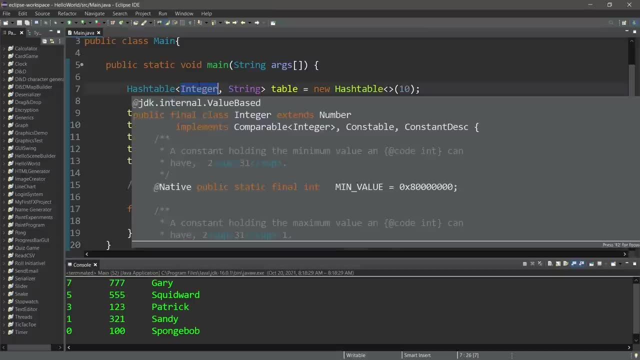 Squidward at index 5, Patrick at 3, Sandy at 1, Spongebob at 0.. Now if our data type was strings, we would use a different hashing formula. So let's change the data type to string and all. 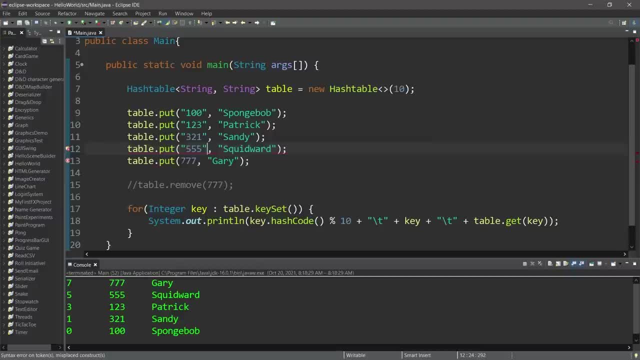 of these keys are now strings. Then let's remove modulus 10 and change the data type of our for loop to strings. String key. Okay, these are the new hashes for each of our keys. This key is the one that we're going to use to hash, So let's change the data type to string. 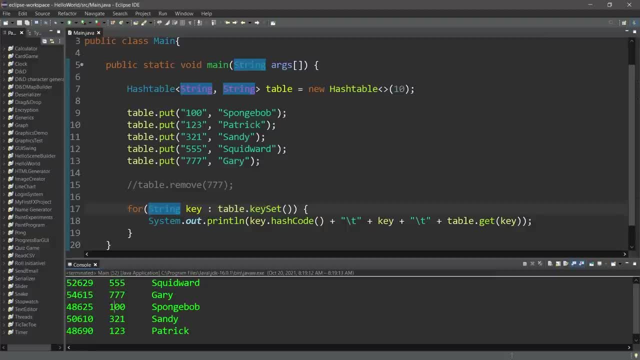 This key has this hash number, This key has this hash number, so on and so forth. So different data types will have different hash code formulas. Now let's calculate the element in which each of these entries is going to be placed by adding, modulus, the size of our hash table 10.. So here, 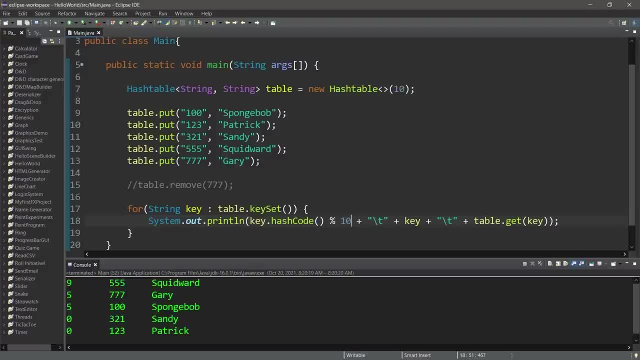 are the elements and we actually have two collisions. We have a collision with these two keys. They're both within bucket 5 as well as these two entries, So both of these will be placed in two buckets. Since there's more than one entry within the same element, we will treat this bucket as a linked. 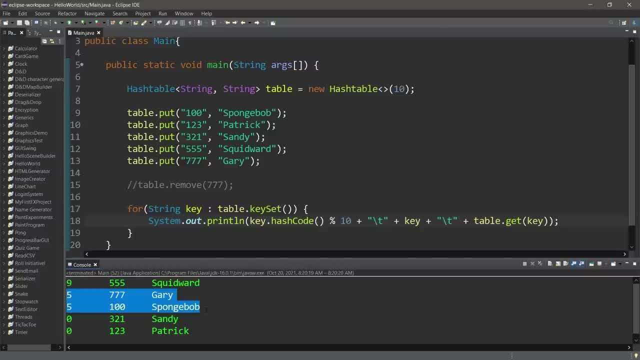 list and just iterate over it linearly until we reach the key that we're looking for Now. one way in which we can avoid collisions is to increase the size of our hash table. If we set this to the default of 11 and change this to modulus 11,, well then these will be placed within different 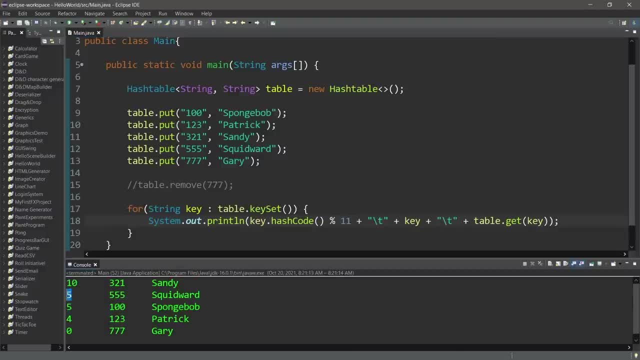 buckets and you can see that they changed. However, we still have a collision with Spongebob and Squidward. So what if we increase this to 21? Do we have any collisions then? Nope, we do not. These keys are within their own buckets. 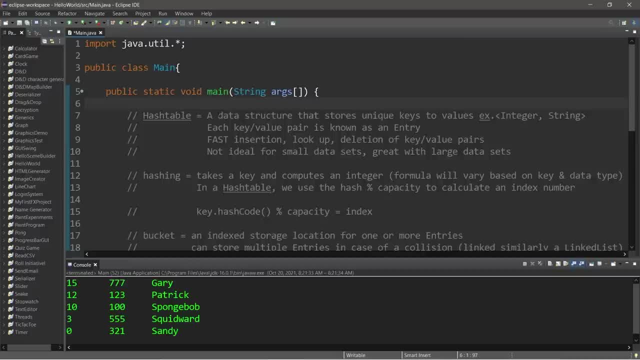 All right, everybody. so in conclusion, a hash table is a data structure that stores unique keys to values. When you declare a hash table, you state the data types of what you're storing, and these are reference data types. Each key value pair is known as an entry and a benefit. 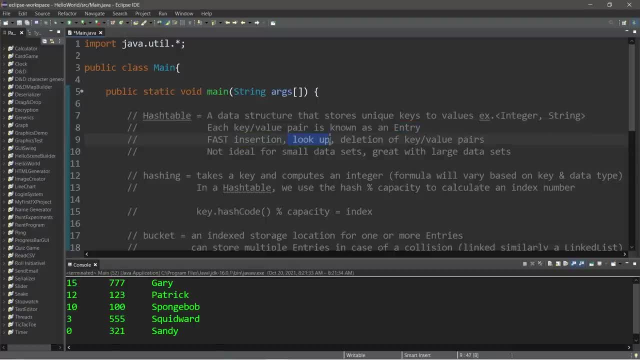 of hash tables is that they have a fast insertion, lookup and deletion. We then calculate the index of the index. This is where you can calculate the index for us. Let's check out the whole idea of an index on this table. So first we have the index orientation of key value pairs, but they're not ideal for 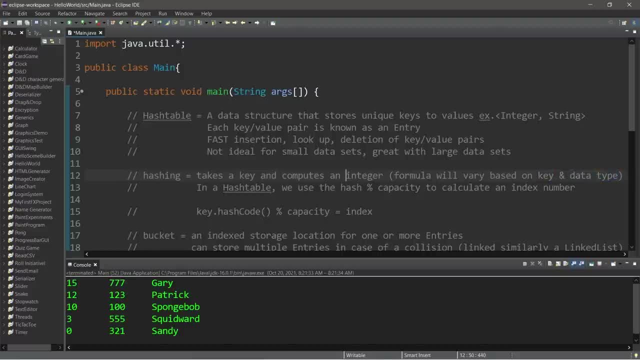 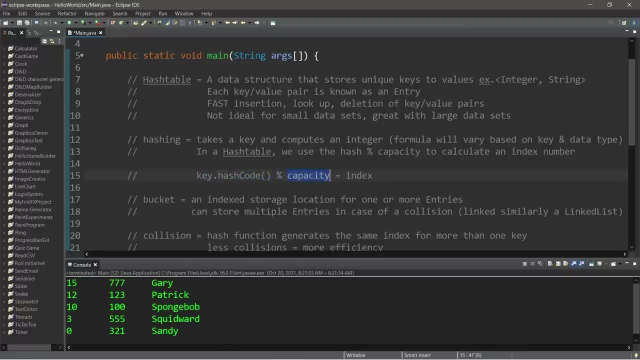 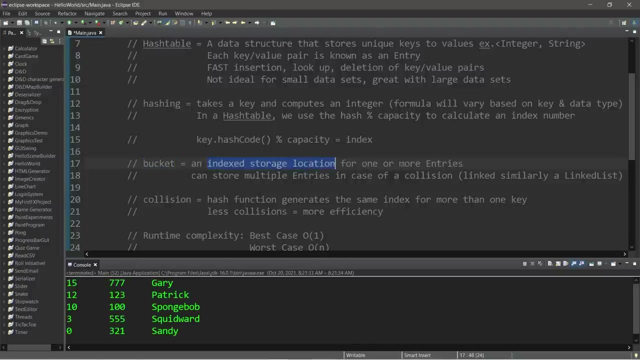 small data sets since there's a lot of overhead, but they're great with large data sets. Hashing in the context of a hash table takes a key and computes an integer. It utilizes a formula which Each index is also known as a bucket. It's an indexed storage location for one or more entries. 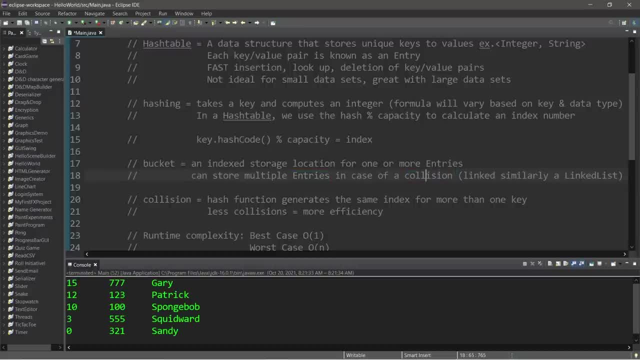 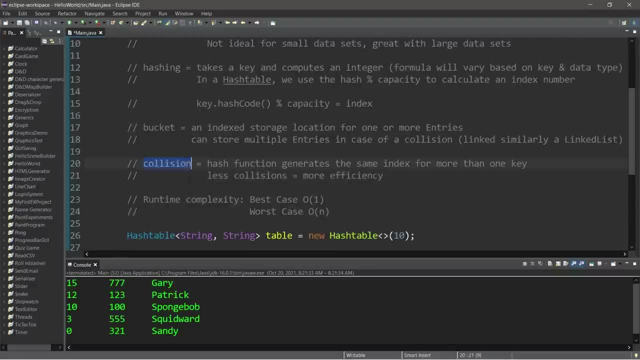 They can store more than one entry in the case of a collision- And in case that happens, we treat each bucket as a linked list. Each entry knows where the next entry is located And, as we discussed, a collision is when a hash function generates the same index for more than one key. 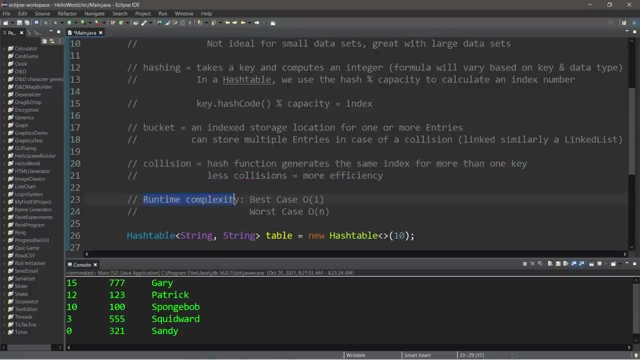 Less collisions equals more efficiency, And the runtime complexity of a hash table varies. If there are no collisions, the best case would be a runtime complexity of O of 1. It runs in constant time. In case there are exclusively collisions, as in, we place all of our entries within the same bucket. 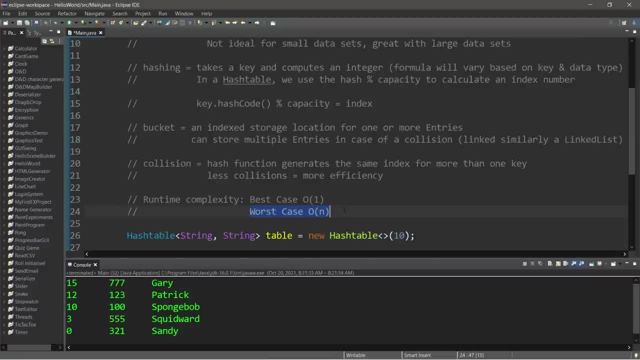 it's going to be one giant linked list And the runtime complexity of a linked list is O of N. It runs in linear time. On average, the runtime complexity of a hash table will be somewhere within this range. So yeah, everybody, those are hash tables. 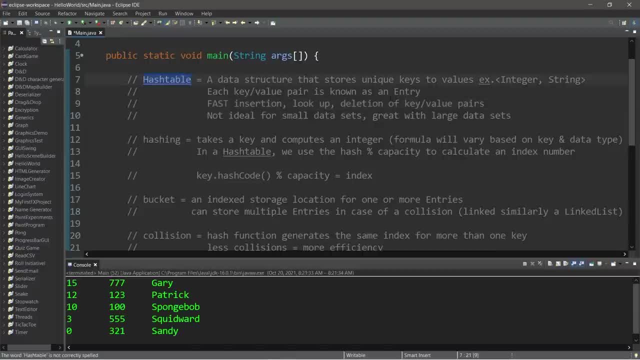 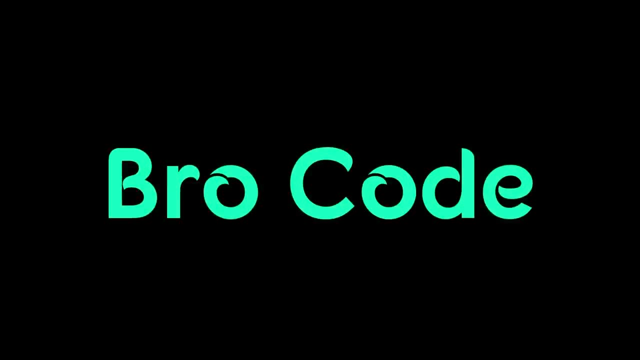 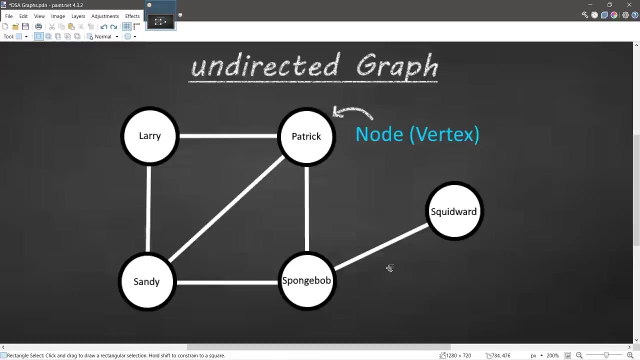 If you would like a copy of all my notes here, I'll post them in the comments section down below. And well, yeah, those are hash tables in computer science. All right, what's going on, everybody? Graphs: A graph is a nonlinear aggregation of nodes and edges. 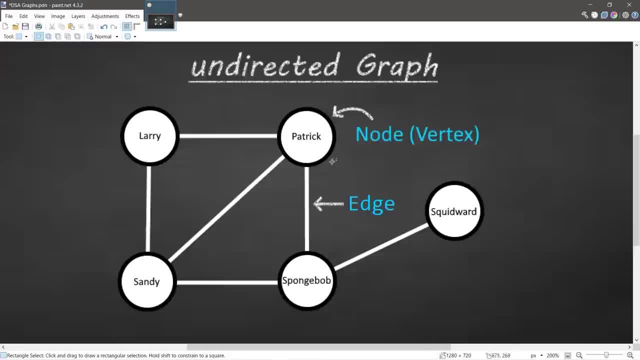 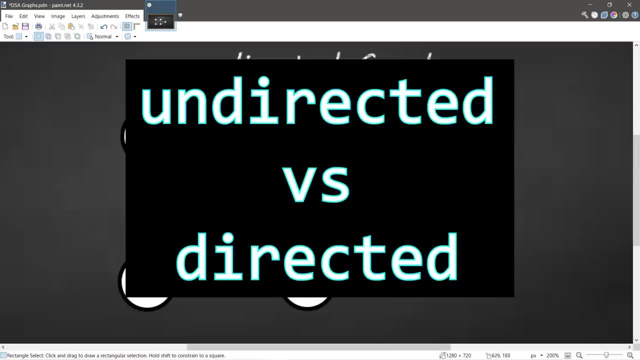 A node, also known as a vertex, may contain some piece of data, And an edge is a connection between two nodes. There are two types of graphs we're going to discuss: Undirected and Undirected. An example of an undirected graph could be a social network like Facebook. 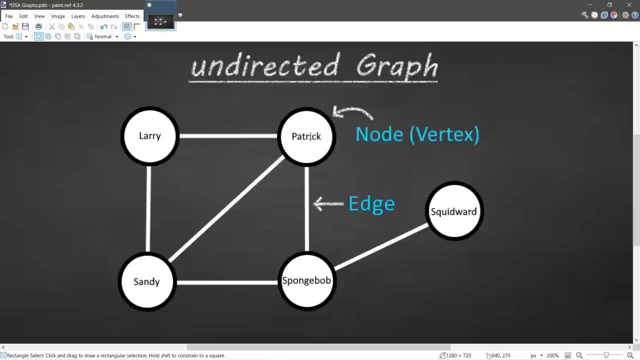 Each node could represent a user, And if one user is friends with another user, well we could establish a friendship, an edge, a connection between these two nodes. If two nodes are connected, they have what is known as adjacency. In this example, Larry is friends with Patrick and Sandy. 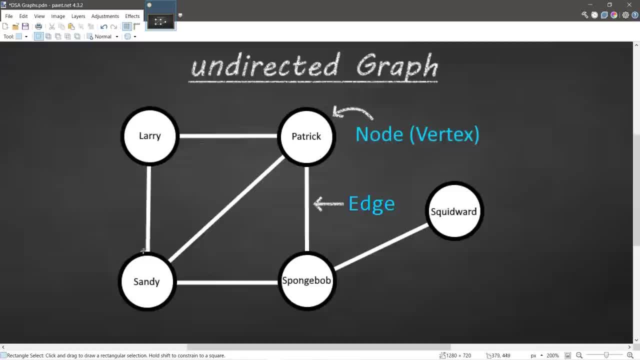 So Larry has adjacency to Patrick and Sandy Patrick is friends with Larry, Sandy, SpongeBob And SpongeBob is friends with Sandy Patrick and Squidward And Squidward is adjacent to only one neighbor, SpongeBob. So a social network could be an example of an undirected graph. 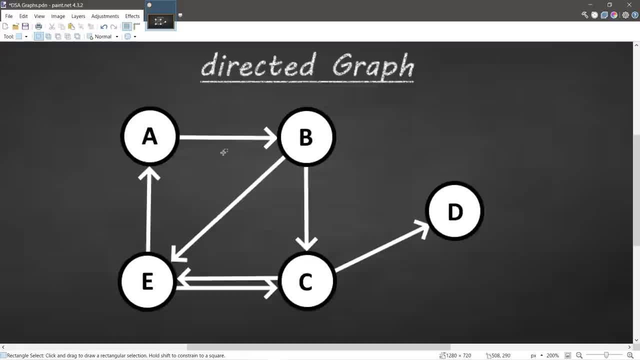 The other type of graph is a directed graph. A directed graph contains edges that will link one node to another. However, these are one way connections. In this example, node A would have adjacency to node B, but not the other way around. 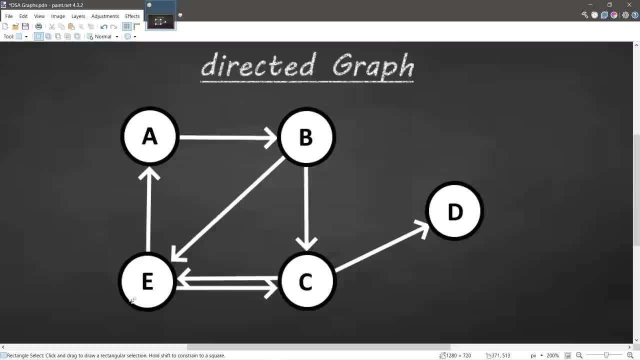 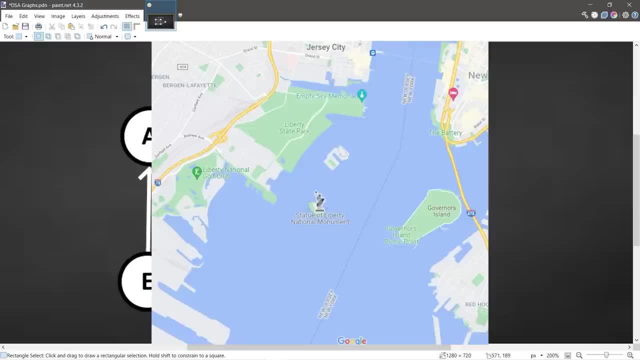 However, it is valid to have one node pointing to another node node and that node could point back to the previous node. An example of a directed graph could be a street map. Let's say you're working on a travel app and each node is: 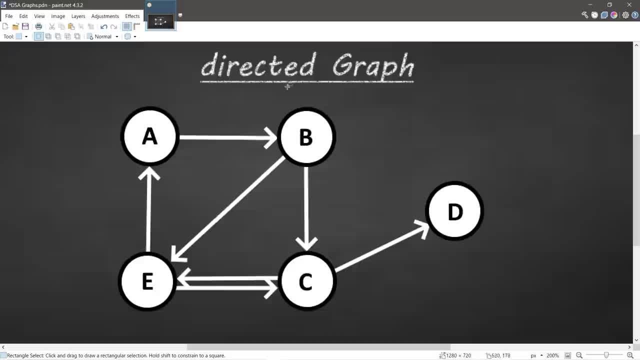 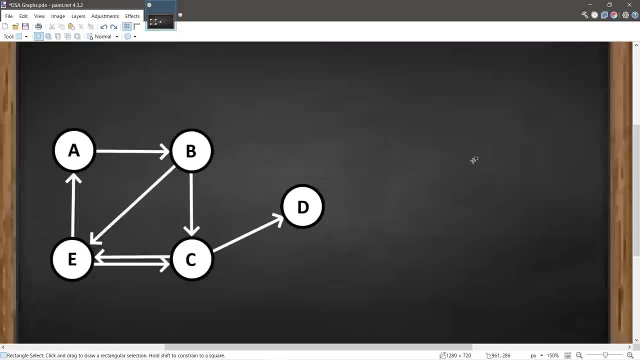 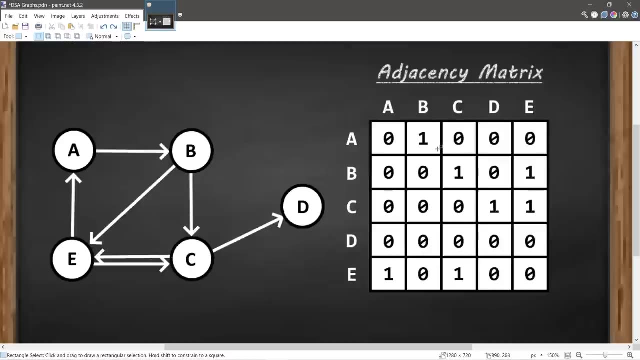 a possible destination. These single edges could be one-way streets and these double edges could be two-way streets. You can move back and forth between these two destinations. There are two popular ways to represent a graph: an adjacency matrix and an adjacency list. With an adjacency matrix, we could create a 2D array or 2D array list. One row and 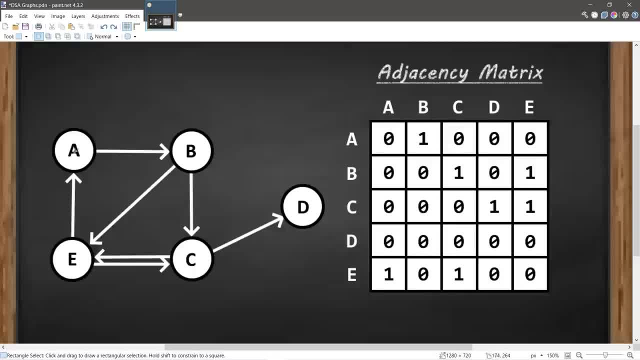 one column for each node. If we need to check to see if there's adjacency between two nodes, we would first find the index of the node we're beginning at, let's say A. So we would go to node A and then find the index of the node we're trying to travel to. so 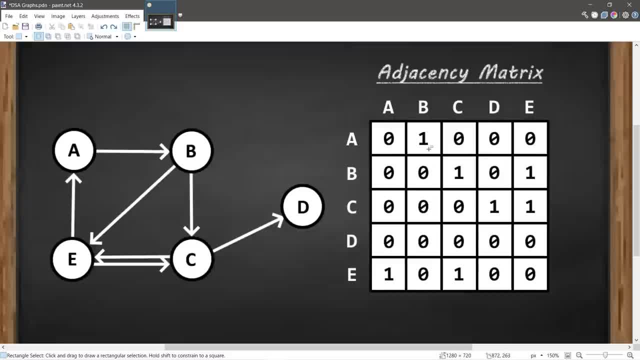 B. So row A, column B: If there are no edges, this would be zero. If there is an edge, this would be one. So since there's one here within row A, column B, well, there's adjacency from node A to node B, But if we take a look at row A, 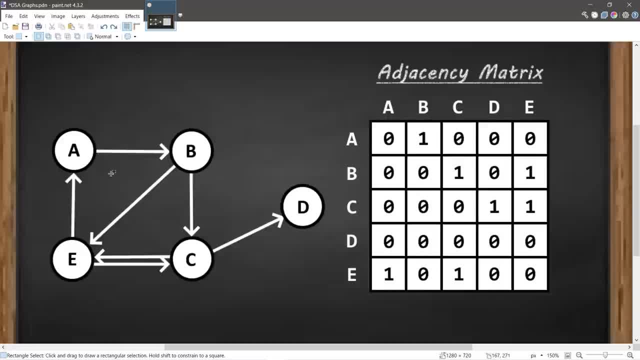 column C. this is zero, so there's no adjacency between A to C. But if there was, well, we would replace the zero with one. then Now there are pros and cons with the matrix. One of the benefits is that the runtime complexity to locate an edge is O. It's constant. All we have to do 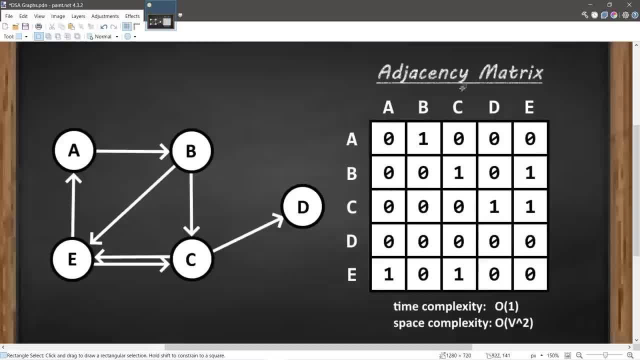 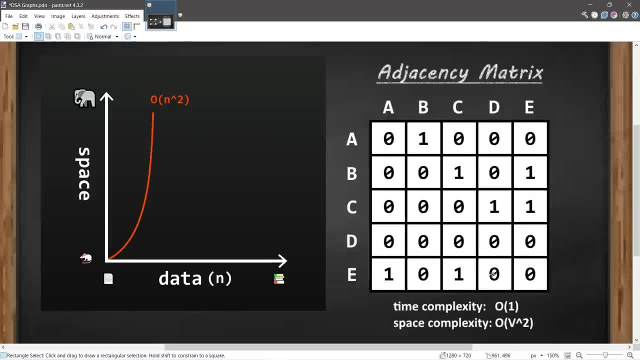 is find two indices, so we have to find the row and the column. However, the space complexity to store a matrix is O- V, as in the number of vertices that we have, But you could also think of that as n? n for the number of nodes, O, So. 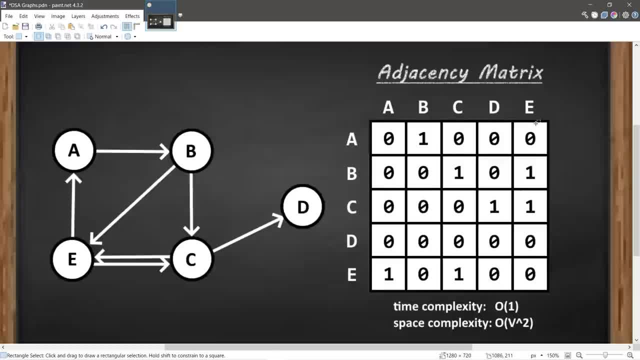 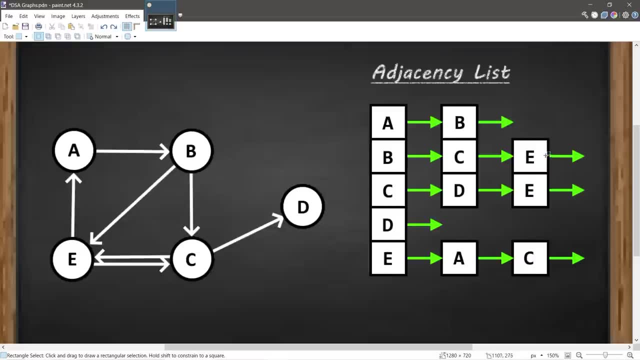 since we have 5 nodes and 5 columns, we would have a total of 25 spaces. So the benefits of a matrix is that it's very quick to look up an edge. however, a matrix uses a lot of room, So it tends to suit graphs that have a lot of edges. On the other hand, we have an adjacency list. 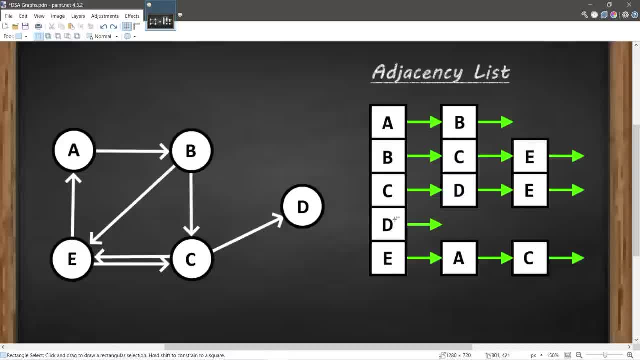 An adjacency list is an array or array list of linked lists. Each element is a separate linked list and each header within the linked list would contain the address of a node. If there's adjacency between one node and another, we would add the adjacent node to our linked list. So to 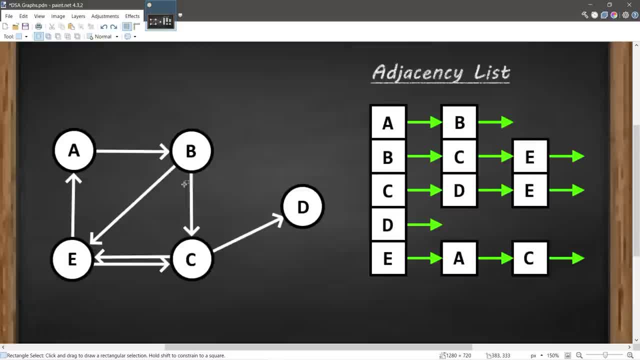 find adjacency between two nodes, we would find the node that we're starting at. let's see if B is adjacent to E. So we would locate index b and travel this linked list until we find the node that we're looking for. That means there's adjacency between nodes B and E. Even if there's. 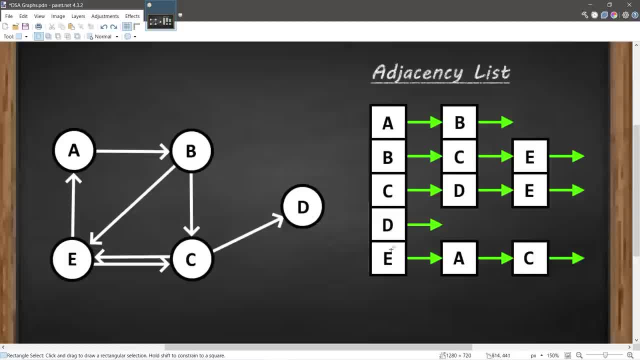 a node that is not adjacent to any neighbors, we would still want to add it to our adjacency list, just in case we do update it. Here are the pros and cons of an adjacency list. The time complexity to locate an element is big Oick. 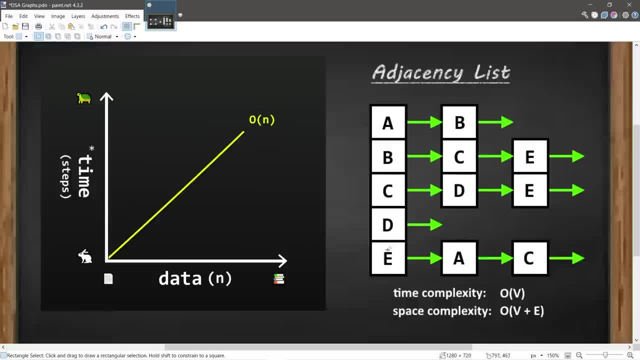 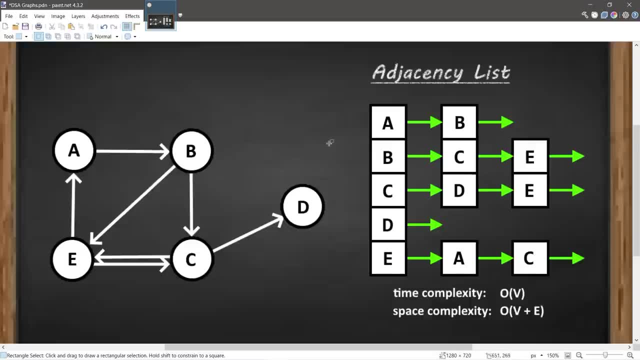 v, v, as in the number of vertices, You can also think of this as n, so this would be big O of n. To locate an edge, we would first access the node that we're beginning at by an index. So let's. 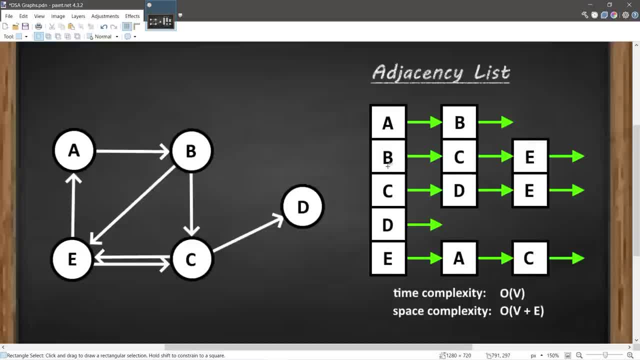 begin at b and we are looking for adjacency between b and e. Since each element is a linked list, we need to traverse this linked list linearly until we find the node that we're looking for. So in that way it's linear. However, a benefit of a list over a matrix is that they use less space. 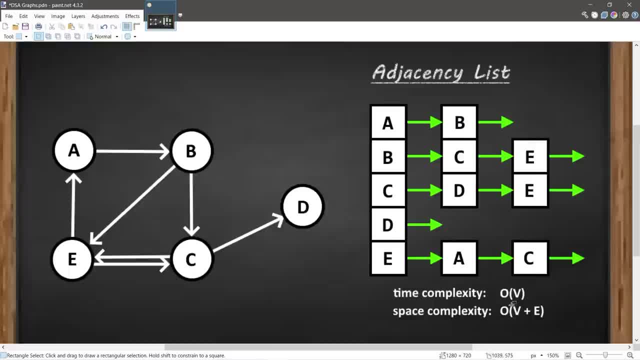 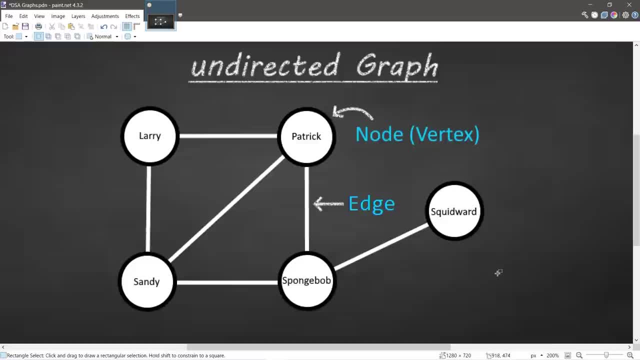 The space complexity of an adjacency list is big O of v plus e: v for the number of vertices, aka nodes, and e for the number of edges. So yeah, everybody, those are graphs. A graph can be used to model a network. Each node is a piece of data within our network and an edge connects nodes. 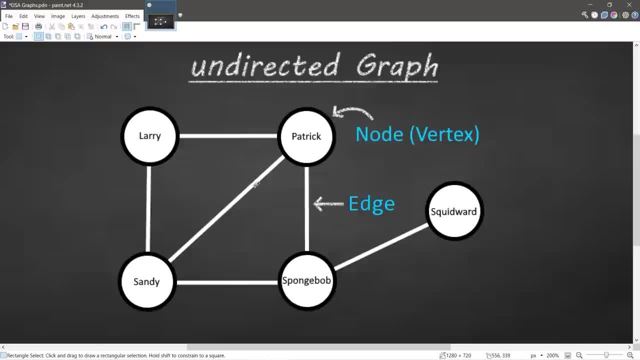 So, like I said, it's a popular way to model networks which don't necessarily have any sort of order. So, yeah, that's an intro to graphs and in the next two topics we'll create our own network. Hey, if you enjoyed this video, give it a thumbs up If you have any ideas of where else you could. 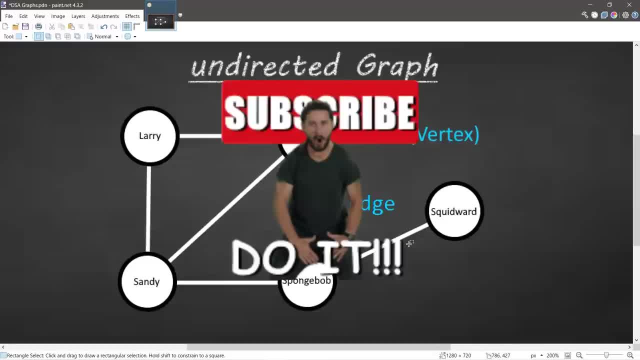 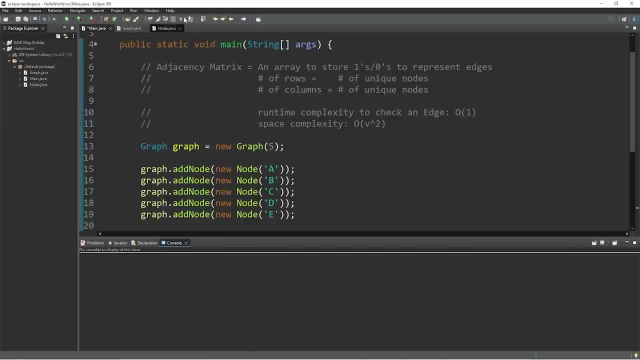 implement a graph, let me know in the comments section and, of course, subscribe if you'd like to become a fellow bro. Hey, yeah, everybody, it's your bro. hope you're doing well, and in this video I'm going to show you one way in which we can create an adjacency matrix in computer science. 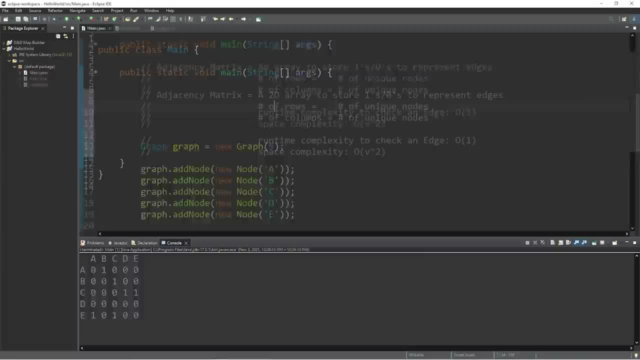 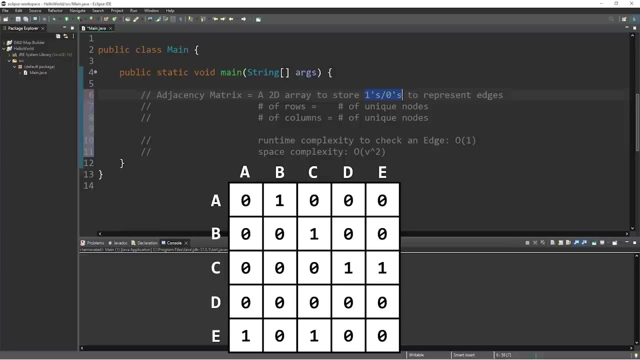 So sit back, relax and enjoy the show. Alright, people? so an adjacency matrix- An adjacency matrix is a function of the number of vertices in a network and it's a function of the number of vertices in a network. So an adjacency matrix is a 2D array to store ones and zeros to represent. 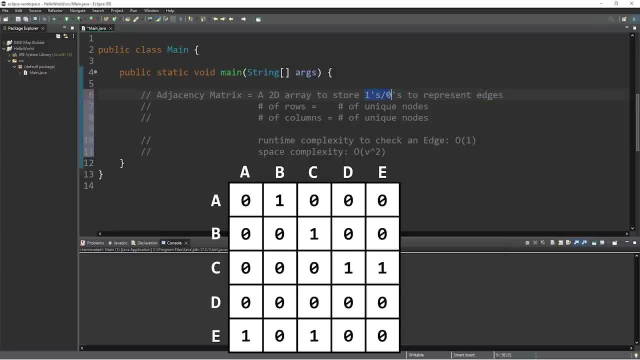 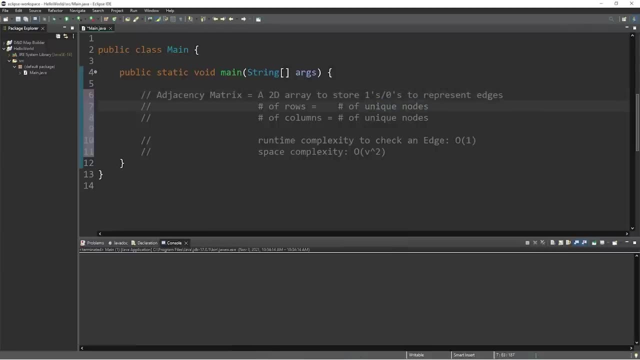 edges between nodes. There are different variations. You could use booleans so you could say true or false depending if there's an edge or not, And basically the number of rows and columns in an adjacency matrix is equal to the number of unique nodes. The runtime complexity to check an edge. 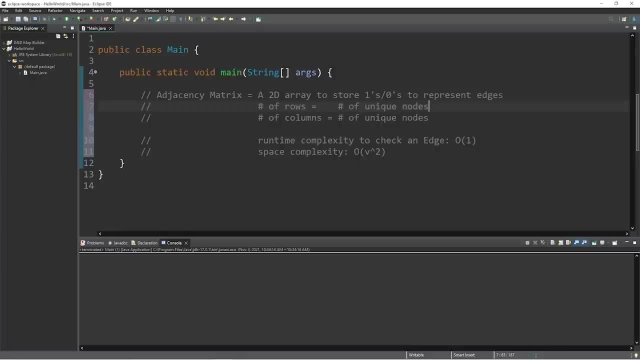 is big O of 1.. It's constant And the space complexity is big O of v squared, So it uses up a lot of space. Now let's create our own adjacency matrix. So let's create our own adjacency matrix. They're actually fairly simple. So I'm going to create two classes, graph and node. So file new. 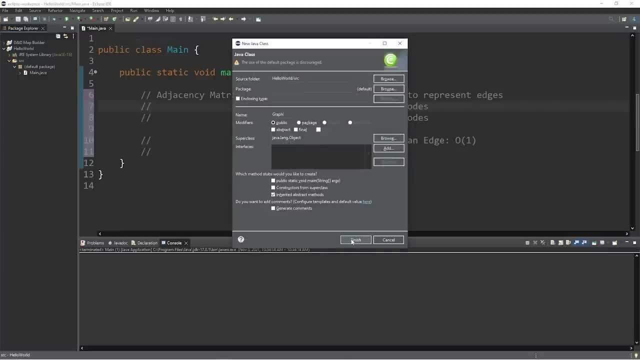 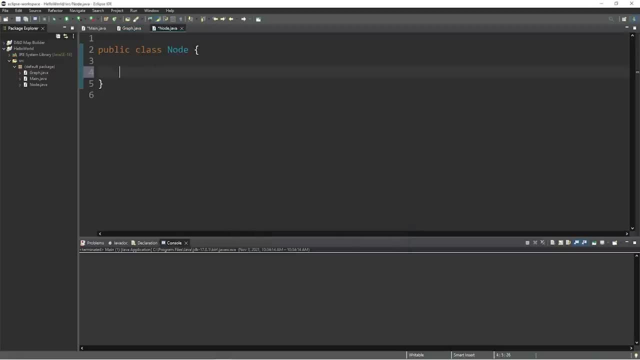 class. I will name this graph: Finish File, new class And I will name this class node. So let's say that each node has some data, maybe a single character, Char data, And I'll create a constructor Node will pass in some data when we create a node- Char data- This 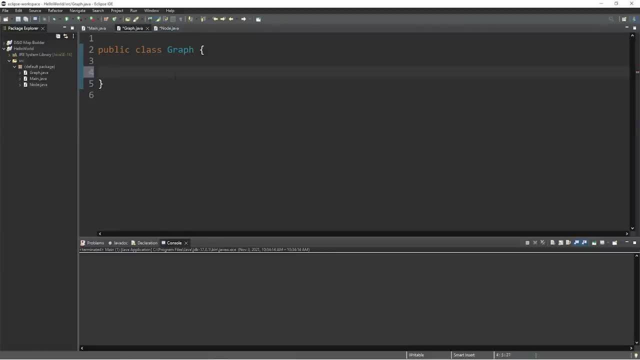 dot. data equals data Within the graph class. I'm going to declare a 2D array of integers, So integer 2D array And I will name this matrix And within the graph constructor we will instantiate our matrix. Matrix equals new int. Now we need to declare a size of this matrix. 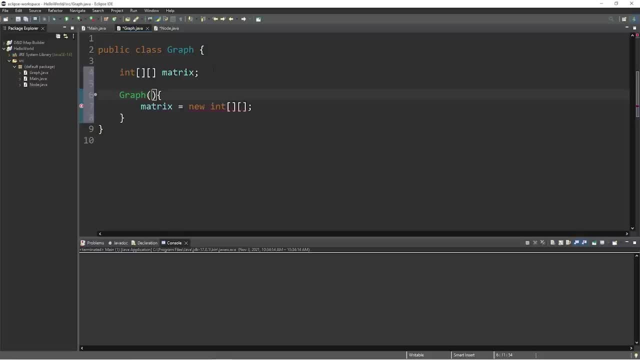 When we construct a graph object, let's set up a parameter, So int size. Size will be the amount of nodes that we have And the size of this 2D array will be size and size. That's why the space complexity is O, squared, It's the number of vertices squared. If we have 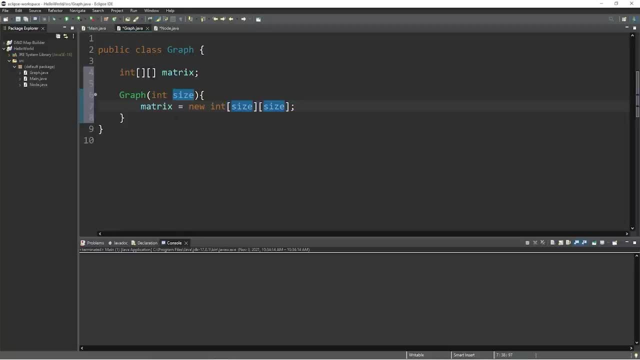 five nodes. well then, the size is going to be a total of 25 elements. Now let's declare a few methods: Public void- add node, And then we will pass in a node, Node, node And add edge. Public void- add edge. Then we need two indices: A source and a destination: Int source, Int destination. 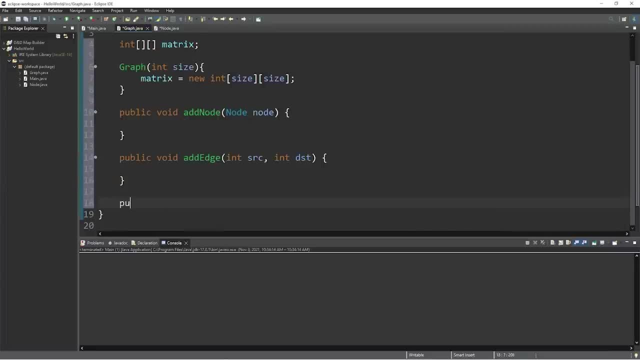 DST for short. We'll need a method to check an edge- Public- And this will return a Boolean value- Boolean check edge- And we'll need a source and a destination for parameters. And let's create a print method: Void print. 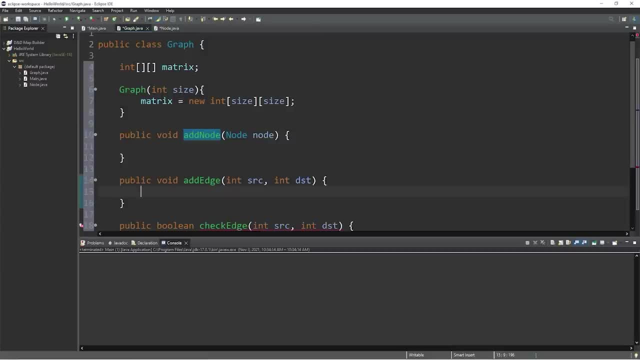 Okay, we'll fill in add a node a little bit Later. So let's fill in add edge. We will pass in a source and a destination, Two indices. So source will be the row, Destination will be the column. So what we're going to do is take our 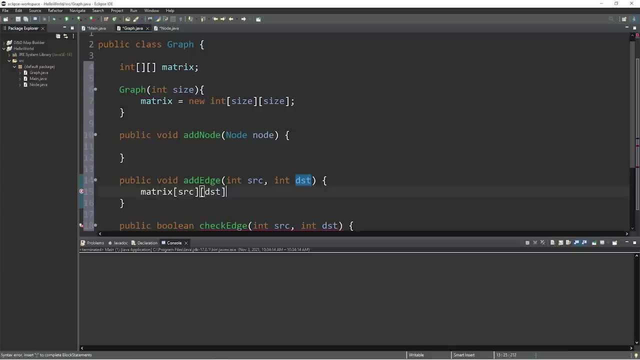 matrix at index of source and destination And set whatever value is in here Which will be zero Equal to one. That means there's an edge between two nodes And that's really it Within the check edge method. we're going to check within our matrix if a given value is equal to one. 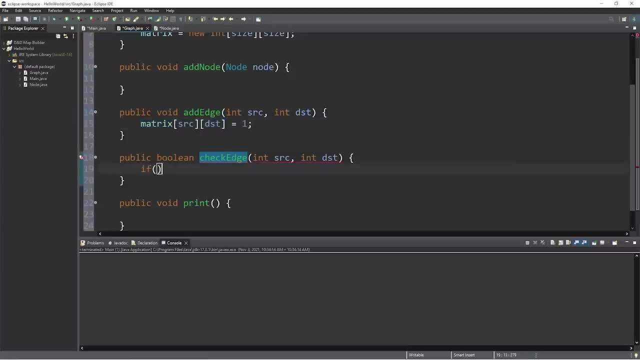 If it is, return true. If not, return false. So, using an if statement, let's check to see if matrix at index of source and destination is equal to one. That means there's an edge. If there is an edge, let's return true, Else we will return false And that's it Okay. Now before. 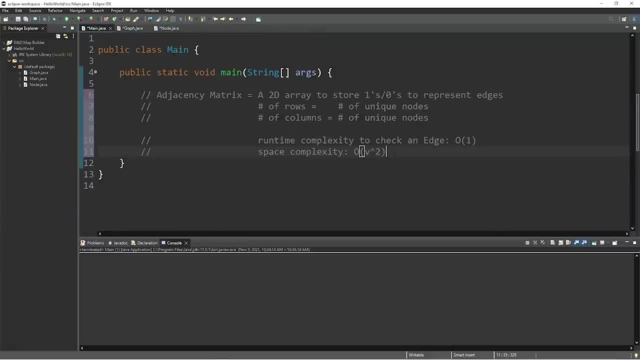 we actually print our graph, Let's actually create a graph. So let's get rid of this Graph. Graph, new graph, And we can add some nodes, although this method doesn't do anything quite yet, but it will in the future, And we need to pass in a size. so let's pass in five, We'll create. 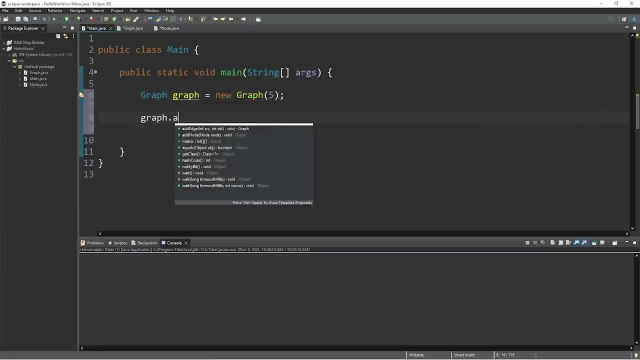 five nodes. So to add a node type graphaddNode- and this is a method that we created And I will pass in an anonymous node or you can use a named one, So we have new node. and then to create a node, we need to pass in some data, because that's what we decided on. So let's pass in the. 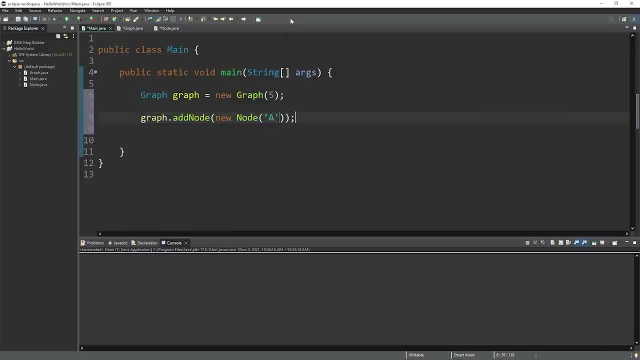 letter A. So this will be node A and we'll create a few more nodes- B, C, D and E, And we also can add edges between these nodes to represent adjacency, So to add an edge type: graphaddEdge. So what we're doing in this example, think of each node as having an index number. 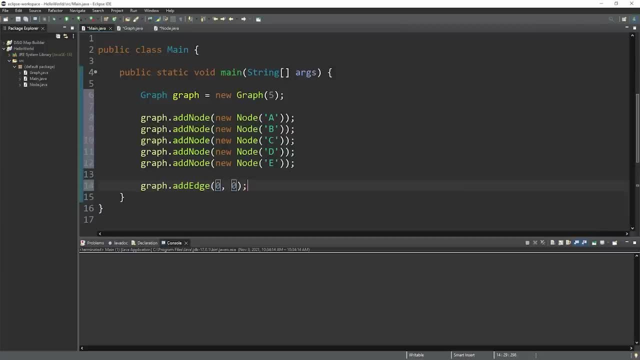 To create an edge type graphaddEdge. So to add an edge between two nodes, we will pass in the index number of each node. If I need an edge between nodes A and B, well, each of these has an index number within our 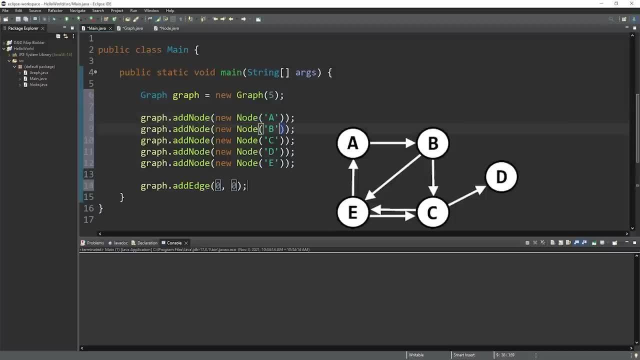 matrix. So this first node would have an index of 0, and the second node would have an index of 1.. If I need an edge between these two, I will add edge between 0 and 1.. And let's create a few. 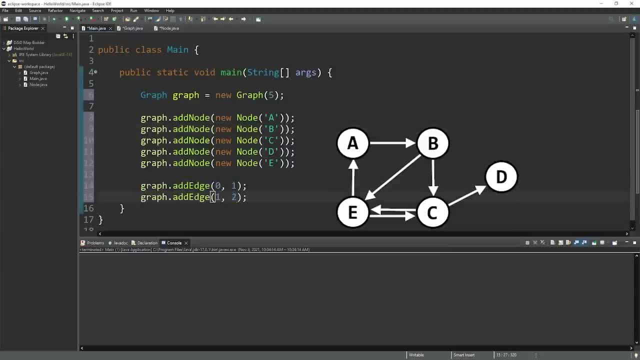 others. So how about B and C? So C would have an index of 2, and C will have two edges. based on the previous video, C will be connected to D, so 2 to 3, as well as E, so 2 and 4.. D won't have any edges. This is a. 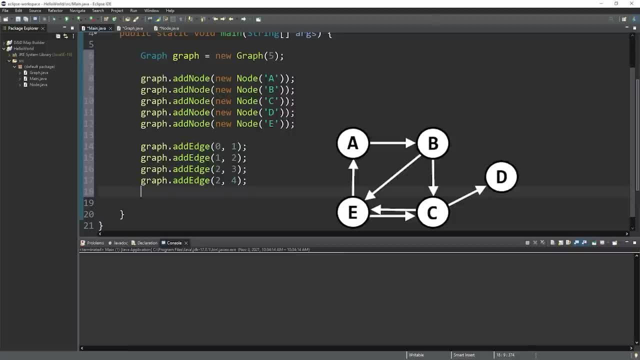 directed graph in this example, and E has two edges. We have E to A, that would be, 4 to 0, and E to C- 4 and 2.. Now let's print our graph, Graphprint, and we need to fill in this method. 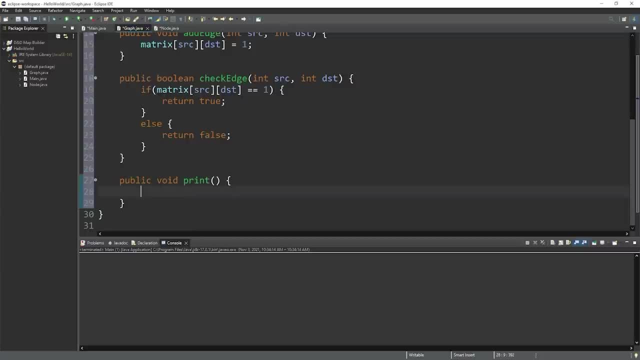 Within the print method of the graph class. we just have to print our 2D array and we can use for loops for that. So this will be the outer for loop: int i equals 0.. We will continue this as long as i is less than the length of our matrix. matrixlength. 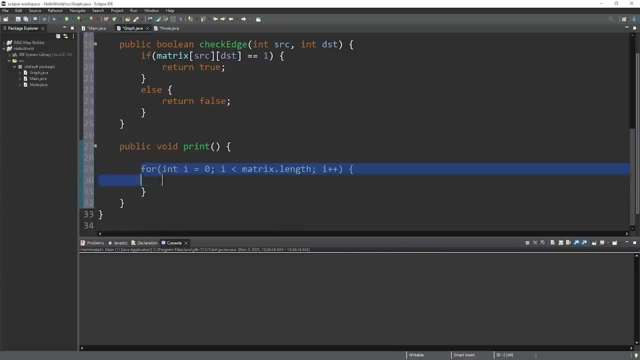 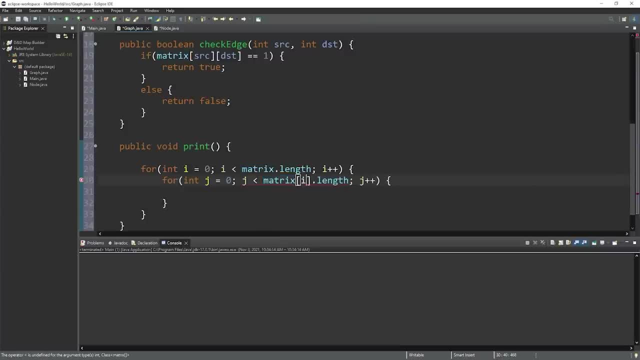 take matrix at index of ilength, this time as the stopping condition, and during each iteration of the inner for loop, I will use a print statement and I will print matrix at indices of i and j, Then I'll add a space between each of these. Oh, then, when you exit the inner for loop, let's print. 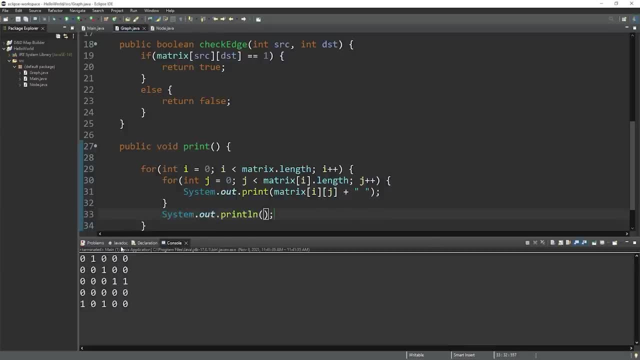 a new line. Okay, and here's our adjacency matrix. Each row corresponds to a node as well as each column. If there's adjacency between two nodes, well then there will be a one at that row and column. This next part really isn't necessary. This is kind of the general idea of an adjacency. 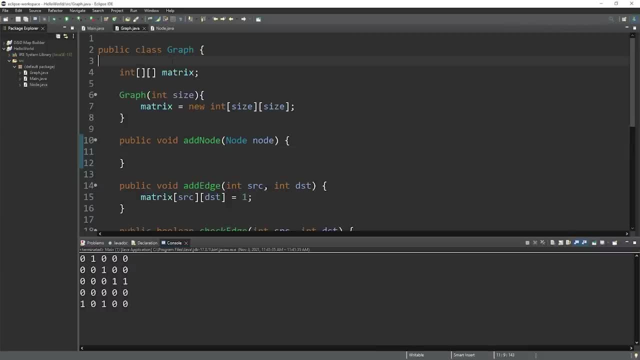 matrix, but let's add some headers to the rows and columns Within the graph class at the top. let's create an array list- Array list and the data type will be node and I will name this nodes. When we construct a graph object, let's instantiate our nodes. array list Nodes equals new. 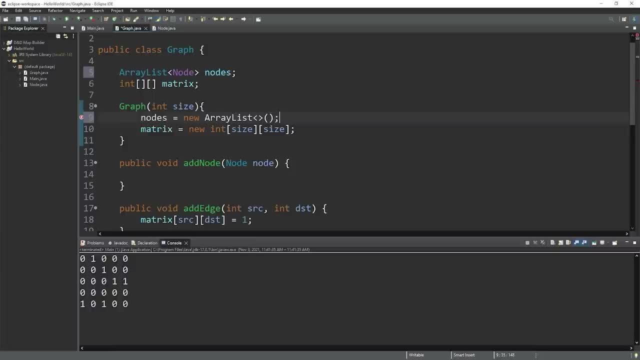 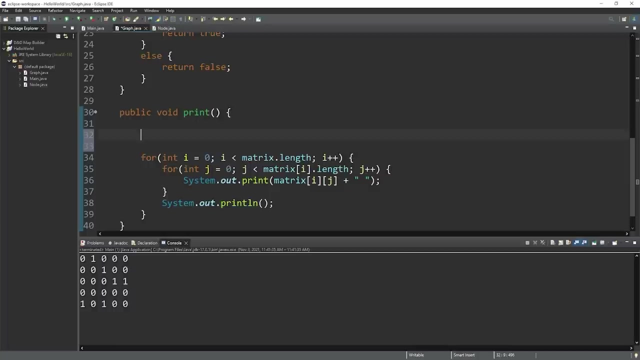 Array list and when we add a node, we just take our nodes- array list, dot add node- and within the print method, let's make a few changes. So, preceding our nested for loops, let's print the data found within each node, so it serves as a header and I can use a for each loop for this, For every node. 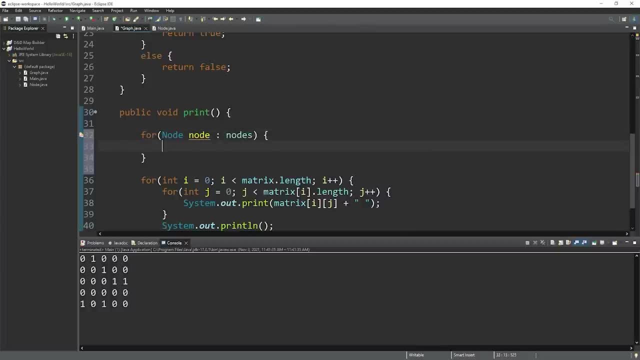 node in nodes, then let's print the data found within each node, and I can use a for each loop for this. So let's print the nodes data, then maybe I'll add a space. Oh, then add a new line. Okay. 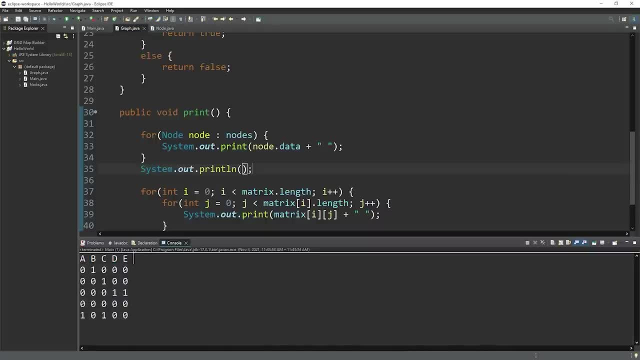 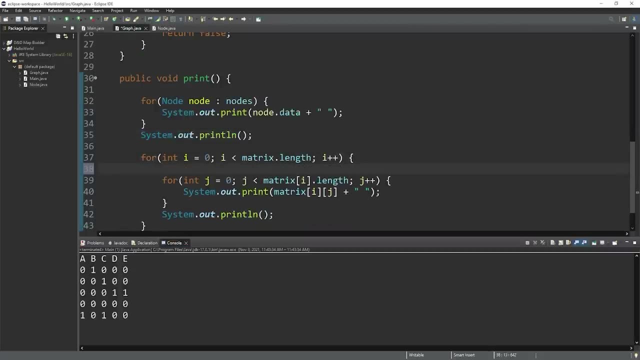 there we go. Each column has the data found within each node, and let's also do the same thing with each of these rows. I think it would look cool. Before the inner for loop, let's do the same thing. Let's copy this line, but this would be nodes dot. get index of i dot. 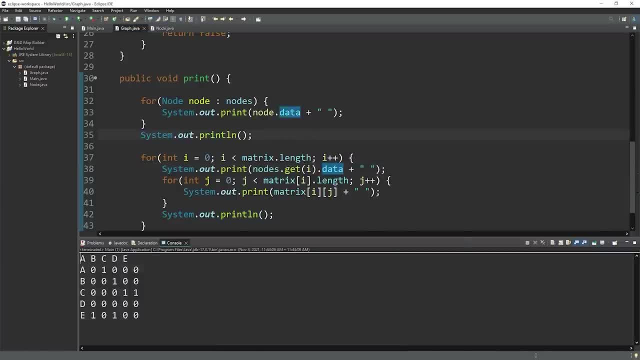 data and let's see how that looks. so far, Okay, not too bad, but let's add a few spaces. So system dot out, dot print and I'll just print two spaces. All right, there's our adjacency matrix. If you're working with more complex data, let's say city names, I would consider using 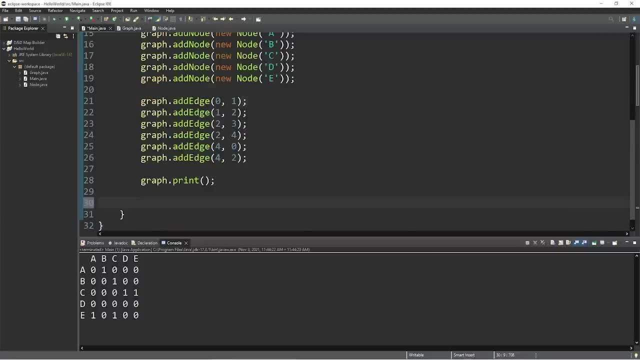 printf statements instead, because you can align things properly. And if you do want to check an edge, we did create a check edge method. So within a print line statement let's invoke the graph dot check edge method and then pass in two indices. So let's see if there's an edge between nodes a. 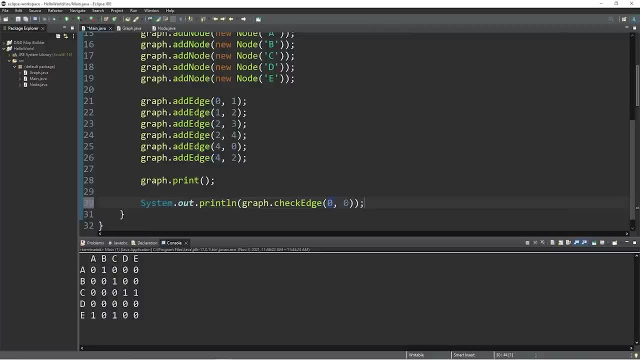 and b. So a has an index of zero, b has an index of one. there is an edge between these two, So this will return true, there is an edge This time. let's check to see if there's an edge between. 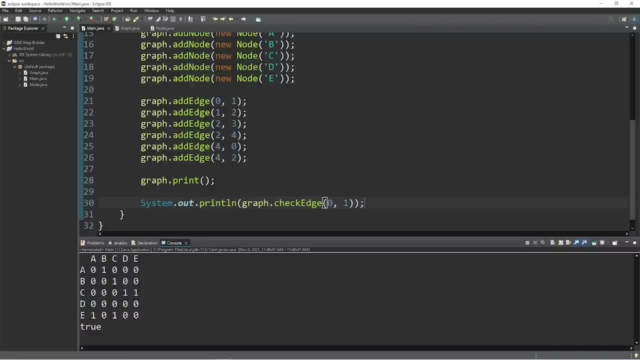 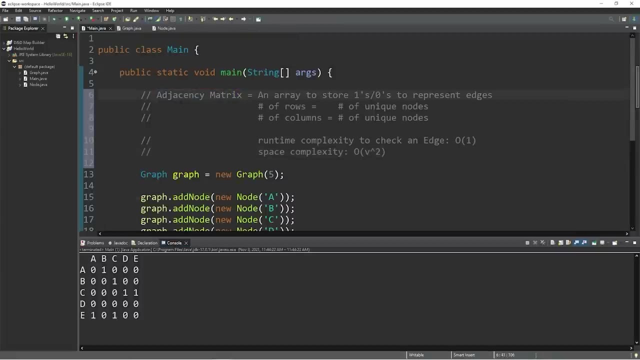 d and c. So d has an index of zero, one, two, three, And c has an index of two, And this returns false. there is no edge, All right people. so that's an adjacency matrix. It's an array to store ones and zeros, to represent edges, The number of rows and number of columns. 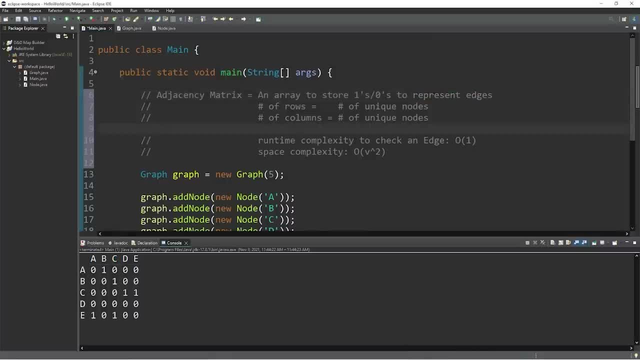 is equal to the number of unique nodes. The runtime complexity to check an edge is big O of one. all we need are two indices. However, the space complexity for an adjacency matrix is big O of v squared. Take the number of nodes you have and square it. So if I have five nodes, five squared. 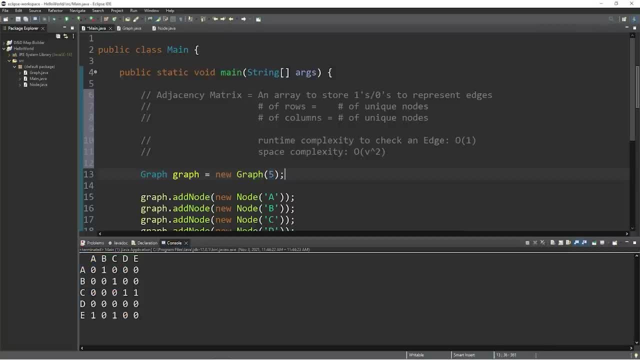 is 25.. We have 25 nodes. So if I have five nodes, five squared is 25.. So if I have five nodes, five squared is 25 elements. All right, so that's an adjacency matrix. If you would like a copy of this, 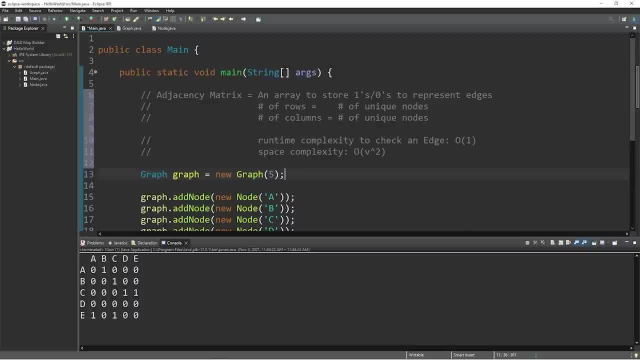 code. I'll post this to the comment section down below. And well, yeah, that's an adjacency matrix in computer science. Hey, what's going on? everybody, It's your bro, Hope you're doing well. And in this video I'm going to explain adjacency lists in computer science, So sit back. 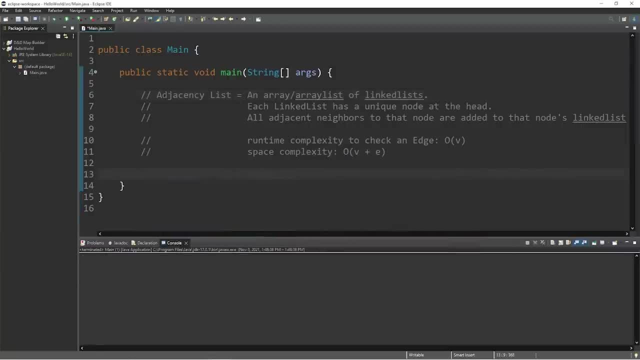 relax and enjoy the show. All right, what's going on everybody? Adjacency lists. An adjacency list is an array or an array list made up of linked lists. Each element is a separate linked list and each linked list can contain nodes And each linked 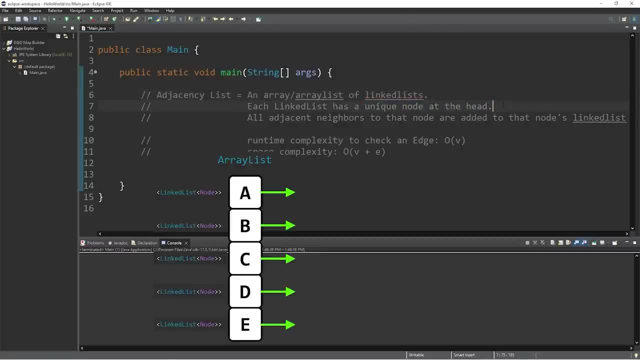 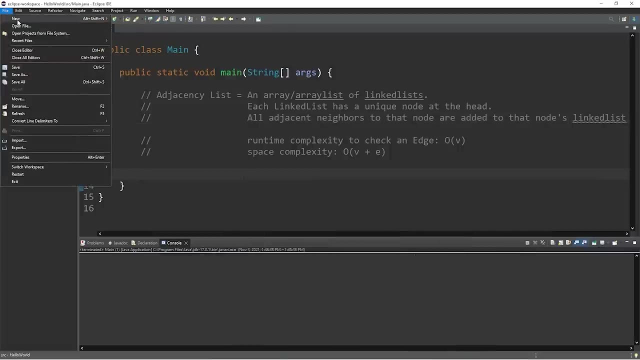 list has a unique node at the head And, basically, speaking, to represent a graph, all adjacent neighbors to a node are added to that node's linked list. If we add an edge, we just add the address of that node to the tail. So let's begin. Let's create two classes: graph and node File. 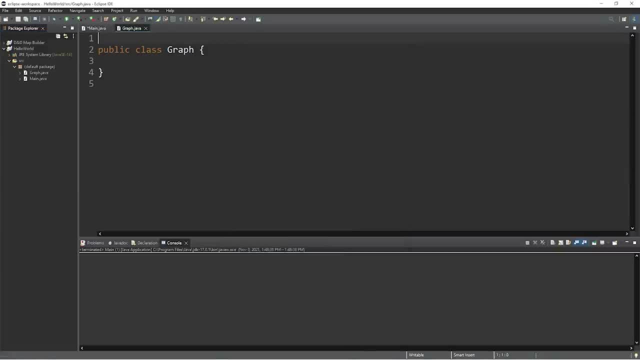 new class. This will be graph Finish, Then file new class node. Let's say we have some data, maybe just a single character, Char data- And we'll create a constructor And then pass in some data- Char data. Thisdata equals data. 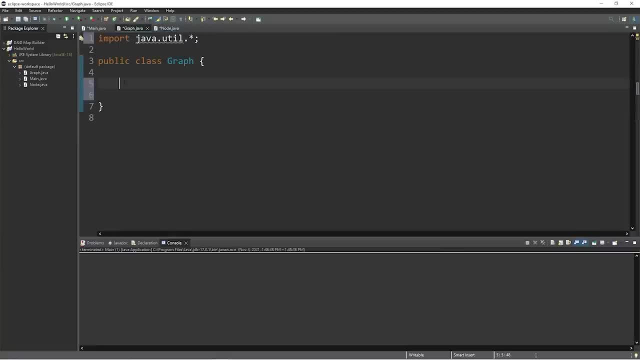 Within our graph class, we need to create an array list of linked lists. Array list And the data type of what's going to be stored are linked lists. What are the linked lists going to store? Well, they're going to store nodes. Let's name this array. 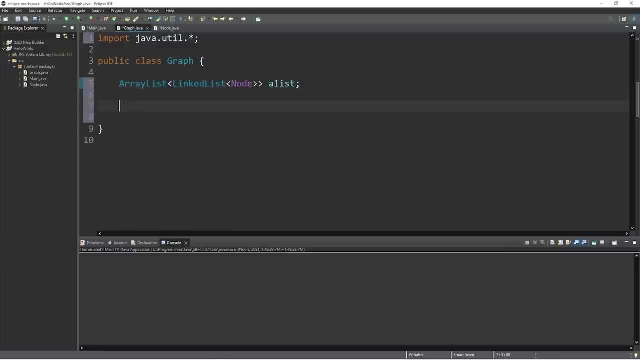 list, just alist for adjacency list. And let's create a graph constructor And we will instantiate our adjacency list. Alist equals new array list. Okay, let's declare some methods. We'll need an add node method, So public void- add node. 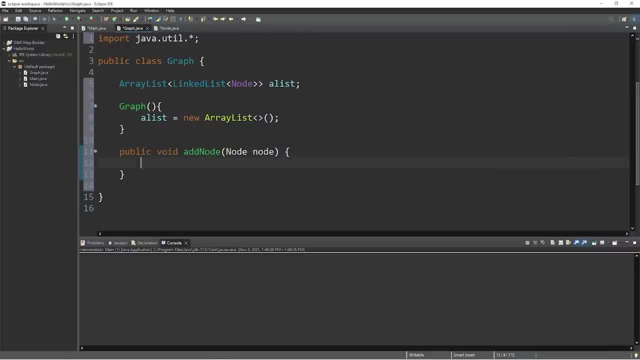 And there is one parameter, a node of the node data type. We'll need to add an edge Public void, add edge. We'll need two indices: a source and a destination: Int. source, int destination: We'll be able to check an edge Public void, check edge. Again, we'll need a source and destination indices And let's print. 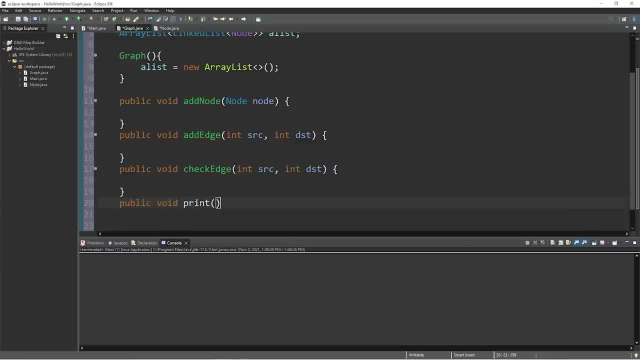 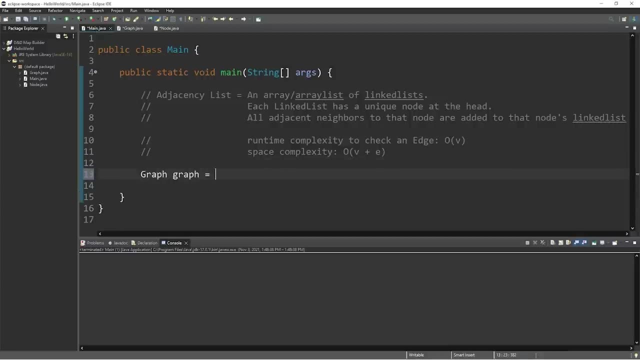 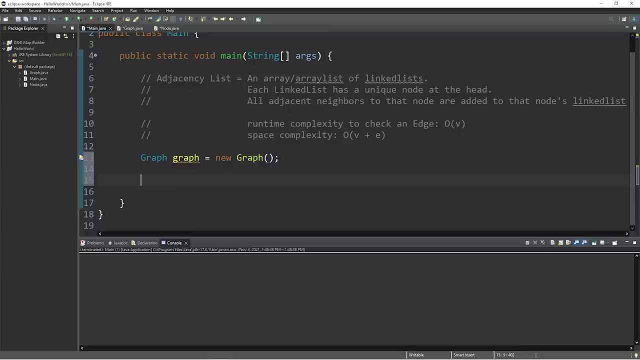 our graph. All right, now let's head to our main class and instantiate our graph. Graph graph equals new graph. We're going to reuse a lot of the same code from the previous topic on adjacency matrices, So let's add some nodes- Graphadd node- And I will pass in an anonymous node- New node- And we need some data. 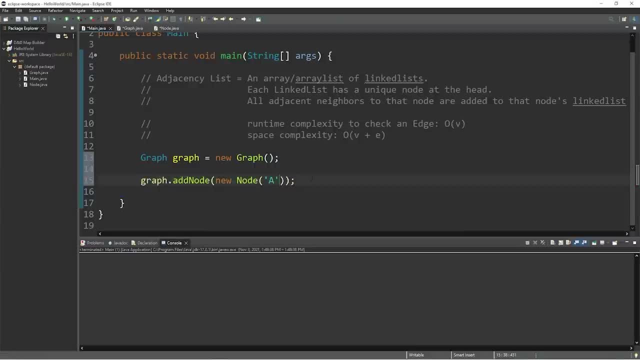 So let's pass in the letter A, Let's copy this and create public void add node. And we need some data. So let's pass in the letter A, Let's copy this and create public void add node. And we need some data. So let's pass in the letter A, Let's copy this and create. 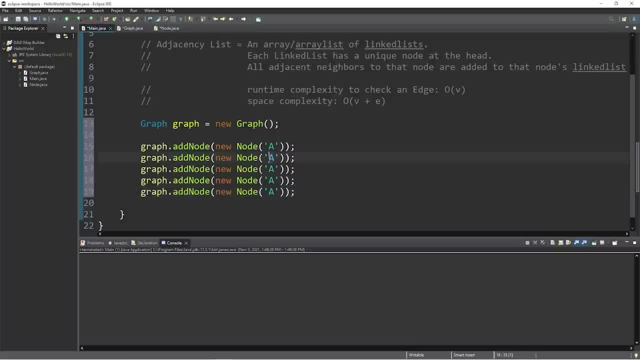 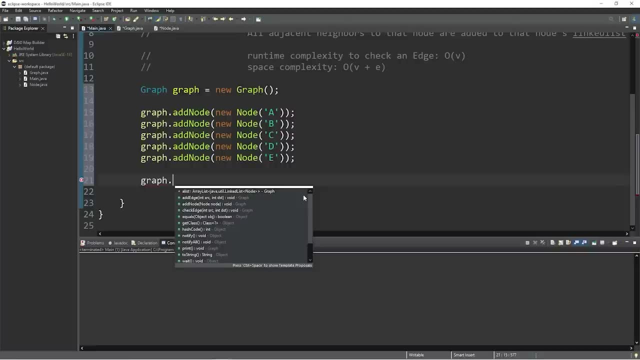 four additional nodes, So B, C, D and E, And we need to create some edges. Again, I'm using the edges from the previous topic, So graphadd edge. Each of these nodes has an index number. The first will be zero, The second will be one, then two, three, four. If I need an edge between nodes A, 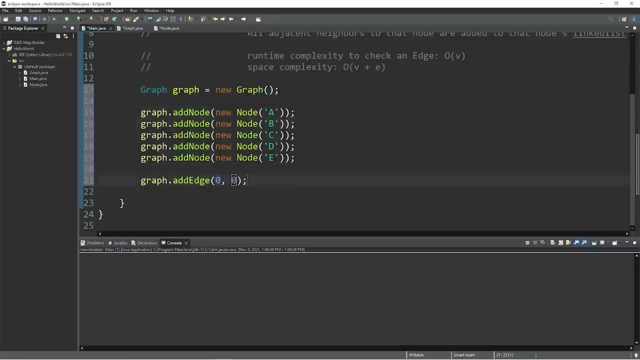 and B. the index in node A is zero. That's the source, And the destination is B, That has an index of one. So zero one. And let's fill in a few others. How about one and two, one and four? 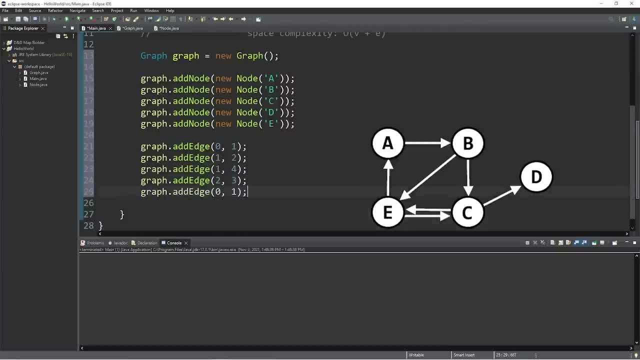 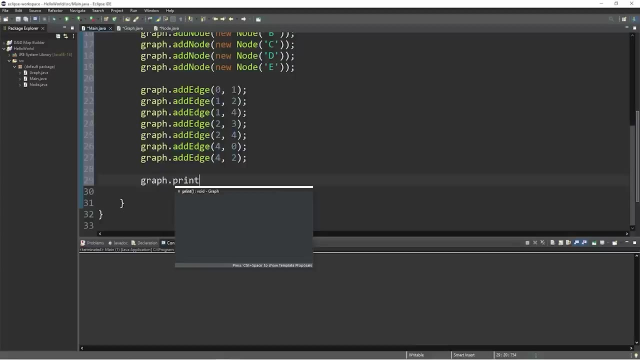 two, three, two, four, four zero and four two. Okay. So then at the end let's print our graph. But we have not yet filled in the methods, So graphprint Okay. So let's head to our graph class. 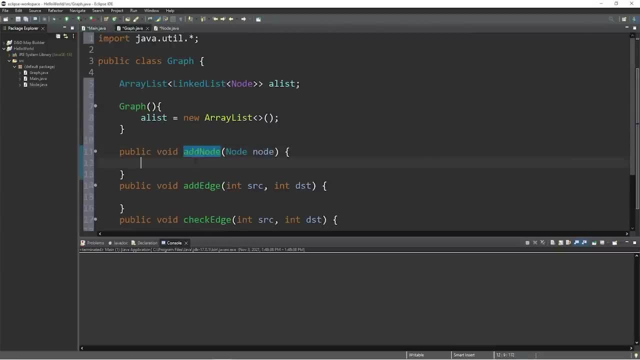 and fill in some of these methods. Let's begin with add node. So in order to add a node, we first need to create a new linked list, So linked list, the data type of this linked list is nodes, And let's name this. current list equals new linked list. After we create this new linked list, we can: 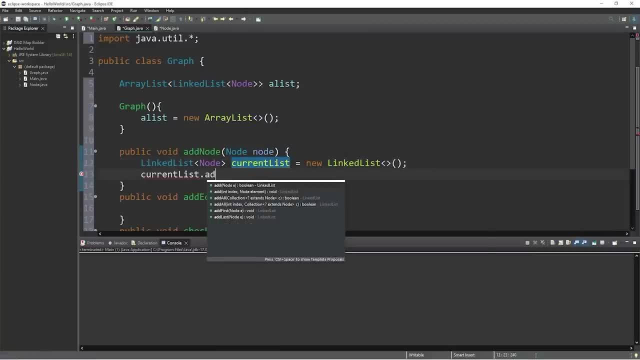 add a node to the list. So let's create a new linked list And let's name this current list And let's add a node to the linked list: Current list- dot- add node. Whenever we create a new node, we will also create a new linked list And the new node will be at the head of the linked list. And lastly, 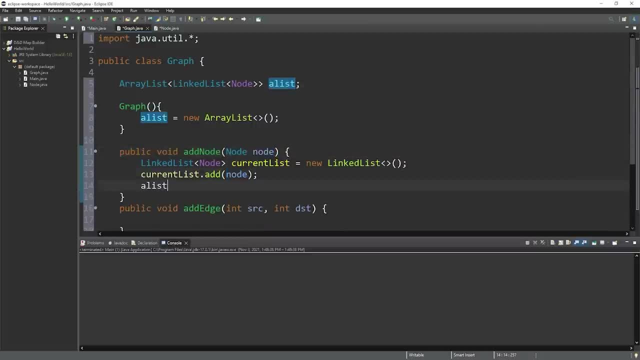 we just need to add this linked list to our array list. a list dot. add current list. Okay, then let's fill in the add edge method. I will declare a linked list And I'll just copy this linked list. current list equals to add an edge. 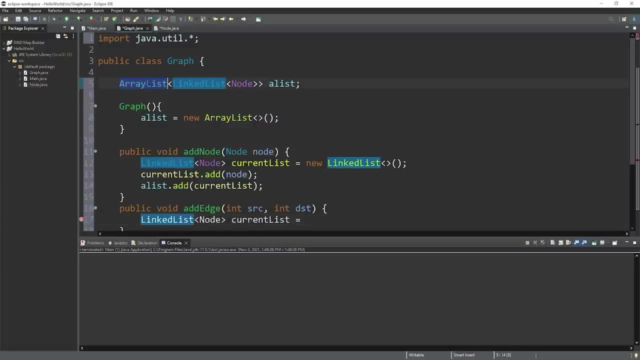 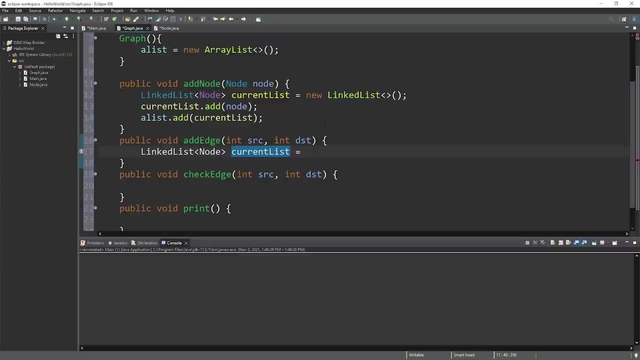 To our adjacency list. we first need to get a linked list from the array list. So let's store that within current list. current list equals to access our adjacency list. we will type a list dot get and then an index and that will be source. This will return a linked list. it's kind of like it's in two. 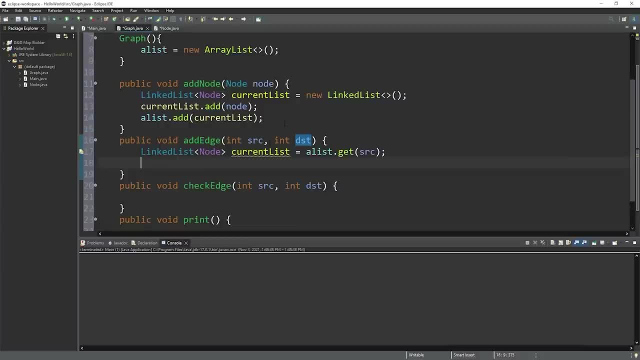 layers. we'll also need to know our destination node. So let's say node destination, node equals. then we'll need to find the array list that this node is located at. the head adjacency list, dot. get our destination index. then follow this with get zero. that is the head of our linked list. So this is the address of the. 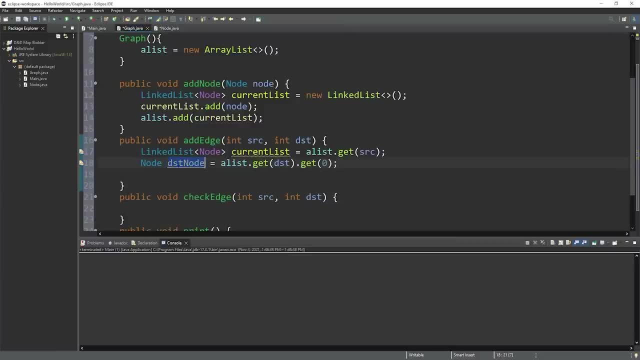 node we would like to link to, And now we just need to add this node to the tail of our current list. Current list: dot add destination node And that's it. we're taking a node and adding it to the tail of a linked list. you can shorten this code if you would like to do so in less steps. 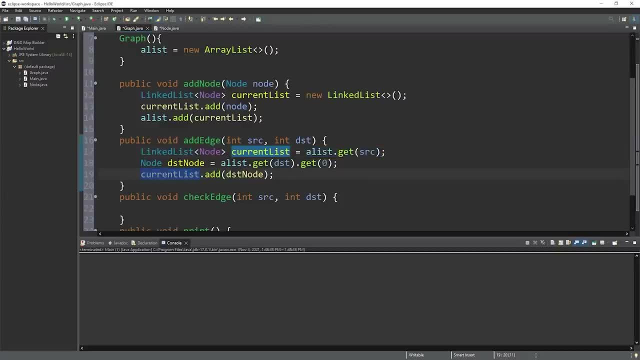 you would just take this portion and replace current list with a list dot, get source. then you technically don't need this line, But it's a little more difficult to read, So you do you. Okay, this time let's check an edge, So we can copy these two lines of code. 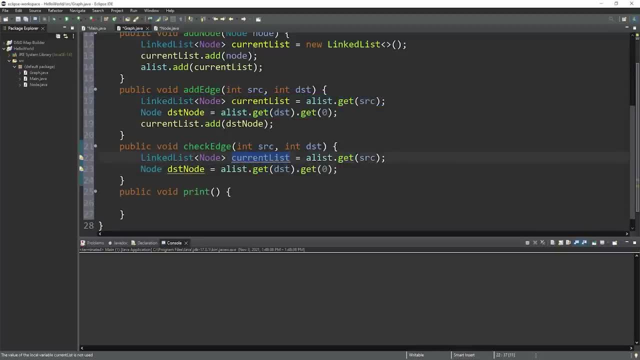 Paste it. What we're going to do is iterate over our current linked list and see if there's a match between a node and our destination node. So let's use a a for each loop and we will iterate over all of the nodes within our current linked list. So the 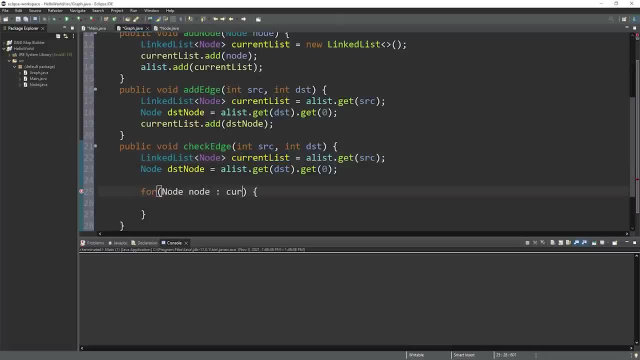 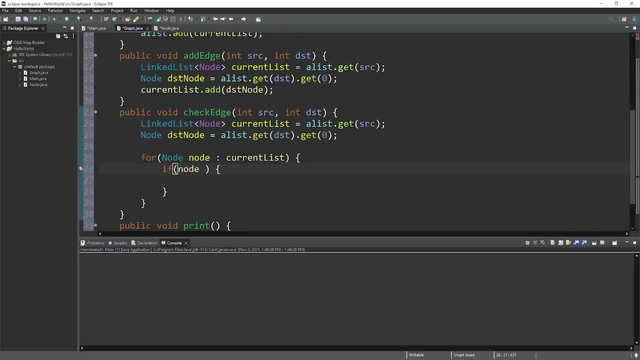 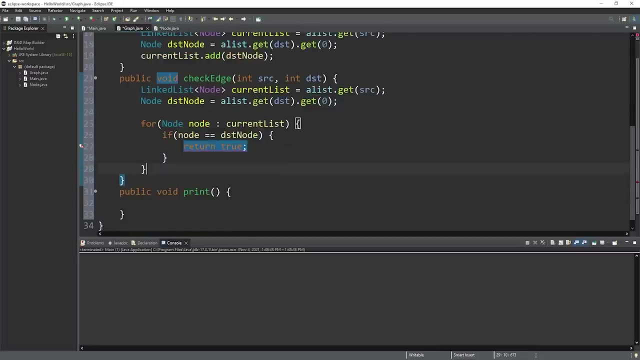 data type is node node in our current list With an if statement. let's check to see if the current node that we're looking at is equal to our destination node. Are these addresses the same? If so, then return true. If we escape the for loop, that means we did not find the node we 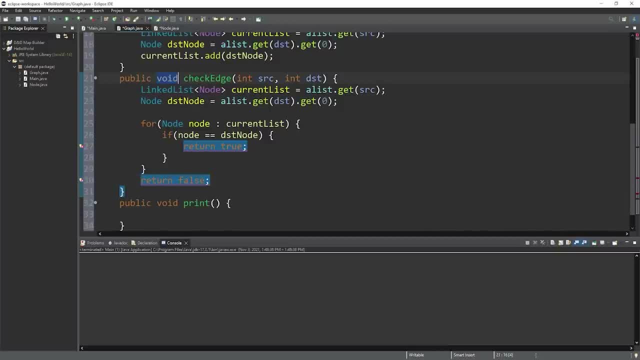 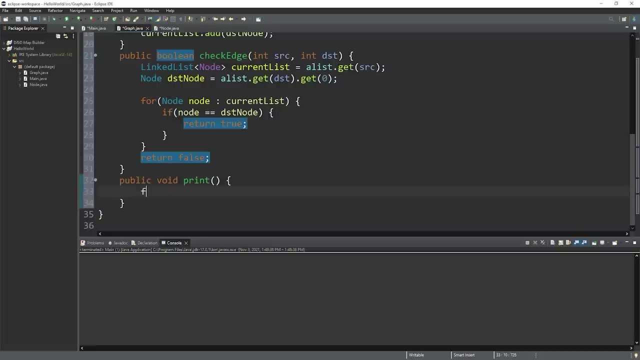 were looking for, so let's return false And the return type of this method is going to be boolean. Okay, we have one more method. We just need to print our adjacency list. We'll use nested for each loops, So we need to iterate over all of the linked lists within our array list. So for linked 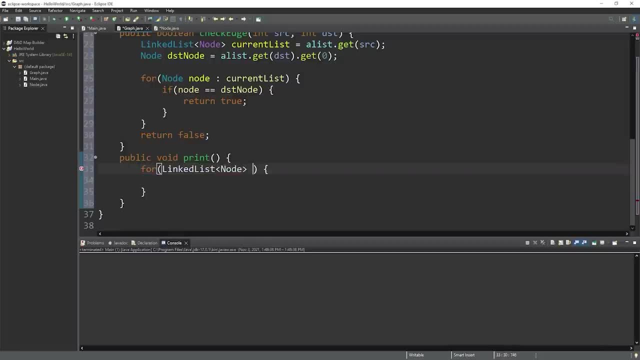 list, the data type is node and let's name this current list, Iterate over every linked list in our array list And then we'll need another for each loop, For every node, node in current list. Then let's use a print statement: Print the node's data. Then maybe I'll add an arrow for flavor to. 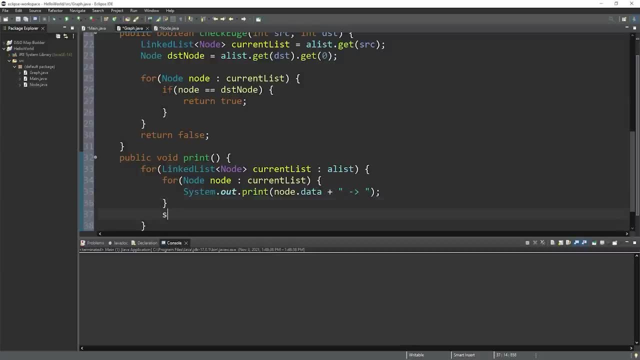 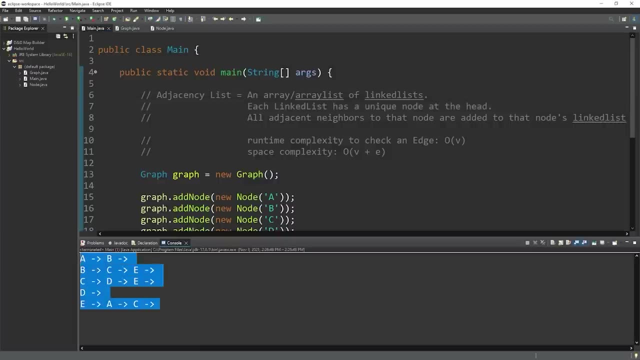 represent a linked list. Then, outside of our inner for loop, let's print a new line, And that should be everything that we need. So let's run this Alright. so there is our adjacency list. Basically, an adjacency list is an array or an array list made up of linked lists. Each linked list has a unique. 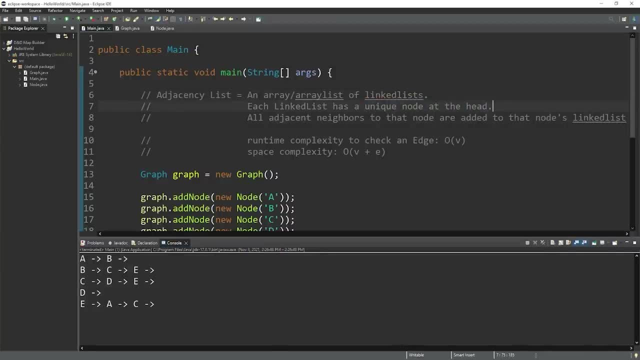 node at the head And all adjacent neighbors to that node are added to the node's linked list at the tail. The runtime complexity to check an edge is O v for the number of vertices. It's because we need to traverse a linked list linearly to find a matching node And the space 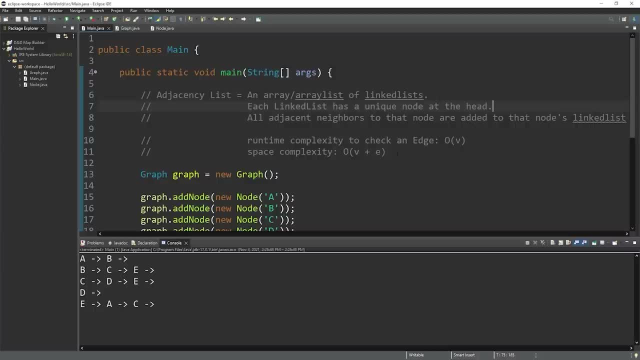 complexity for an adjacency list is O, v as in the number of vertices, e as in the number of edges. So, yeah, that's an adjacency list. It's an array, or an array list made up of linked lists. It's used to represent a graph. If you would like a copy of this code, 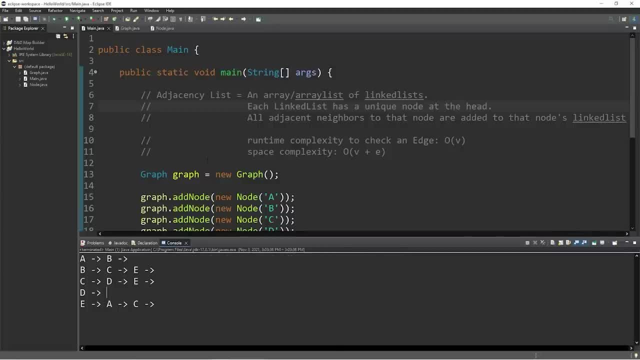 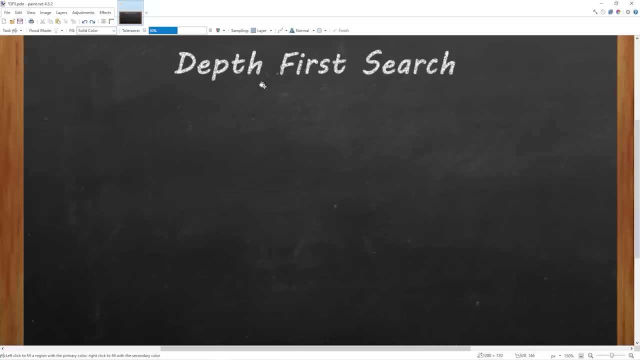 I'll post this at the comment section down below. And well, yeah, those are adjacency lists in computer science. Alright, everybody. depth-first search- Depth-first search- is a search algorithm for traversing a tree or graph data structure. We can break this down into three steps. When navigating a graph, we will pick a route And we 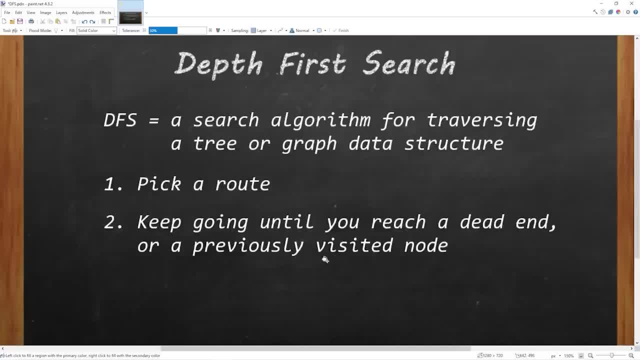 we will keep on going until we reach a dead end or a previously visited node. If we do, then we will move on to step three. We will backtrack to the last node that has unvisited adjacent neighbors. Let's navigate this maze using a depth first search approach. Here's the entrance and here's. 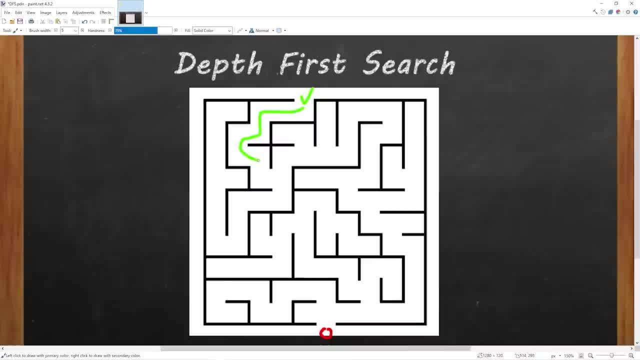 the exit. So the general concept of a depth first search is that when we reach more than one adjacent neighbor, we're just going to pick a route. Let's say we prefer right turns over left turns. but you can really set any rule that you want When faced with more than one adjacent neighbor. I'm just 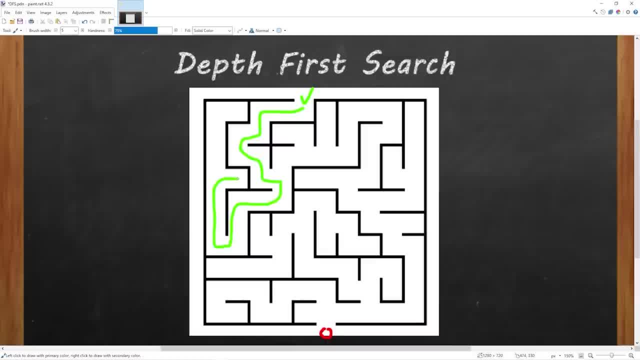 going to pick a route and keep on going, And if we reach a dead end then we're just going to backtrack to a node that has some unvisited adjacent neighbors, So there's no more place we can go. So we're going to backtrack all the way back to this intersection, right here, This route. 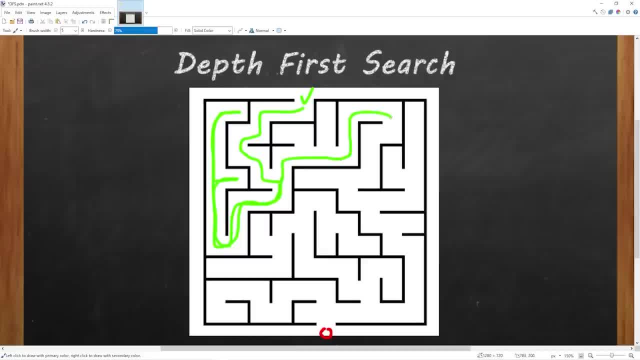 is unvisited, so we will continue going, Not backtracking yet There's no dead ends, but now there is. So we backtrack and keep on going. So this is what this looks like, sped up, And we have reached the end. Let's use a depth first search approach to navigate this graph. 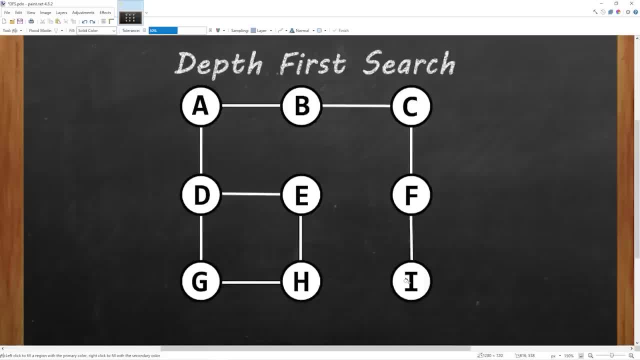 Maybe we're at node A and we need to travel to I, but we don't know where I is. One way in which we can keep track of our position is to use a stack, or we can use a stack to navigate to I. 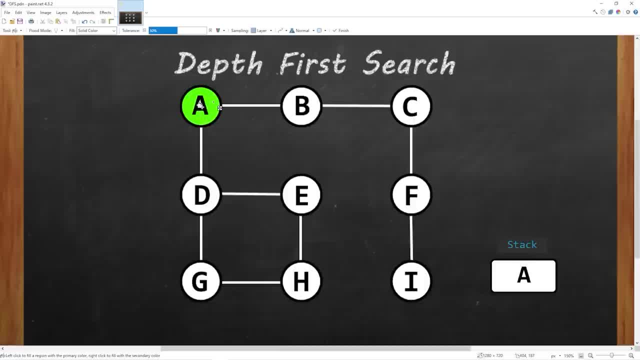 Or, in the case of recursion, we can use a call stack. Whenever we visit a node, we will push it onto the stack. We can either travel to nodes B or D, So we will mark D as visited and push this node onto the stack. Then we can either go to E or G. Let's go to G. 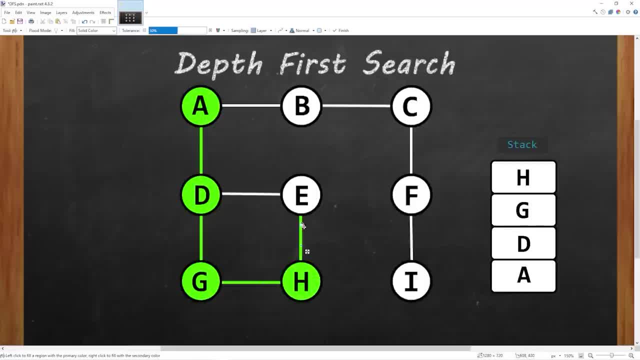 We'll push that onto the stack. Then H, E, And now we circled around back to D, but D is already marked as visited, So we're going to backtrack to a node that has unvisited adjacent neighbors, which is A. 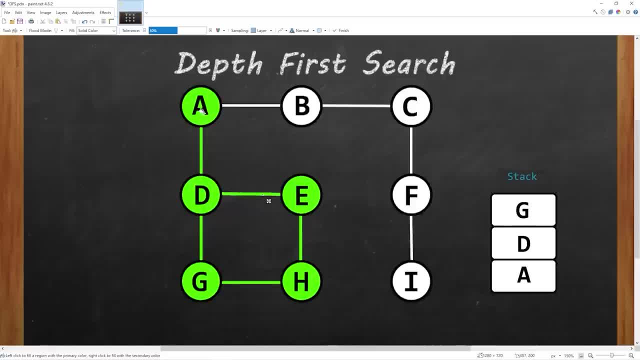 So we will pop all of these nodes off of the stack all the way back to A, which has unvisited adjacent neighbors, And this time we will go down this route and push all of these nodes onto our stack And we have reached the end Using a depth first search approach. when simplified, you pick. 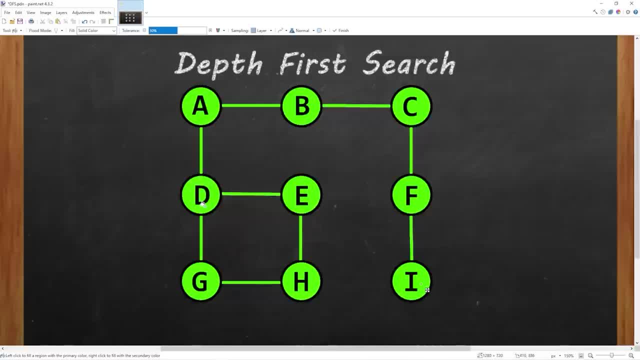 a route you keep going. When you reach a dead end or a node you already visited, you backtrack to a node that has unvisited adjacent neighbors And you repeat steps one through two. All right, well, let's implement this in code now, And here we are people, So I'm going to be using a graph that. 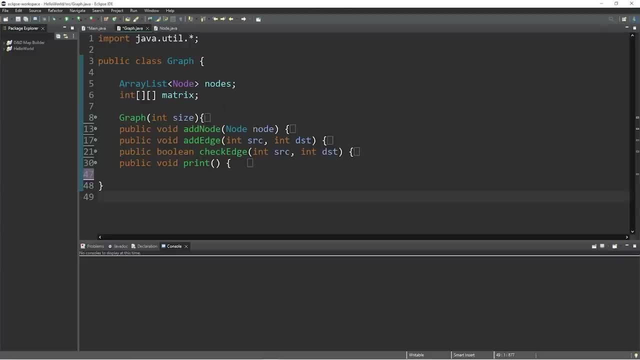 utilizes an adjacency matrix. If you're using an adjacency list, the code's just going to be a little bit different, But the concept is really still the same. I'm using code from the previous few videos. we have a node class, a graph class And in the previous videos we've already populated. 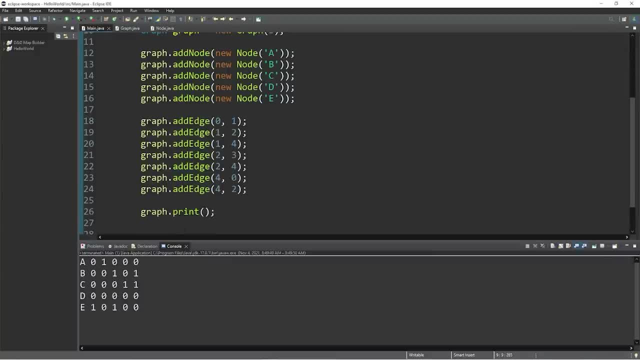 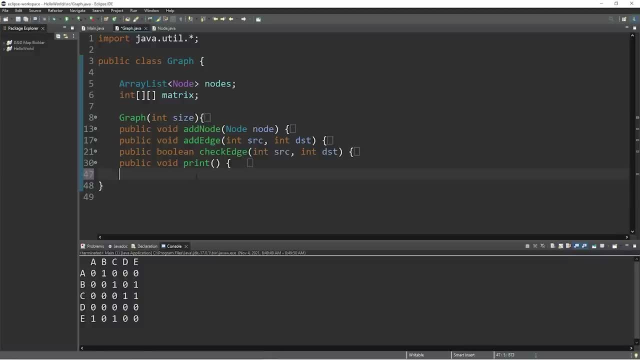 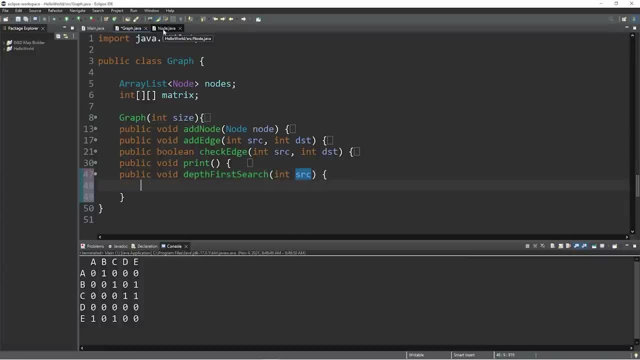 To keep track of the nodes that we've already visited. what some people like to do is that they will create a Boolean within their node class, such as Boolean visited, and they'll just mark it as false or true. However, it's very easy to forget to change. 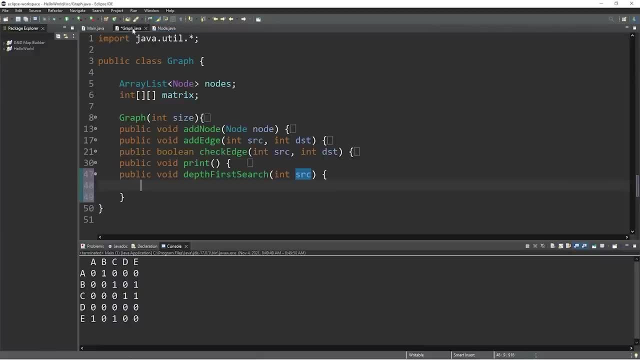 these back to false when you exit the depth first search. So what I'm going to do instead is create an array of Booleans, and the size will be equal to the length of the matrix. So let's create a Boolean array And I will name this: visited equals new Boolean. 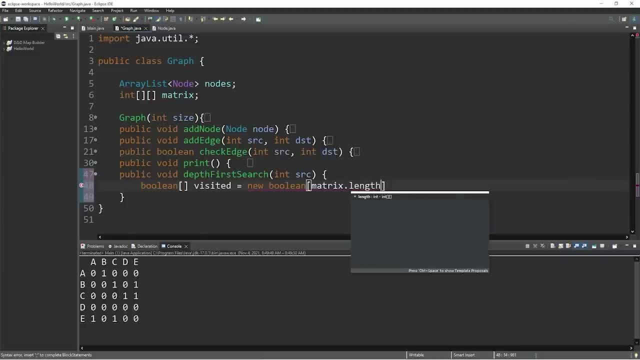 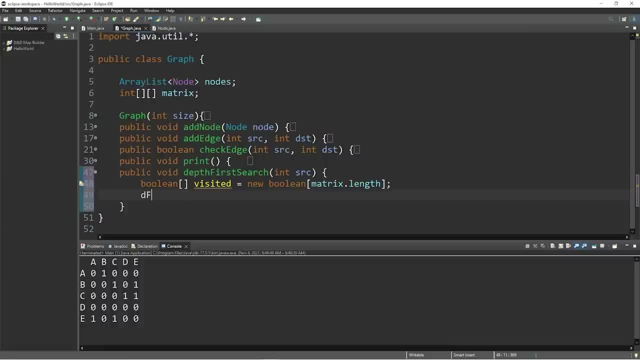 And the size of our array is the length of our matrix. Then, lastly, we will implement a helper function, So let's name this DFS helper And we will pass in our source and our Boolean array visited. Then we just need to create this. 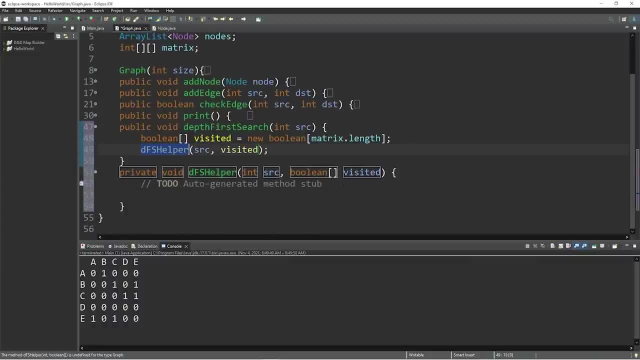 method, private void, DFS helper, And there are two parameters: int source and an array of Booleans named visited. You can either implement a depth first search iteratively using a stack or you can utilize the call stack if you use recursion In this example. 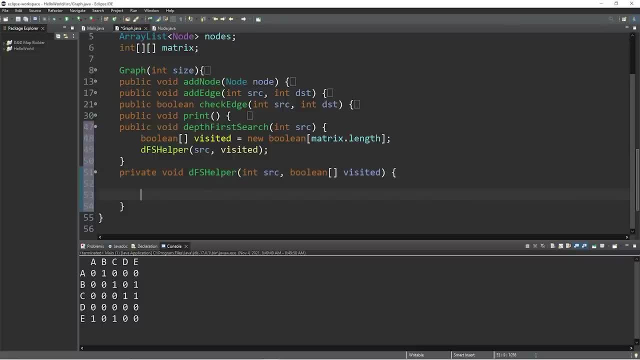 we're going to use recursion. When we invoke this helper function, we're going to check to see if the current node that we're on is visited or not. We can use an if statement If our visited array at index of source is equal to true. 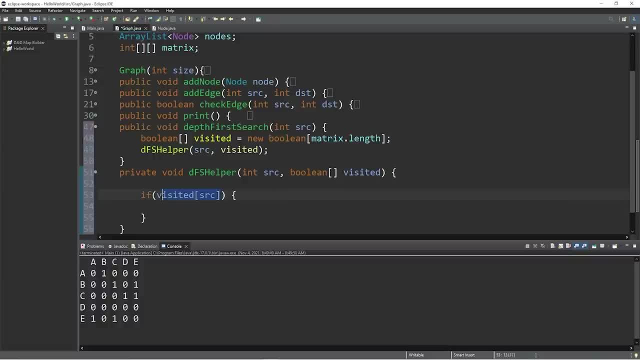 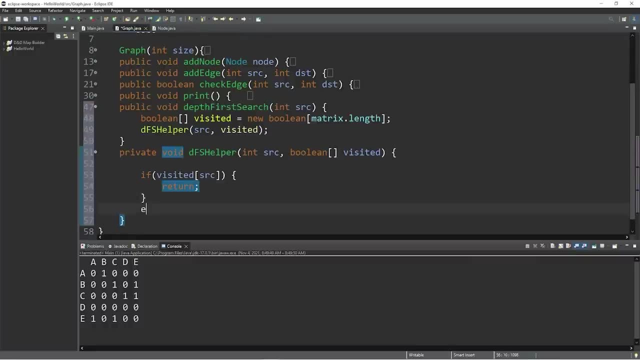 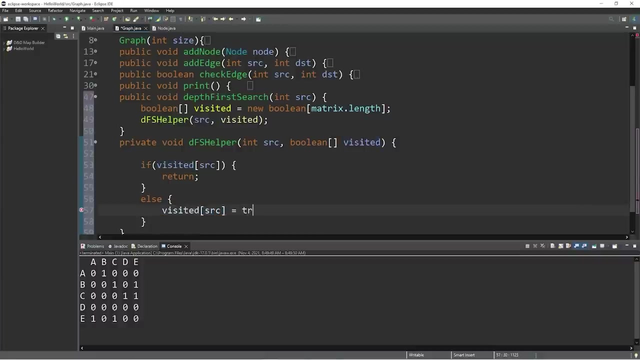 Or you could write the shorthand and just say if visited at index of source, since this returns a Boolean value. If we've already visited this node, we're going to return, else We will mark this node as visited Else. visited at index of source equals true, If you would like, although this part's not necessary. 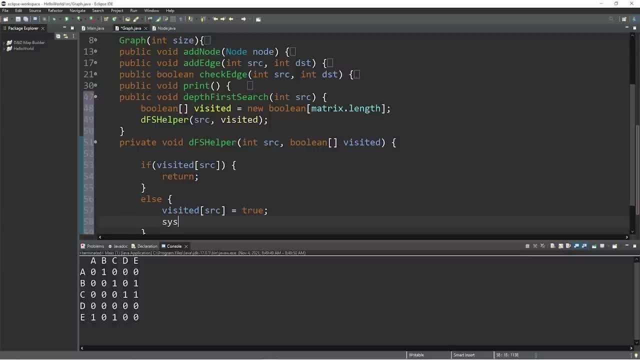 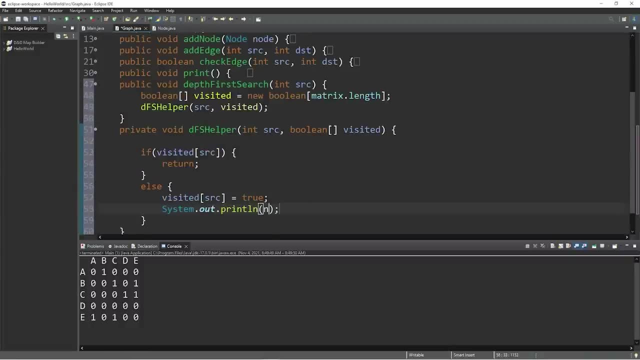 within my console. I'm just going to print that we visited this node. So within a print line statement I do have my nodes within an array list. I'm just going to access the data of one of these Nodes: dot. get source dot data plus equals visited. This part technically isn't necessary. 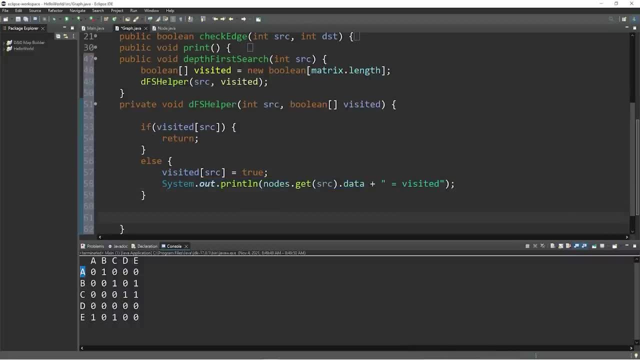 but it's going to help with my demonstration. In this example, maybe we start at node A. We need to find any adjacent neighbors. If we're using an adjacent neighbor, if we're using an adjacency matrix, we need to iterate over this row. We can use a for loop for that. 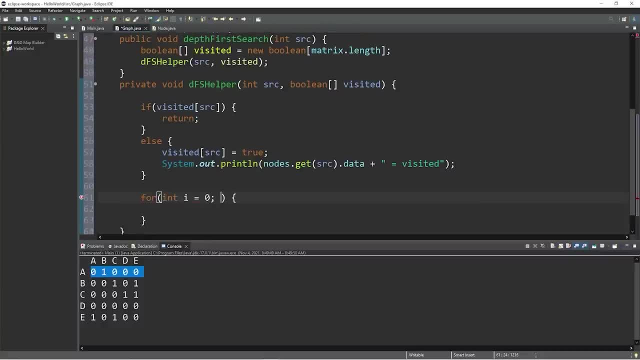 So int i equals zero. We will continue this as long as I is less than R matrix at index of source dotlength. This equals the length of a row And then increment i by one. We're checking to see if one of these elements is a one, That means that's an adjacent neighbor that we can. travel to using an if statement, or maybe if we're just bringing a node up to the node, we'd have more information. Keep in mind, instead of running this node for a second time, we're idling the nodes until we're in the next node. So if there's no node number, then we're operating directly at the. 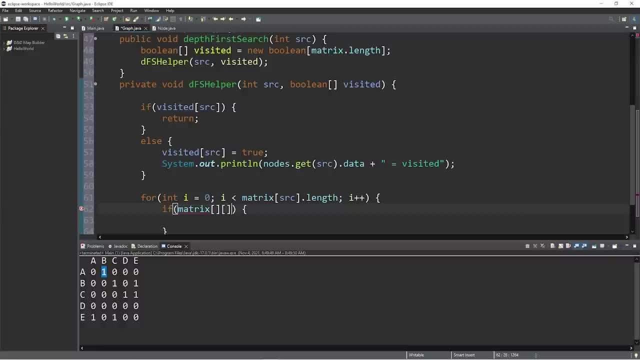 Boolean line statement. we don't need time. We need to include the node together when eats They're if matrix at indices of source and I. Source is the row that we're working with, I is the column. If this is equal to one, then we will invoke the DFS helper method again. So this is recursive. We. 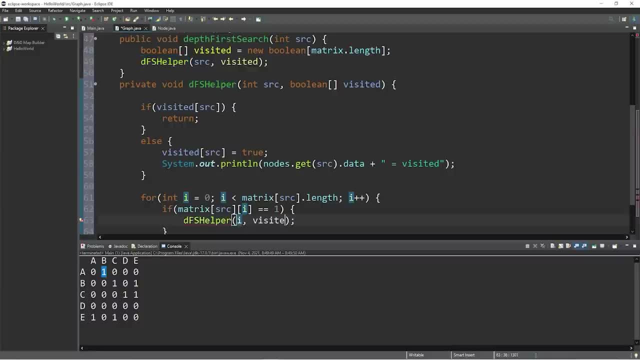 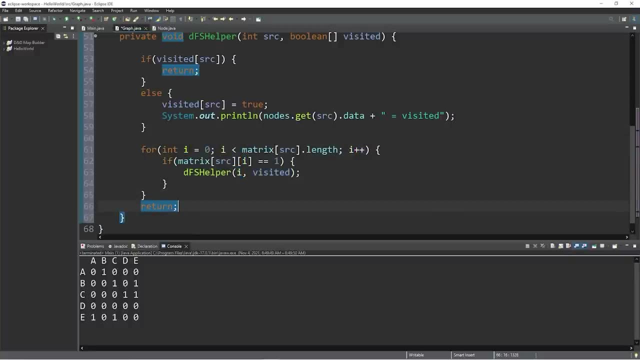 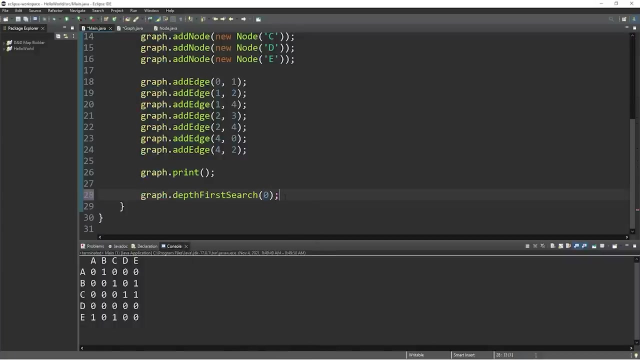 will pass in I as well as our Boolean array named visited. If we successfully search through an entire row outside of the for loop, let's return, And that's it. So let's run this Within my main class. I will call the graphs depth first, search method and pass in an index of a starting node. 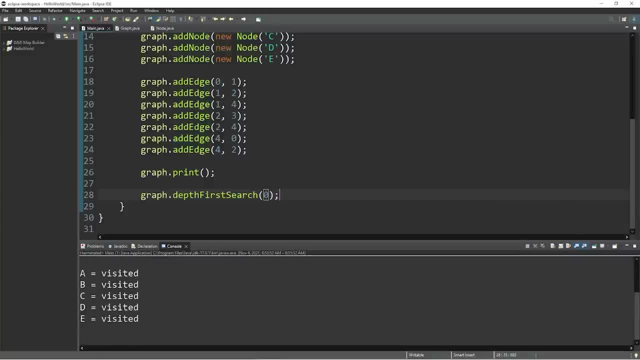 So let's begin at 0.. We visit A first, then B, C, D, E. Let's try B, which has an index of 1. B, C, D, E, A, C, which has an index of 2. C, D, E, A, B. Okay, 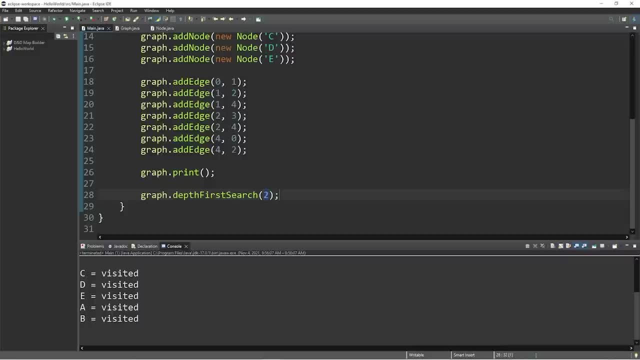 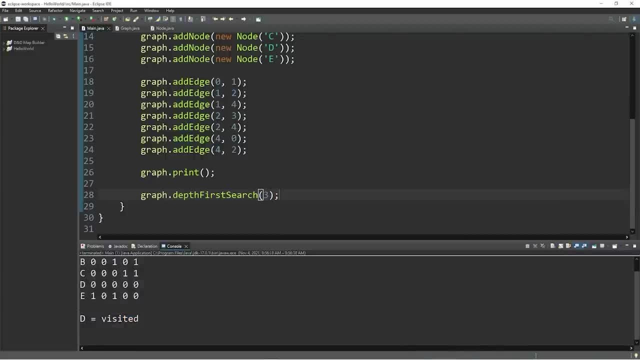 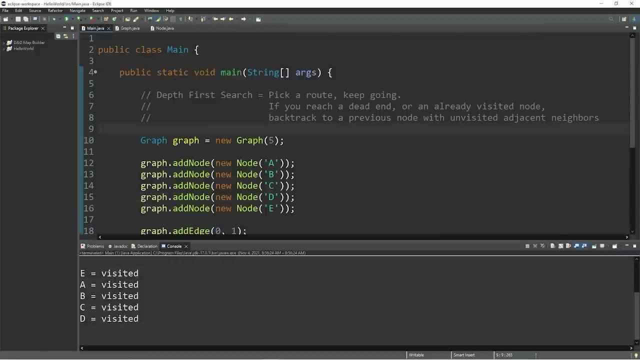 we can go. so we're stuck at D, We only visit D. And lastly, we have E, which has an index of 4.. E, A, B, C, D, All right, everybody. that is the depth first search algorithm. You pick a route. 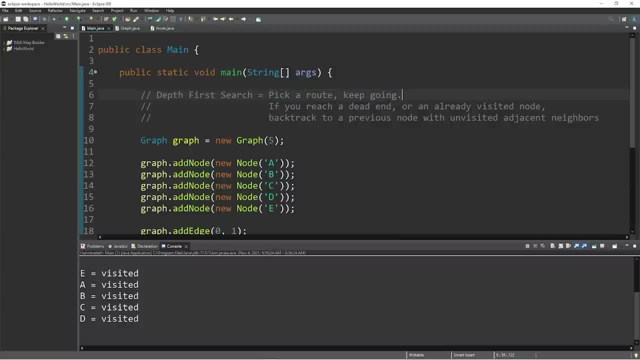 you keep going. If you reach a dead end or an already visited node, you backtrack to a previous node with unvisited adjacent neighbors. If you would like a copy of this code, I'll post this to the comment section below. Thanks for watching. 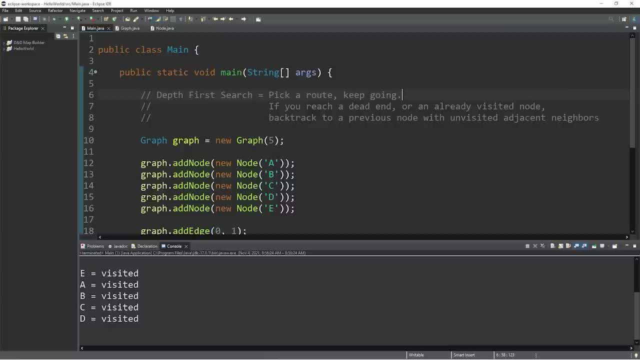 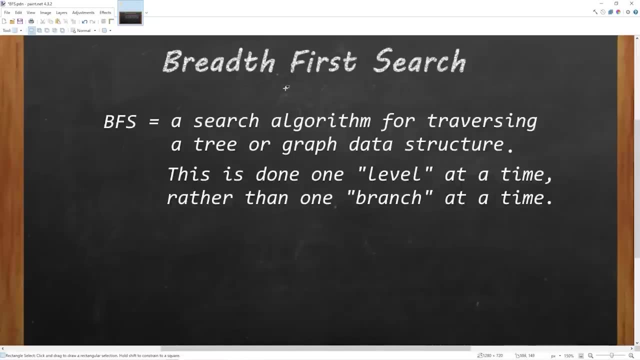 Don't forget to give this video a thumbs up, leave a random comment down below and subscribe if you'd like to become a fellow bro. All right, what's going on? people Breath first search. Breath first search is a search algorithm for traversing a tree or graph data structure. This is done one level at a time. 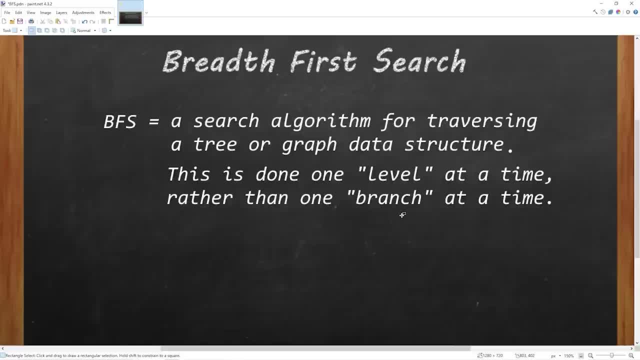 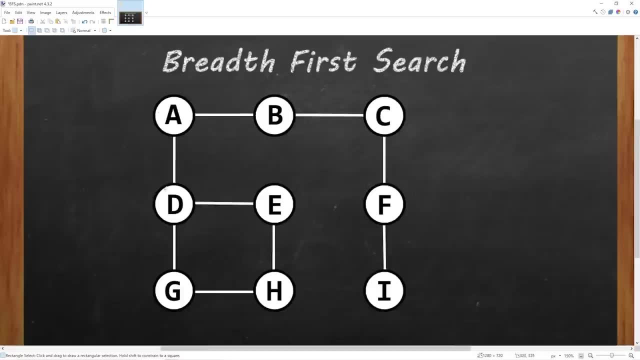 rather than one branch at a time, like what you see with depth first search. Here's an example In the previous topic on depth first search: we would navigate a graph one branch at a time, But in a breadth first search approach we would navigate this. 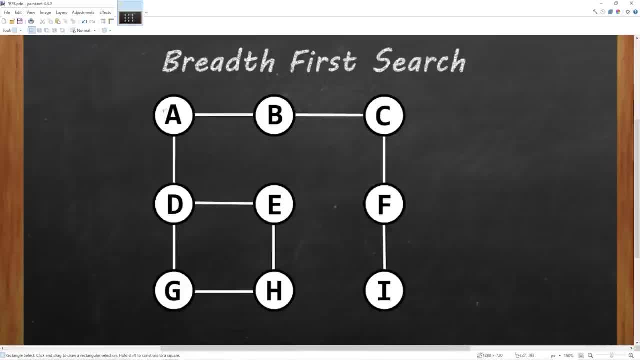 graph one level at a time. So let's begin at node A and we are attempting to travel to node I. Instead of a stack, we'll use a queue. All unvisited nodes we will add to the queue. So we're currently at A. We'll add that to the queue, Then add any unvisited adjacent neighbors. 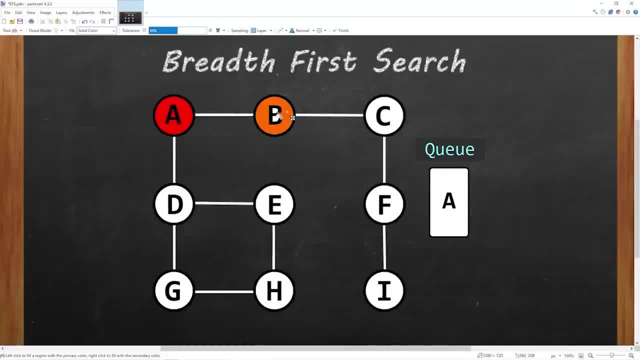 to the queue as well. We have both B and D as neighbors, So we will add these to the queue, Then add any unvisited adjacent neighbors of nodes B and D. That means we will add C, E and G, And for the next level we have F and H And lastly, I. 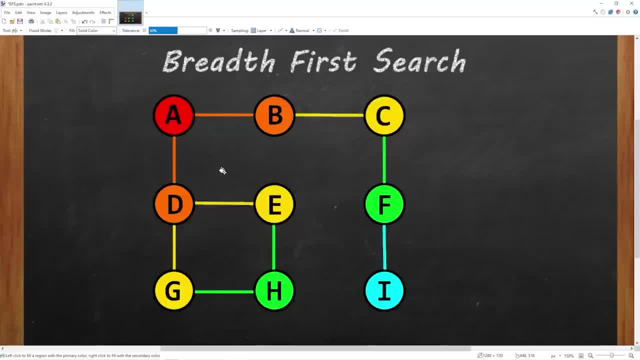 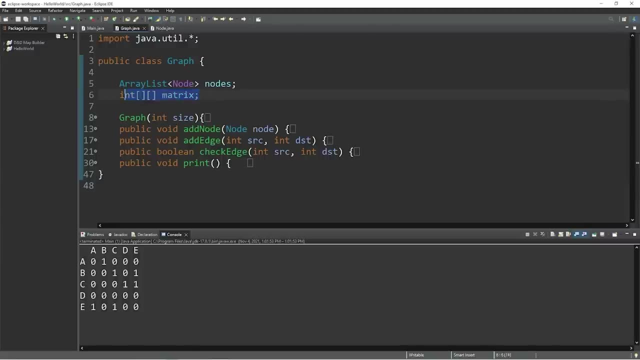 So that is a breadth first search approach. We will navigate a graph one level at a time using a queue, rather than one branch at a time using a stack, like with depth first search. Let's implement this in code now. Okay, everyone. so in my graph, I'm utilizing 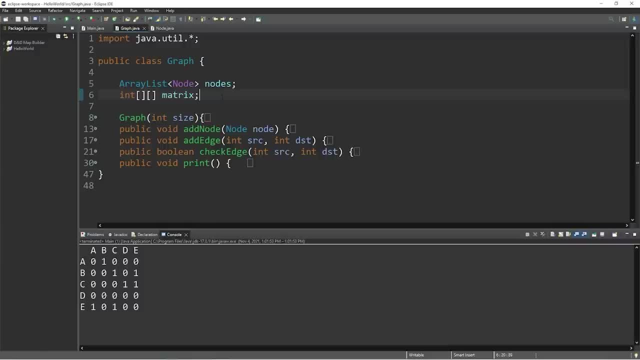 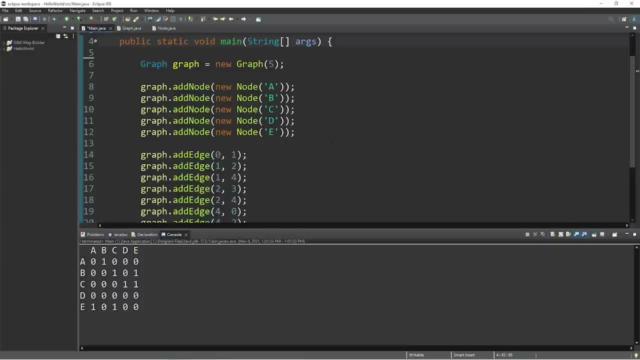 an adjacency matrix. We're re-using the same code from the previous few videos And we have a node class that contains some data, and I went ahead and populated this graph already. It's the same data from the previous few topics. Heading to our graph class, let's create a breadth first: search. 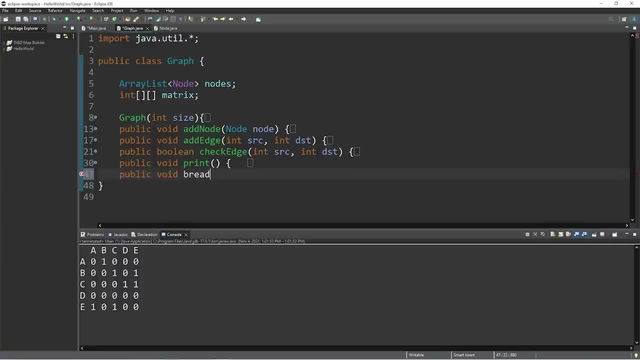 method: Public void breadth: first search And we will call the columns group of search b running. For the time being. we'll keep them inside of a field, Guarding it and crabbing them into the child. we will take an integer named source. This will be the index of the node we would like. 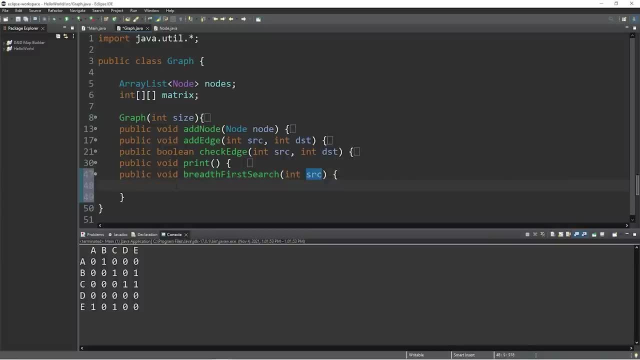 to begin searching at and with a breadth-first search, we can utilize a queue, So queue. we will store integers, these will be indices and I will name this queue Equals- new. Now queues are actually interfaces. we need to use a data structure that utilizes the queue. 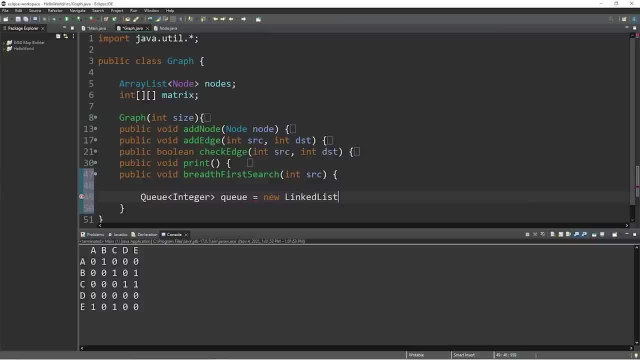 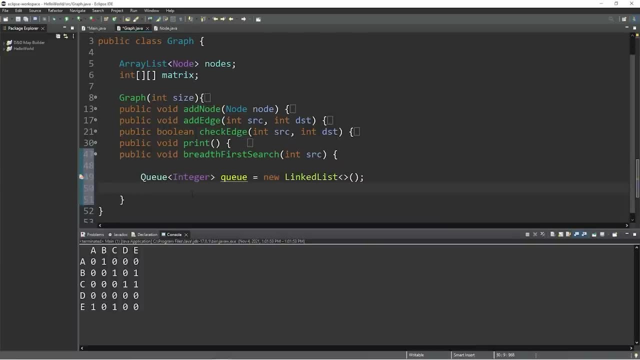 interface, one of which is a linked list. Okay, so we have our queue and we're going to create an array of booleans to mark if a node has been visited or not. So let's create a boolean array named: visited equals new boolean and the size will be matrix dot length. 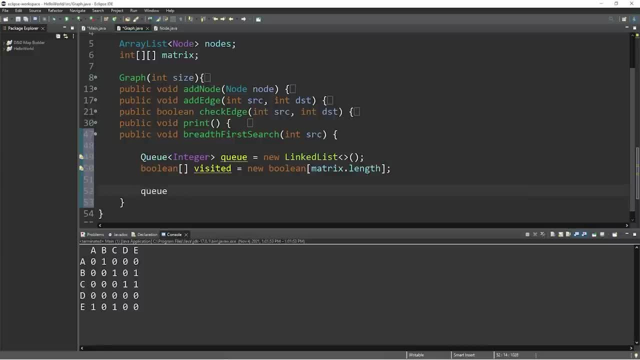 With the node that we'll begin at. let's add that to the queue. Queue dot. you can use add or offer And then pass in the index of the starting node. Then, within the boolean array of visited, we will mark this as true At. index of source equals. 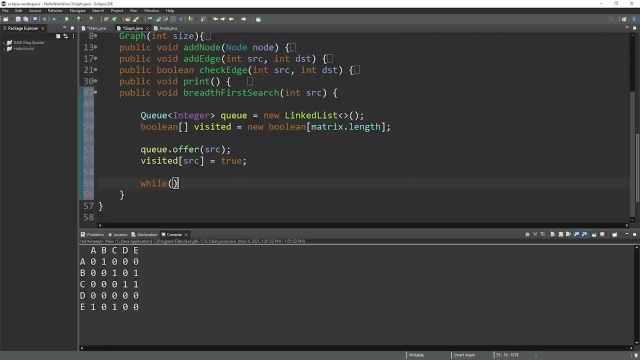 true, And now we'll need a while loop. Our condition is that we'll continue this while loop while the queue's size method does not equal zero. We'll assign our source equal to whatever is at the front of the queue. Queue dot pull. 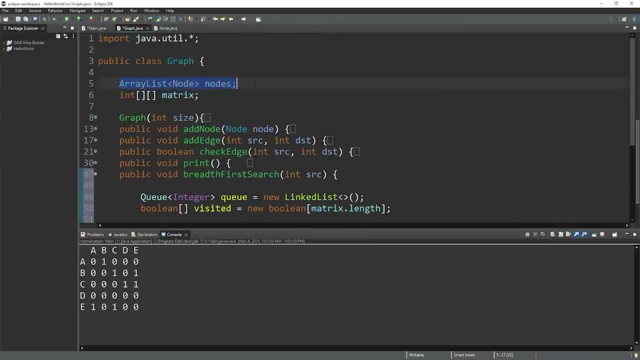 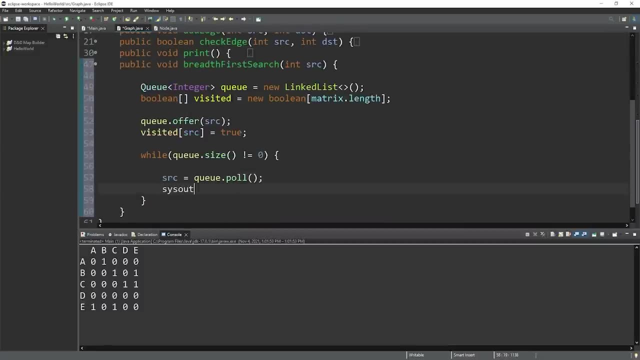 to remove an element With this code that I've written. I've already went ahead and created an array list of the nodes to access the data. Whenever we pull a node, I'm going to display the data. So this part technically isn't necessary. Nodes dot get source dot. 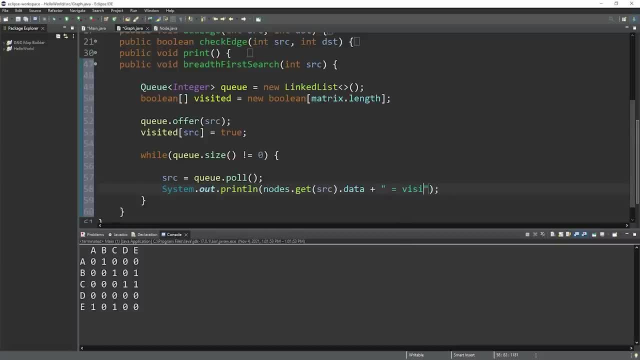 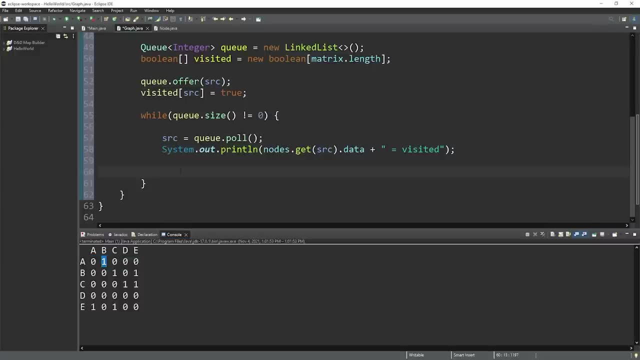 data plus equals visited. Let's say that we're at node A. We're going to iterate a bit over this row and look for any adjacent neighbors, So let's use a for loop for that. For int, i equals zero. We will continue this as long as i is less than our matrix at index. 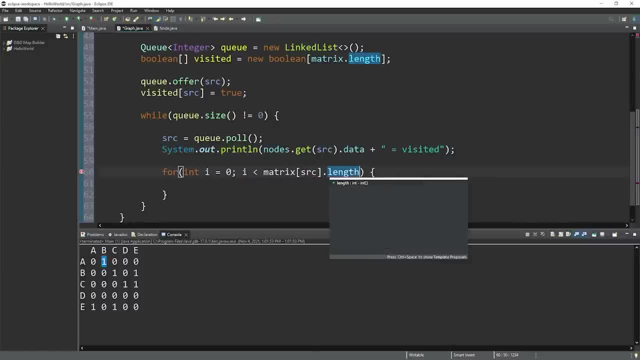 of source dot length. This means the length of the row, Then i plus plus. During each iteration let's check to see if this value is one and the node that we're trying to visit has not already been visited. If, then, matrix at indices of source and i is equal to one, 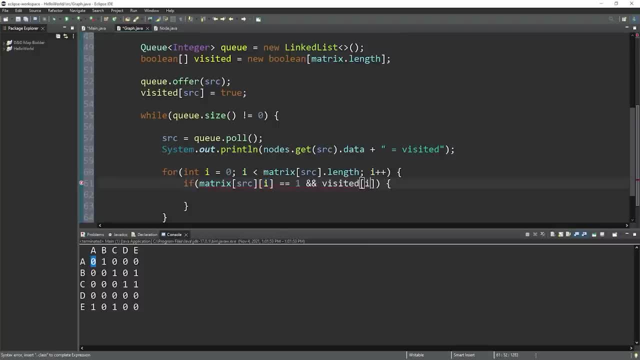 And visited at index of. i is not true, So we can use the not logical operator. If we have an adjacent neighbor that's not been visited, then we will add the index to the queue And that node is going to wait in line Queue. 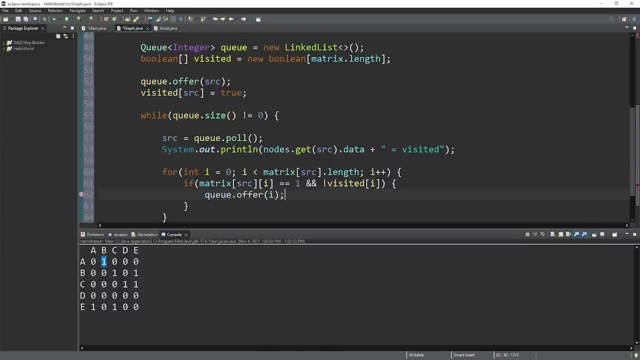 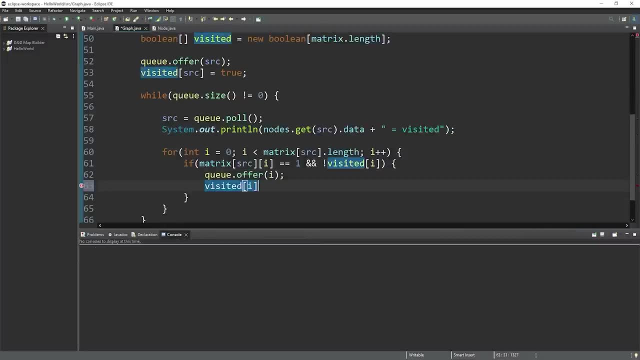 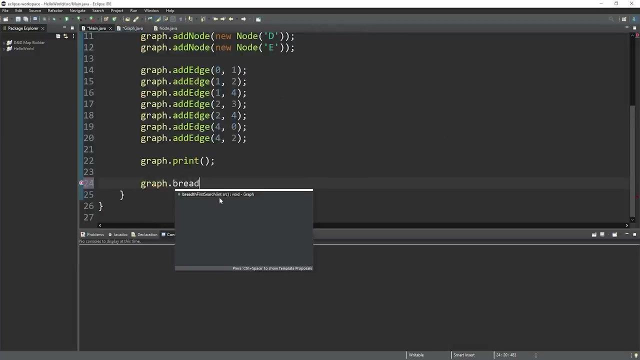 Dot offer i, And i is an index, And then mark this node as visited. So take our boolean array: visited at index of i Set the sequel to true And there we go. Let's invoke the breadth first, search of our graph class, Then pass in an index of a node we would like to. 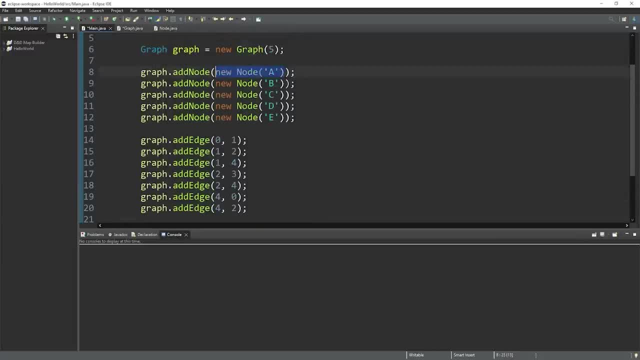 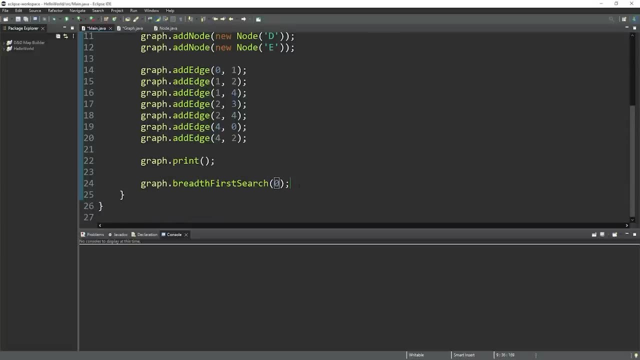 begin at. In this example, node A has an index of zero, B is one, C is two, So on and so forth, a breadth-first search beginning at node A. We will cover these nodes in this order: A, B, C. 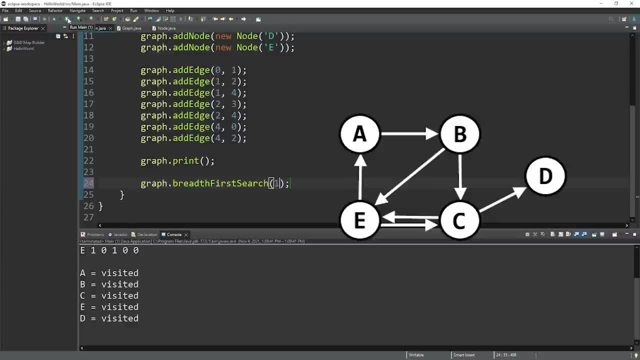 E, D. Let's change this to 1.. That would be node B, B, C, E, D, A. 2 is C, C, D, E, A, B, 3 is D. We can't go anywhere from node D, so only D is visited, And E, E, A, C, B, D. Now, before we wrap, 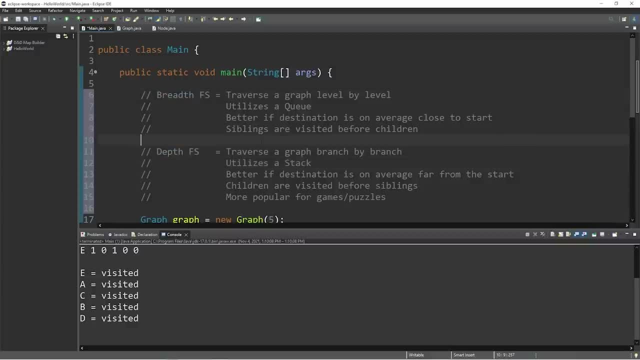 things up. here are the differences between breadth and depth-first searches. Breadth traverses a graph level by level. Depth traverses a graph branch by branch. Breadth utilizes a queue. Depth utilizes a stack. Breadth tends to be better if the destination is, on average, close to the 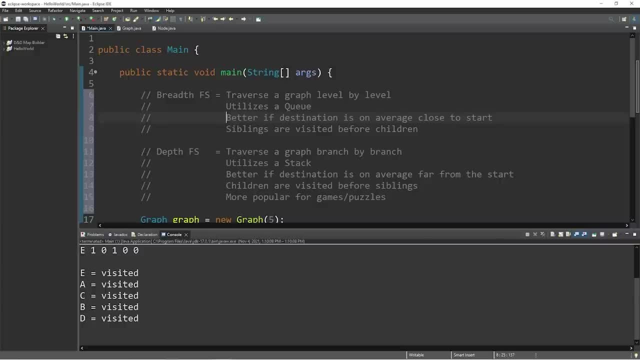 start And depth tends to be better if the destination is, on average, far from the start. In a breadth-first search, siblings are visited before children. In a depth-first search, children are visited before siblings. And if you ever plan on creating video games, depth-first searches tend to be more. 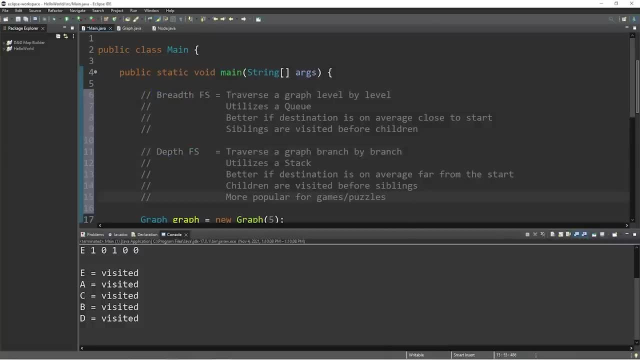 popular than breadth-first searches. Alright, everybody, that is the breadth-first search. If you would like a copy of this code, I'll post this to the comment section down below. Don't be afraid to give this video a thumbs up. drop a random comment down below and subscribe. 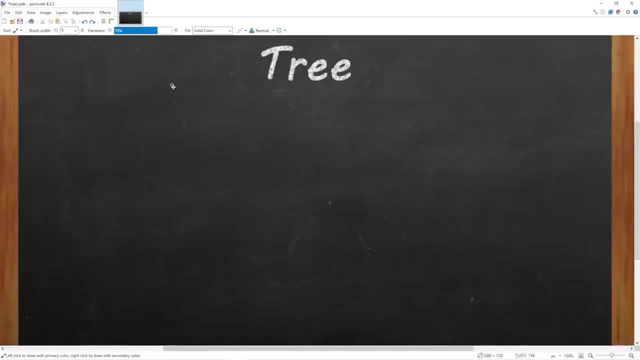 If you'd like to become a fellow bro, Alright, everybody. here's a quick introduction to trees. In this video we're only going to cover some of the terminology. A tree is a non-linear data structure where nodes are organized in a hierarchy. This could be one example of a tree. It's made up of nodes and edges. Nodes could be: 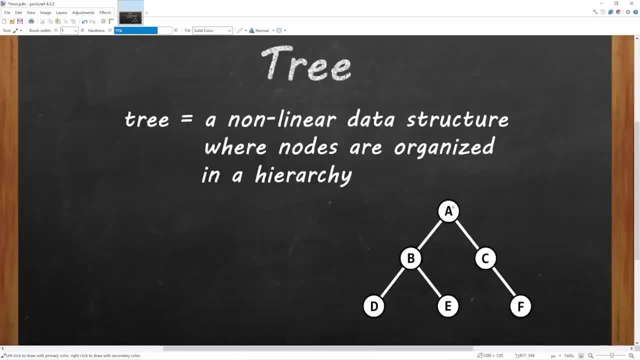 some piece of data and edges represent a relationship between two nodes. A real-life example of a tree could be a family tree. Maybe we're at node D, That's us or me or you. B is a parent. E is your brother or sister. A is a grandparent. C could be an. 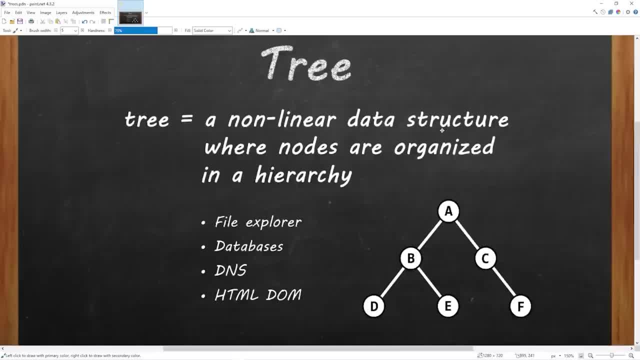 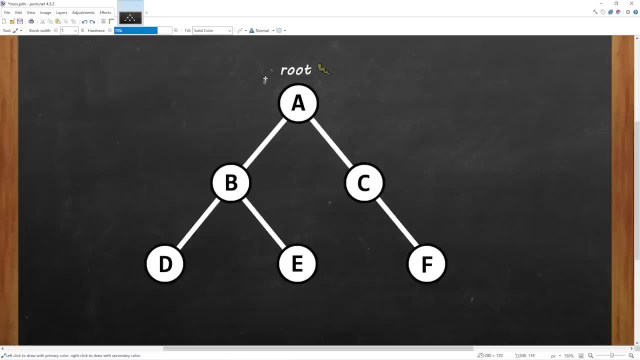 aunt or uncle and F is your cousin. A few examples of where a tree data structure would be used in programming or technology would be file explorers, databases, domain name servers and the HTML document object model. The top of the tree is known as the root node. The root node doesn't 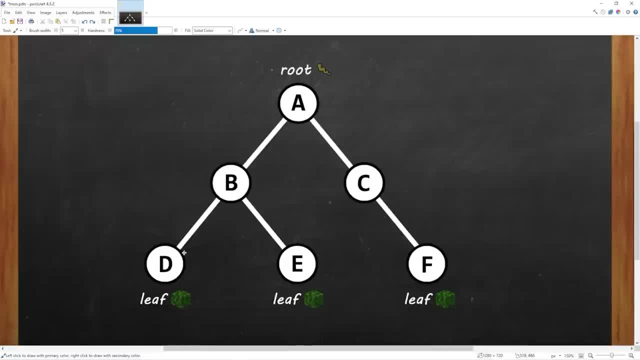 have any incoming edges, only outgoing edges. Any nodes at the bottom of a tree are known as leaf nodes. They do not have any outgoing edges but they do have incoming edges And branch nodes are in the middle. They have incoming and outgoing edges. Here's a few other terms: Any nodes with 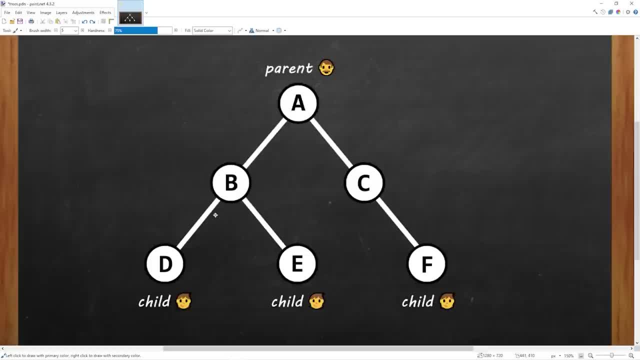 outgoing edges are also known as parents. Any node with an incoming edge is known as a child node, And nodes can be both parents and children if they have both incoming and outgoing nodes. Any two children that share the same parent are known as siblings. Nodes D and E both share the 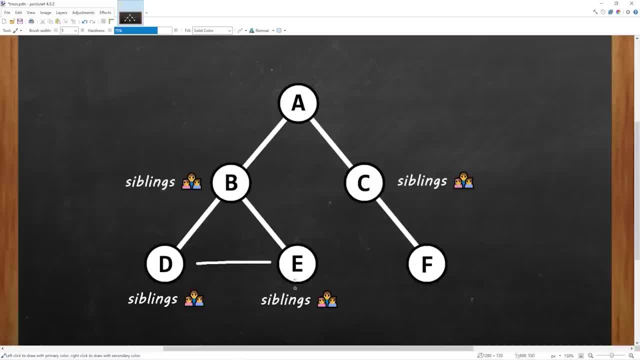 same parent of B, So D and E are both siblings. The same thing goes with B and C Nodes B and C share A as a parent, so these two nodes are siblings. It's just like a family tree. A subtree is a smaller tree held within a larger tree. You could say that this portion is a subtree. 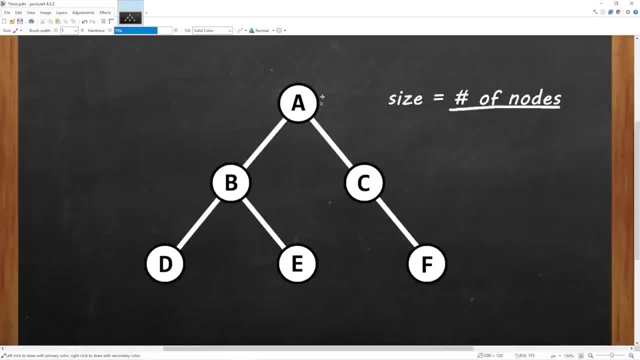 The size of a tree is equal to the number of nodes. So what's the size of this tree? We have one node, two, three, four, five, six. The size of this tree is six, Six nodes. The depth of a node is the number of edges below the root node. Our root node would have a depth of 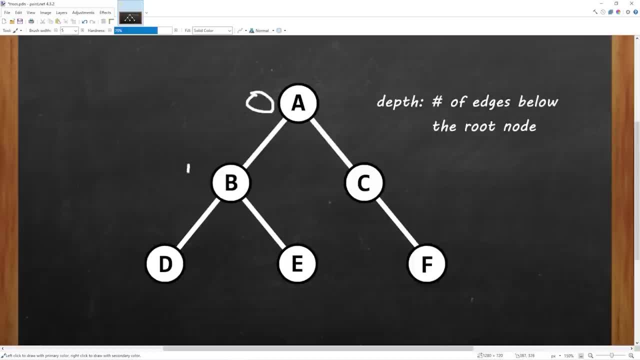 zero. Then, as we move down, levels B and C have a depth of one, D, E and F have a depth of two. And lastly, the height of a node is the number of edges above the furthest leaf node. All of these 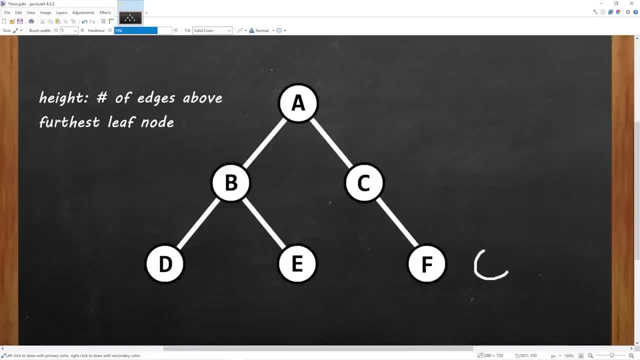 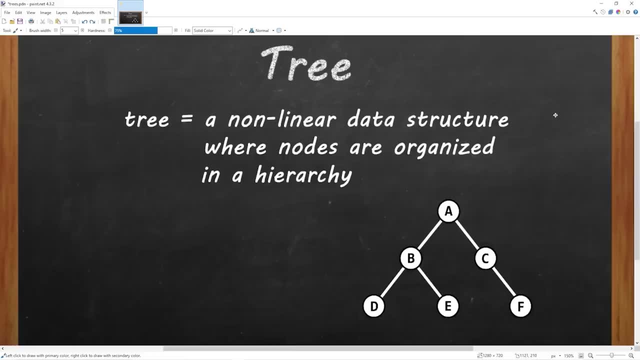 are the same distance away from the root node, These would all have a height of zero. B and C have a height of one And A has a height of two. Well, alright then everybody. That is a quick introduction to some of the terminology around trees. It's a non-linear data structure where 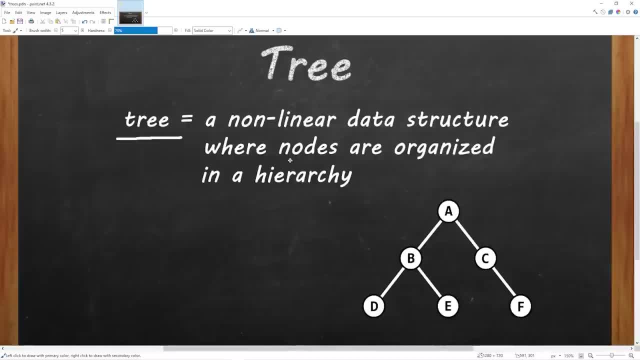 nodes are organized in a hierarchy And in the next few topics we'll get a little more in-depth with trees. If you found this video helpful, please help me out by smashing that like button. leave random comments down below and subscribe if you'd like to become a. 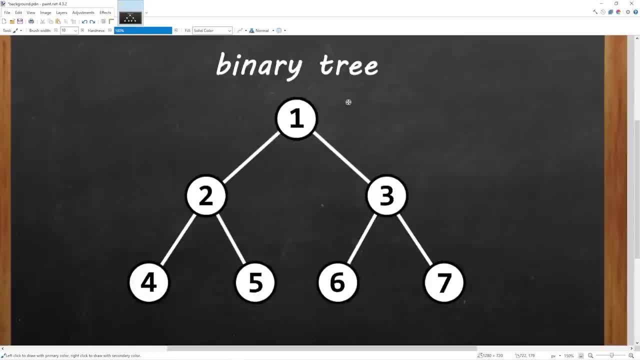 friend, Thanks for watching. Alright, what's going on? everybody, In this video we're going to discuss binary search trees, But first we'll need to know what a binary tree is. A binary tree is a tree where each node has no more than two children. That's why it's binary. In this example, node one has two children. 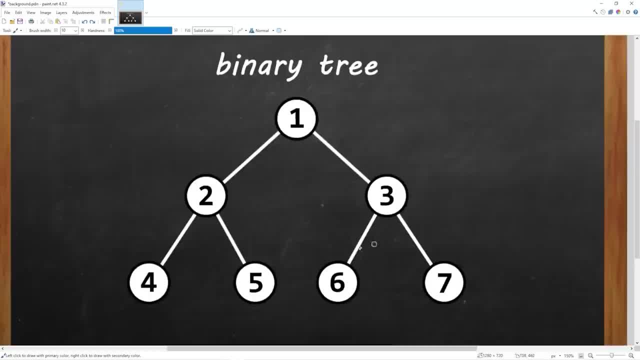 two and three, And each of these children have their own children. They have no more than two children. Nodes four and five are the children of two, And nodes six and seven are the children of three. In this similar example, this would also be a binary tree. 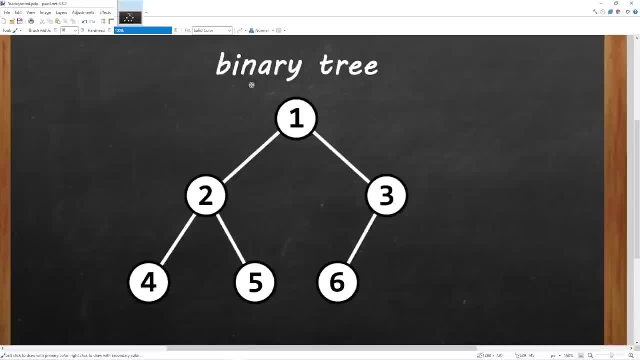 Node three only has one child. node six, But with a binary tree, no node has more than two children. Since node three has one child, that's fine, But if node three had three children, well, that would no longer be a binary tree. Now what makes a binary search tree different? 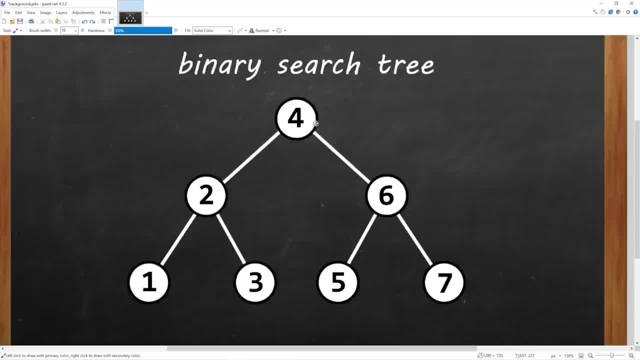 from a binary tree is that the values are arranged in a certain order. Here's the order: The root node should be greater than the left child, but less than the right child. Four is greater than two and four is less than six. That's the pattern that this data structure is built around. 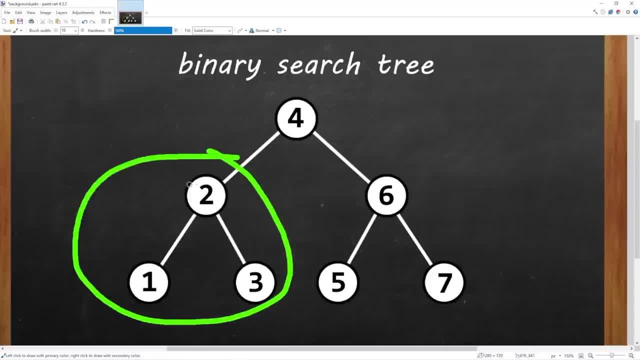 If we take a look at some of the subtrees, let's say this: one, Two is greater than one but less than three, And in this subtree, six is greater than five but less than seven. If done correctly, starting at the root node, the left, most child should be the least value. 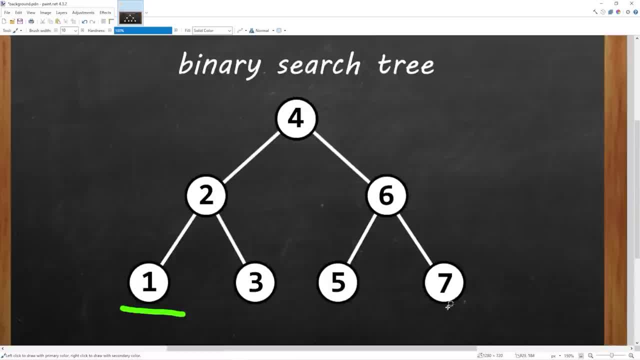 And the left most child should be the least value. And the left- most child should be the least value. Again, starting from the root node, the right most child should be the greatest value. The reason that these nodes are arranged this way is for quick lookup, Let's say we're looking for 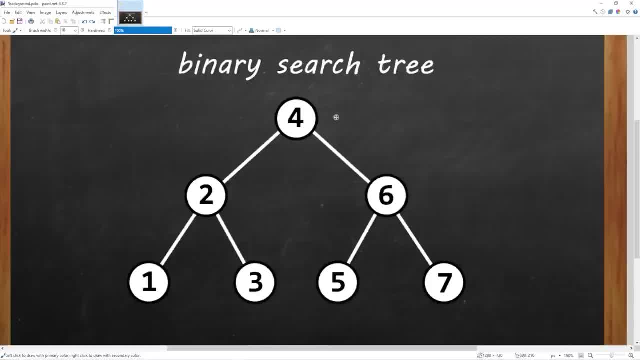 five. What we'll do is compare five to the root node. If five is equal to the root node, well then, we found our answer. If five is greater than our root node, we will move down to the right branch and do the same thing again. Is five equal to six? No, it's not. However, 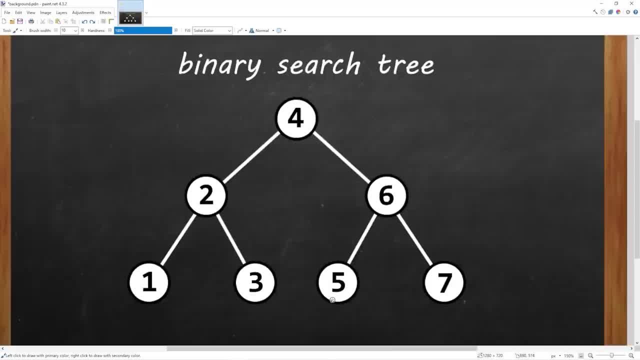 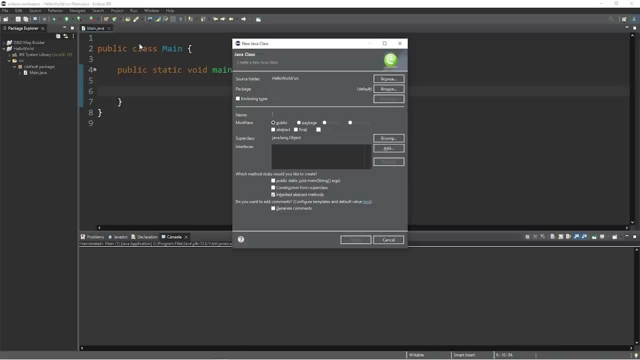 it's less than six, so we know to go down this branch. The runtime complexity defined a value within a binary search tree is O in its best case. So let's code a binary search tree now. Okay, let's begin. Let's create a node class file, new class. I will name this: 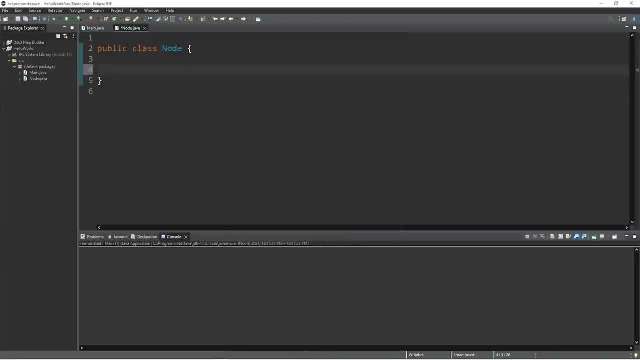 node and finish. Nodes will have some data, maybe an integer, this time Int data, And the node class should contain at most two nodes: Node left for the left child and node right for the right child. If a node is a leaf node, well then these will be null, But we would still like to allocate space. 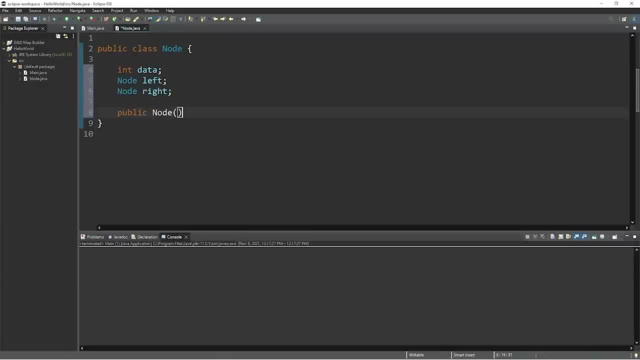 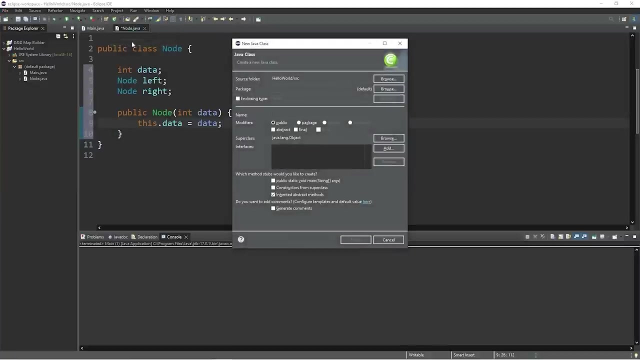 to hold children. And within the constructor, we will pass in some data- Int data- and assign it. This dot data equals data. Now let's create a binary search tree, class File, new class, Binary search tree. And within our main class, let's instantiate: 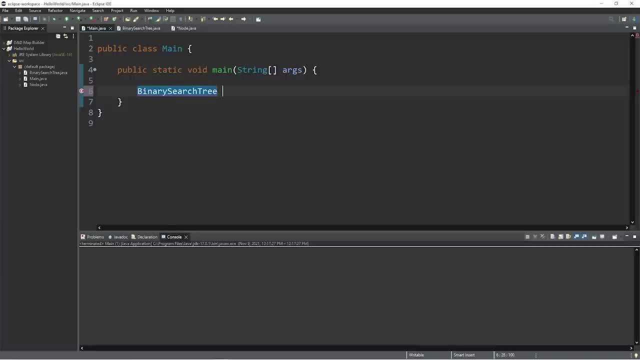 a binary search tree. object: Binary search tree. I'll name this tree- equals new binary search tree And within the binary search tree class each binary search tree should have a root node, Node root. Here are some methods. We'll need an insert method to insert nodes Public void insert. 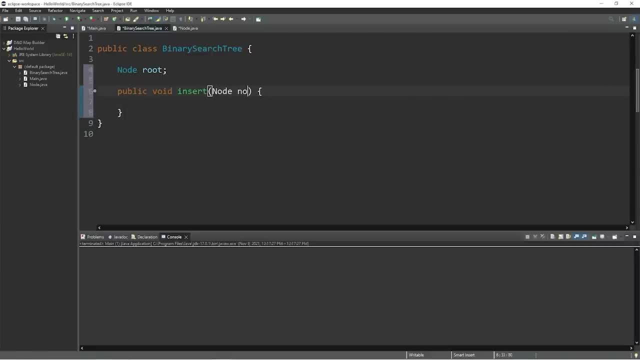 And there is a parameter of a node, Node, node. Now let's create a second method. This next method will be a helper method of the insert method, So the insert method is going to call its helper method And this will be private. 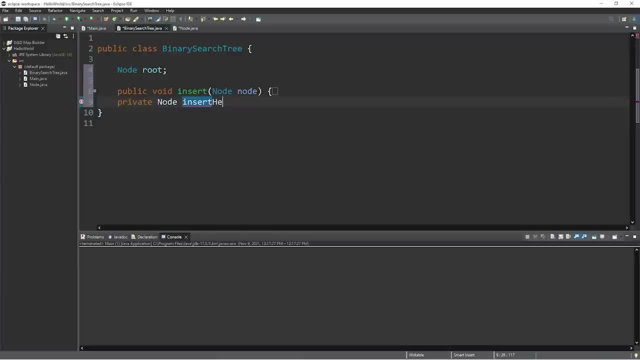 The return type is node Insert helper. We need a root node, Node root And a node Node node In order for our program to compile. we do need to return something. so, just as a placeholder, I'm going to return null. 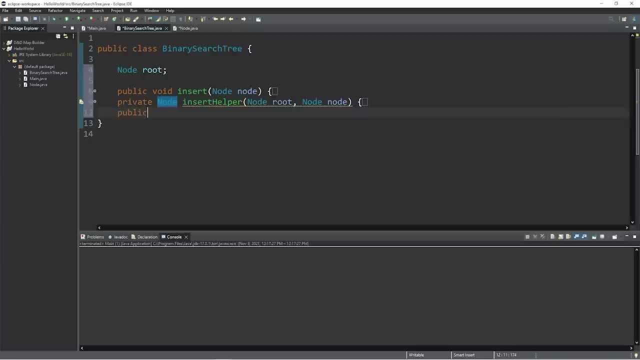 Okay, for the next method we need a display method- Public void display- And a helper method- Private void display, helper. And this has one parameter: a root node, Node root. Next method is a search method- Public. 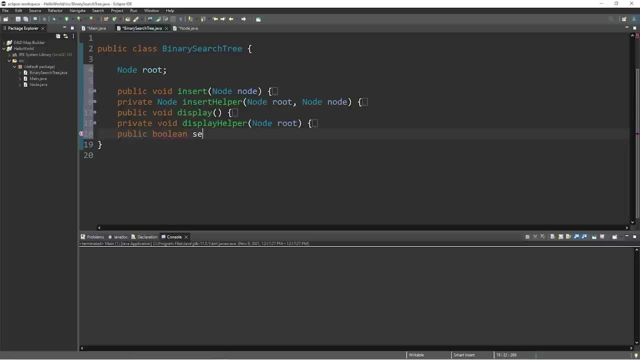 boolean. We're returning a boolean Search And the parameter is int data And we will need a helper method: Private boolean Search helper. There are two parameters: Node root And int data. Again, we do need to return something. 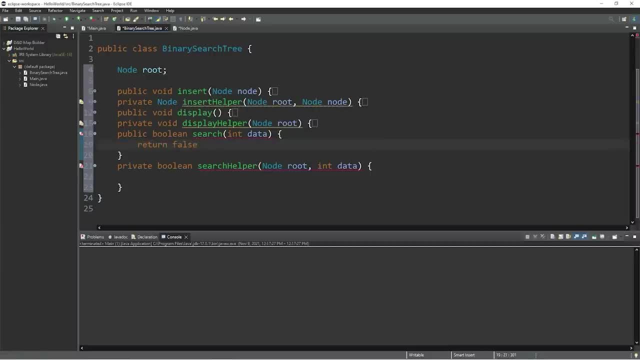 I'm going to return false just as a placeholder. Okay, next method is a remove method: Public void remove And the parameter is int data And we'll need a helper method. The return type is node Remove helper. The two parameters are node root and int data. 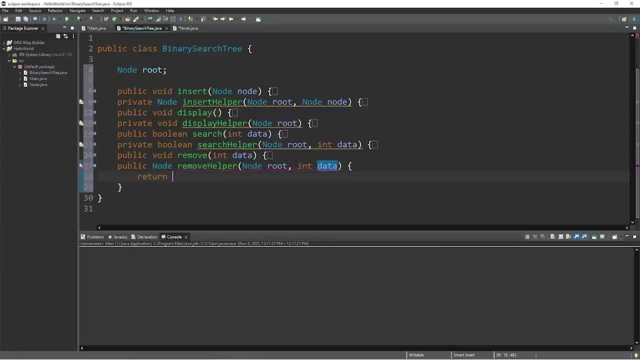 We do have three of those have to return something, so as a placeholder, I'm going to return null. Our remove helper method is also going to rely on two separate methods: one to find a successor and another to find a predecessor. This is in case we're. 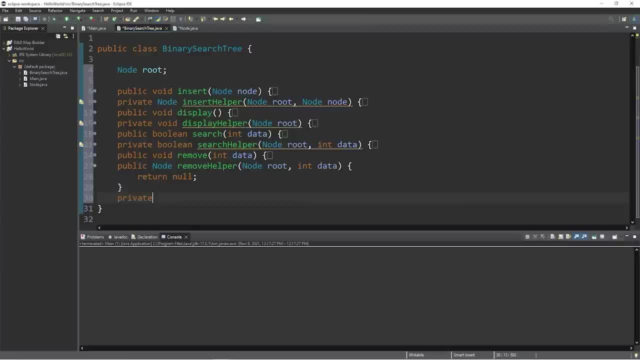 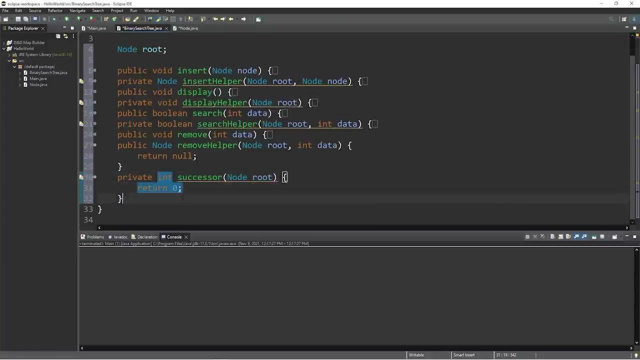 deleting nodes. we have to shift nodes around, So this will be private int successor and we will pass in node root And we need to return something. let's return zero as a placeholder And let's copy this, paste it and this will be. 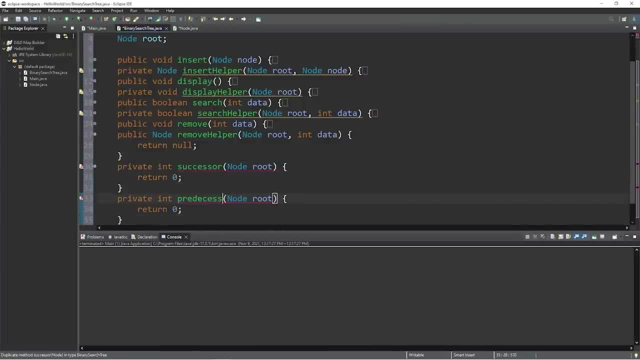 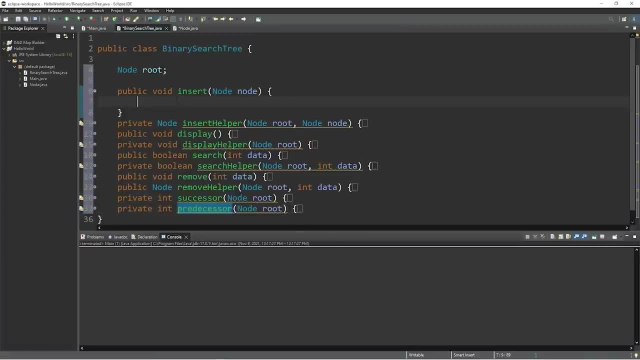 method predecessor, And that will be it. So let's close these for now and begin with the insert method. So with the insert method we will assign our root node equal to insert helper method. pass in our root node and node. So the reason: 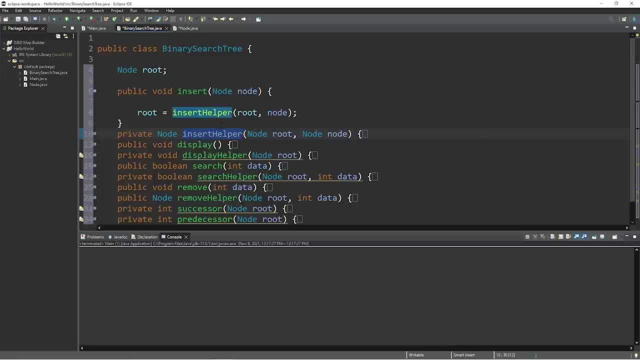 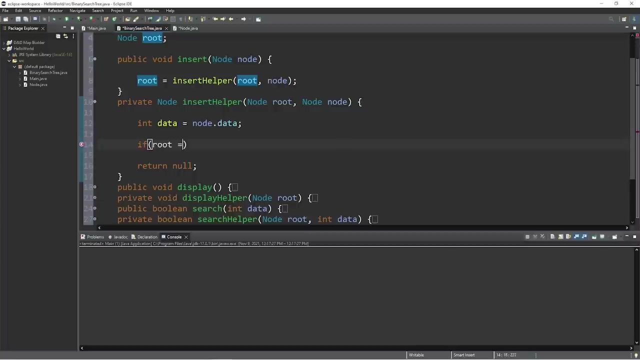 that we're using helper method is because we want to make sure that our node is assigned to the root node. So let's check to see if our root node is assigned or not. So if our root is equal to null, then we should probably assign. this node to the root node because, well, this is the root node that we're assigned to. So let's check to see if our root node is assigned or not. So if our root node is assigned to the root node, then we should probably assign this. 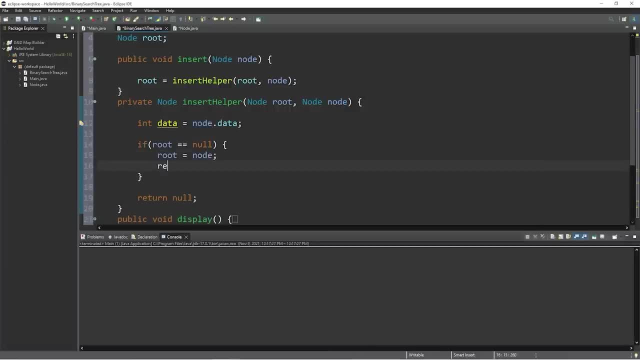 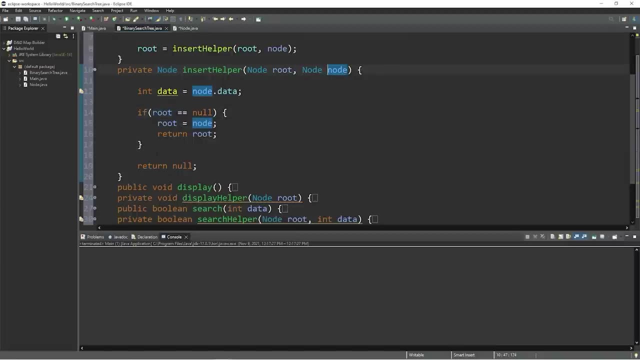 the first node, Root, equals node Return root. If root is not null, we have to compare the data to see if it's less than our root or greater than our root. Else, if our data is less than the data of the root node, then we are going to. 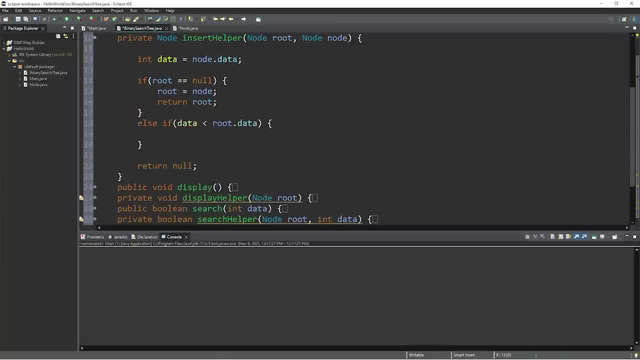 assign this node as the left child of our root node. Our root's left child rootleft equals and we will use recursion. insert helper method, Pass in our root's left node and our node- The root node is going to change with recursion At first. 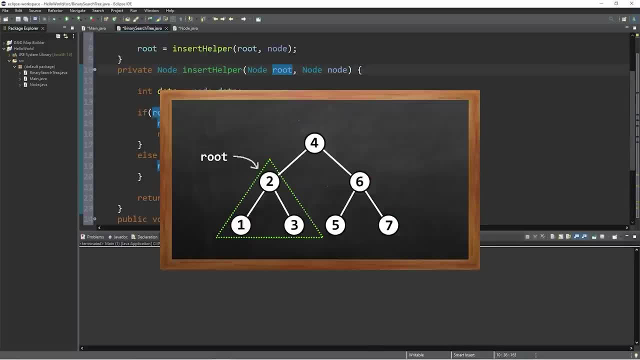 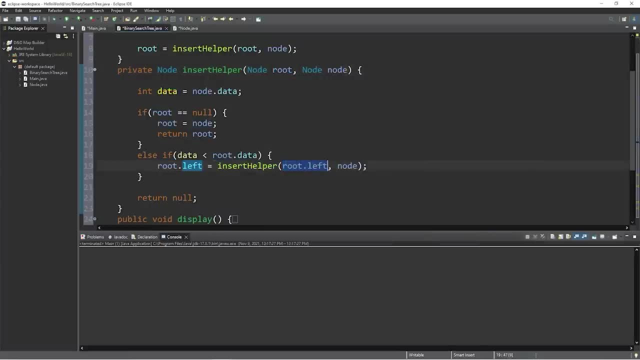 it's going to be the root node of the entire tree. After recursion, we're examining the root node of a subtree. So if we're passing in the left child of the original root node, well then that left child is now the root. 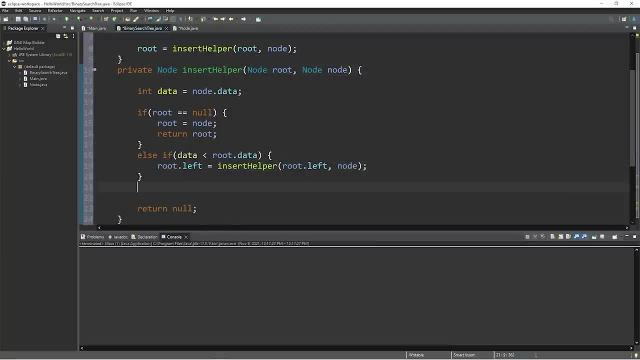 node of a subtree that we're currently working with. So LSF, if the data is less than the current root node, we go left. If it's greater than the root node, then we will go right. Else root dot right. that's the right. child equals insert helper method. 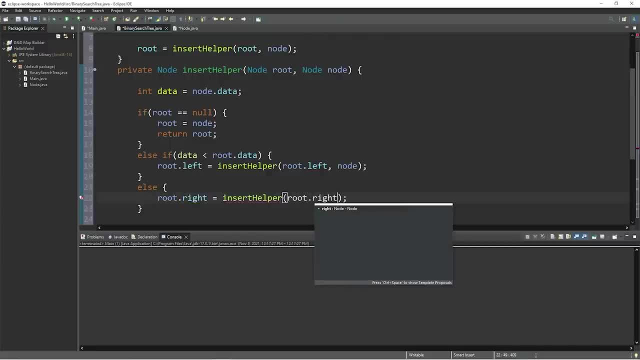 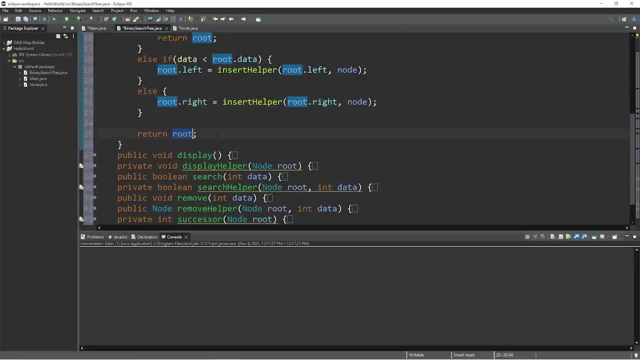 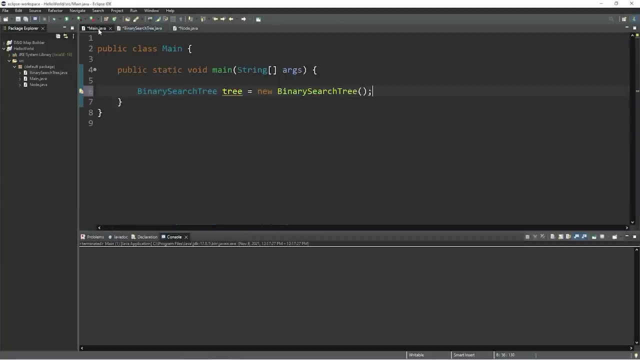 pass in root dot right and our node, And it's the same process all over again And at the end we will return the current root node. Okay, that is it for the insert method and the insert helper method. So let's insert a few nodes, although we can't yet display them. 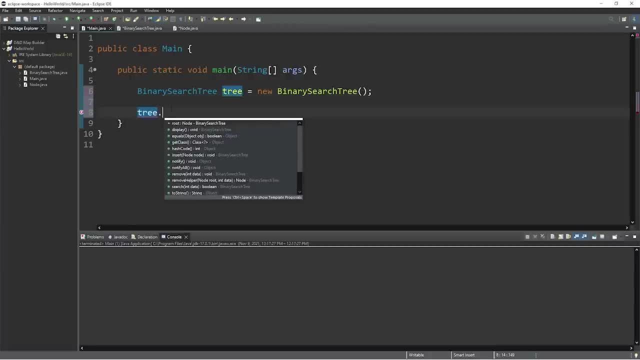 Let's insert some anonymous nodes: Tree dot insert and we can pass in a node, either a node name or an anonymous node. So let's pass in some anonymous nodes. Let's pass in the number five or some other number You're choosing. And let's pass in a bunch of numbers. How about one and nine? make sure these. 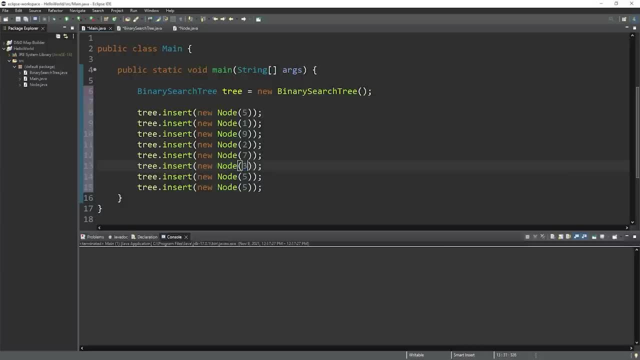 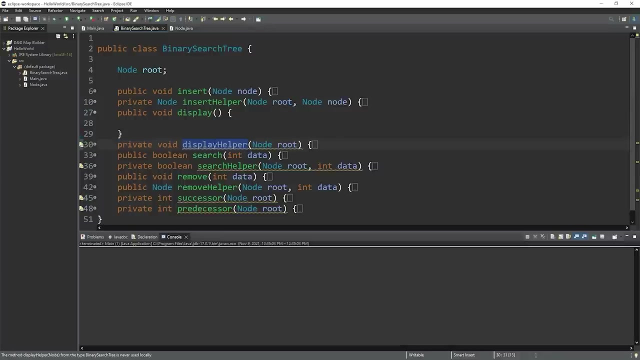 are not in order: Seven and three, six, four and maybe one more Eight. If you run and compile this, there is nothing obvious that really happens. So let's work on a display method next. So with the display method, we will invoke our helper method. Display helper pass in the root node. 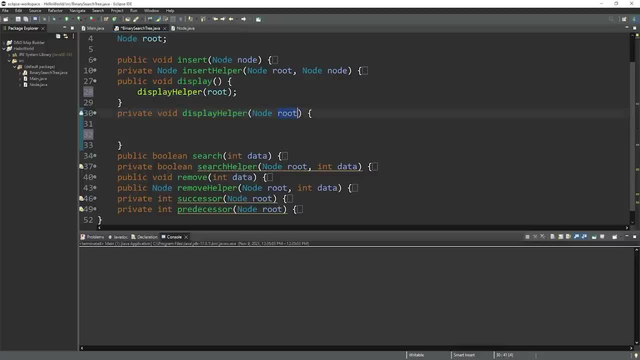 Within the display helper method, we're going to check to see if the root node of our subtree does not equal null. So if root does not equal null, if you would like to display these in order, we can use in order traversal, And that uses recursion. So invoke the display helper method, Pass in the. 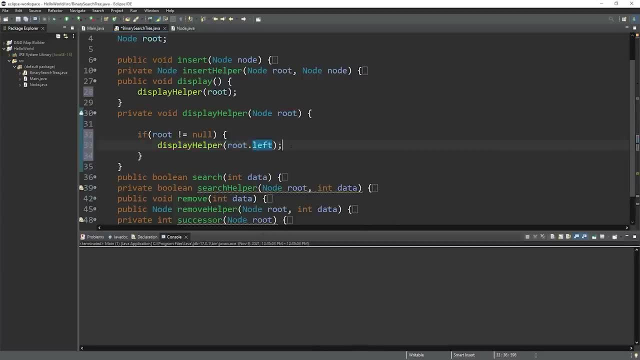 root child's left node. root dot left. If we're using recursion, the first piece of the display data that's displayed is the least value, and these values will be displayed in increasing order. Technically the term is non-decreasing, but think of it as ascending order. So the very first value. 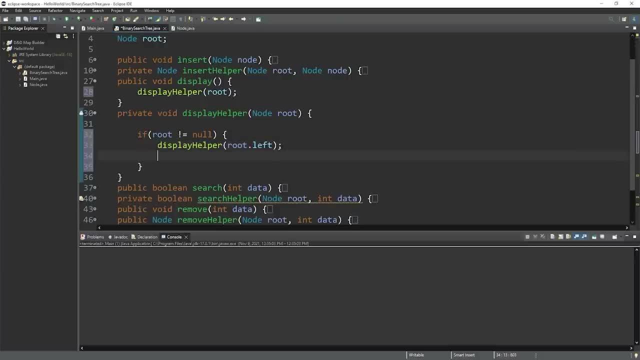 is going to be the least one, followed by the root node of this subtree: Systemoutprintln- rootdata. In our first subtree, the data all the way to the left is 1, and the root node of that subtree is 2.. Then we need the right child, which should theoretically be 3.. So again, we'll invoke 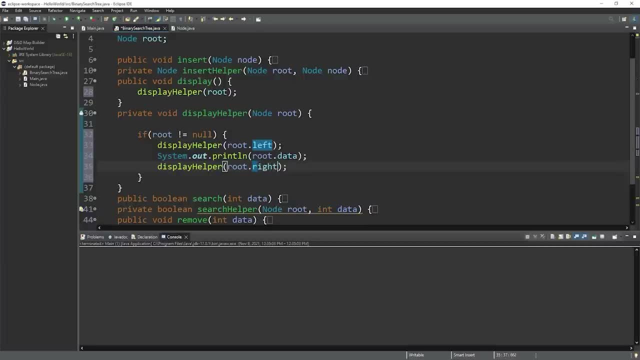 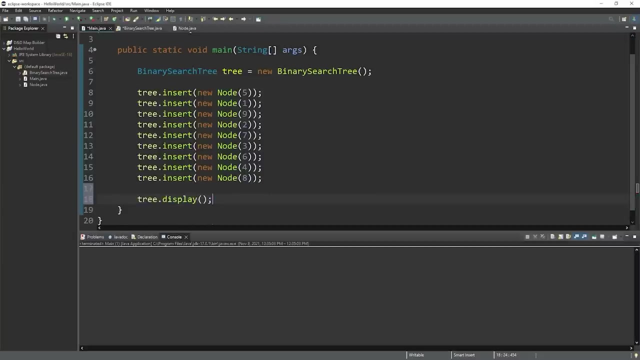 the display helper method and pass in the right child. So this is in order traversal. All of the nodes will be displayed in non-decreasing order. So let's try this At the end of our main class, let's invoke treedisplay and see what happens. Yeah, there we go: All of the nodes within our 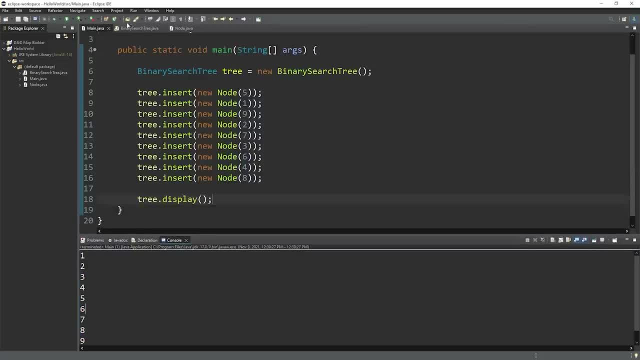 binary search function are displayed in non-decreasing order. All of the nodes within our binary search function are displayed in non-decreasing order. All of the nodes within our tree are now in order. If you would like this in reverse order, you can just change these methods. 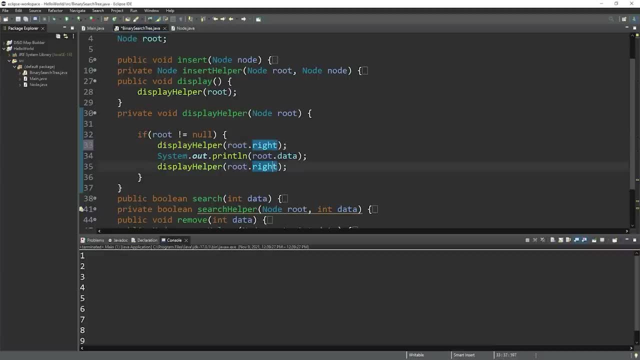 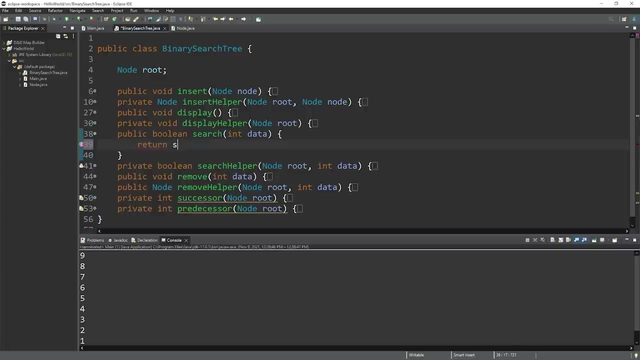 around. Replace left with right and right with left, And these are now in decreasing order, But let's change that back. Okay, up next we have the search methods. Okay, search will return. Then invoke the search helper method. Pass in our root node as well as some data within the 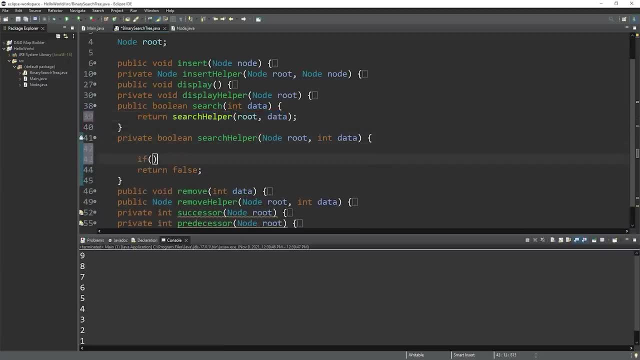 search helper class. We'll check to see. if root is equal to null, That means our tree is empty, So of course we can't search for anything. Return false, Then add else. if our rootdata is equal to data, That means we found the data that we're looking for. There's a match. 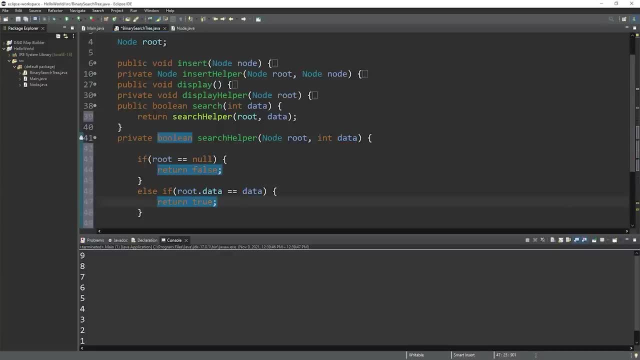 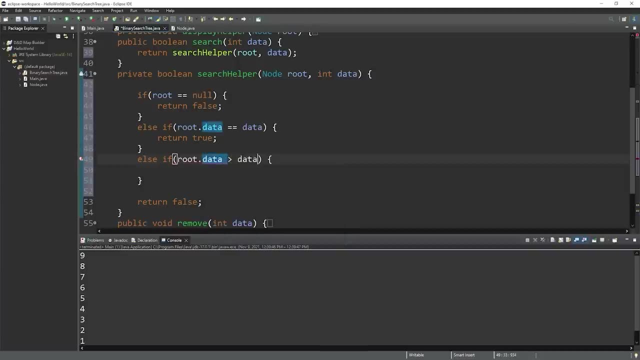 Then we're going to return true, We found what we're looking for. Else, if our root's data is greater than our current data that we're looking for, that means we need to go left, So return, Then invoke the search helper method. 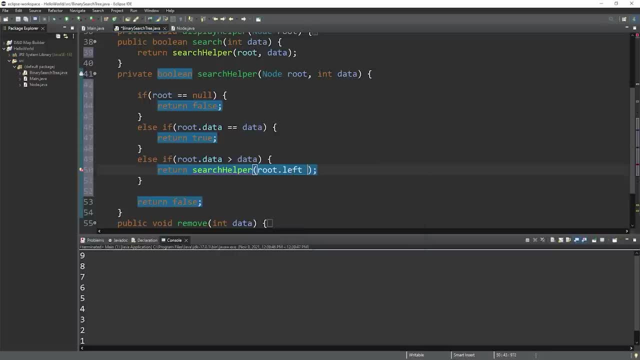 Pass in the left child, rootleft, And the left child is now the root node of the subtree. And then you need to pass in data as well, Else we go right. So copy this, paste it: Return search helper: rootright And data, And we can get rid of this return statement at the bottom. 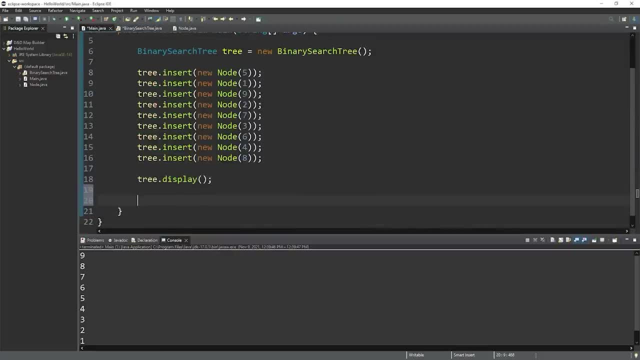 Okay, let's try this. So at the end of my main class, let's use a println statement And I will type treesearch And let's search for zero. None of my nodes have zero as a piece of data, So this should return false. Let's search for one now And that returns true. There's a. 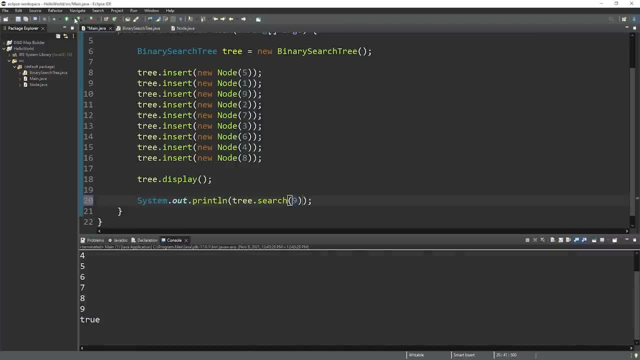 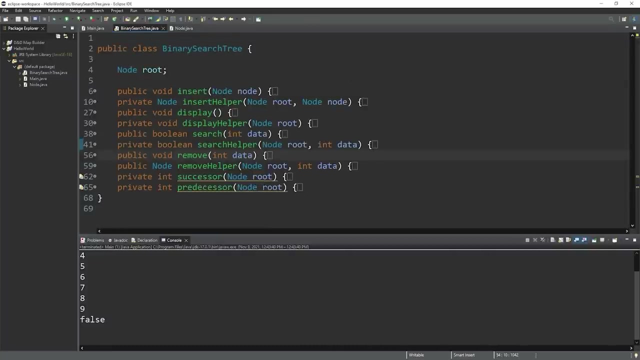 one within one of my nodes. What about nine? That is also true. And let's try 10.. And that is false. Okay, so those are the search methods, And, lastly, we have the remove methods, as well as successor. 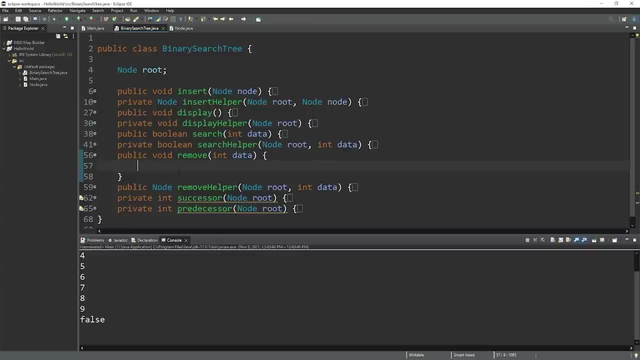 and predecessor. Now these methods are going to be a little bit tough, but I'll try my best to explain it. So within an if statement, let's check to see if this data even exists first. So let's invoke the search method and pass in our data. So this returns a Boolean: true or false. 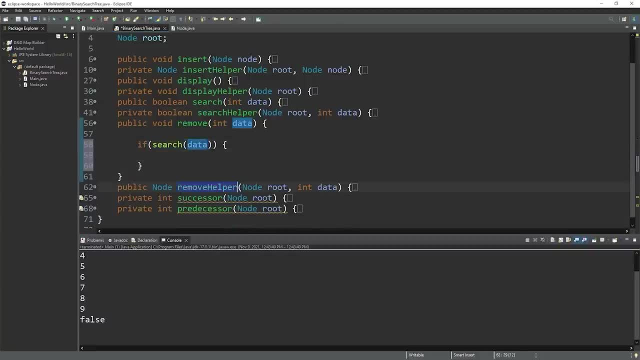 If we do find the data that we're looking for, then let's invoke the remove helper method Pass in our root node as well as our data. Then, within an else statement- and this part's optional- let's let the user know that we can't find that data. Data plus could not be found. 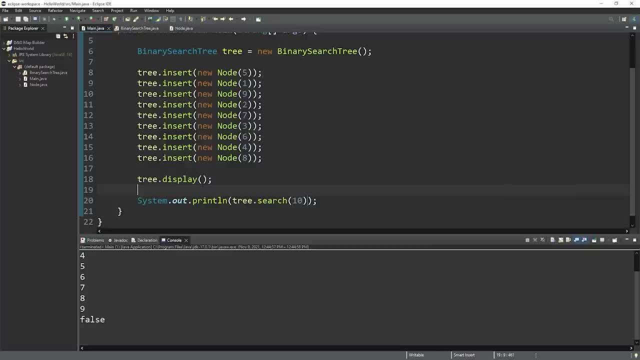 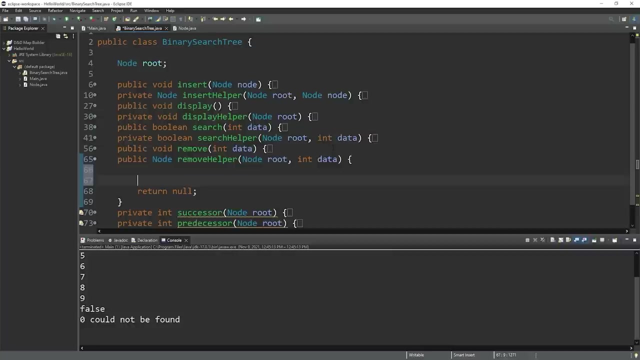 So just to test things real quick, I'm going to remove some data that doesn't exist. Tree dot: remove zero. Zero cannot be found. Now let's move on to the remove helper method. The first thing that we'll do is check to see if our root node is equal to null. 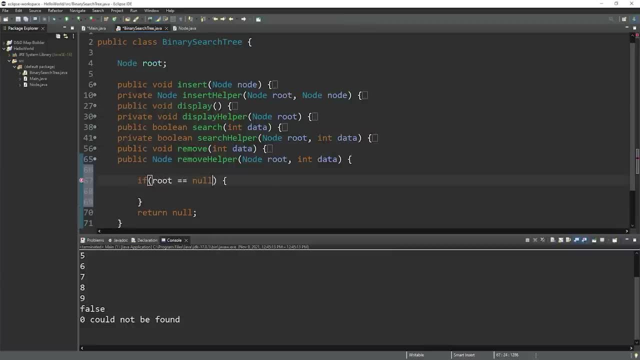 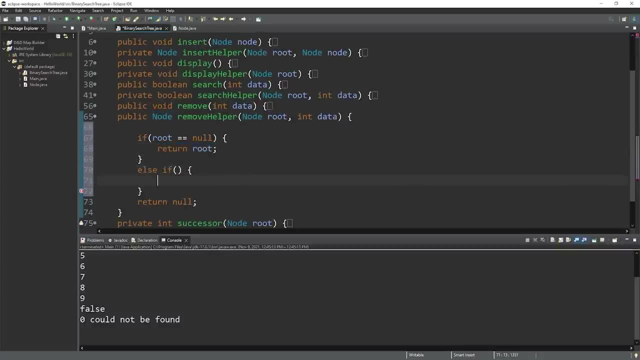 If our root node is equal to null, then let's return the root node. Then, within an else if statement, let's check to see if the data that we're trying to remove is less than the data of our root node. If it is, we need to go left down the binary tree. Root dot- left equals. 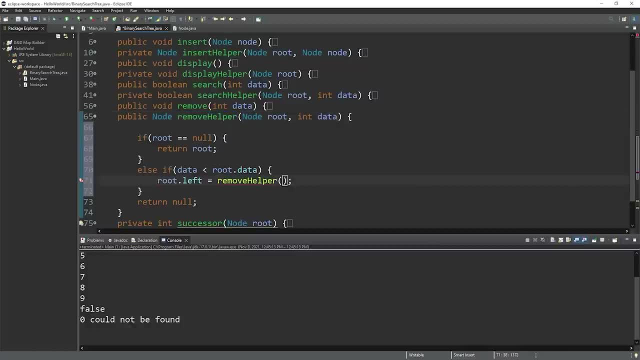 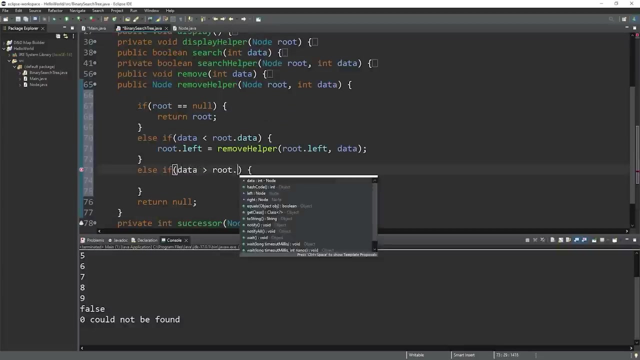 then invoke the remove helper method, Pass in the left child of the root node- root dot left- as well as our data. So we're going to go as far left as we can. Then add an else if statement, Else, if data is greater than the data of the root node, then we will go right. So let's copy this. 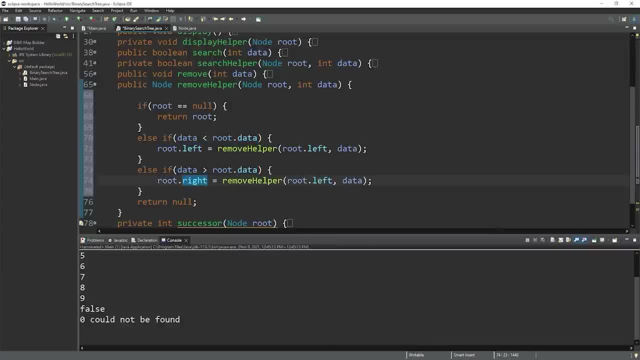 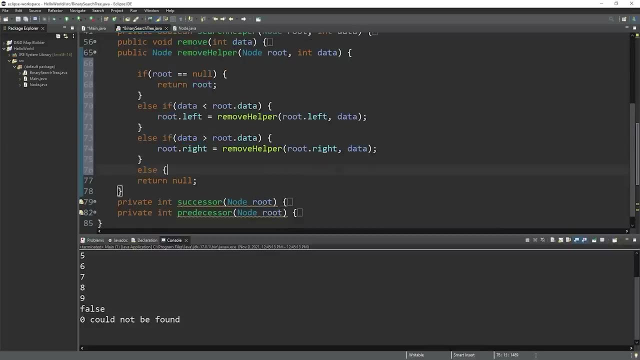 paste it. Root dot right equals remove helper. pass in root dot right as well as our data. Then add an else statement. If we reach the else statement, that means that we have found our node. And I'll just add a note to explain that If the node we're trying to remove has children, 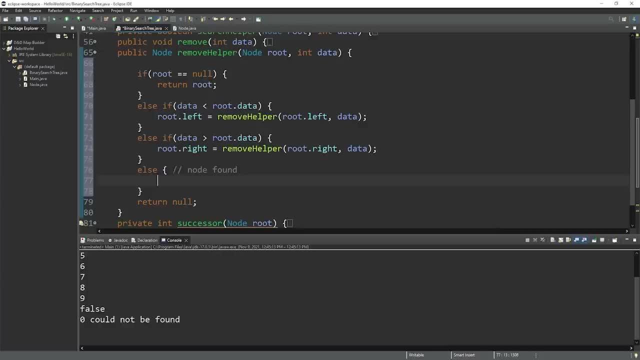 that kind of complicates things. then we have to shift the nodes a little bit. So we're going to shift the nodes around, But first let's check to see if it's a leaf node. Then that's really easy. Within an if statement we will check to see if the left child is equal to null. 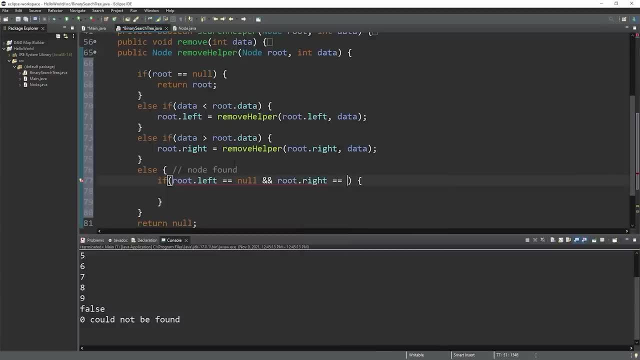 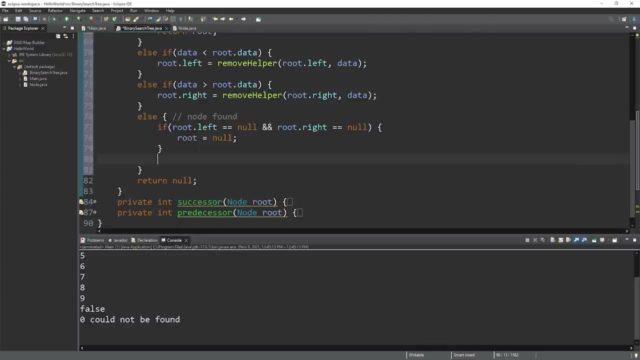 and the right child is also equal to null. That means that the node that we're trying to remove is a leaf node, And that's really simple. We don't need to shift any nodes around. We can just set this current root node equal to null. However, if the node we're attempting to 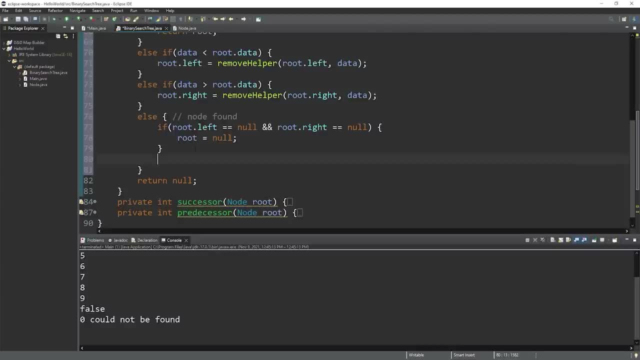 delete has a right child, we'll have to shift those nodes around and find a successor. Else, if root dot right does not equal null, that means there's a right child and we need to find a successor to replace this node. So we will assign root dot. data is equal to the successor method. 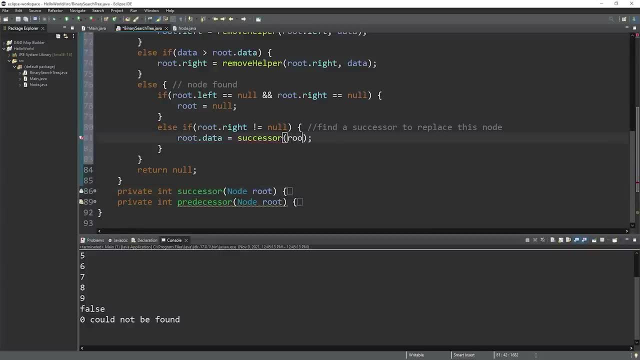 which will find a successor for us, and pass in the current root node. Then take rootwrite equals and invoke the remove helper method, Pass in the write child rootwrite as well as rootdata. So when we delete a node that will create a gap And if there's a child, well, we don't want that child to be lost. We don't. 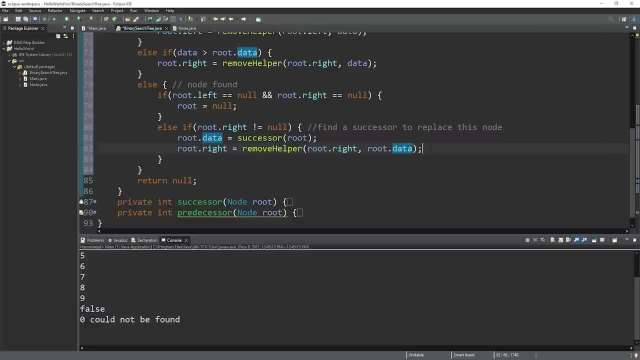 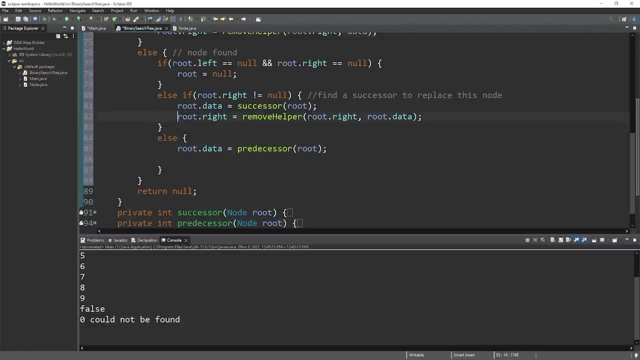 want that child to become an orphan, So we will link a child to that spot where we deleted a node. Now, if there's a left child, we have a slightly similar procedure, So we can use an else statement. Take rootdata and invoke the predecessor method. Take this line of code, paste it rootleft. 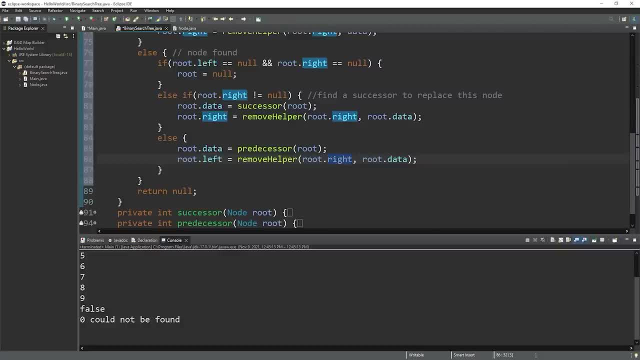 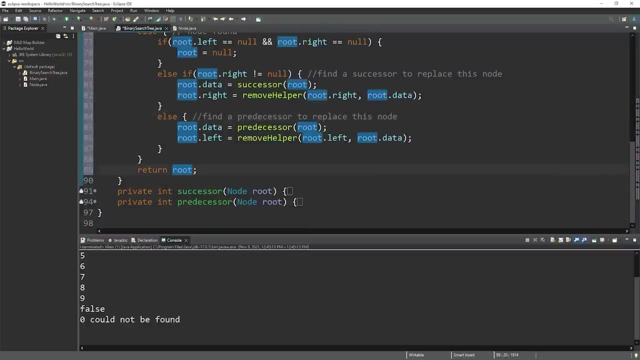 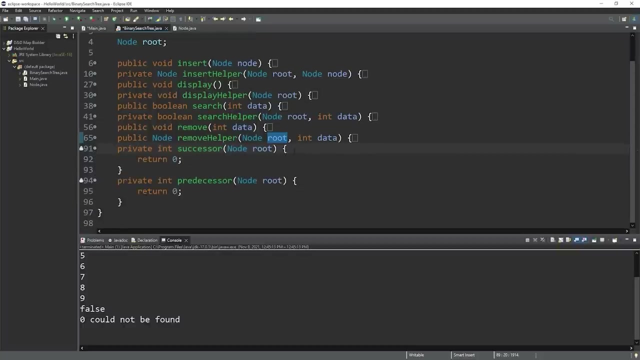 equals remove. helper method: Pass in the left child of the root node. This else statement will find a predecessor to replace this node And at the end we will return root. So we can close out of these two methods and we can open up the successor and predecessor methods. What we're doing with the successor method is that we're 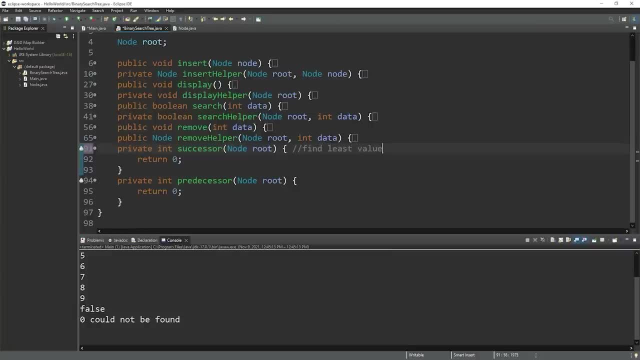 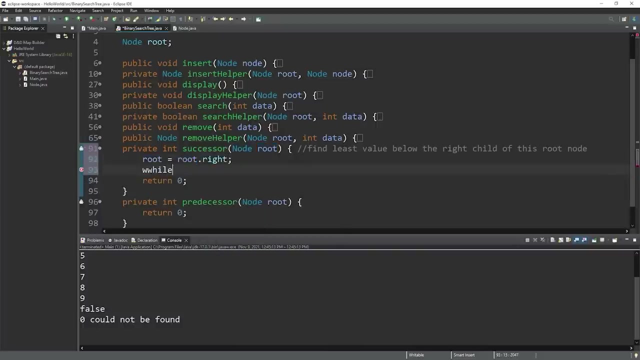 attempting to find the least value below the write child of this root node, We will assign the current root node equal to rootwrite. Then, within a while loop, we will take rootleft and check to see if it is not equal to null. While this condition is true, take root, set this equal to rootleft And, at the end, return. 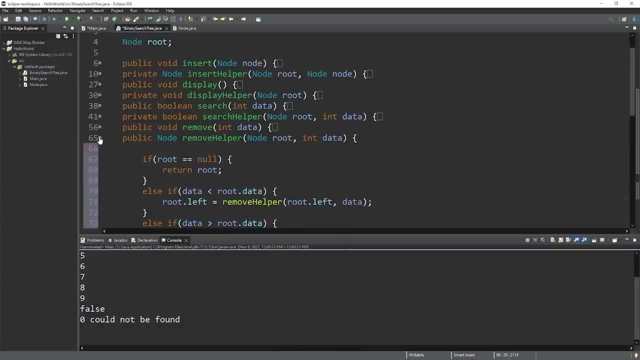 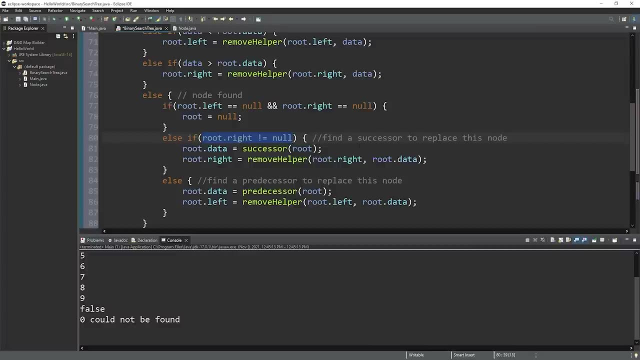 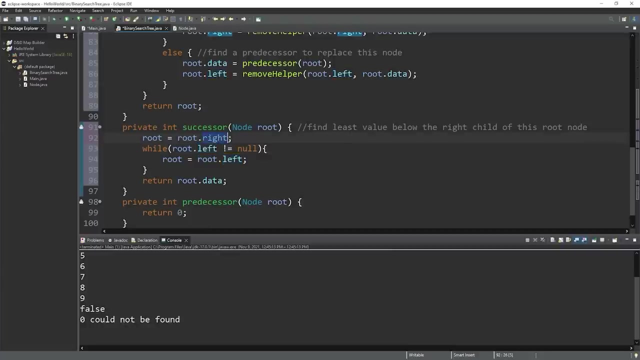 rootdata. So what's happening here? within the remove helper method, if the node we're trying to delete has a write child, we need to find a successor to fill in, And that successor should have the least value. So we will go right and look as far left as we can. 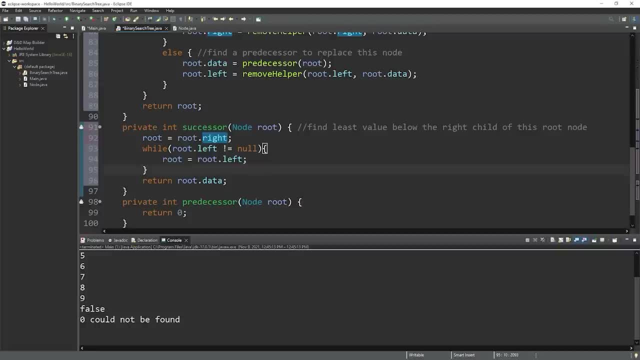 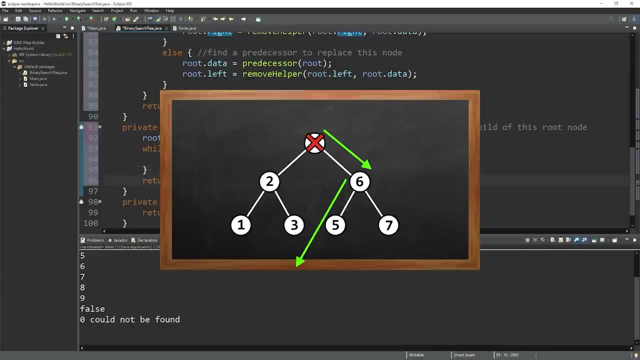 because values on the left are less than the root. Numbers on the right are greater than our root. After going right, we will go as far left as we can to get the lowest value, then return it. So that's what we're doing when we're assigning a successor to fill in that gap. when we delete a. 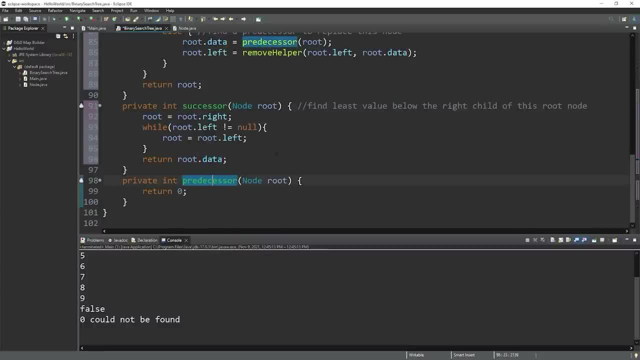 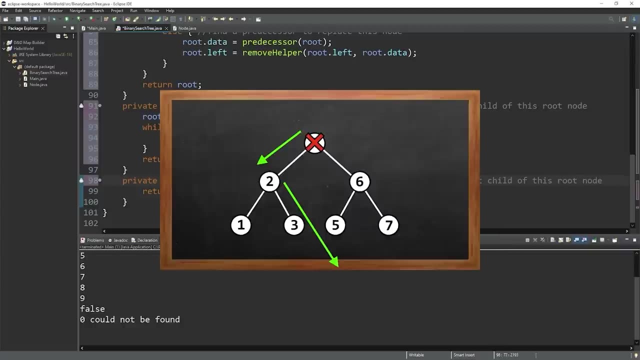 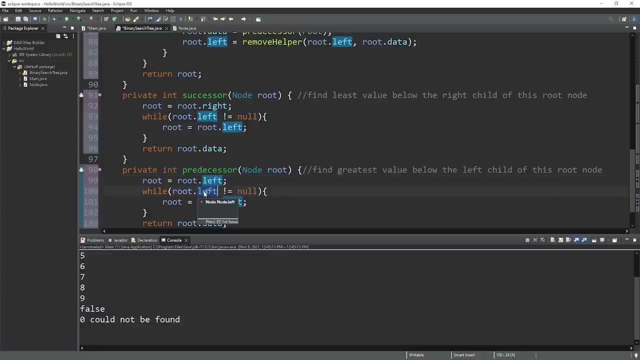 node that has children, And then the predecessor method is going to be very similar. We will find the greatest value below the left child of this root node. So we can copy all of this, paste it. This time we will go left, then go as far right as we can go. 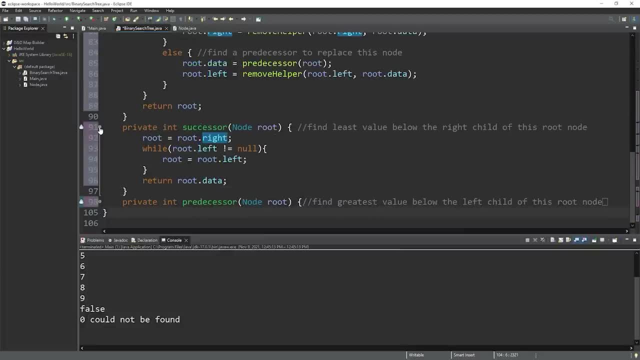 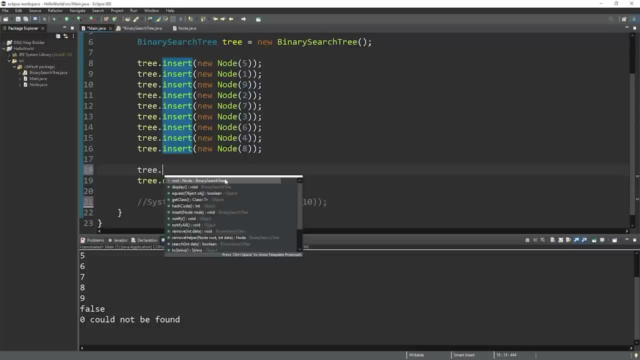 I do apologize. this is a lot to take in. Recursion can be very confusing. But yeah, that's everything. Let's attempt to remove a node. So before we display our tree, let's take treeremove and then pass in the data of a node you would like to remove. 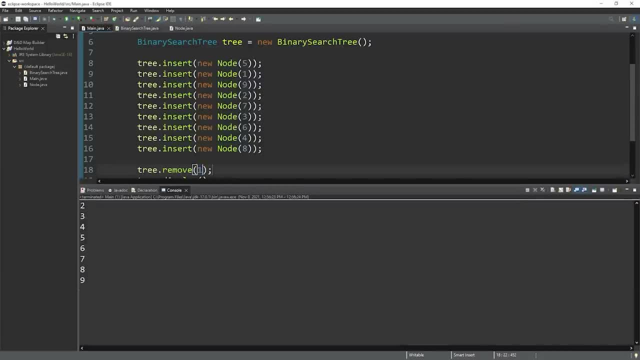 Let's remove a tree. Let's remove one, And here are the remaining nodes. We have two through nine, all in order. Let's remove five. Okay, one, two, three, four, six, seven, eight, nine. Let's remove nine. 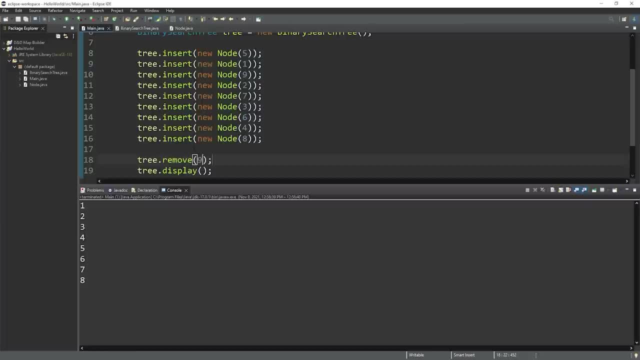 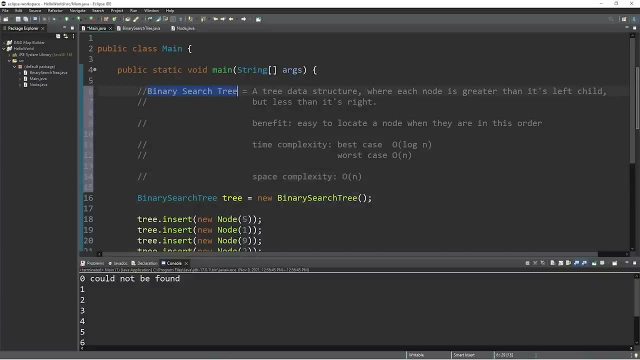 Nine is no longer there, And let's remove a node that is not within here. like zero, Zero cannot be found. All right, then everybody. that is a binary search tree. Just so you're aware. the order in which you insert nodes into a binary search tree does matter if it's. 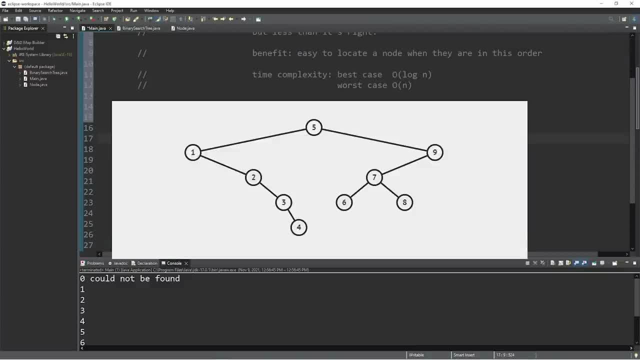 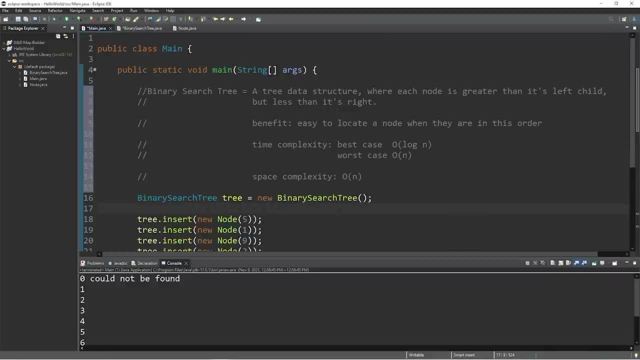 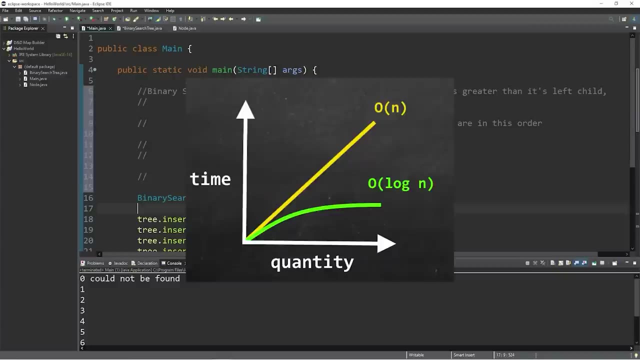 unbalanced. Technically, my tree follows all the rules. However, it's fairly lopsided. There is a way to balance binary trees, but that's a topic for AVL trees. That's why the runtime complexity has a best case scenario of big O of log n, but a worst case scenario of big O of n. 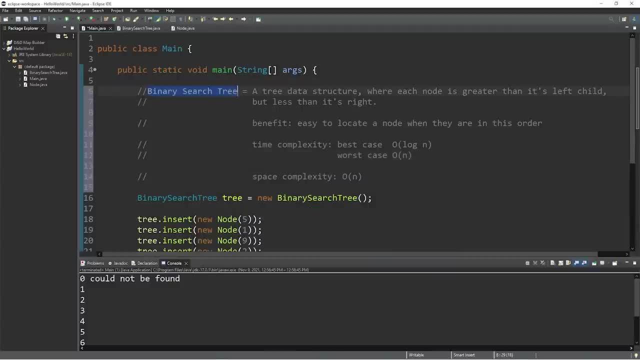 depending on how balanced it is. But basically, a binary search tree is a tree data structure where each node is greater than its left child but less than its right. The benefit of a binary search tree is that it's easy to locate a node when they are in order. So yeah, those are binary. 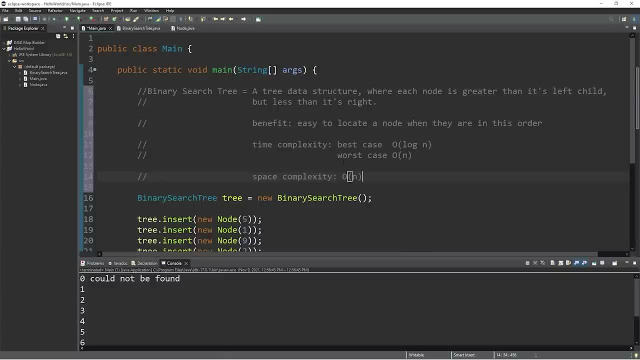 search trees. If you would like a copy of this code, I'll post this to the comments section down below. Don't be afraid to smash that like button, leave random comments down below and subscribe if you'd like to become a fellow bro. Hey, yeah, everybody. so let's talk about 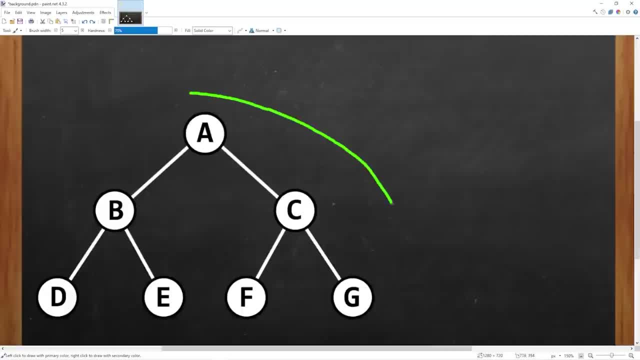 tree traversal. Tree traversal is the process of visiting all of the nodes of a tree. We don't have random access, so we begin at the root node and follow a certain procedure to visit all of the nodes of a tree, And there's three that we're going to talk about In order 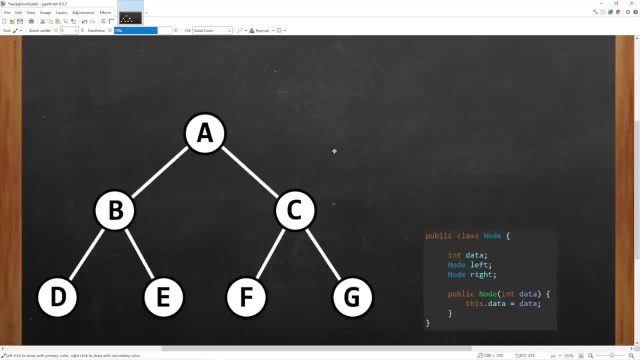 post order and pre-order traversal. In this example we will be working with a binary tree, not a binary search tree, because these values are not in binary search tree order. So each node has at most two children: a left node and a right node. Let's begin with an in. 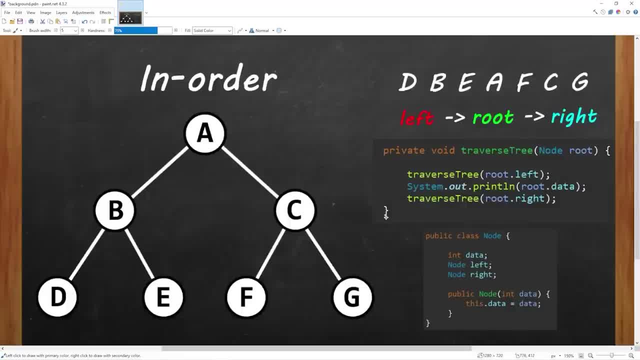 order traversal. Here's a recursive method that will navigate a tree in order. Using recursion, we visit as many left nodes as we can, followed by the root node and then any right nodes. The entry point is always the root and, using recursion, we will go as far left as we can. 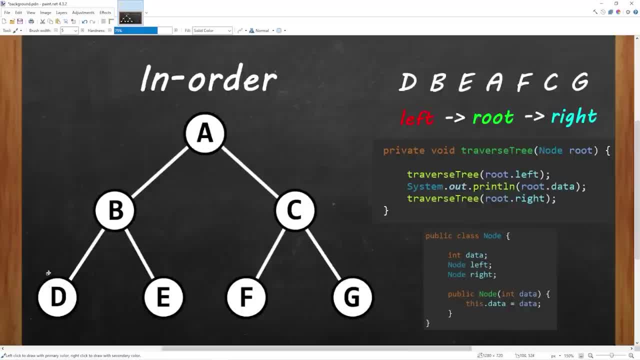 So we go from A to B to D, So we will mark this node as visited, then visit the root node next, and then the right node. Since we can't go left anymore, we're going to visit the root node A. All that's left is to go right. so we will go to C. 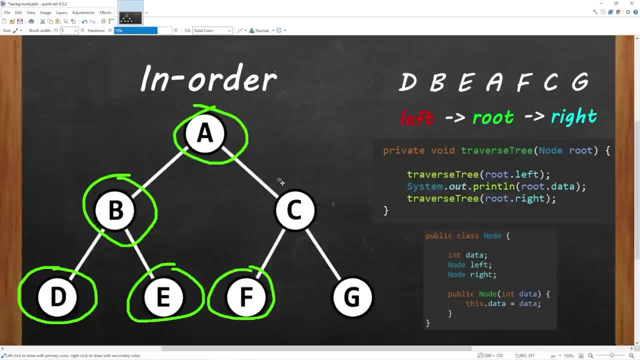 however, we can go left, so we will visit F first, then C, then G. So this is in order traversal When used in the context of a binary search tree. we will visit all of these nodes in non-decreasing order. So again, that was D, B, E, A, F, C, G. We go left. root right. 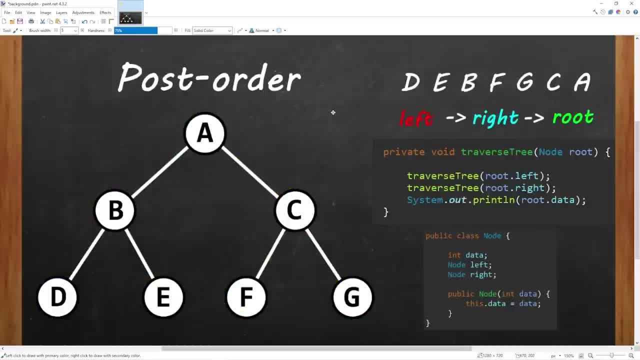 And here's that method again: Post-order traversal. It's used to delete a tree from leaf to root and we follow this pattern: Left, right, root. We will use recursion to visit the left children, then the right children, then the root. So A is our entry point. we are going as far left as we can Go from A to B to D. 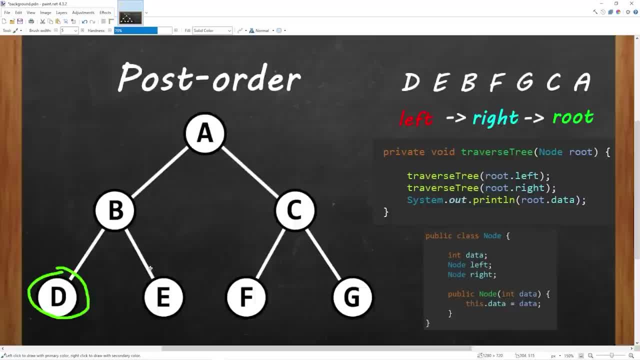 Mark D as visited. then we go right using recursion, Go from D to E, then root, Left, right root, So we go back up, go as far right as we can, unless we encounter a left child, which we did. 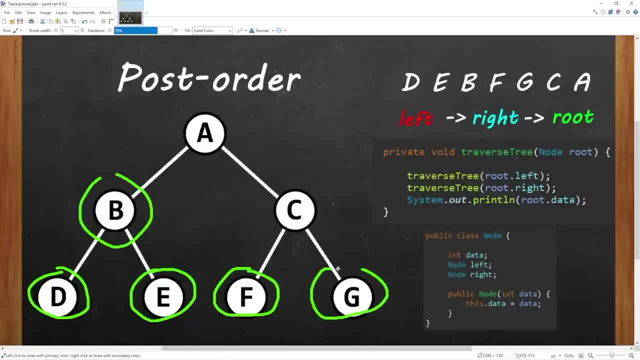 so we will mark F as visited, then G- right root, Left, right root, And all that's left is the root node. So that is post-order traversal. It's used to delete a tree from leaf to root. And lastly, we have pre-order traversal. Pre-order traversal is used to create a copy of a tree. 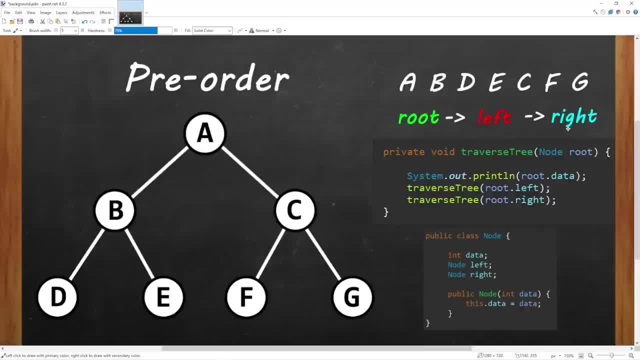 We visit any root nodes first, then left, then right. So we will mark A as visited, our entry point, then visit the left child and we will continue to go left, then go right. So we can't go left anymore, we're going to go right. 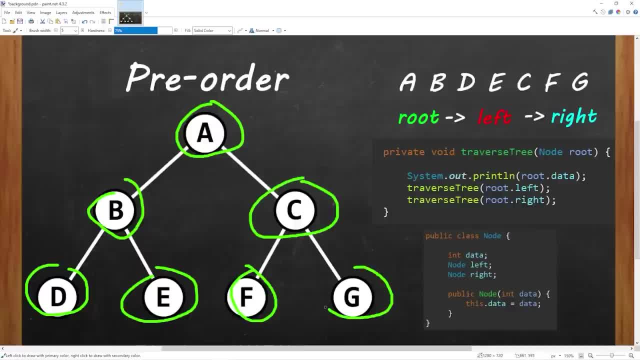 mark the root as visited, then left, then right. This is used to create a copy of a tree. but in order to create a copy of a tree you need to create a root node and a branch node to hold the leaves. So again, that's. 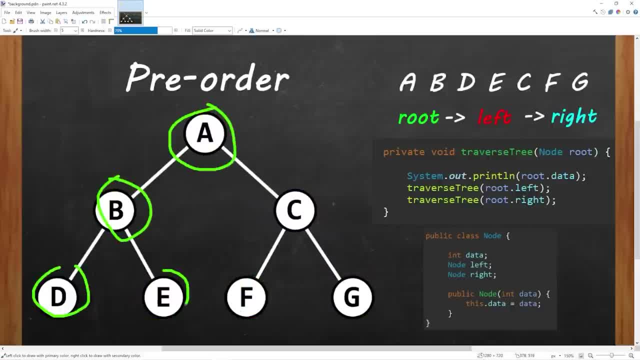 root left. we're still going left, right root left, right, A, B, D, E, C, F, G. That is pre-order traversal. It's used to create a copy of a tree. Well, okay then, everybody. 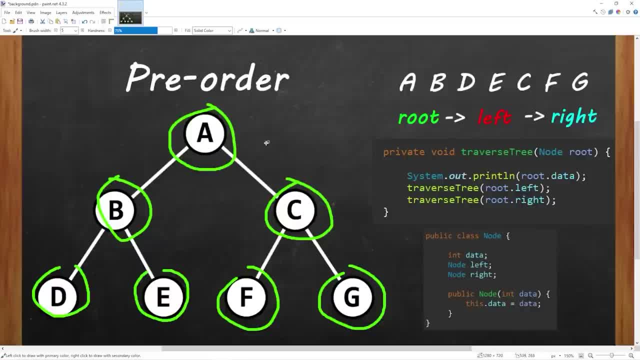 that is a few ways in which we can traverse a tree. Like I said, normally we don't have random access, so the entry point is the root node and you can either follow an in-order, post-order or pre-order traversal, depending on what you need to do with this tree. 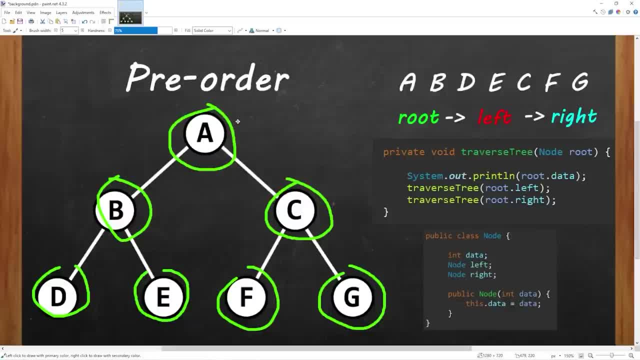 So that's tree traversal in computer science. If you liked this video, please be sure to give it a thumbs up, leave a random comment down below and subscribe if you'd like to become a fellow bro. Hey everybody, in this video I thought I would show you all how you can get the runtime of a 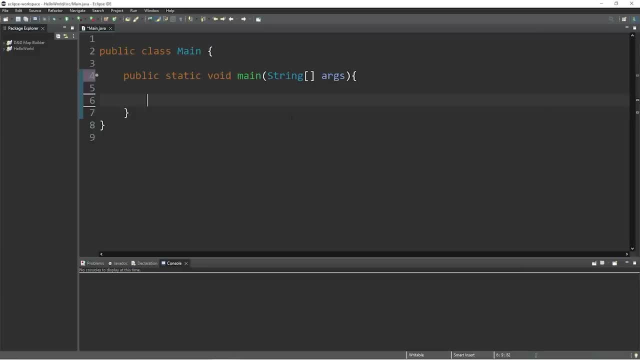 program. I thought it might be useful now that we know how data structures and algorithms work for the most part. So within the entry point of your program you'll need the start time and we'll store this within a long data type. I'll name this. start equals then type system dot nano time. 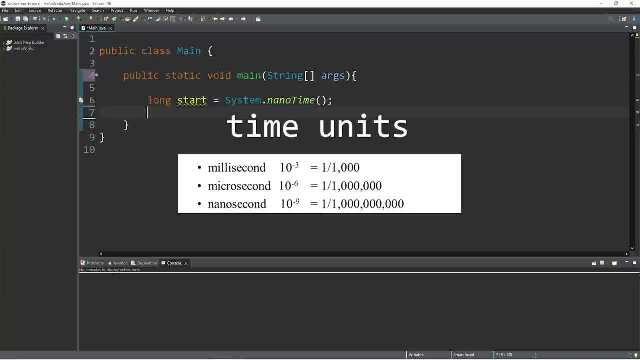 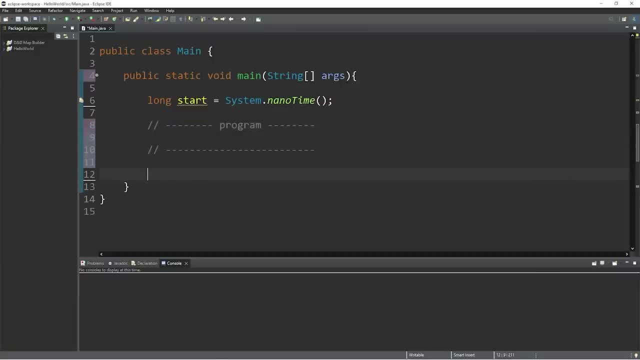 A nanosecond is a billionth of a second. And then we have our program, Whatever it is, And then at the end of our program we will get the duration. This will be of the long data type Duration equals. and then we need the current time System, dot nano time. 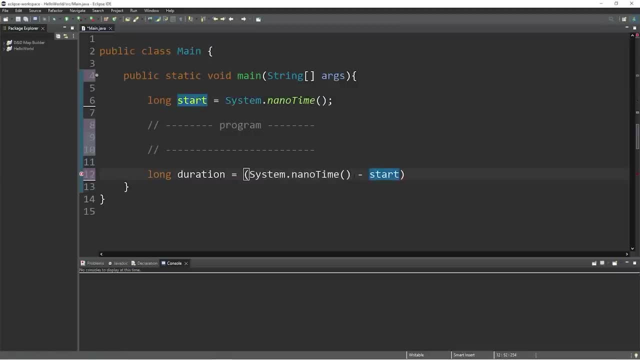 minus our start time. This returns a time in nanoseconds. If you need milliseconds, you can divide this number by 1 million. Okay, then let's print the duration System dot out, dot print line: Duration plus milliseconds or some other unit to measure time. Okay, so with our program.